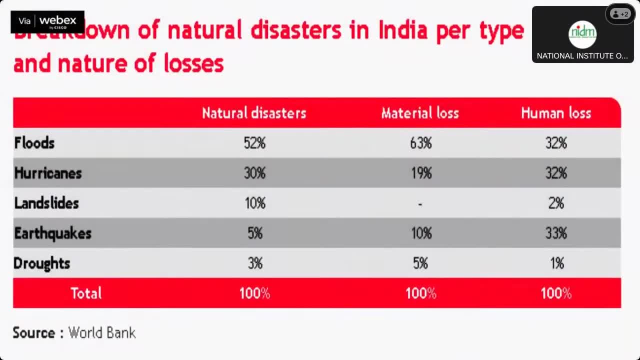 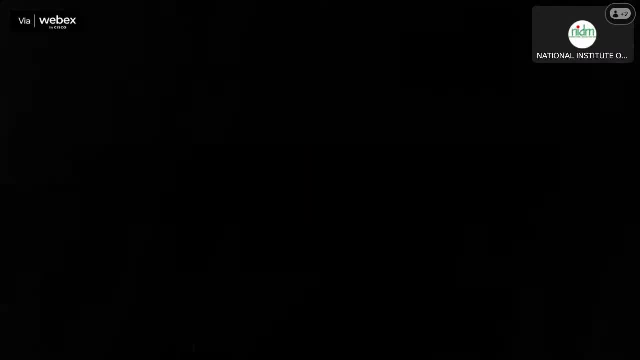 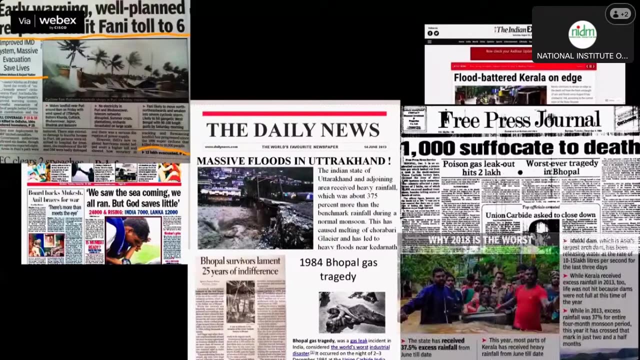 of these calamities and suffer heavy due to their detrimental impacts. Disasters also disrupt development, leading to a slowdown in the economic growth rate. Therefore, to be able to achieve the desired targets of Sustainable Developmental Goals- SDGs- progress should remain resilient. 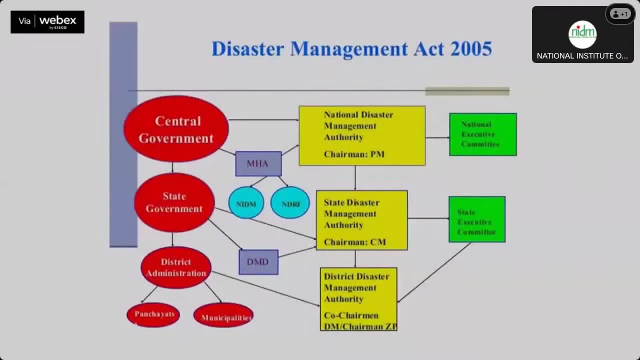 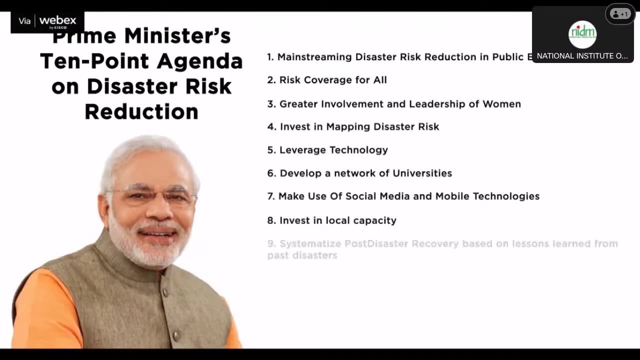 and uninterrupted. The DM Act 2005,. along with the Prime Minister's 10-point Agenda on Disaster Risk Management, DRM realm calls for integrating the principles of disaster risk reduction across all developmental sectors. Also the Sendai Framework for Disaster Risk Reduction. 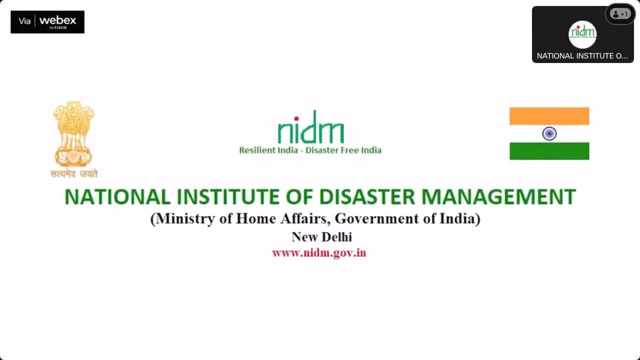 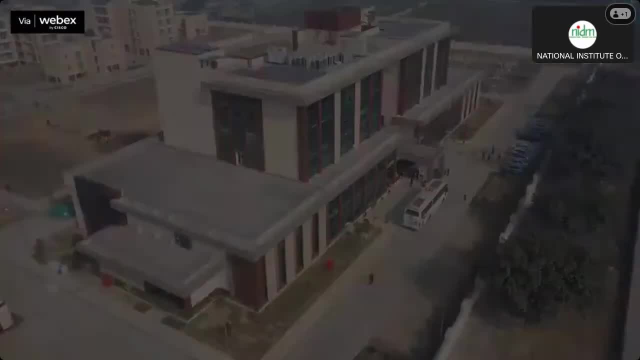 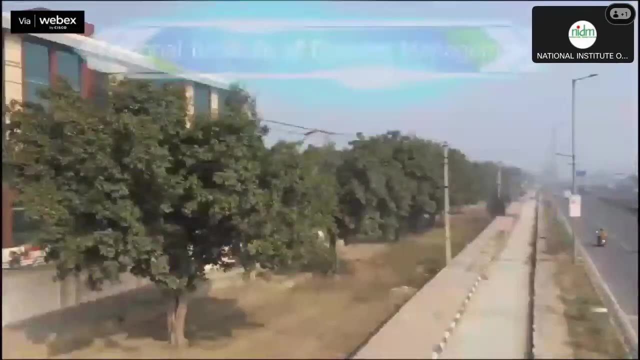 or DRR, to which India is a signatory. under its four priorities and seven targets, focuses on building economic resilience and promote ease of living. With this aim of making our nation disaster resilient, the National Institute of Disaster Management was established on 11 August 2004 at New Delhi. 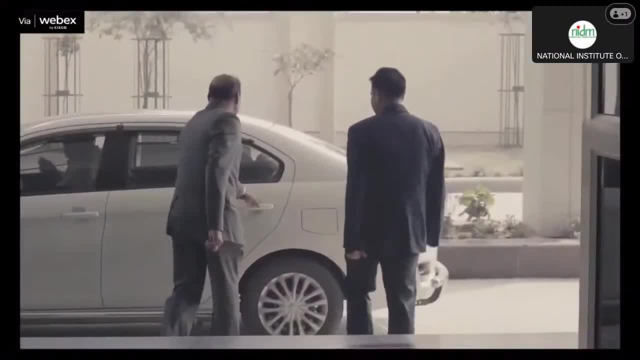 with the responsibilities for human resource development, capacity building, training, research, documentation and research and capacity building, training, research, documentation and research and capacity building. training, research, documentation and research and policy advocacy in the field of disaster management. 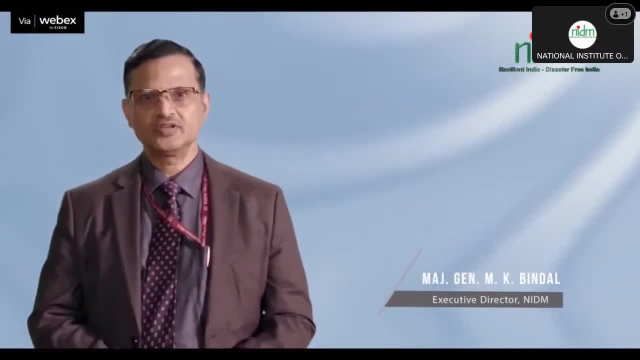 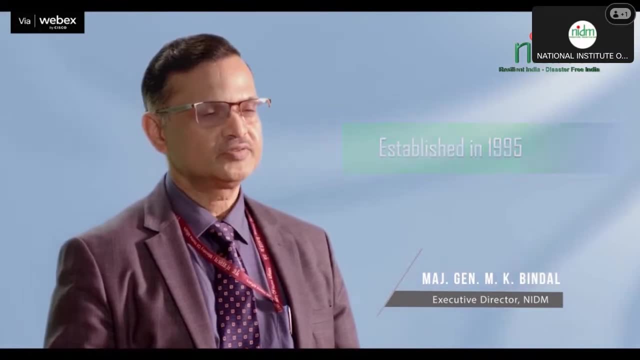 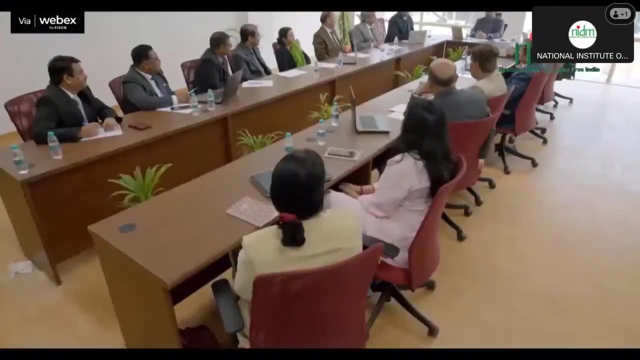 and policy advocacy in the field of disaster management. In the backdrop of the international decade for natural disaster reduction, a National Centre for Disaster Management was established in 1995 in the India Institute of Public Administration by Ministry of Agriculture and Cooperation. The centre gained impetus. 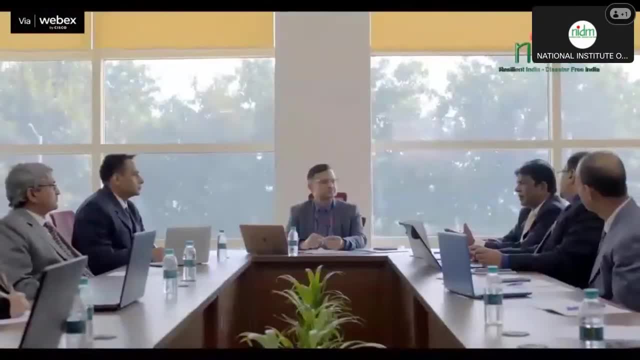 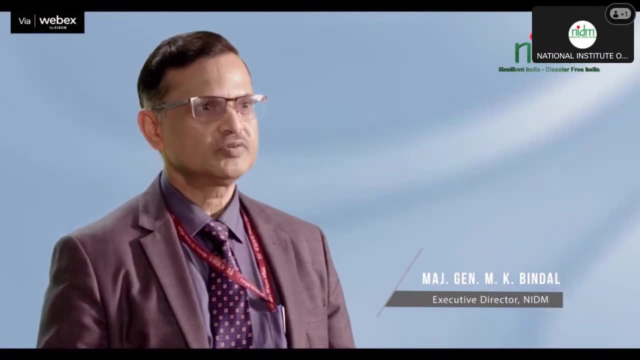 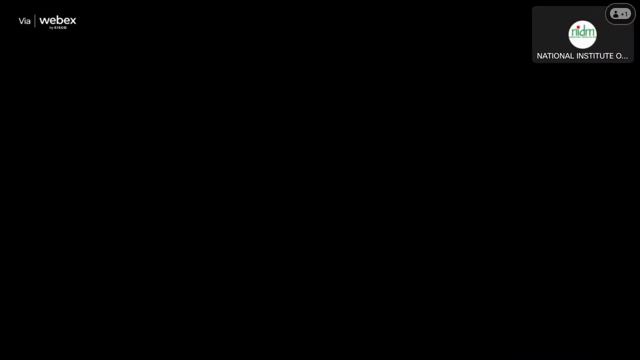 with its redesignation as National Institute of Disaster Management under Ministry of Home Affairs. under Ministry of Home Affairs, which was constituted under the Disaster Management Act 2005 as a premier institute for training and capacity building for disaster management, The campus of the National Institute of Disaster Management. 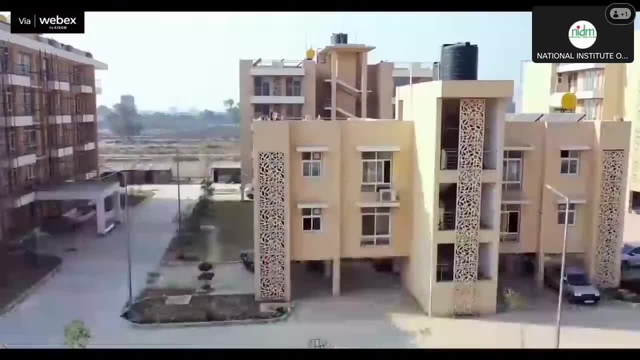 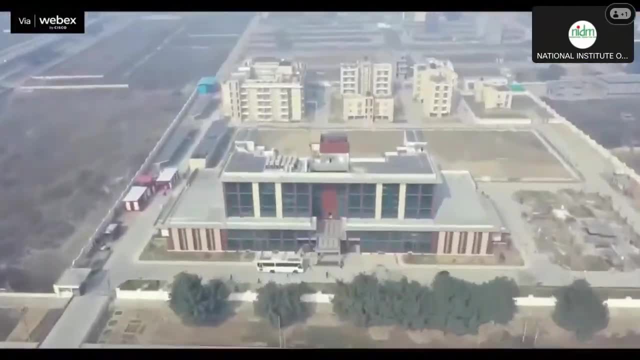 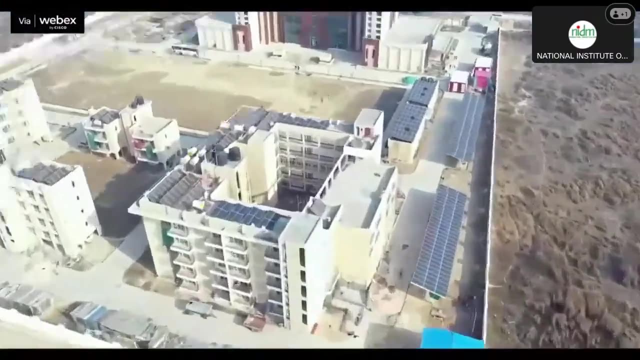 spreads across seven acres. This campus has been constructed with modern technologies, following latest and green building norms. State-of-the-art infrastructure facilities has been provisioned for the faculty members, staff and researchers who can work in a highly conducive environment to achieve the vision of NIDM. 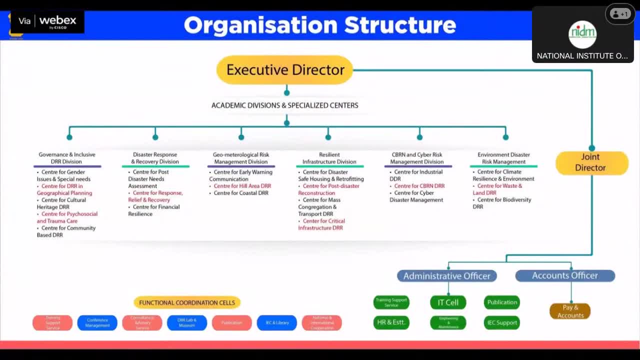 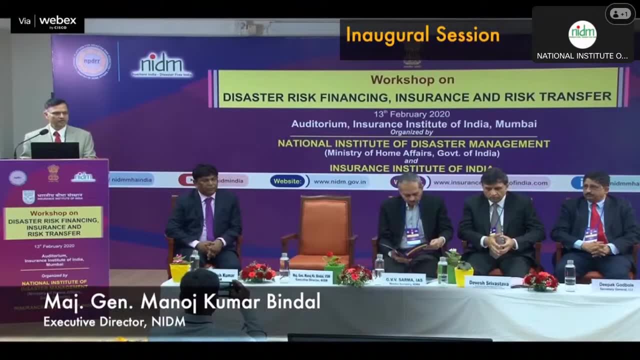 Executive Director of the institute, who is also the member secretary of the institute and its governing body, runs the day-to-day administration of the institute. runs the day-to-day administration of the institute. NIDM has total 86 sanction posts. 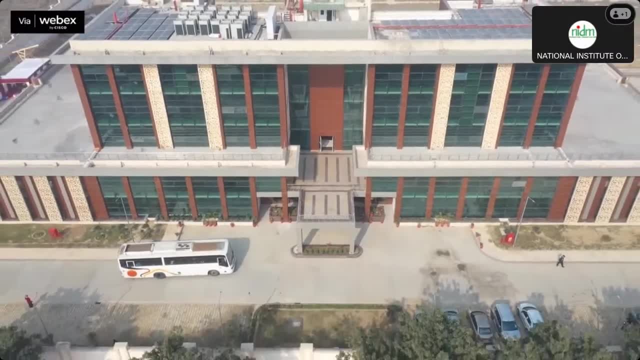 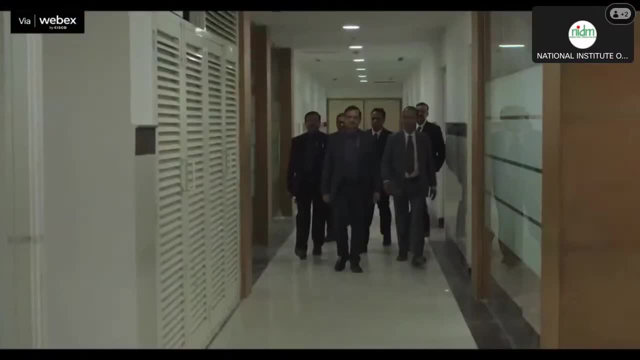 NIDM has total 86 sanction posts- 57 for New Delhi campus and 29 for Southern campus. To make the country a resilient nation. To make the country a resilient nation, highly dedicated and proficient NIDM team. highly dedicated and proficient NIDM team. 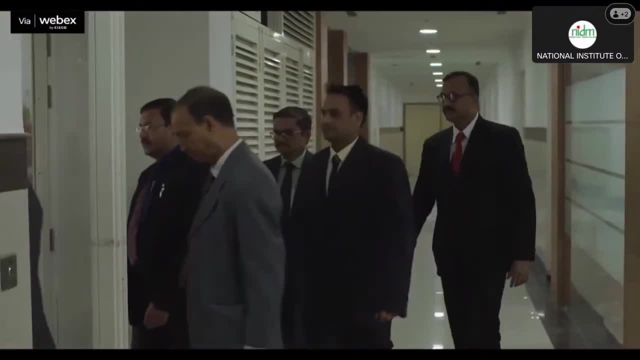 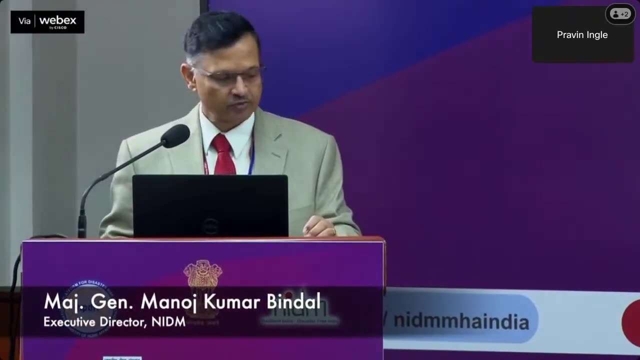 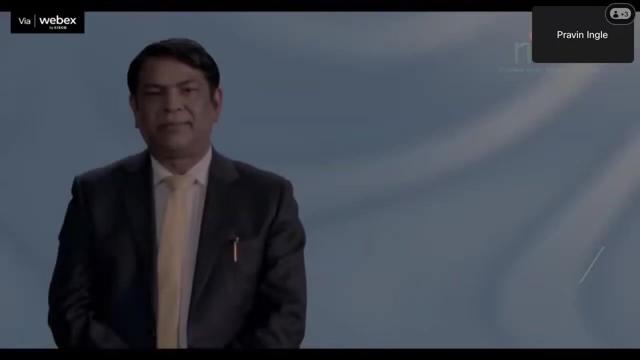 that has been selected constitutionally work relentlessly along with the executive director, British civil medal recipient, Major General Manoj Kumar Pindal, to achieve the mission of resilient and disaster free India. NIDM is engaged in international. NIDM is engaged in international capacity building process too. 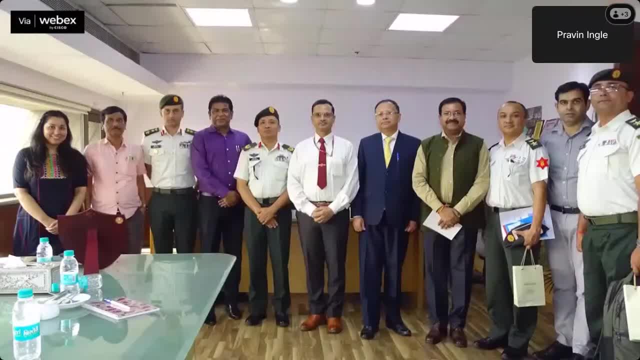 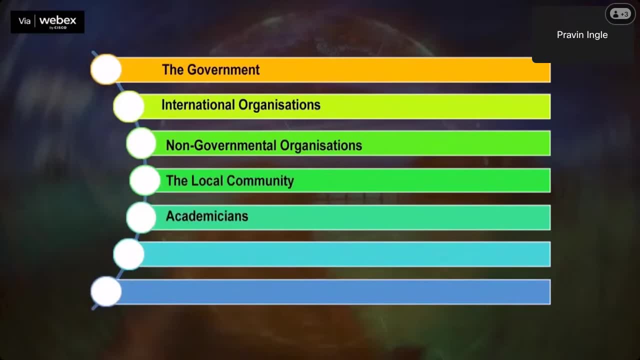 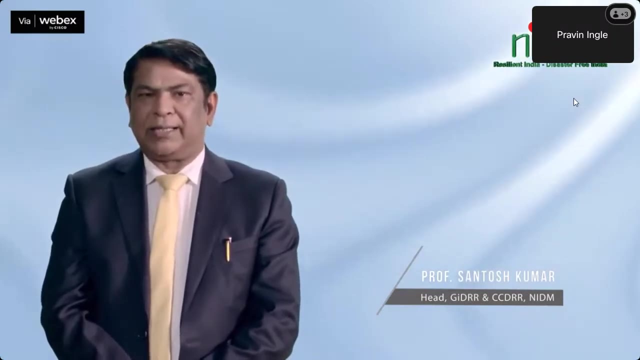 International cooperation is one of the. International cooperation is one of the and most important mandates for building resilience. where we have been engaged on a regular basis, Inclusive DRR with leaving no one behind is our motto. Establishment of child-centric DRR Center for Gender Studies. 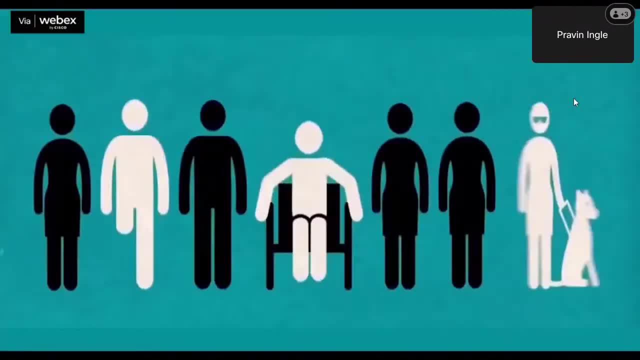 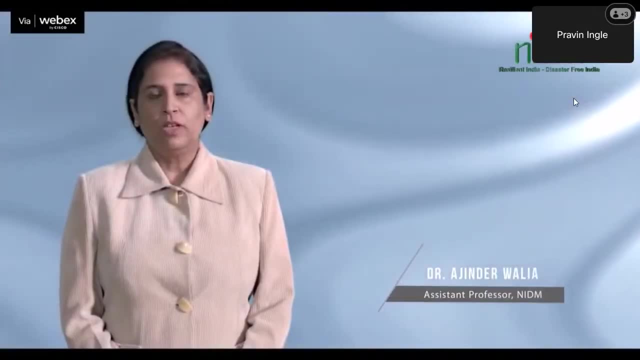 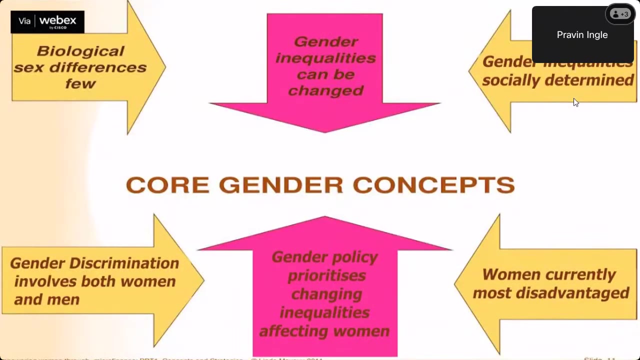 and special focus on persons with different abilities are the key interventions in this regard. NIDM is committed to the agenda of mainstreaming gender in disaster risk reduction. The institute maintains a strong focus on integrating gender concerns in the disaster management cycle. For this, capacity building programs are run exclusively on the issue. 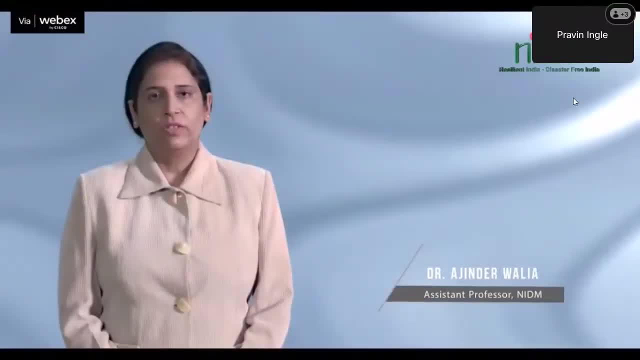 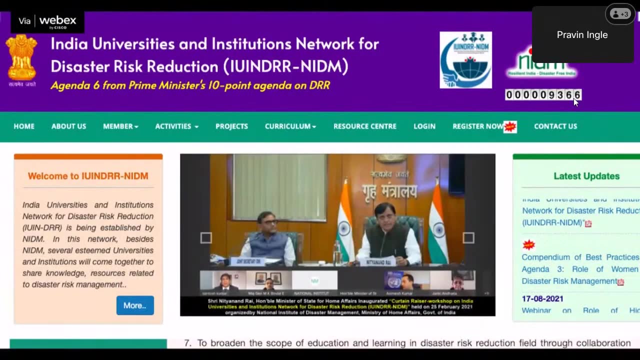 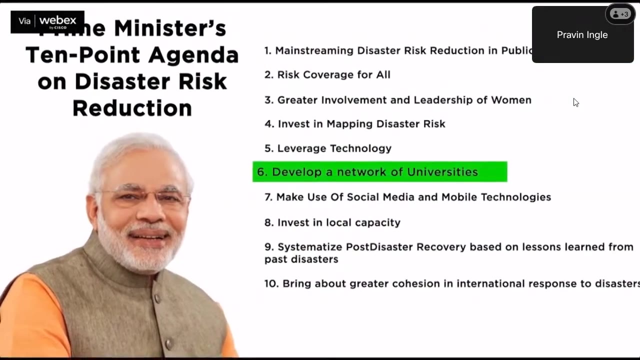 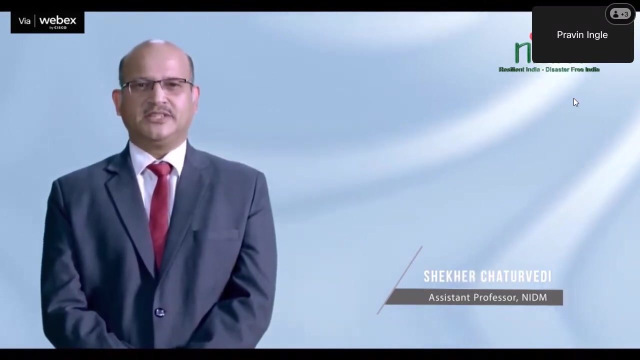 along with including it as a cross-cutting issue in other initiatives. NIDM has established India Universities and Institutions Network for Disaster Risk Reduction to address the Agenda 6, a top 10-point agenda for DRR of Honorable PM, which stresses on the need to develop a network of universities to work on disaster issues in India. 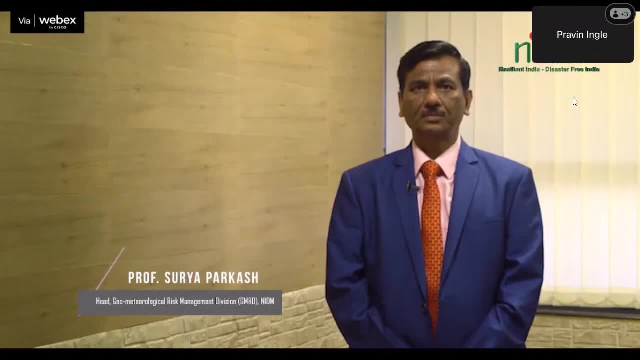 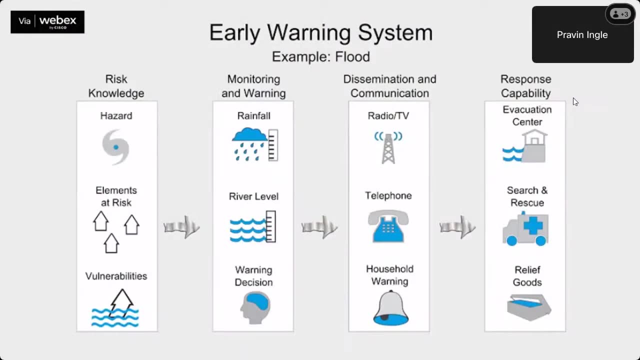 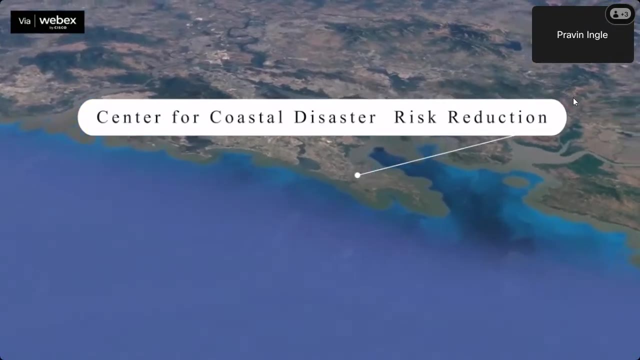 NIDM has a Geometriological Risk Management Division that hosts three specialized centers: Center for Early Warning and Communication, Center for Hill Area Development and Center for Coastal Disaster Risk Reduction and RAGILEAS. In NIDM we are committed to developing a network of universities to work on disaster issues in India. 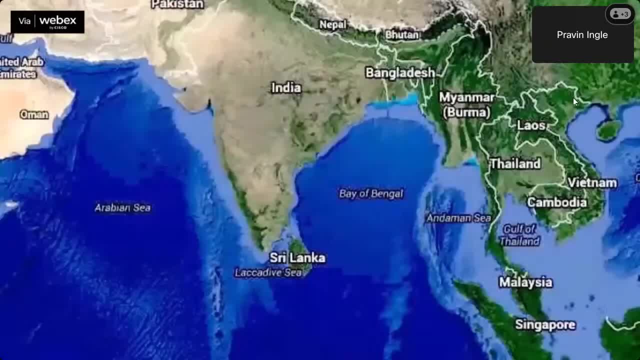 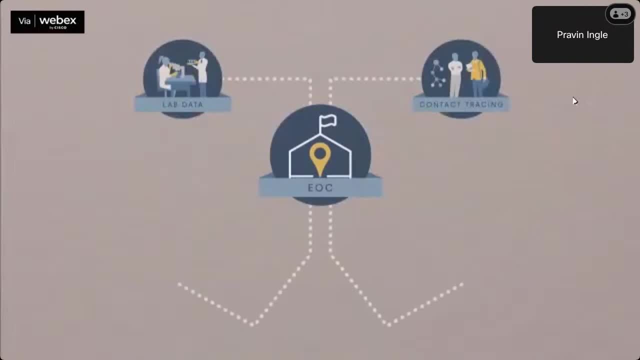 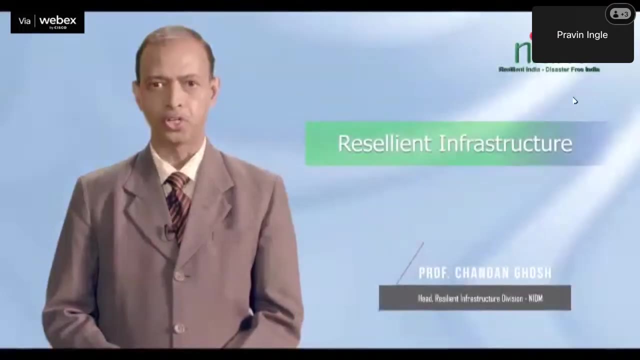 In this generation. it has three more centers: one center for flood monitoring, the second one on Emergency Operations Center and the third one is World Center of Excellence on Landslide Disaster Reduction. Resilient Infrastructure Division of the institute caters to training and capacity building. 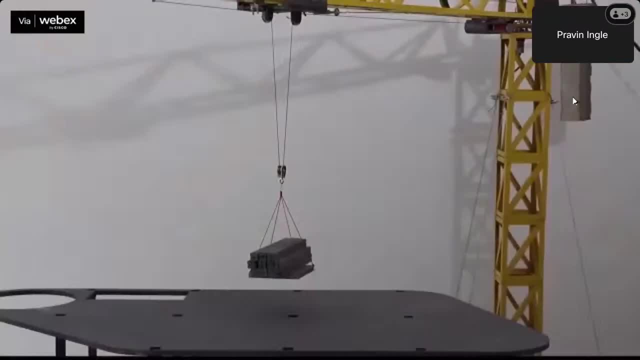 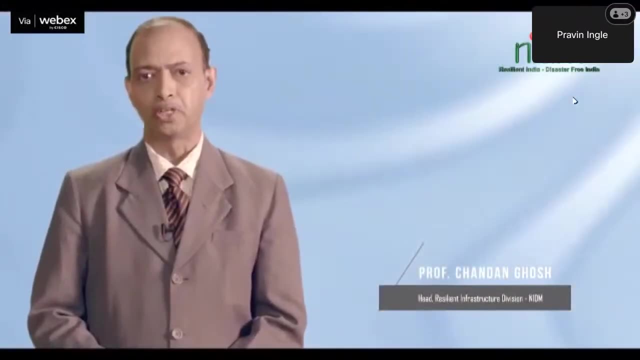 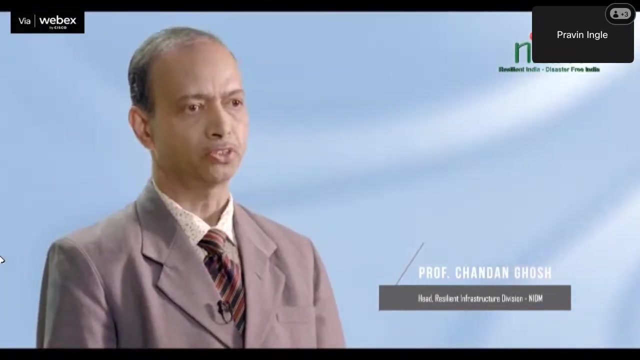 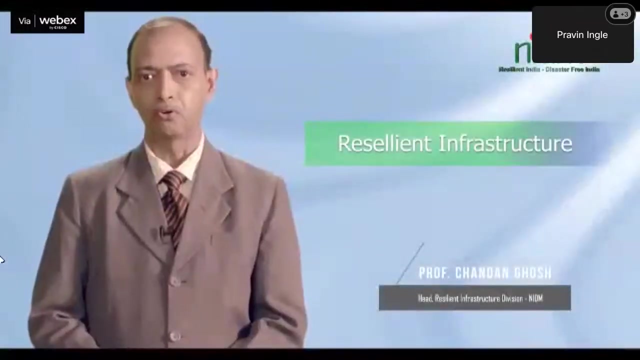 of the engineers, architects and town planners of the country serving various line departments, as for example municipalities, PWD, PHE, rural engineering, towards the vulnerability standards, documenting disaster-affected sites for reconstructions and implementing all the things under National Building Code developed by Bureau of Indian Standards. 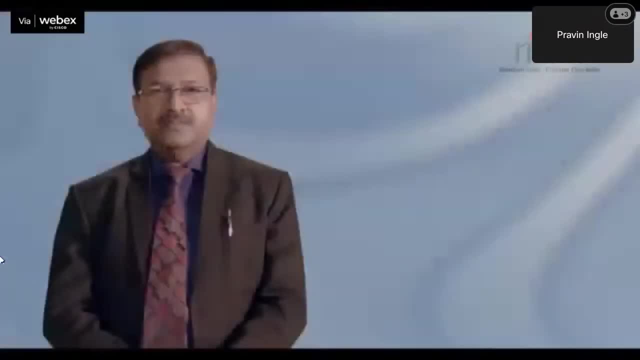 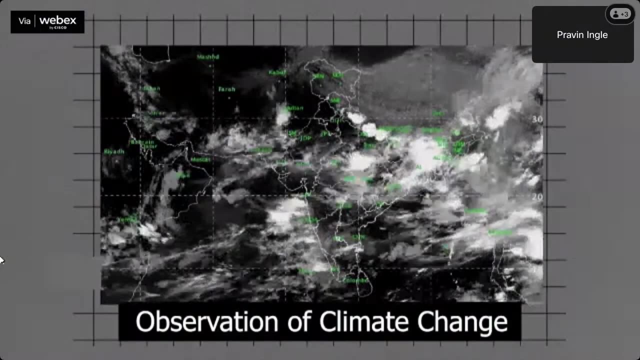 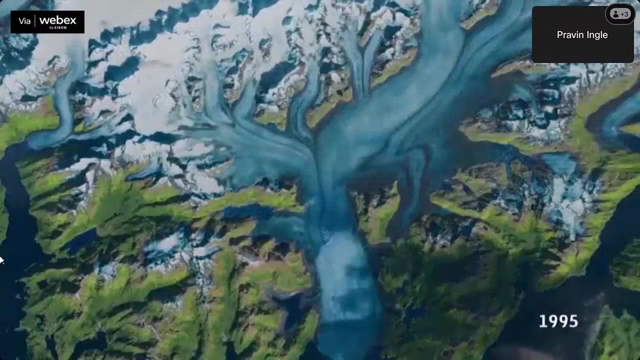 NIDM, since its inception, has considered climate change, disasters and extremes at the fore of its research policy and training agenda. At NIDM, we focused on environmental changes as a key driver of risk. that includes not only climate change. 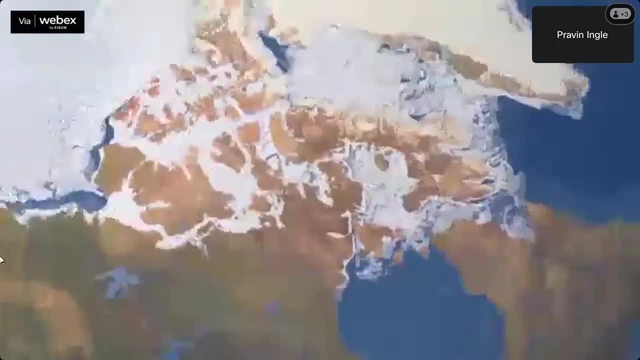 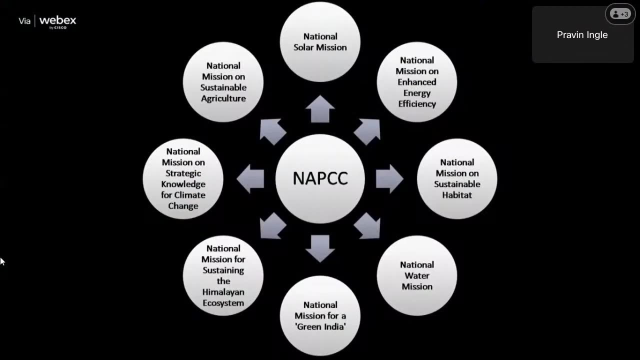 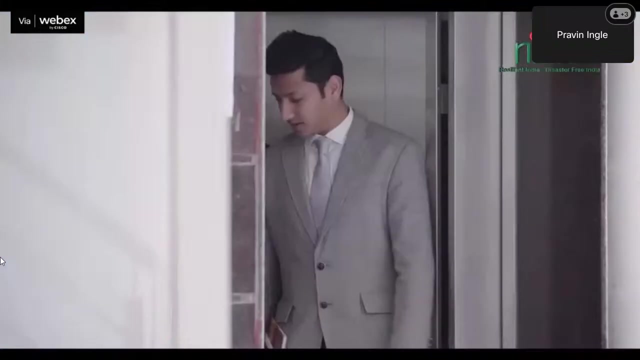 but also the attributes like land use, landscape and natural resource degradation. We host a Center of Excellence on Climate Resilience under the National Action Plan on Climate Change. NIDM provides year-round internships and dissertation opportunities for students pursuing masters and higher studies. 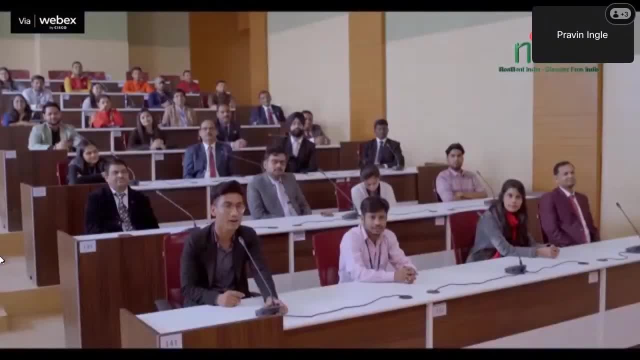 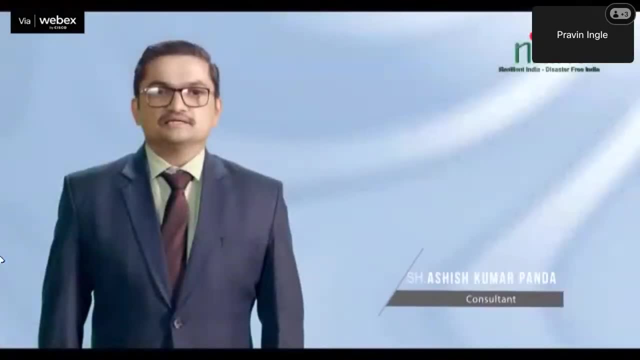 from various disciplines across India Under the mentorship of NIDM faculty members. Forestry, biodiversity and animal-inclusive disaster risk reduction section of the ECDRM Division of NIDM is basically concerned with imparting training and enhancing capacity building. 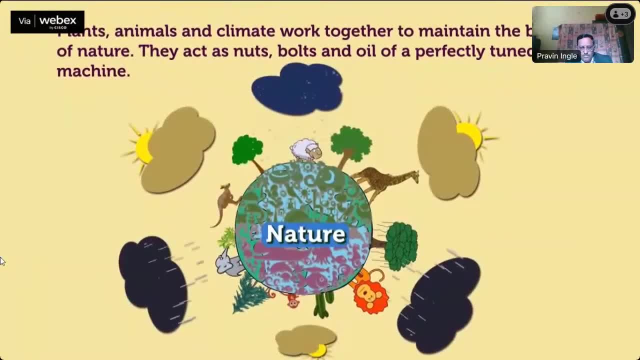 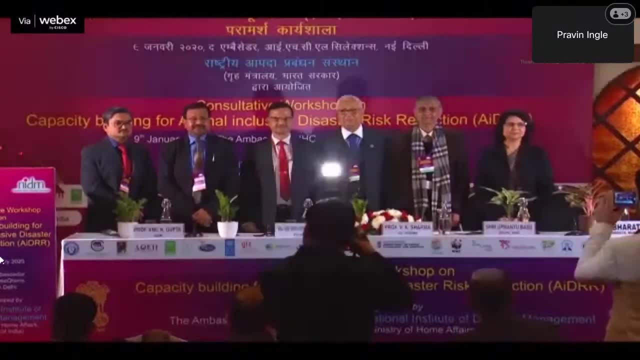 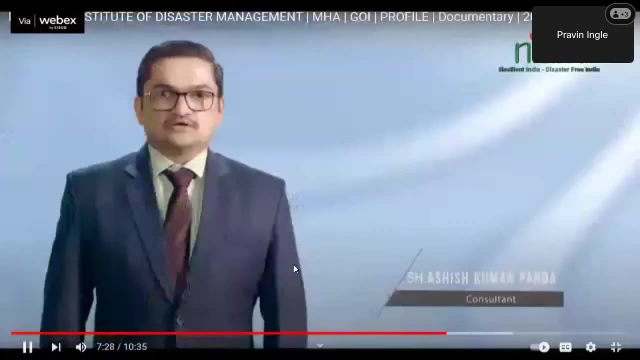 in the areas of forest conservation, forest fire management, agroforestry, conservation of biodiversity, mitigation measures to lessen the threats to it. associated global and national acts, regulations, policies, nature-based solutions for climate crisis and its impact on the three segments of forestry biodiversity. 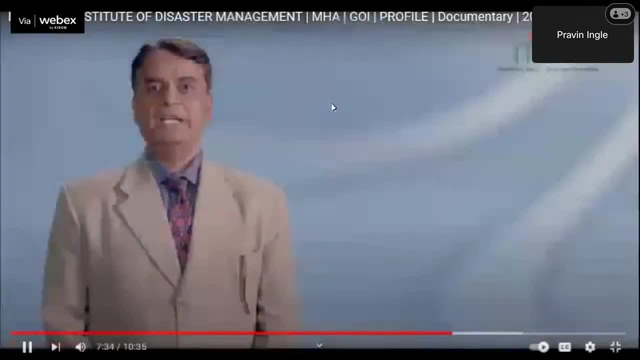 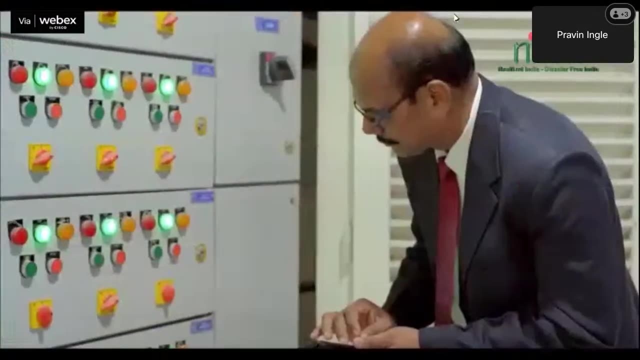 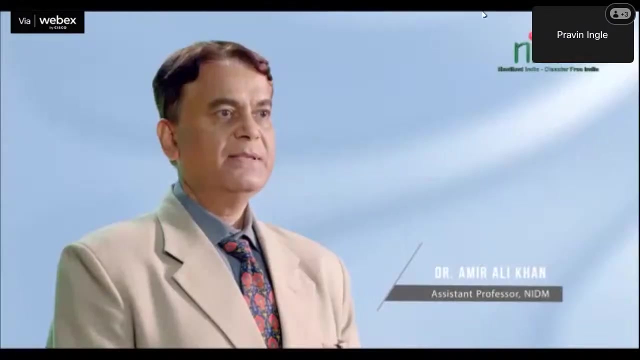 and animal-inclusive disaster risk reduction. NIDM is building capacity of stakeholders like engineers, architects and urban planners for making urban development as resilient development and to make cities disaster safe. NIDM is also helping various cities in developing disaster management plans of urban areas. 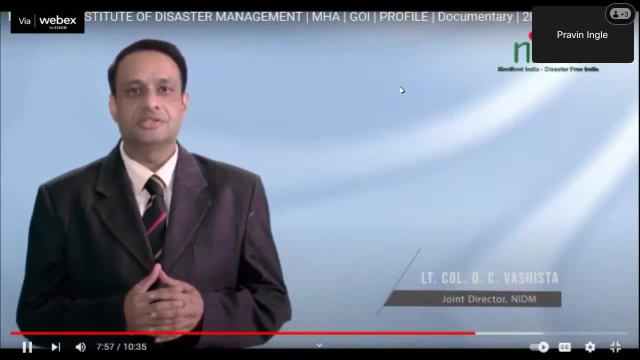 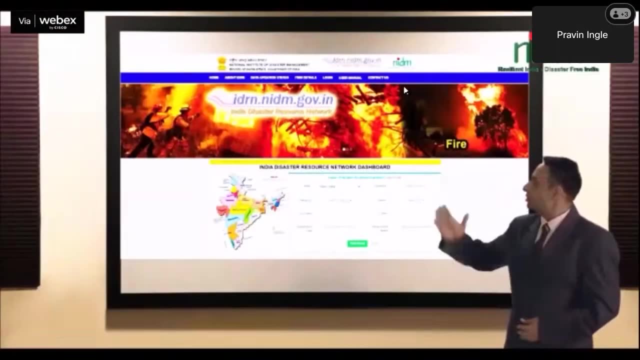 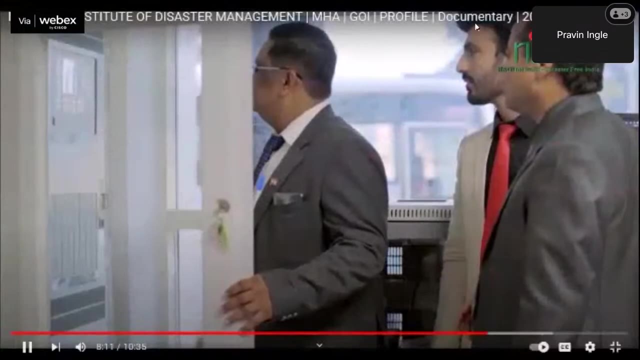 India Disaster Resource Network is a web-based platform for managing the inventory of equipment, skilled human resources and critical supplies for emergency response. NIDM campus is equipped with latest IT infrastructure, including internet, leased line Wi-Fi connectivity, CCTV surveillance, latest office equipment, IT-enabled training halls. 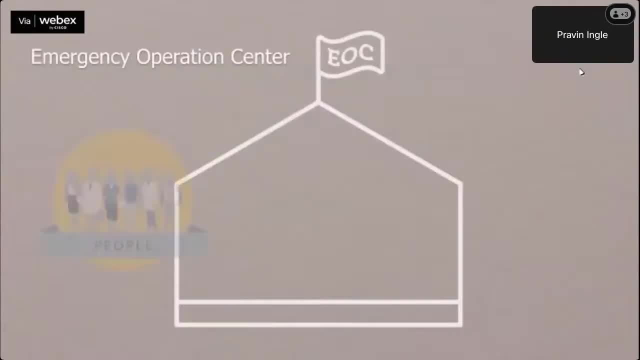 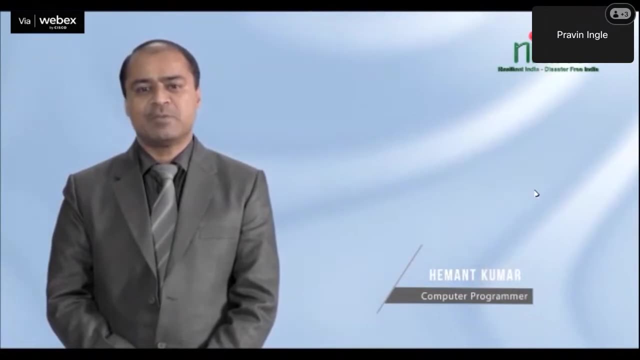 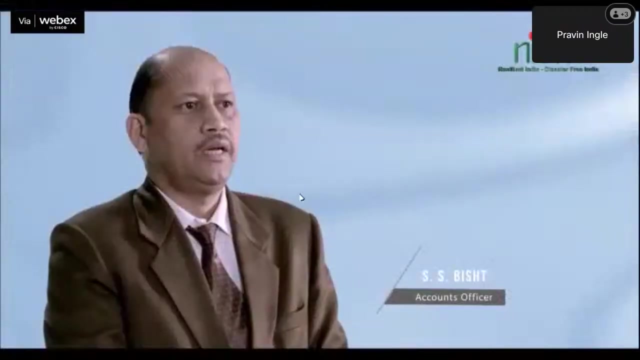 video conferencing tools, emergency operations center, etc. Even during the COVID-19 pandemic, NIDM continued its capacity building activities with the help of latest e-learning tools. NIDM receives 100% grant from Ministry of Home Affairs. Recently, NIDM has established its two campuses. 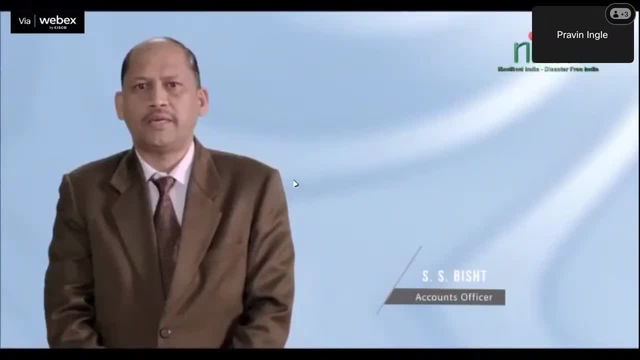 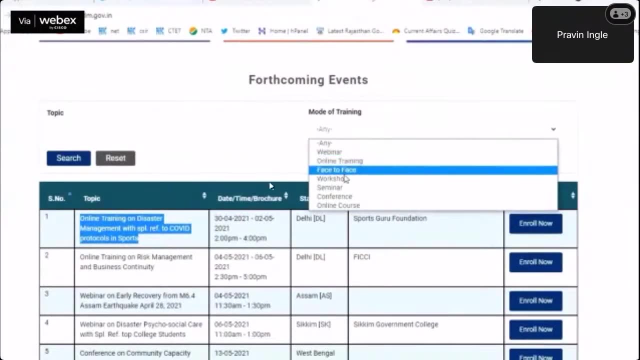 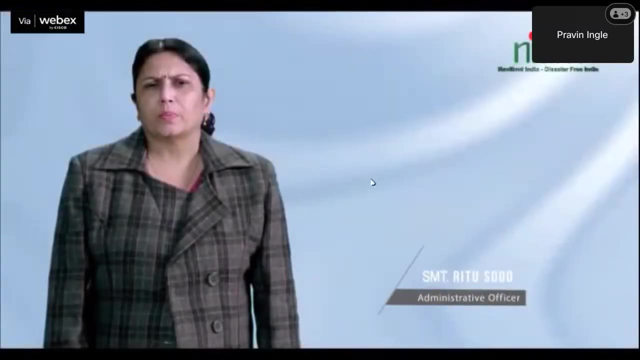 at Kohang, Delhi and Southern Campus at Krishna District of Andhra Pradesh. NIDM is promoting capacity building in disaster management through online courses and self-study programs which are informative, convenient and user-friendly. NIDM imparts training both in-house and off-campus. 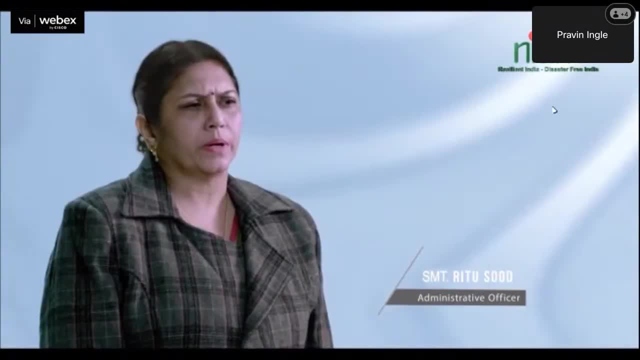 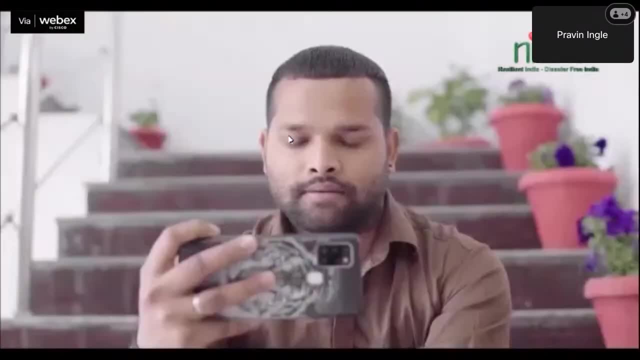 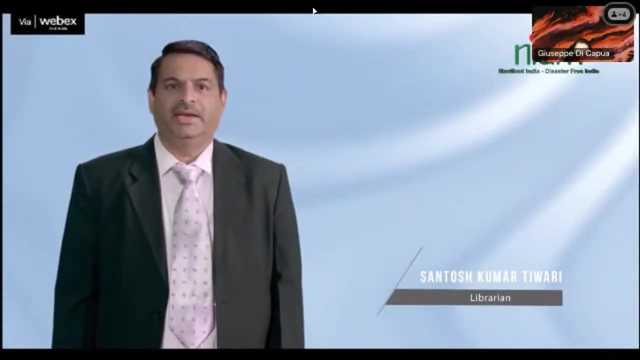 in collaboration with state and UT governments, to senior and middle level officials, non-government organizations, researchers, students and grassroots members working in the department. The library of the National Institute of Disaster Management has been acting as a crucial resource and learning center to meet the information needs of its faculty staff members. 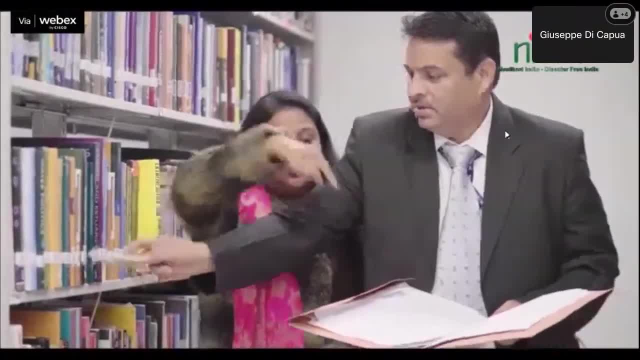 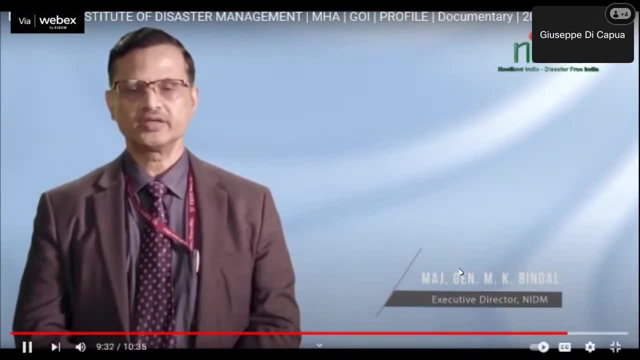 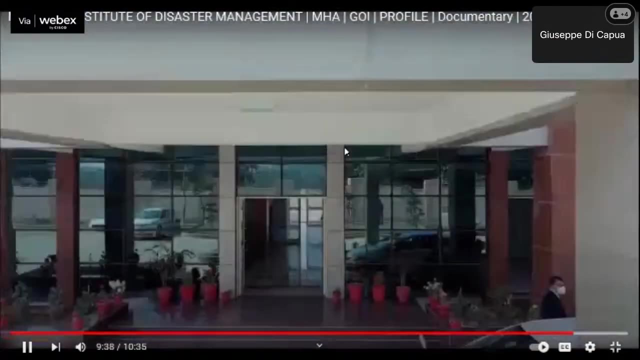 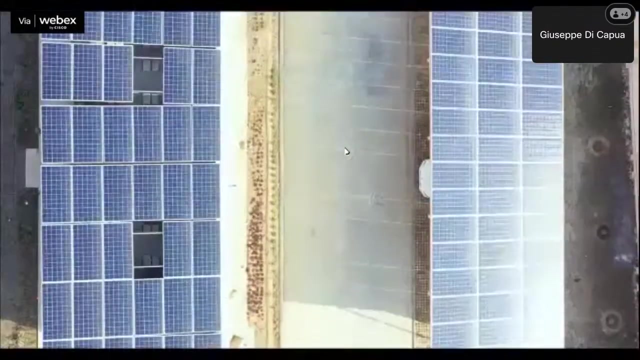 and our preferred scholars from India and abroad. The Institute is diligently working towards fulfilling its core mandates with utmost zeal and commitment, and envisions to become a full-fledged university in its endeavors to make India disaster resilient. The vision of the Institute is to be a premier institute of excellence. 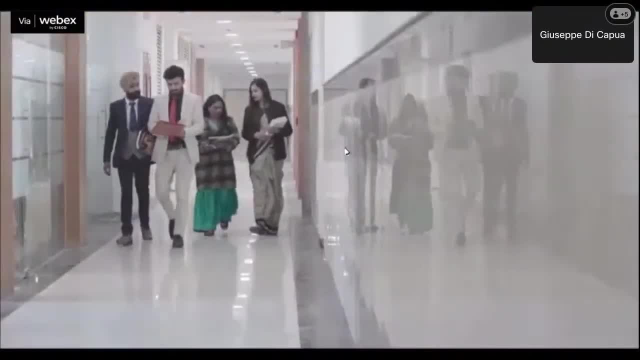 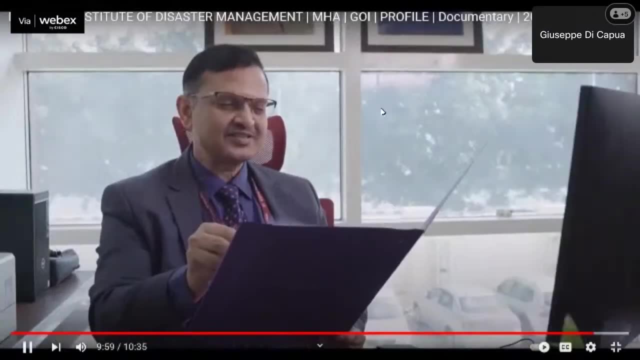 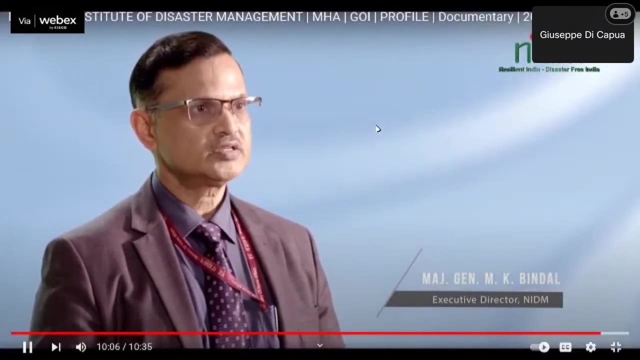 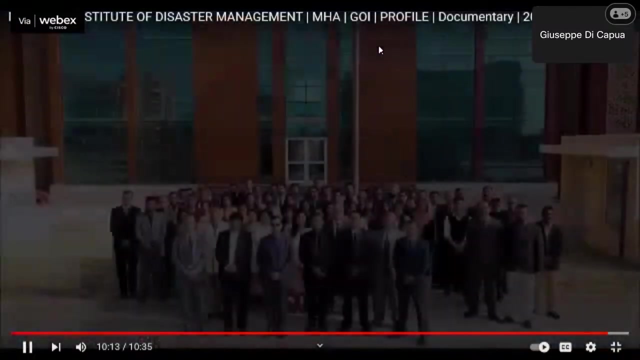 for training and research in disaster risk reduction, Also be recognized as the leading institution at international level in the realm of disaster management and strive relentlessly towards making a disaster-resilient India by promoting the culture of prevention and preparedness at all levels. NIDM is ever-evolving. 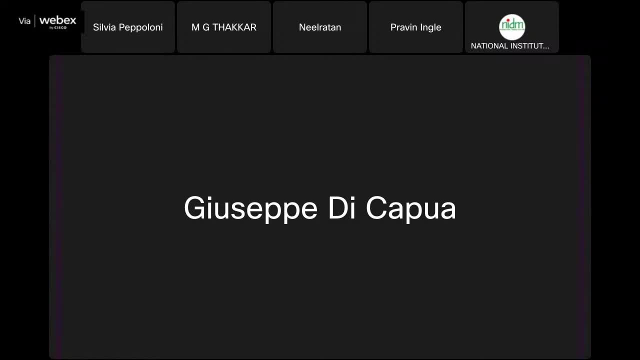 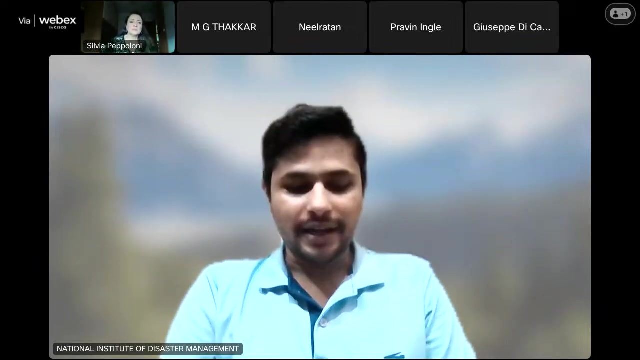 We have a number of Good afternoon to all. Myself, Shubham Badola, young professional at National Institute of Disaster Management Centre for Hill Area Development, and I welcome you all to this webinar on International Geoethics Day, titled Geoethics with Focus on Geoheritage, Geotourism and Geoconservation. 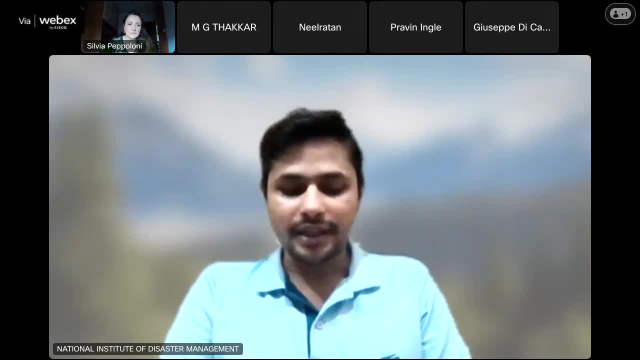 First of all, I would like to thank our partner, Sri Rajendra Ratnu, IAS, Executive Director, NIDM and Programme Chair, Professor Surya Prakash, for giving us this opportunity of conducting this webinar. I would also like to welcome our keynote speaker. distinguished speaker- programme convener. 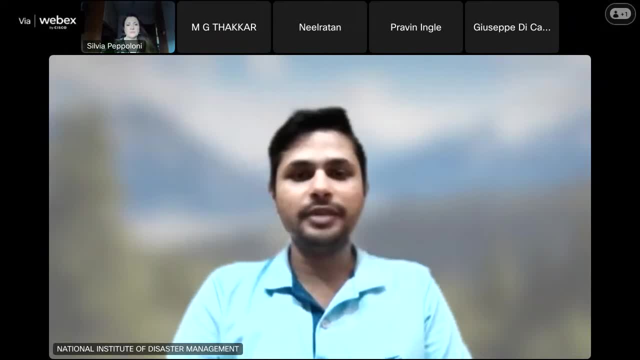 and my programme coordinators, who are there today with me for conducting of this programme. I would like to give a short glimpse of the Geoethics Day. International Day of Geoethics is an annual observation dedicated to the development of geoeconomy and geoscience. 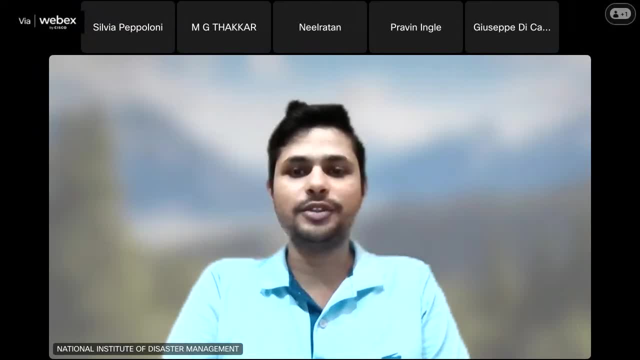 To promote ethical and responsible behaviour in the field of geosciences and environmental sciences. this day, celebrated on 1st Thursday of Earth Science Week each year, highlights the importance of considering ethical principles in the study, exploration and stewardship of the earth and its natural resources. 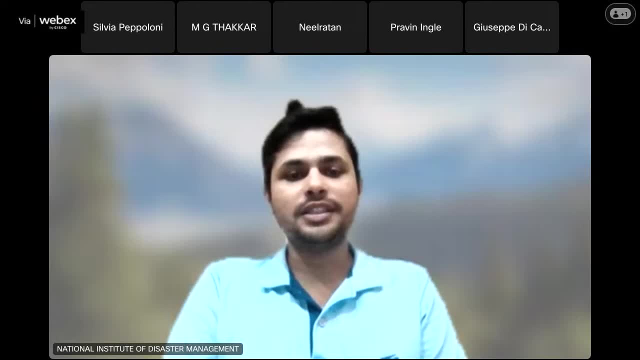 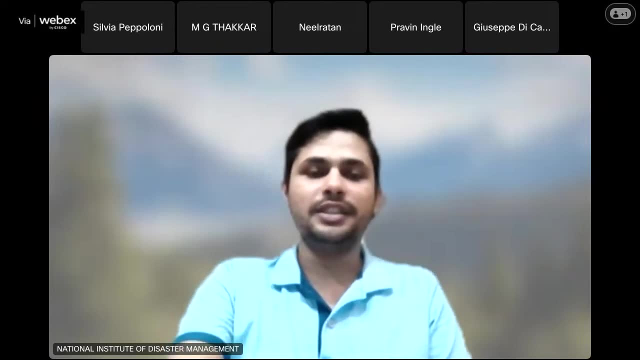 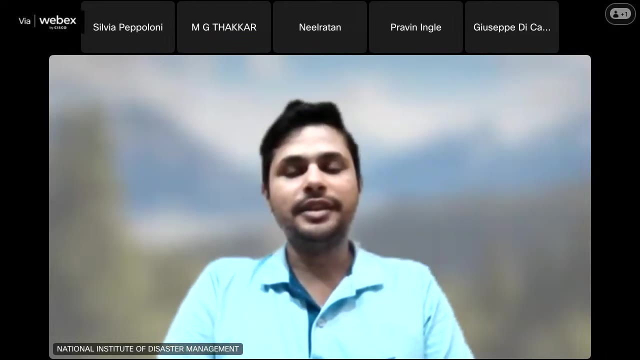 It serves as a reminder that the pursuit of scientific knowledge and sustainable practice should always be guided by ethical considerations. To protect our environment, we must always be aware of the importance of ethical principles for our planet and future generations. So with this, I would like to call upon Professor Surya Prakash to please give welcome address. 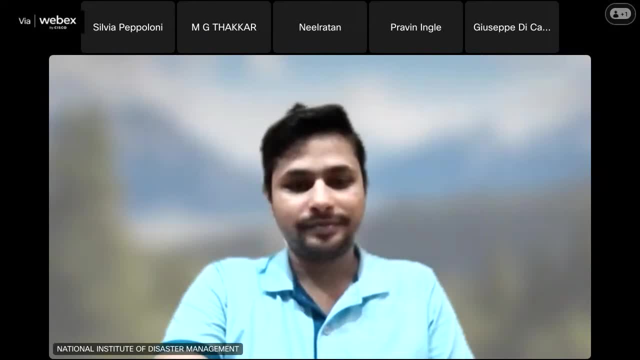 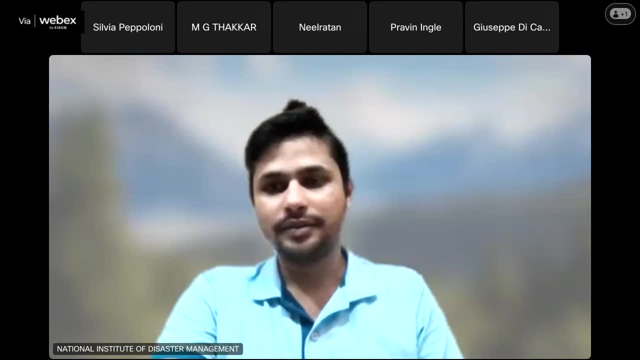 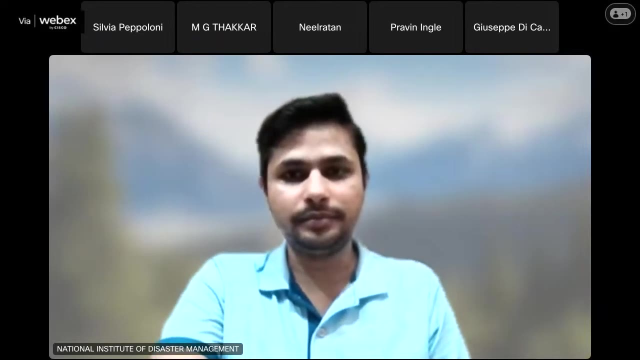 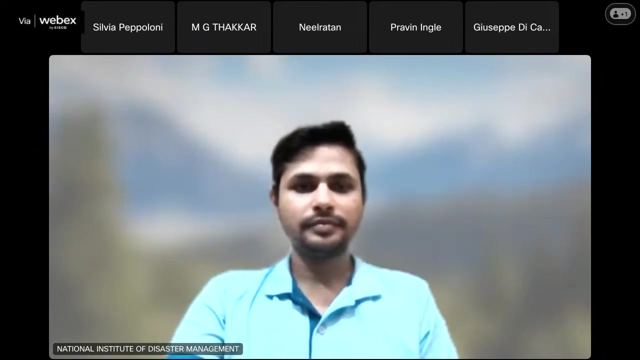 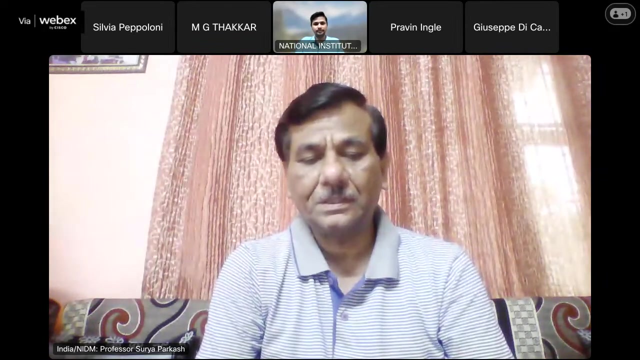 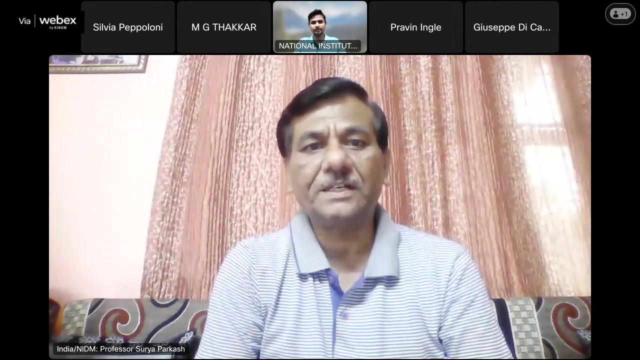 for this webinar Over to you, sir. Thank you, Shivamji. Am I audible? Yes, sir, you are audible. Okay, I think some network signals are poor. So first of all let me congratulate and wish you all the best for the International 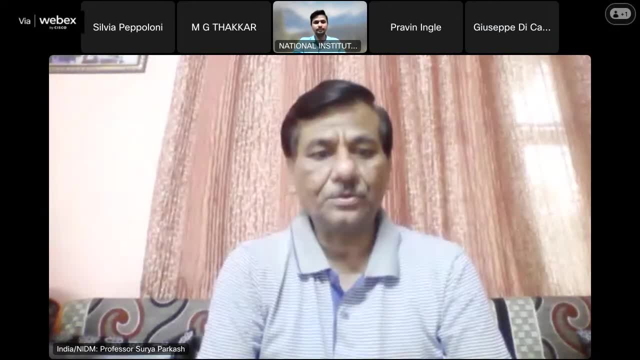 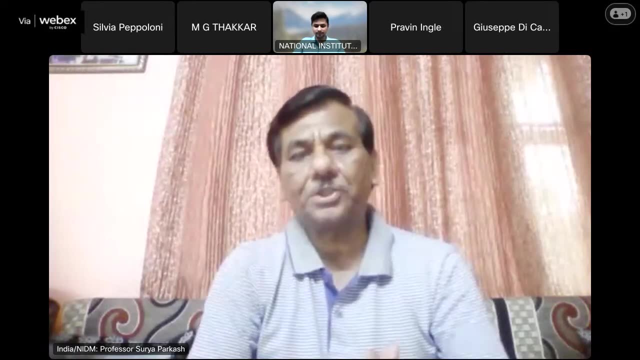 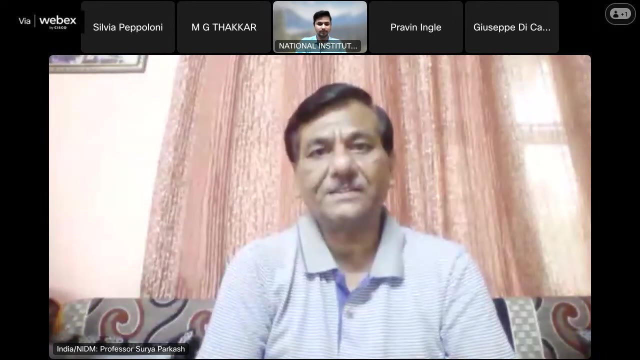 Geoethics Day that we are observing during this week of this year. We have a. We have been actually working for geoethics for quite a long time now And the other related areas of geosciences which pertains to our geoherities, geodiversity. 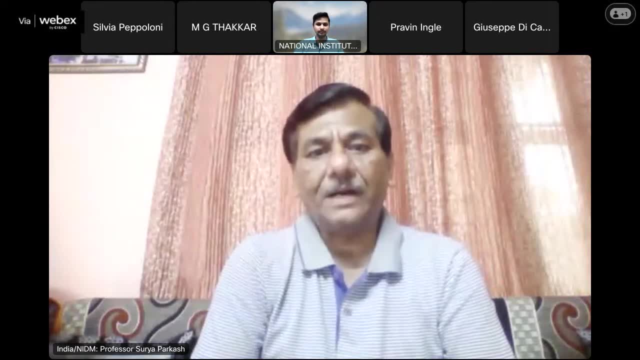 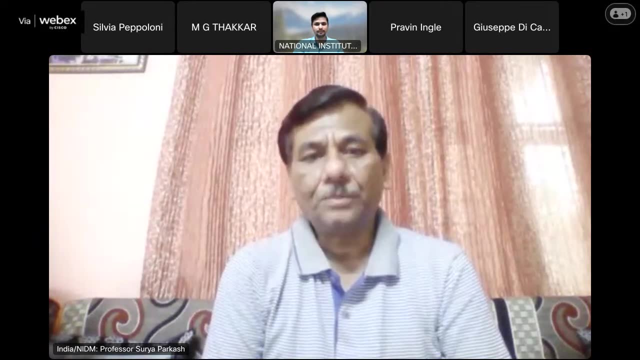 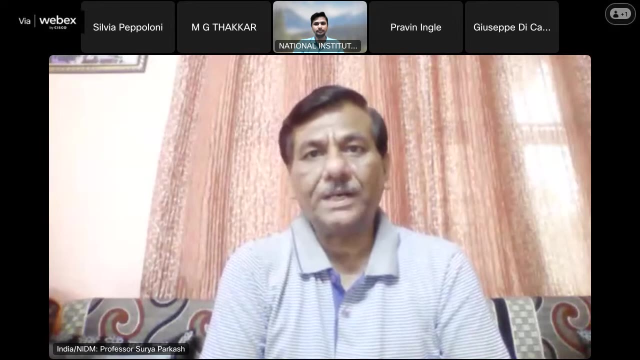 geo-tourism. geo-parts and other related areas have also been well integrated into this discipline of geoethics to take care of our projections and values related to geoscientific importance. And before I go ahead, I must thank our Secretary General of International Association for Promoting. 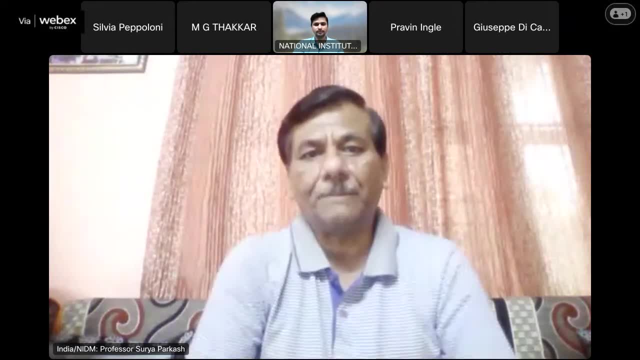 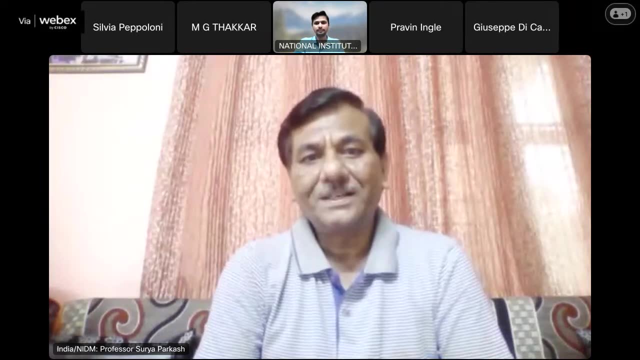 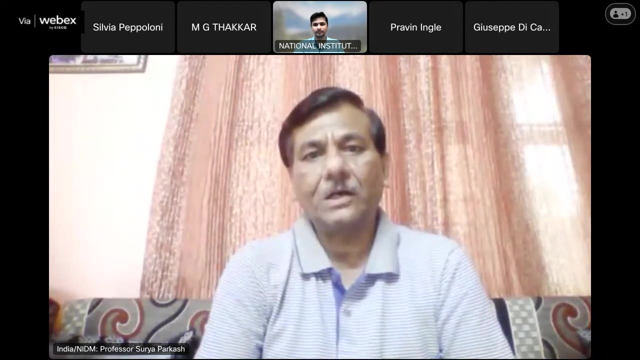 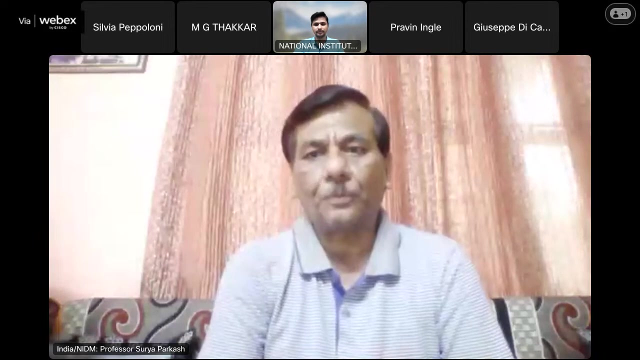 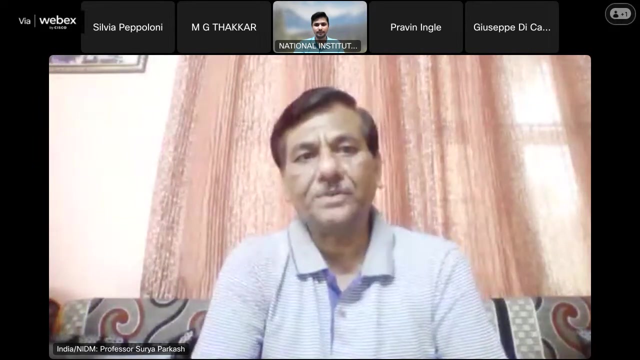 Geoethics, Ms Sylvia, Dr Sylvia Papaloni, who has been one of the pioneers and key drivers to taking this movement of geoethics forward at the global level, taking all the national coordinators along with us. And thank you also to our 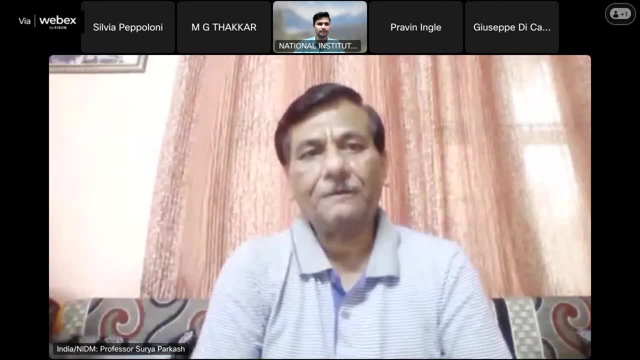 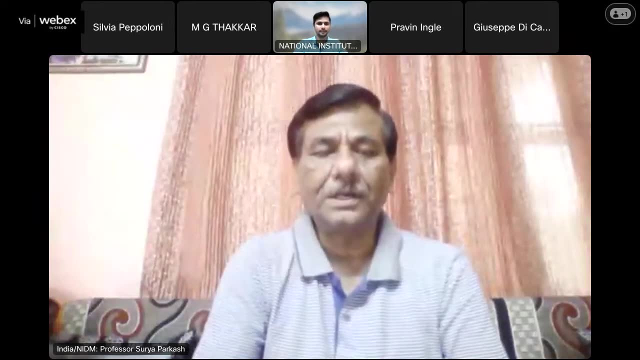 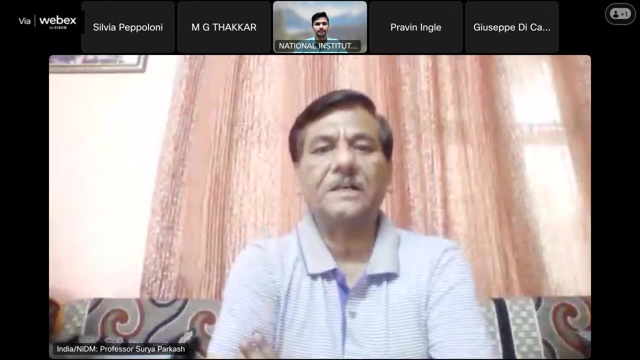 coworkers at the headquarter, professionals and also our treasurer Giuseppe Di Capua, from Italy, who also kindly joined with us, And let me also welcome, on behalf of IELP India, Professor Dr M G Thakkar, who is currently the Director for the National Institute of Paleobotany, which is located in Lucknow. 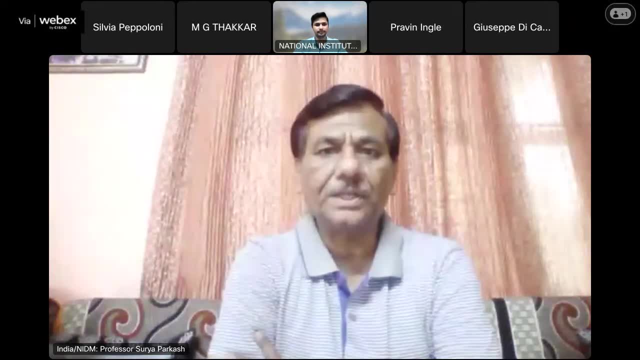 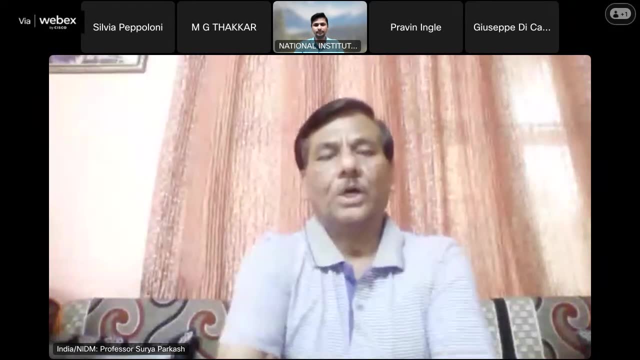 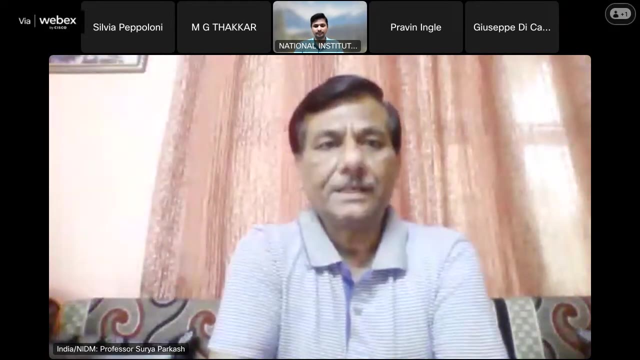 Dr M G Thakkar, who is currently the Director for the National Institute of Paleobotany, which is located in Lucknow. He has very kindly agreed at a very short notice, along with our other expert speakers, like Praveen Engle and also our supporter, Dr Neel Ratan from Central Institute of Mines. 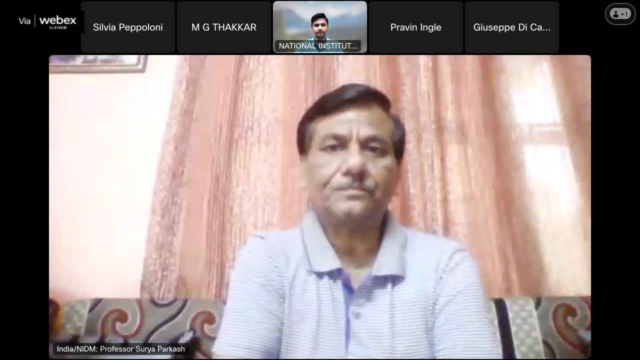 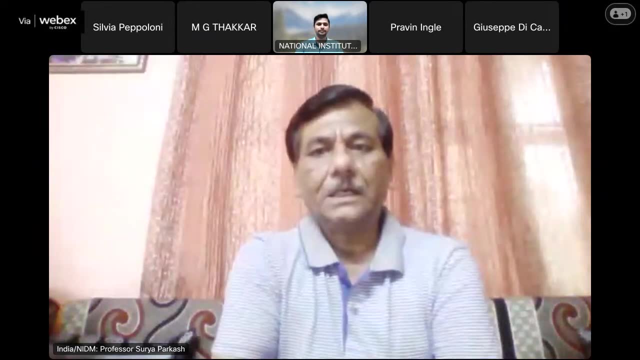 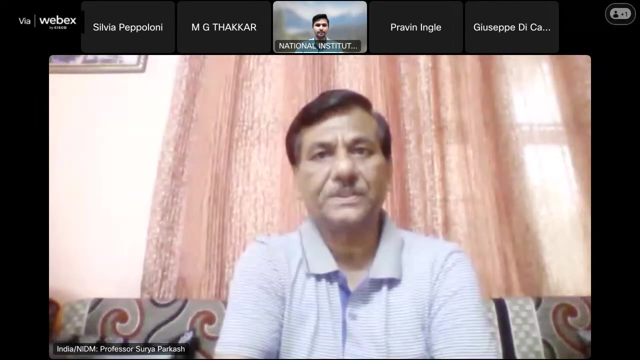 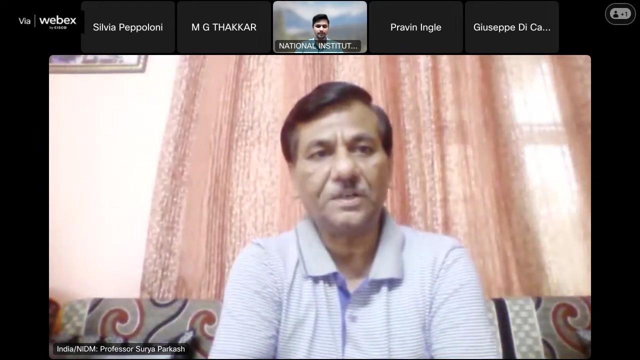 Fuels and Energy Research Wing of Council of Scientific and Industrial Research in India. We have actually been supported not only by these limited number of resource persons and experts or distinguished speakers. In fact, we received support from all our professional associations related to geosciences and earth sciences. 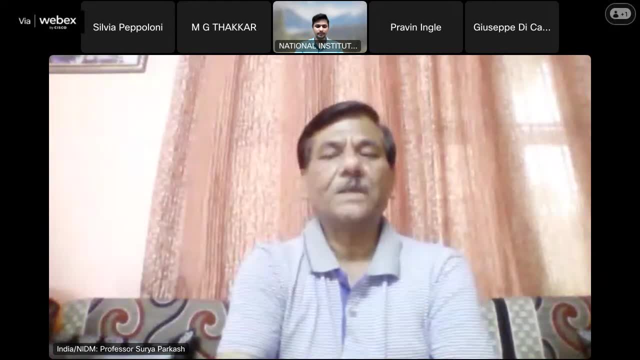 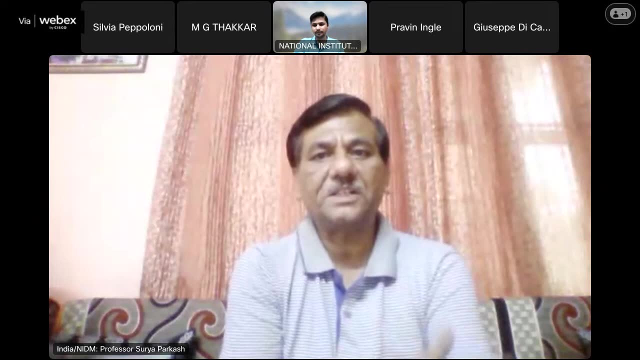 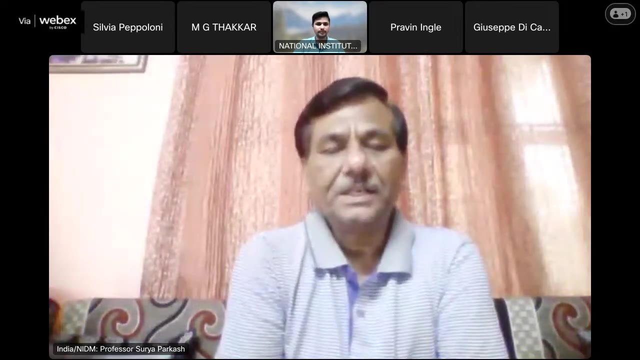 be it the Indian National Scientific Academy, be it the Geological Survey of India or Geological Society of India, and, at the global level, International Union of Geosciences. We have also joined hands with IAPG in spreading the message of geoethics. 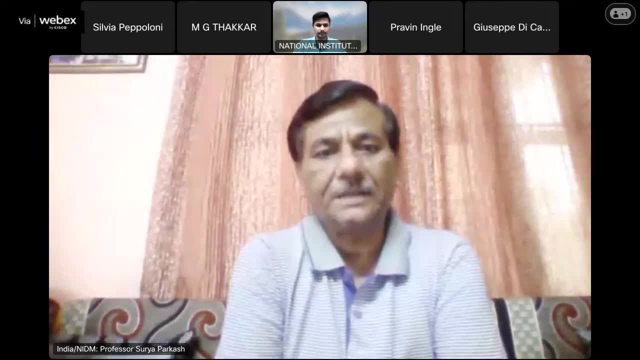 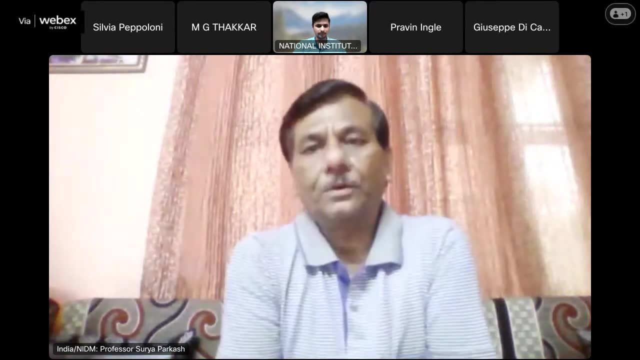 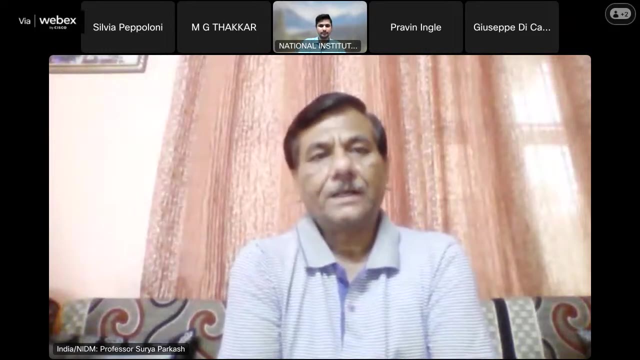 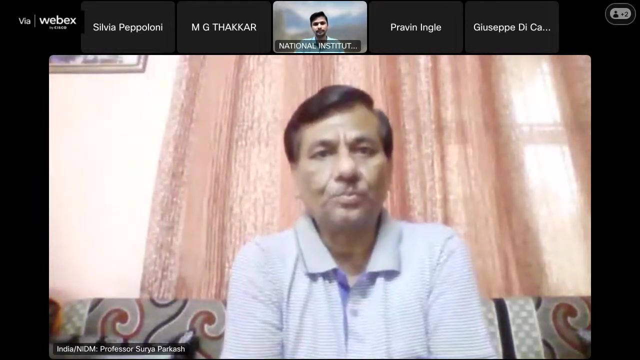 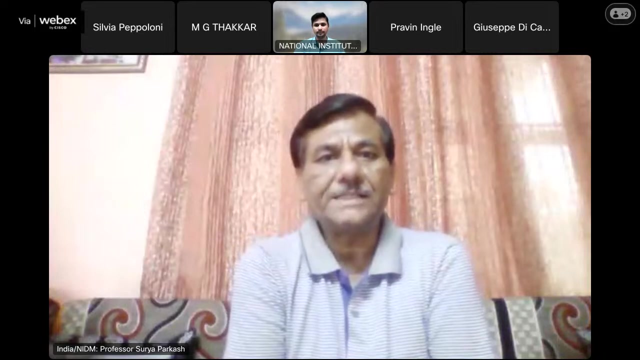 which is one of the prerequisites for earning credibility amongst the society to attach values to the geoscientific outcomes and research education, which needs attention from our society. Earth science, particularly in India, has not been very popular. in that area, Most of the students who do well, they go either to engineering or to other scientific and technological lines rather than geosciences. 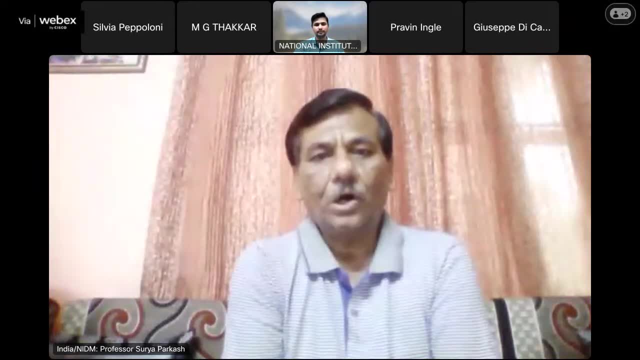 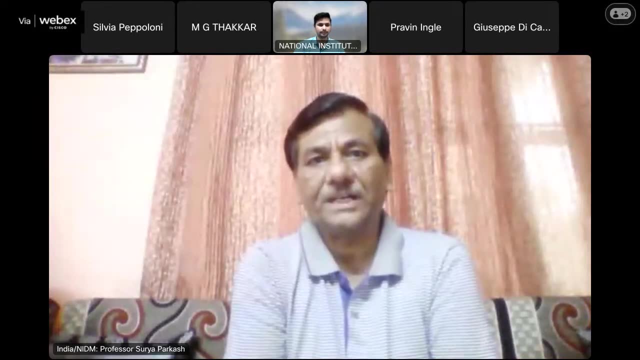 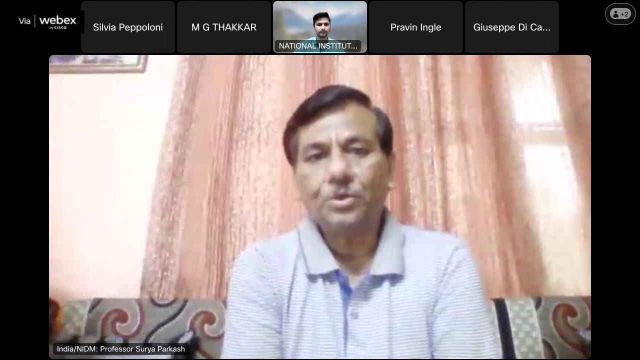 However, geoscience has contributed a lot, because all developments which take place are happening on the land And it's the earth scientists who know the best about the attributes of these land areas and landscapes and land processes which help them to do better. 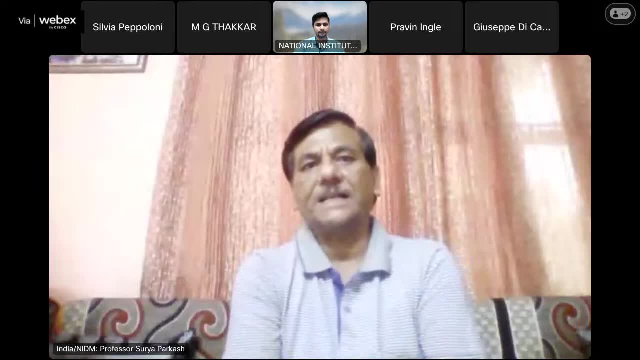 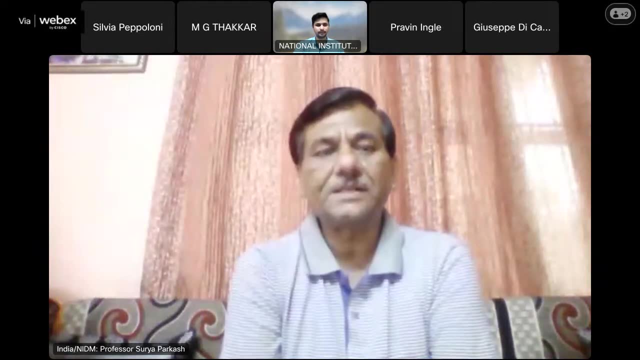 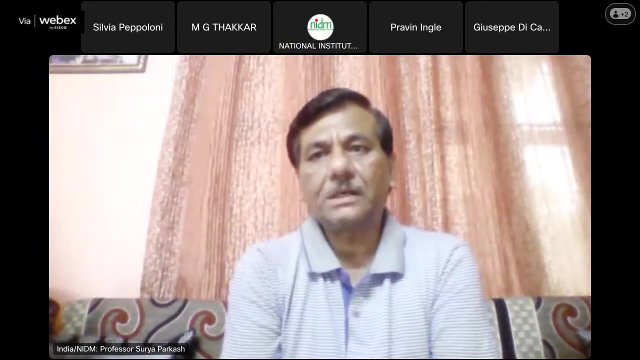 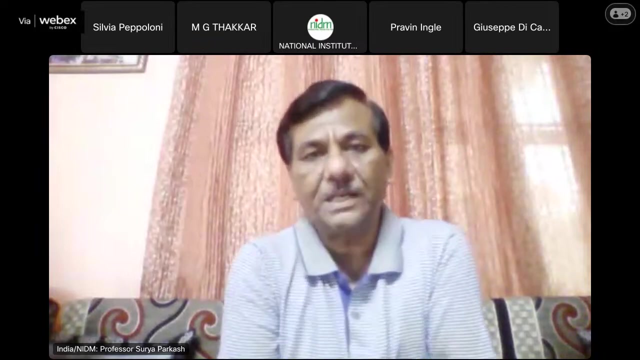 And more effectively for the developmental purposes than any other profession. However, the society yet needs to be convinced and conveyed about the importance of geosciences through our works, which require attention because a number of our geological possessions of high value, which carry even the legacy values, have been lost because of the developments. 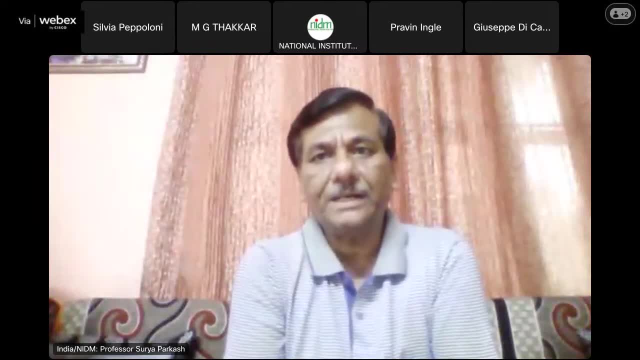 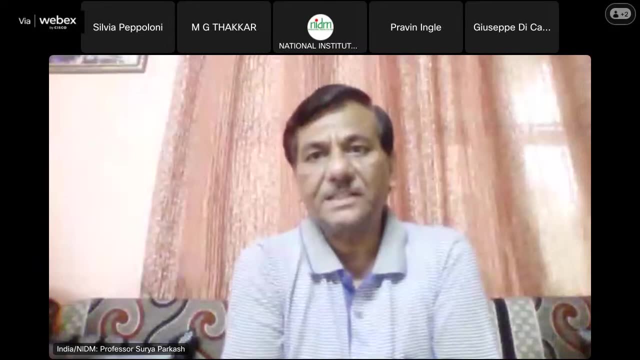 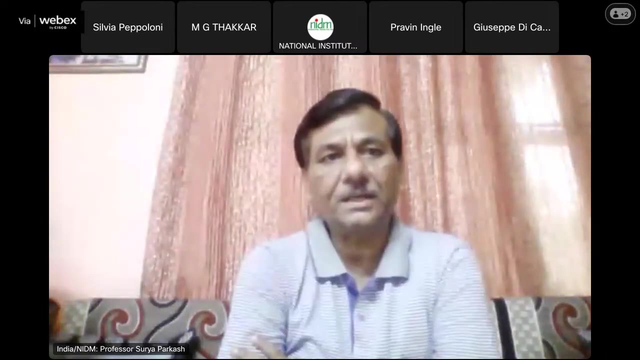 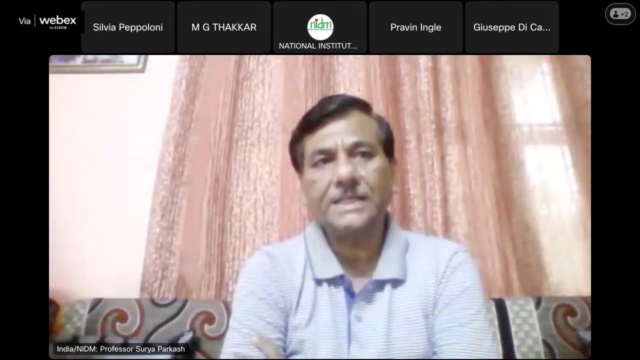 which are quite chaotic Sometimes and unplanned, without caring for the geological treasures they come across, which actually reveal us the history and evolution of the earth, its processes and the resources that we are obtaining from the earth. So, therefore, we have come together and we have been organizing a number of activities, along with other activities. 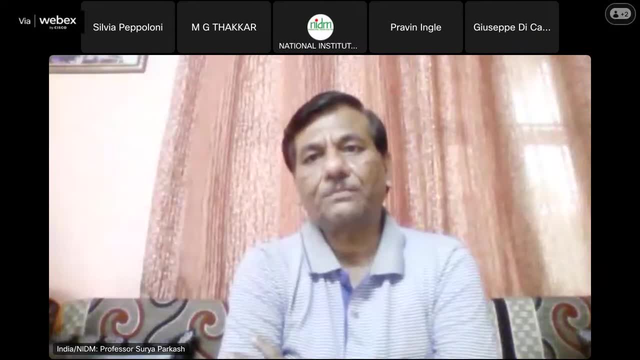 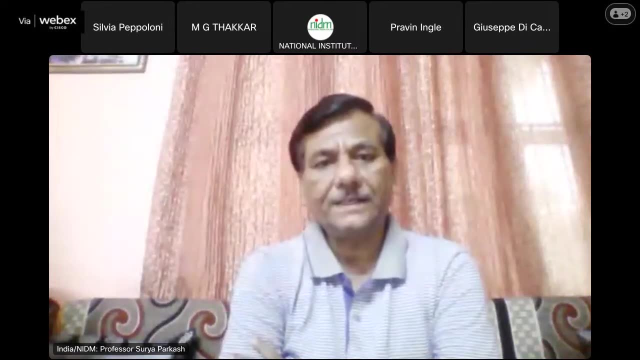 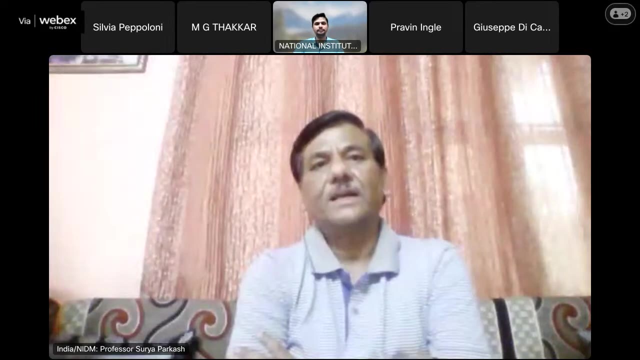 Also, we are including lectures on geoethics So that we can emphasize the importance of ethics in all our practices, And also, on the other hand, we have been requesting our colleagues to kindly come up with standards, guidelines, policies, regulations. 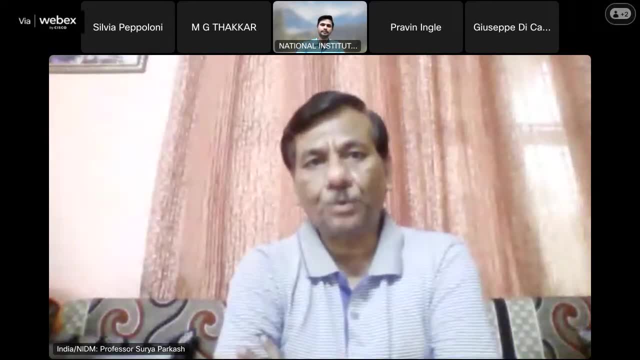 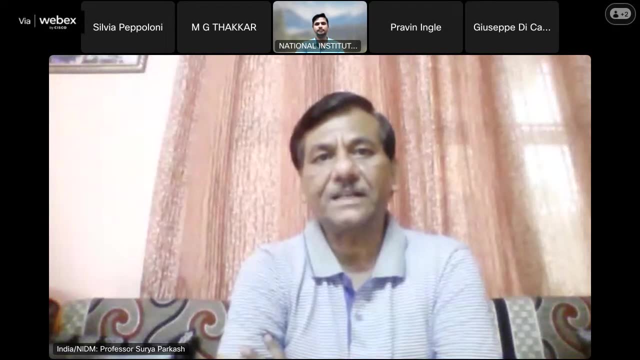 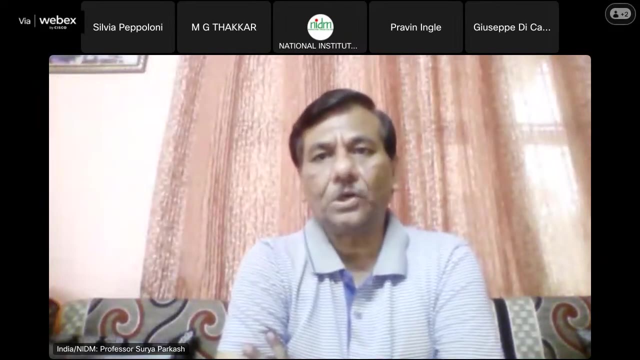 and even, if necessary, some legal provisions or laws or statutory measures which can help us undertake necessary activities to preserve, to protect and to continue. Thank you, Thank you very much, Mr Gopal. Thank you, Thank you. Thank you, Mr Gopal. 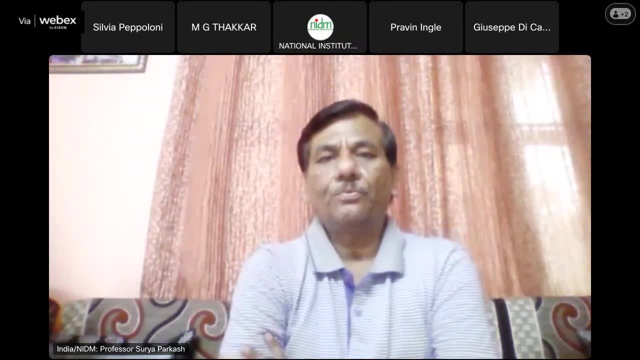 Thank you. So I would like to welcome Mr Shantanu, Mr Patil and Mr Hemant. Mr Hemant, especially in terms of geological studies, you have been concerned about the importance of heritage to the future. 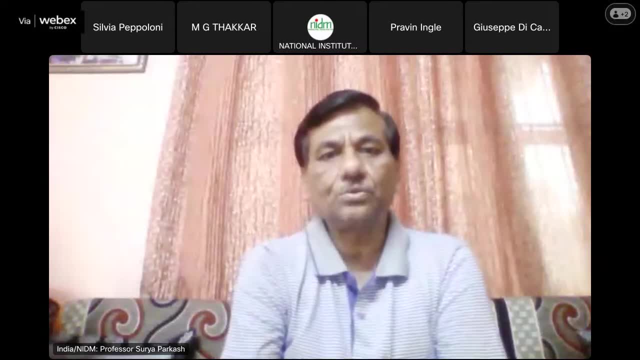 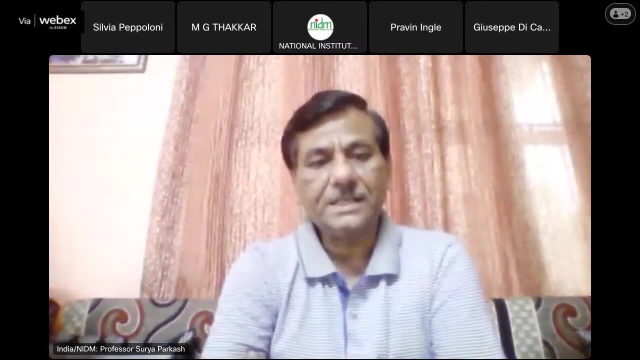 Yes, in terms of nature, you are right. This is the most important thing that I would like to bring to the discussion of the future as an education practice. in addition to the education and education to be a reality, I think that if we take a look at the historical history, we should also take an example of 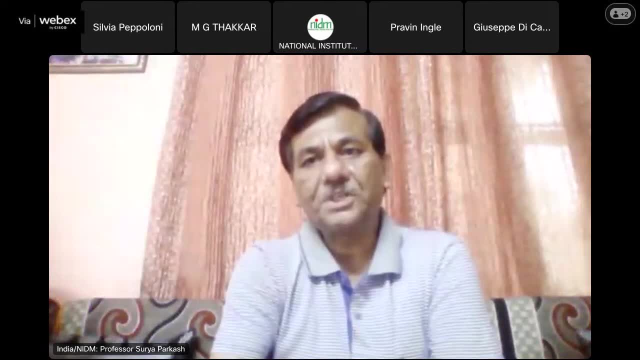 the our heritage down to the future. When we think about the long history of our land, we should not think of the history. We should think about the history of our land, which is the history of the past as well, uh, which should be enjoyed by our future generations too, as we have done so. so these 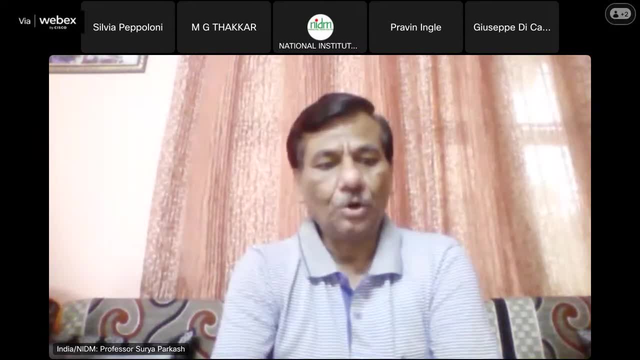 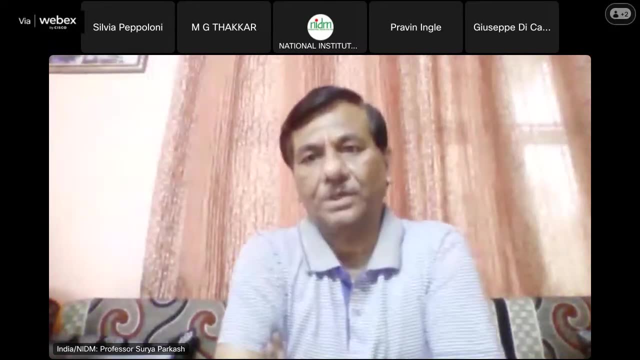 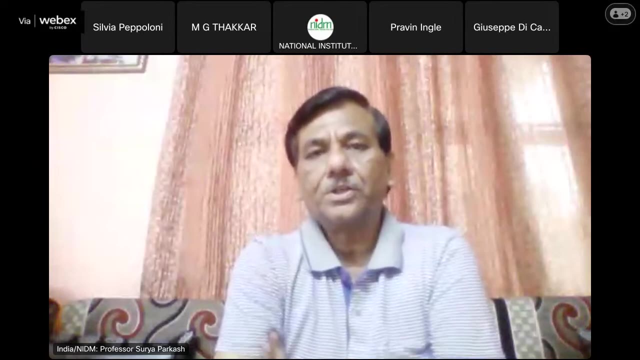 words. i welcome everyone and hope we will focus on all these important areas of the. this year. we have also again observed the international day for biodiversity as well, and we are also working on geo heritage, geoparks and geotourism too. in india, we have got around. 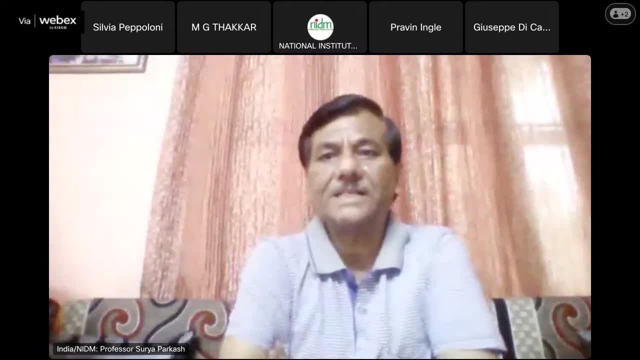 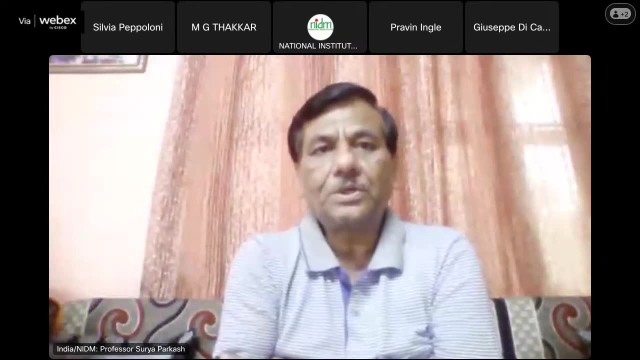 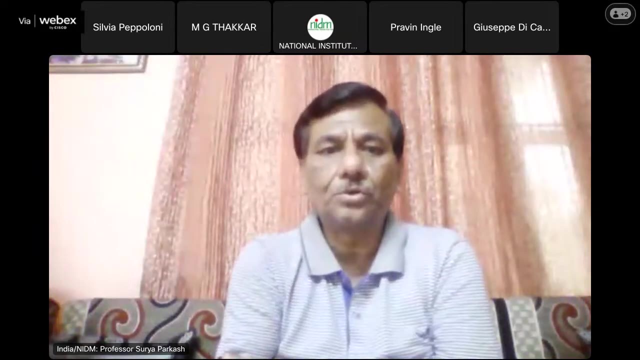 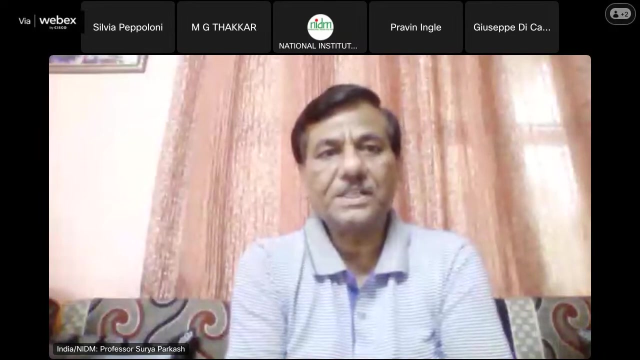 more than about three dozens of sites of geological importance which have been declared at geo heritage sites, and also about more than dozen of sites have been actually set out for geotourism as well. we are in the process of identifying the geodiversity areas which also need to be preserved, protected and conserved. 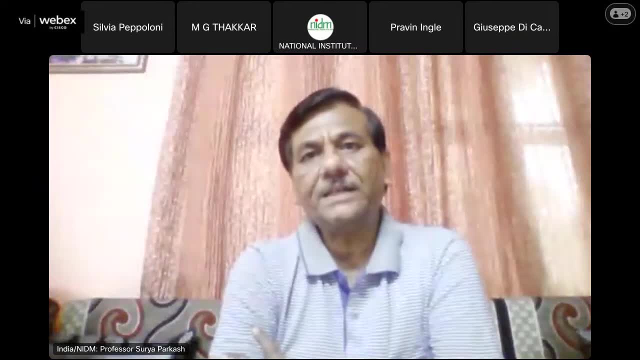 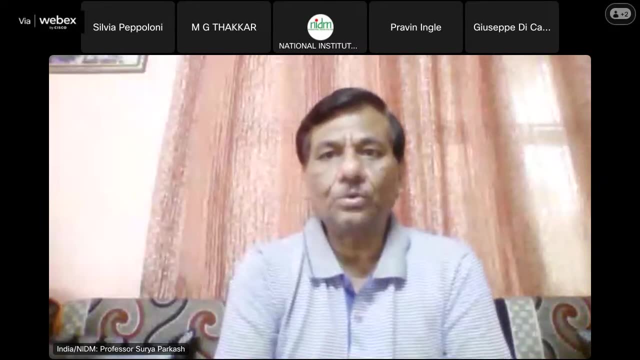 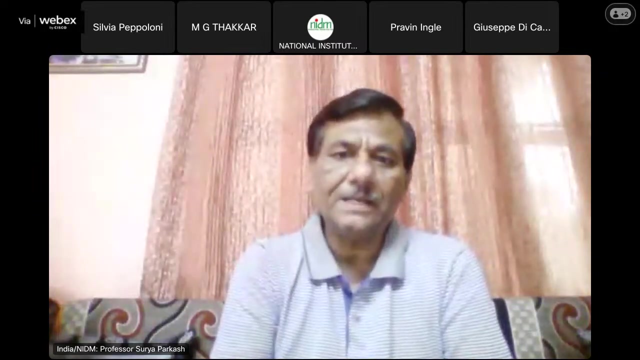 against the destruction of mankind. so, basically, in geoethics, we are focusing on our human activities related to the arts environment where, through our interventions, we are actually destroying the heritage and treasures of the earth which need to be protected. so so, and that is one of our side, the other side, we are also talking of the behavioral practices. 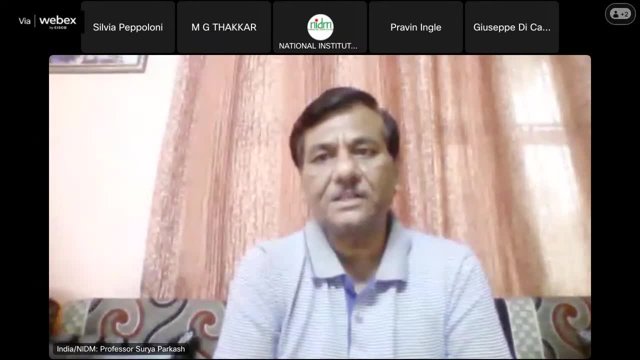 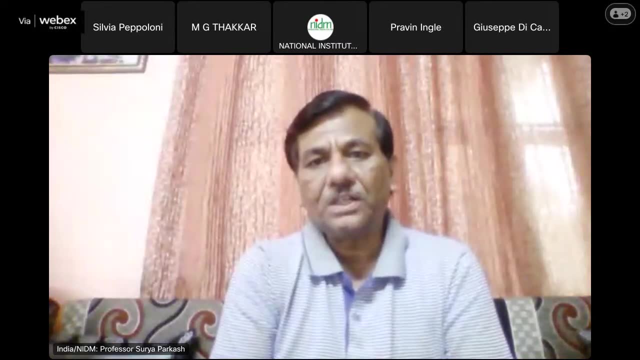 and actions being taken by our geoscientific professionals too, and their duties and responsibilities towards our society, so that we carry our duties with moral responsibilities which are to be executed at, i would say, in all the levels and all the scales, be it at the global level, we say 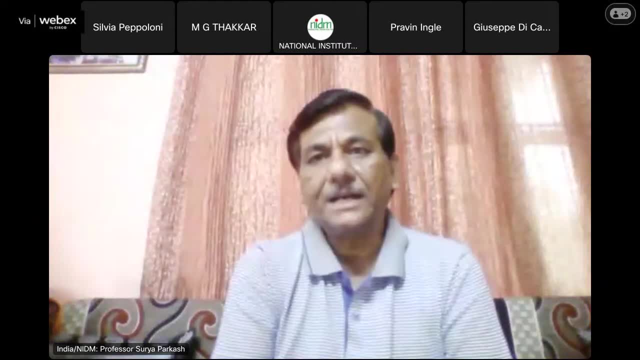 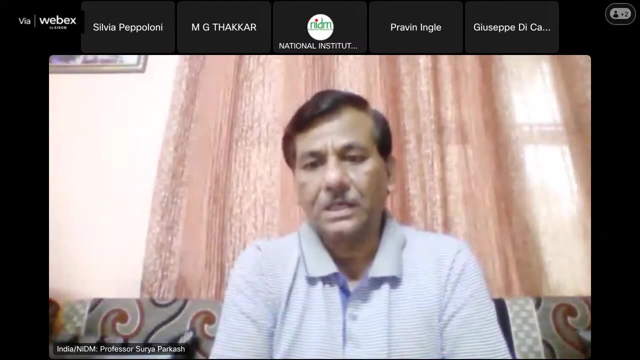 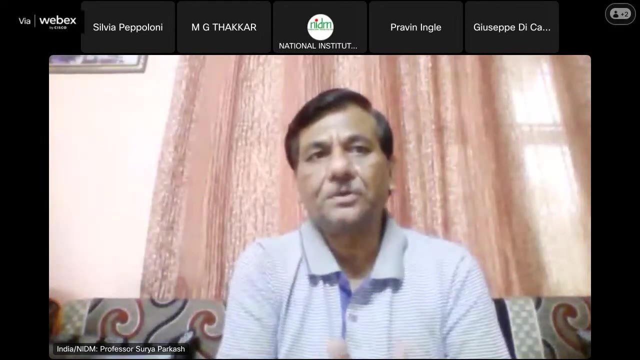 the global level of ethics, which is universal and should be followed by everyone at any place at any time, and then national level, which are projections at the countryside levels and need to be taken care, then provincial and social as well as individual levels. so we have to have objective as 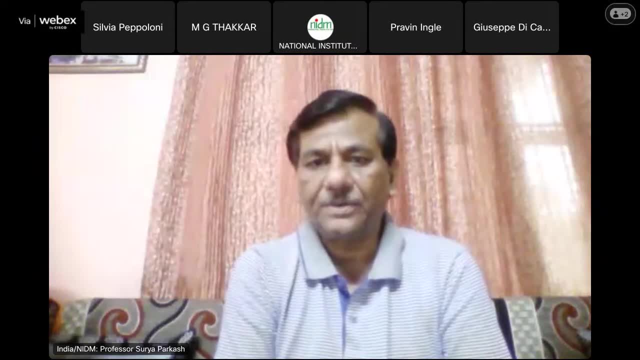 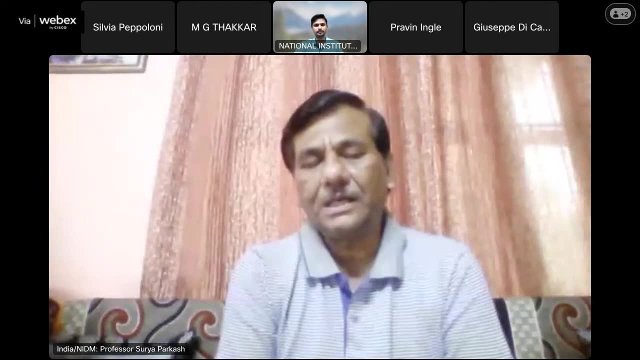 well as subjective ethical practices amongst ourselves. and this will not follow until unless we have a good conscious and we actually try to learn the value of it in our practices and behaviors and activities. so with these words i would say what vivekanandji has said, that the time has actually alerted us. 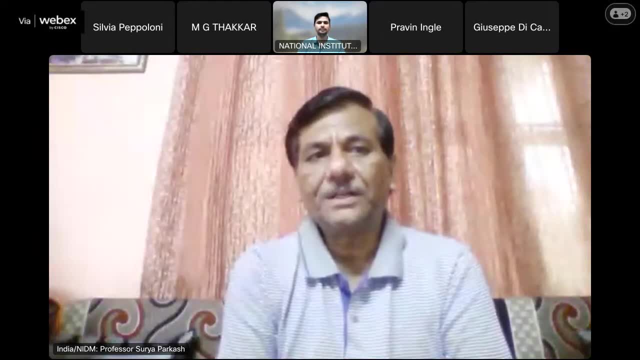 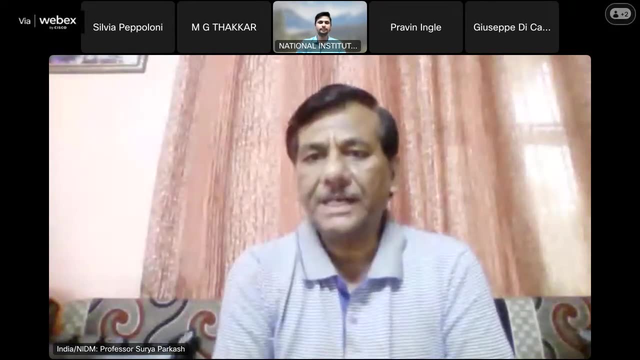 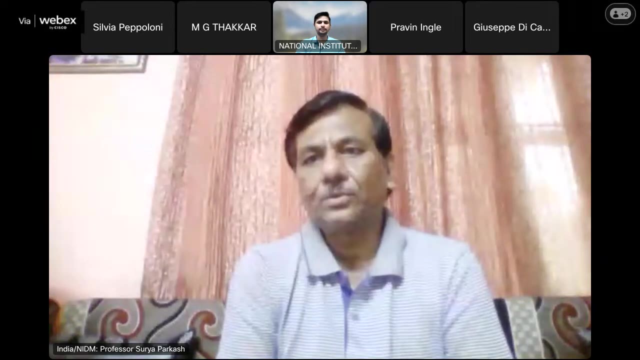 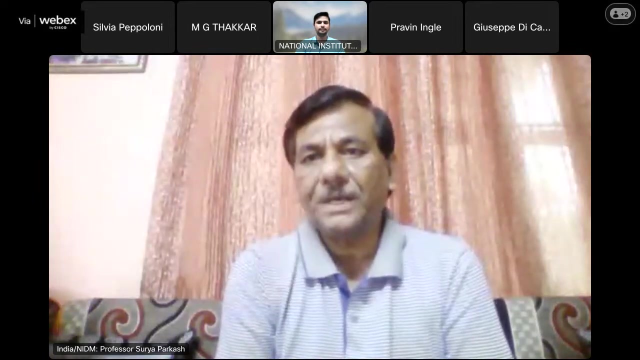 so kindly arise, awake and stop, not till our goal is achieved, and our goal is preservation: protection and conservation of geological heritage and attaching significant values to the geoscientific professions in the society. so with these words, i thank the organizing committee for providing me this opportunity to share my views. i am sure our 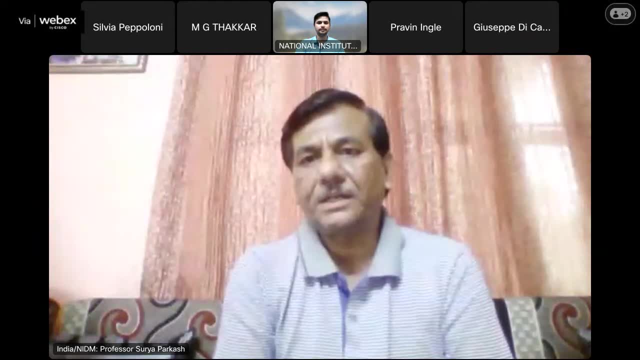 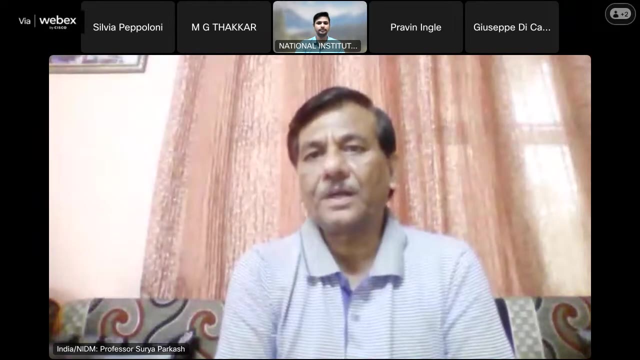 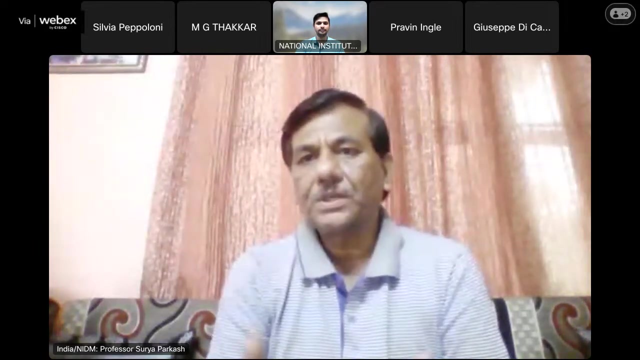 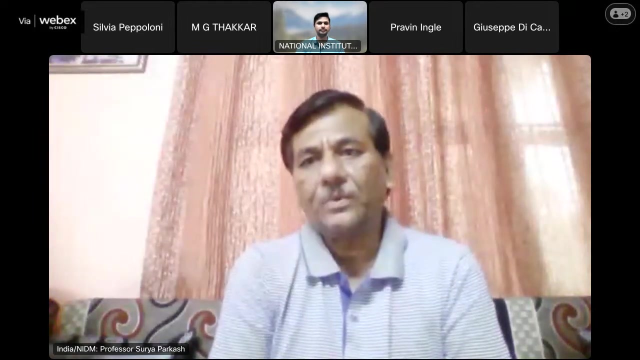 experts will surely talk very details about how we are proceeding ahead and what can be the effective road map to achieve our goals and go ahead with our more effective practices, with the adequate standards, codes, guidelines, procedures, regulations and laws that may also be parallelly required. i have always been persuading. 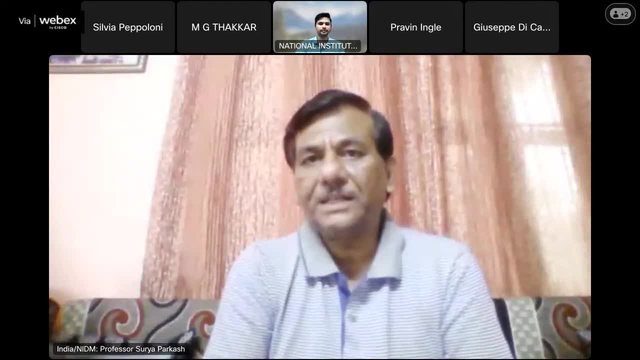 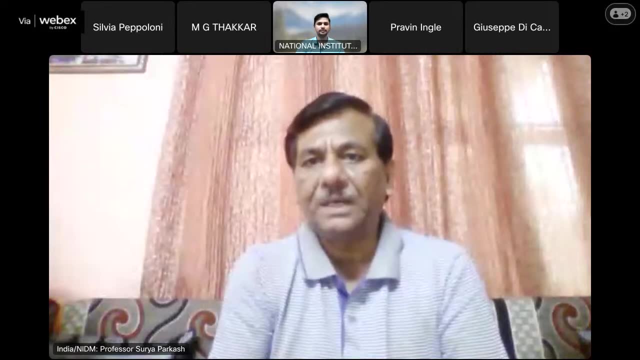 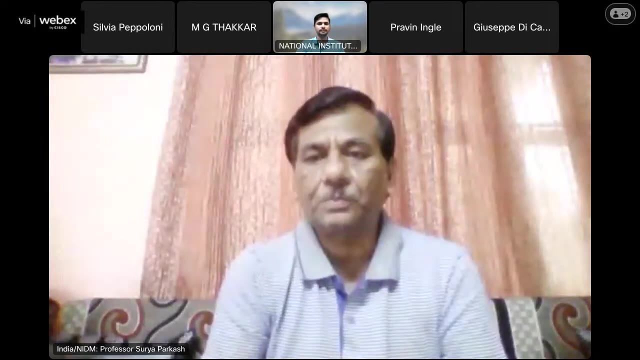 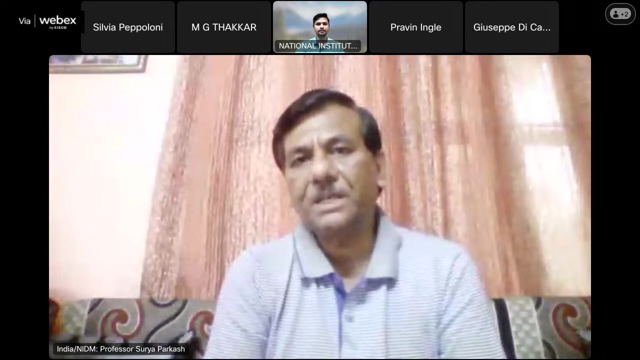 my colleagues for following up a new subject area as social geology, which can actually integrate society and geology together and can bring together the social tools for the geologists and also to the sociologists, philosophers and psychologists and the values of geological information which can be carried. 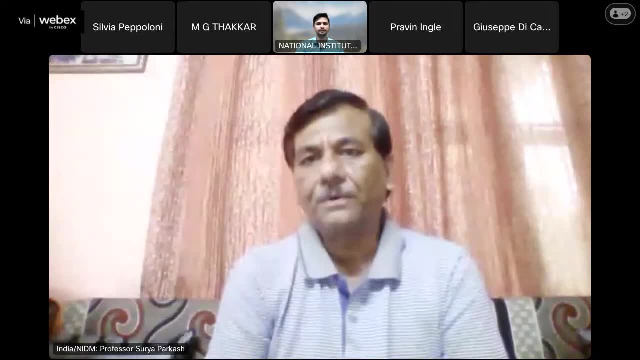 forward and utilized for the betterhood of humanity, as well as environment and our resources. this will also help us in disaster risk reduction and resilience, too. so these were the main points that i would like to share with you today. thank you very much for your attention, and i will see you in the next session. 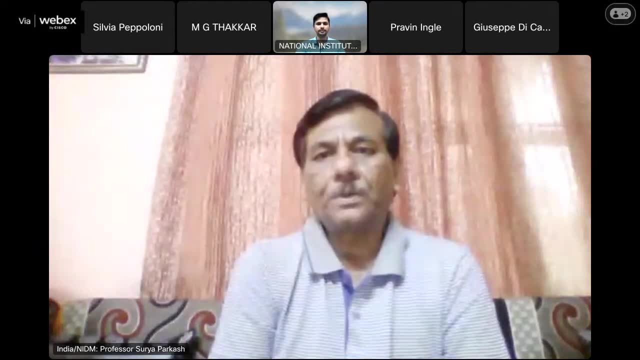 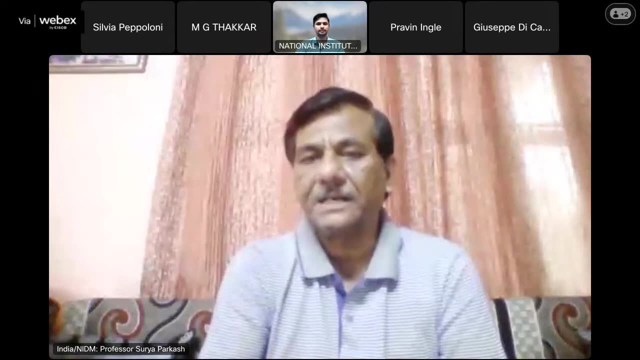 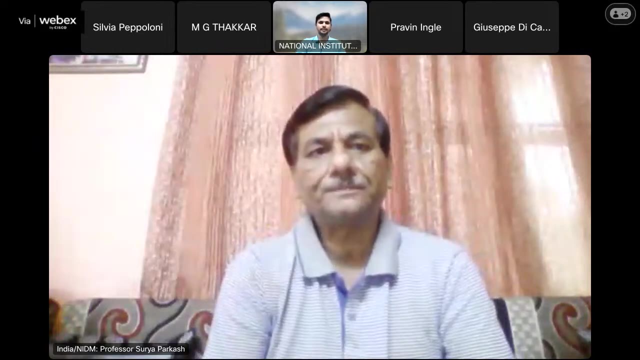 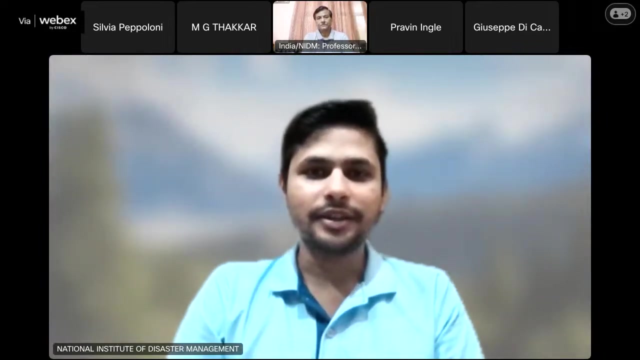 thank you very much. so, with these words, i thank and hope and wish all the best to everyone of you, along with the distinguished speakers, the guest dignitaries, delegates and the participants of today's program. thank you very much. back to you, shubhamji. thank you very much, sir. 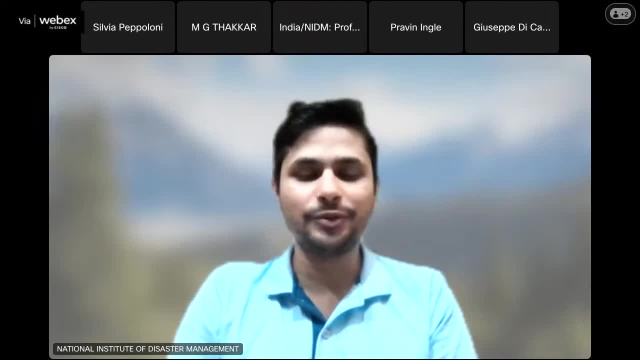 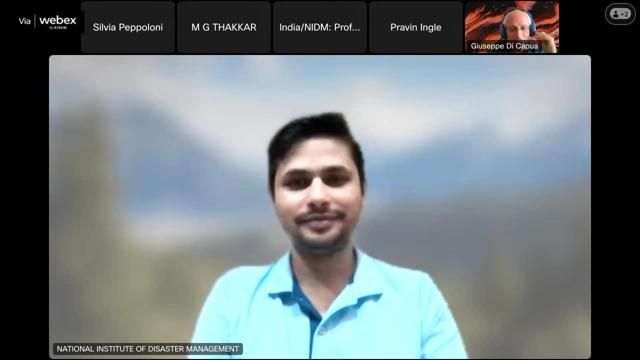 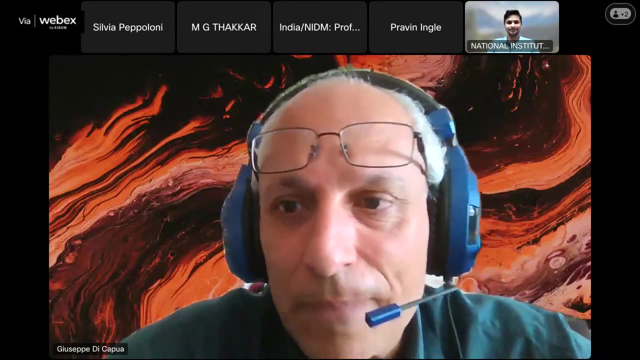 for motivating and welcome address. since we are joined with your cpd qpa sir, i would request him to please say few words on this verse webinar over to you. sir, thank you for giving me, uh, the possibility to to say a few words. i i really happy that ipg india, and then dim, has organized this event. this is the seventh edition. 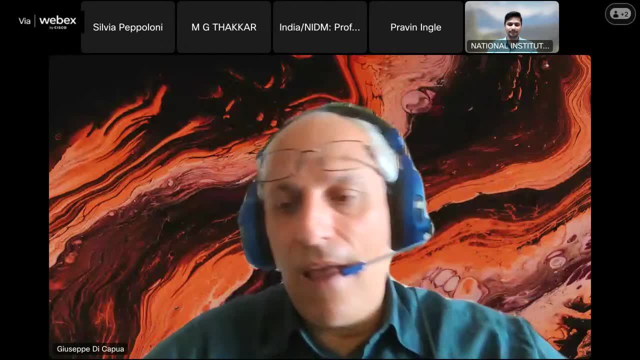 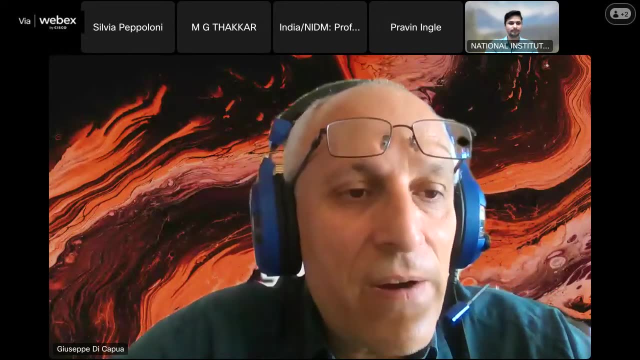 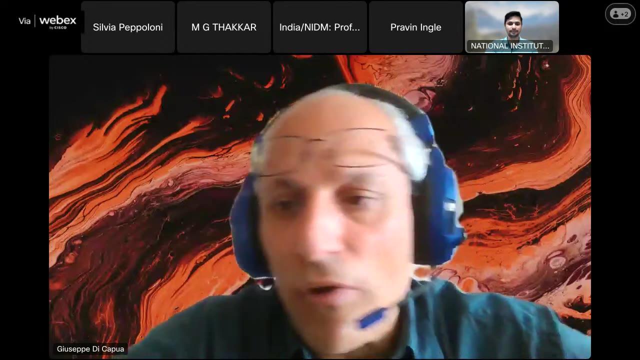 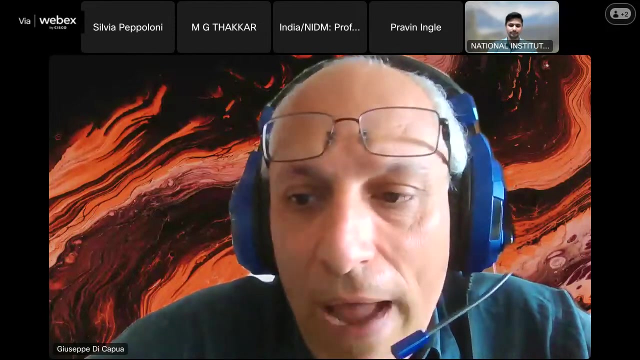 of the um- international geotics day, um and uh. i hope that also in the in the in the next years we will have the same success as this year. um i i have also included in the in the chat the link to the website of the international association for promoting geoethics. 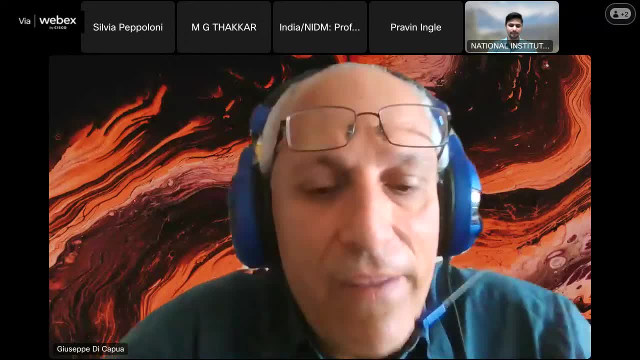 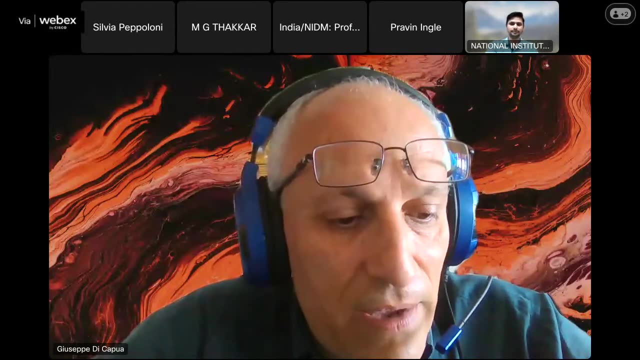 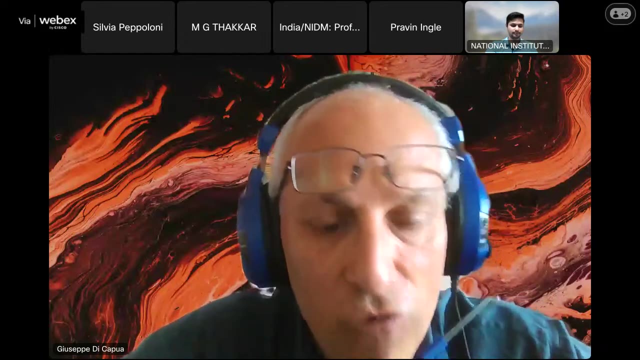 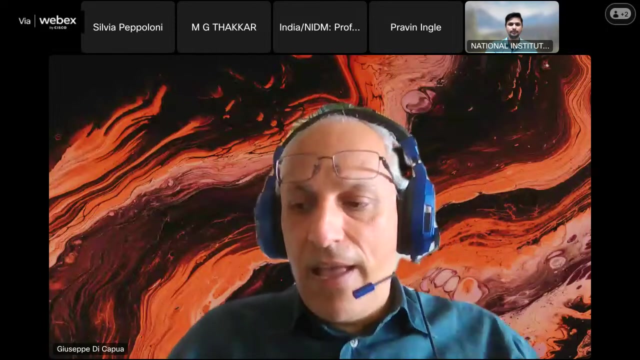 i invite you all to to follow the activities of the of the iapg. i remind you that now iapg has, in cooperation with the iugs, has created the iugs commission on geoethics, so now there is also a branch of the iu, of the ipg, that is developing activities directly within the. 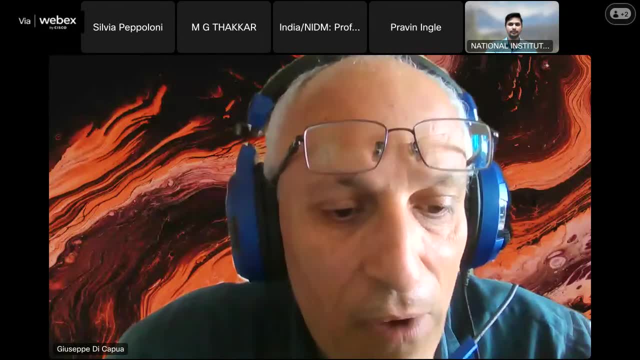 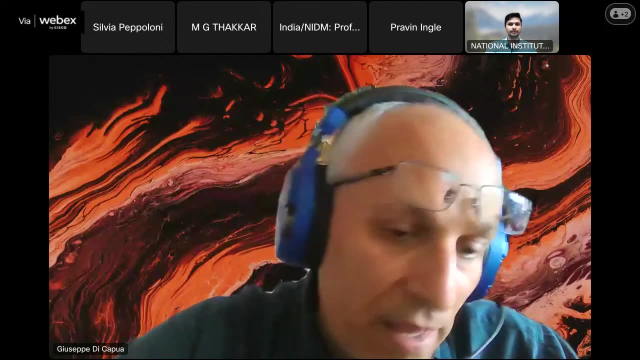 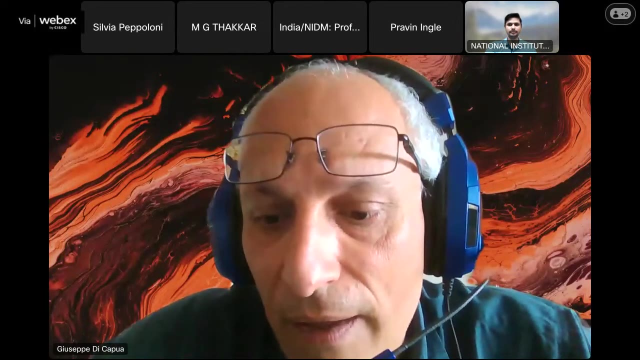 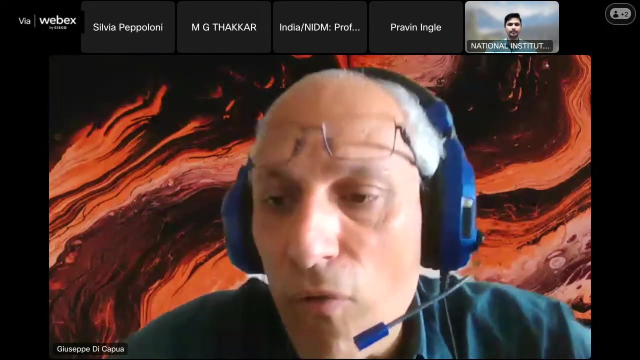 international union of geological sciences. this is a great recognition for our activities in the last in in the in the past 10 years. so in i remind you that becoming members of the ipg is without fees, so i invite you all to become members of the ipg if you are not already. 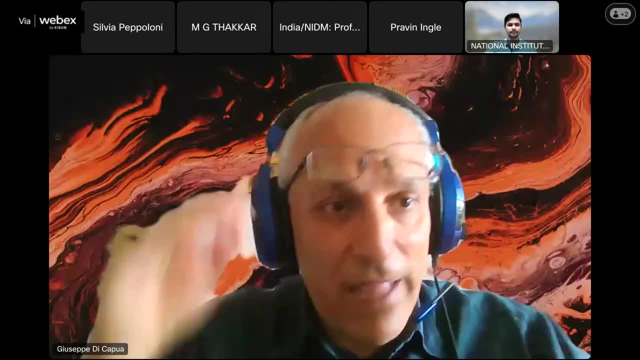 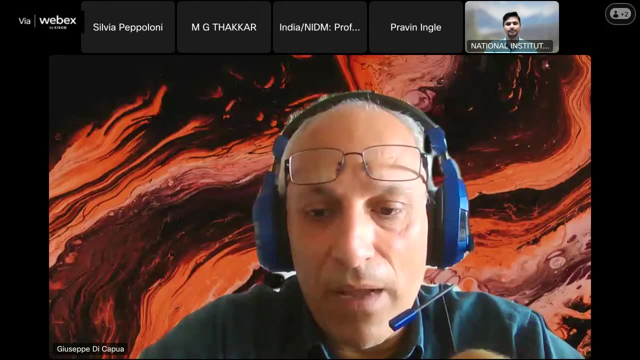 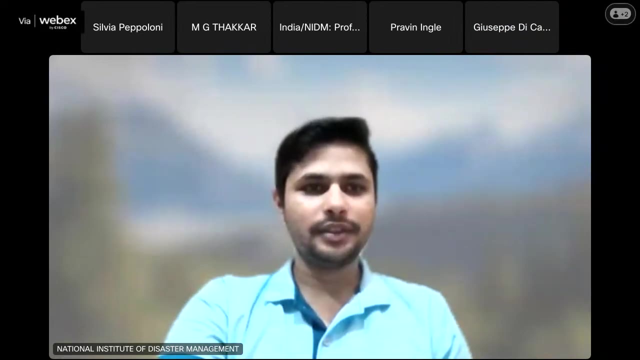 в Pipes is possible or not, or or are not broken. so that has been fully понимad in the in the past. thank you, thank you, and have a nice, uh nice, a nice work for this webinar. thank you, thank you very much, sir. so, moving forward now, i would like to call upon 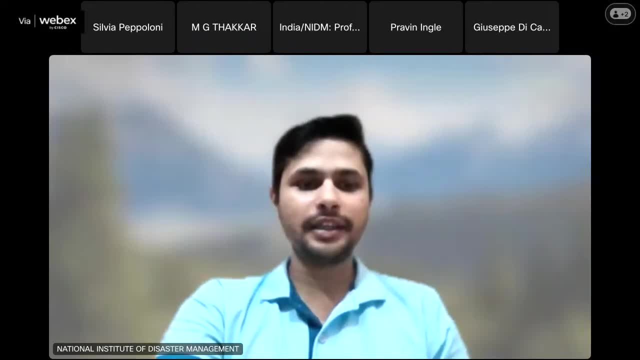 professor mg thakkar. before that i would like to give a short introduction about him. currently as a director at Birbal Sahani Institute of Paleo Sciences, and he has been working as a geologist after completing his PhD in Neotectonics Geology from MS University Varudhra. 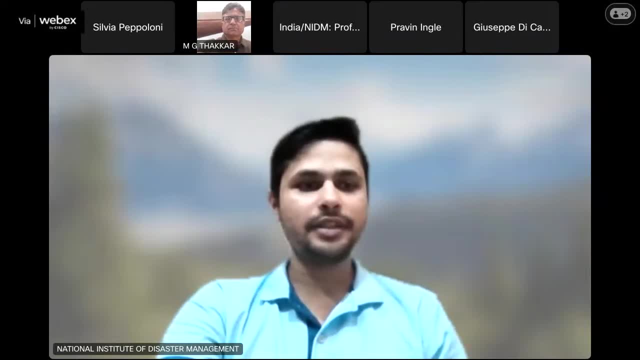 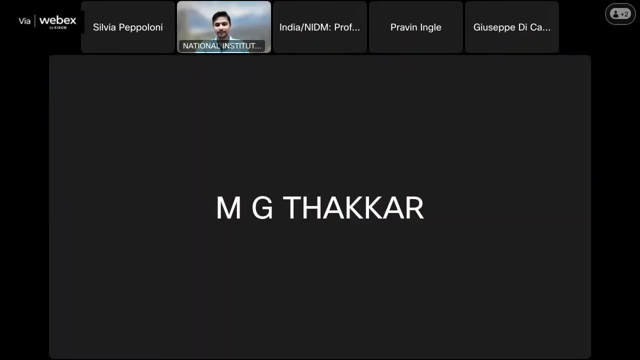 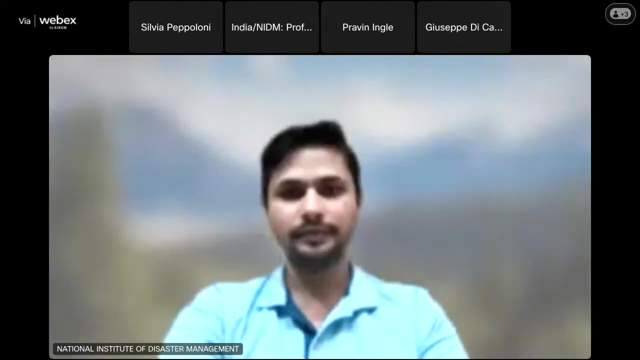 and he has also been awarded with many awards. along with his research interest, he has also authored many books, research articles, also presented many international and national conference papers. with this, I would give the stage to you, sir, please. Hello, Hello, Hello. My video is not visible, I think. 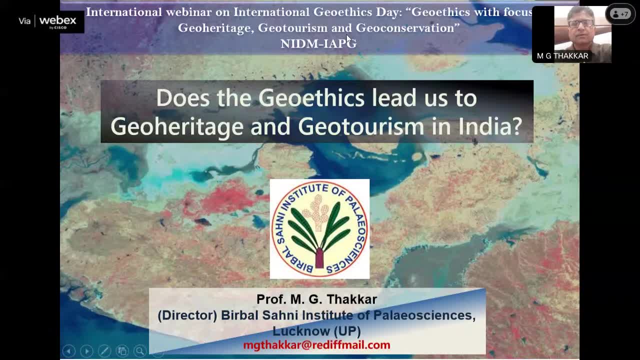 I say you, Is it visible Video? Yes, sir, yes, Okay, and I'm audible, okay, Yes, sir. Actually my laptop is not working, so I have requested Neil to present on my behalf the operator slides on my behalf. okay, So Good Afternoon, everybody, and good afternoon oh, the organizers and renowned speakers international. 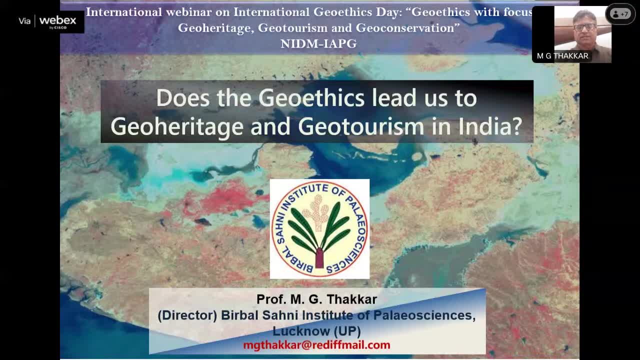 speakers, my topic for this keynote is, seems that's the geo ethics leads us to geo volcanism and geotourism in India. The topic is very critical in terms of the defence areas work confusingly. I will start off by examining particular aspects of this topic, which are extremely important. 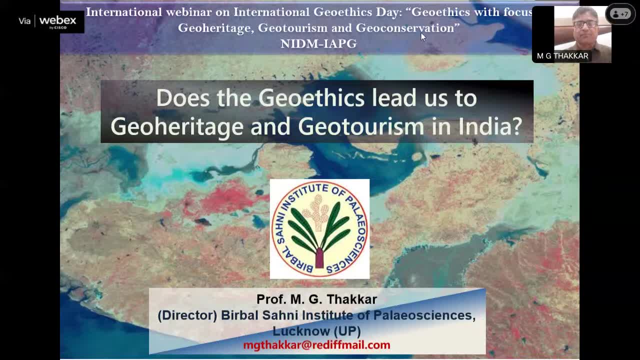 during theوس about based on relevance of the field of geohlie ticking includes sourcing geohl sagte deciring concepts. it is cabecear in particular, audio as a meeting place in uh, the development, the development in the sense, the infrastructural development, mines and in other. 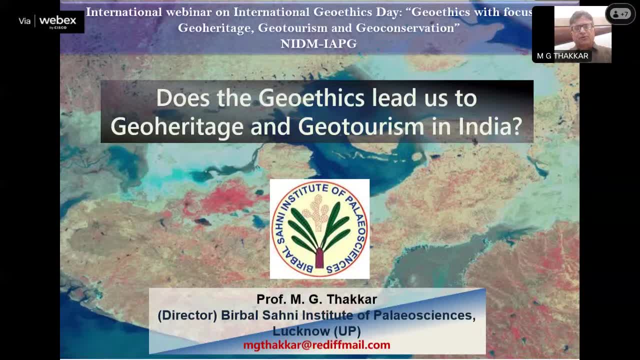 industrial development. but before we have talked much about the- I'm talking about the Indian scenario- we have talked much about the geo heritage. last maybe five years we have been uh discussing about the geo heritage and there are hundreds of sites we have discovered. basically, it is not the game of last two to three years, but since last two centuries we have identified several. 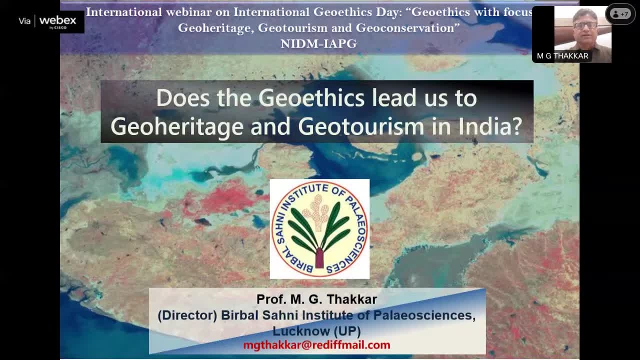 hundred uh sites, geologically important sites, but we did not give the tag as geo heritage. but uh, last two and a half decades when we come to know that, yes, this, all sites has to be preserved, and preserved for the conserve for the next generations, because once it has been lost it will not come again and we we cannot see it. 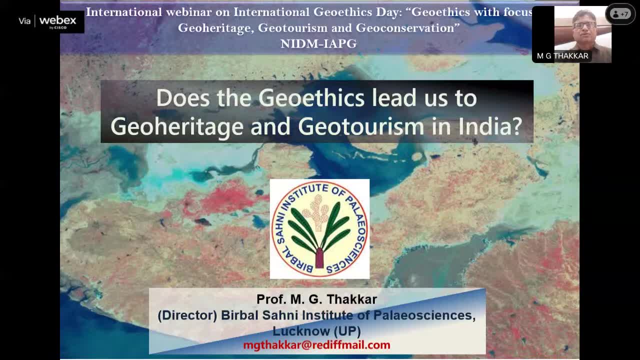 because ruthless minings are there everywhere in the world. so, uh, we must now learn about something where we can stop the things. but if we stop the mining and other activities, infrastructural activities, there will be a big issue whether we will go for the proper uh development. but what is proper development? so the sustainable. 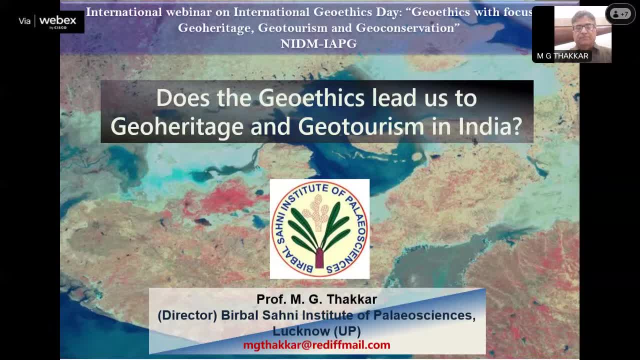 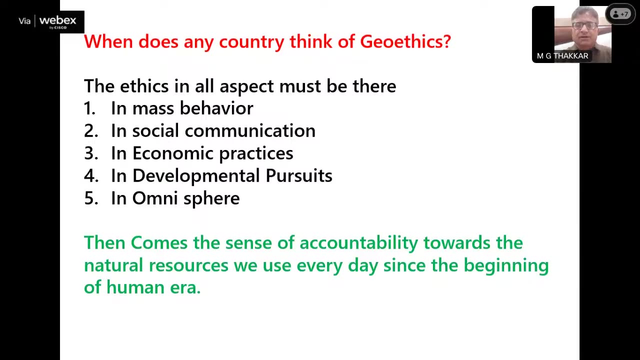 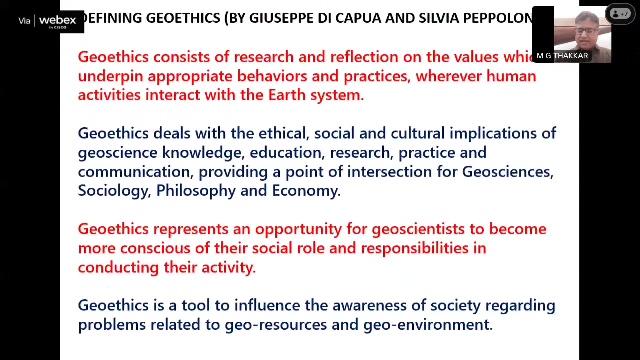 goal came, uh, in front of us. but before we go for the system as far as India is concerned, uh, we must learn about the geoethics, the stalwarts, those who are uh today, uh, uh, in the meeting. meeting, they have actually given the uh proper definition of the geoethics. okay, uh, can you change the slide? so we, uh, we now think we must think about. 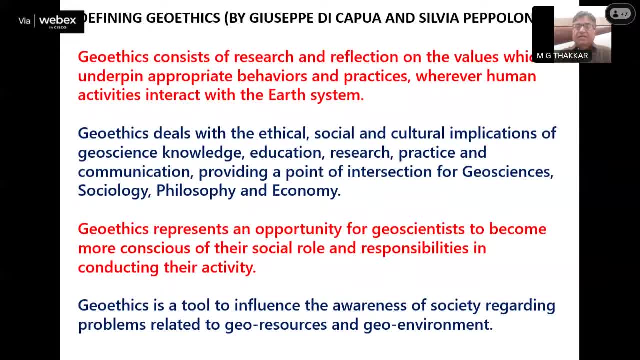 uh, when does any country? uh, think about geoethics? your ethics is a larger terminology, but before that we must think about the ethics in all sense. ethics in all aspects, in mass behavior. we should be more ethical in social Communications, in economic practices, in developmental pursuits, in Omni sphere. 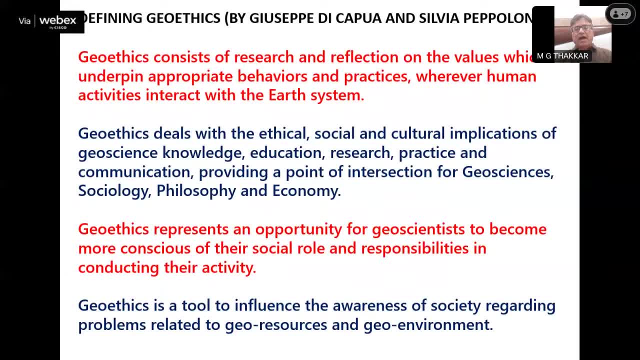 we have to be ethically strong, and then we actually think about the geoethics. so then comes the science of the accountability towards the natural resources we use every day. this is the beginning of the human era, but we are more concerned with the last two centuries, since 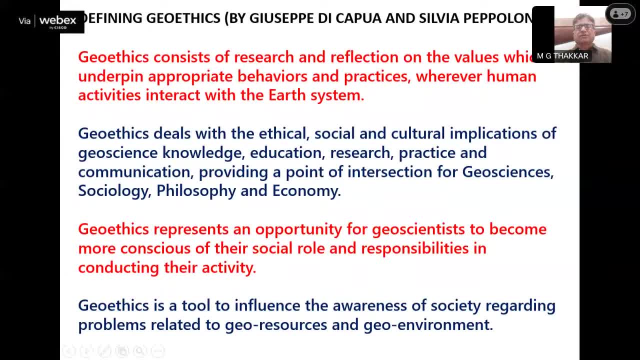 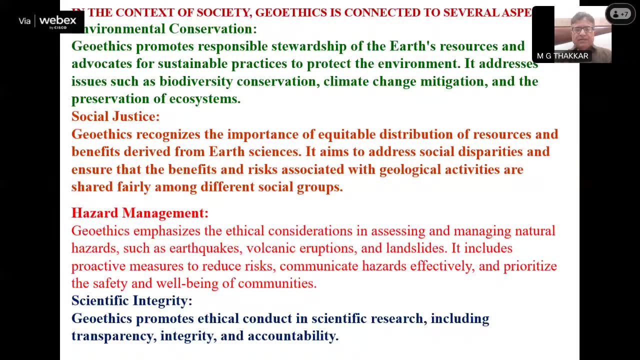 then we have industrial development and we have cut the mines and many other geological resources, natural resources, ruthlessly, so that this, actually this word, came so next, uh, defining this: geoethics: the uh, the, the uh. the speakers, today's speaker, they have actually uh given us these definitions, which I would like to read. 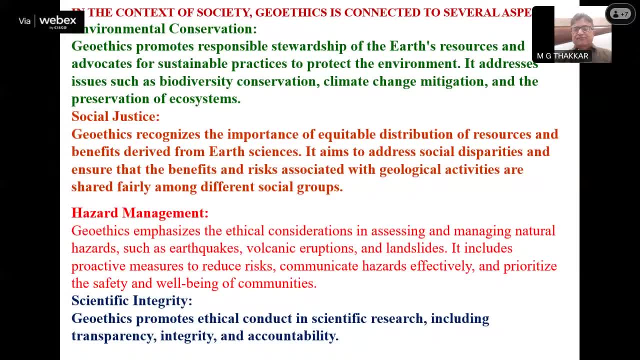 just now. geoethics consists of the research and reflection on the values which underpin appropriate behaviors and practices, ethical, social, cultural implications of science, knowledge, education, research, practices and Communications. providing a point of interactions for geosciences, sociology, philosophy. it represents an opportunity to do geoscience for geoscientists. 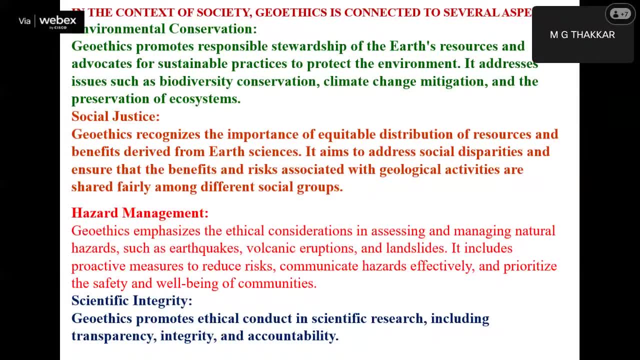 to become more conscious for their social role and responsibilities in conduct activity. it is a tool to influence the awareness of society regarding problems related to the geo resources and geo environment. so these are: this: encompass everything. you, if you have seen the definitions, uh, it means uh. it encompasses almost all spheres of the life which the human uh dome, we, we have. 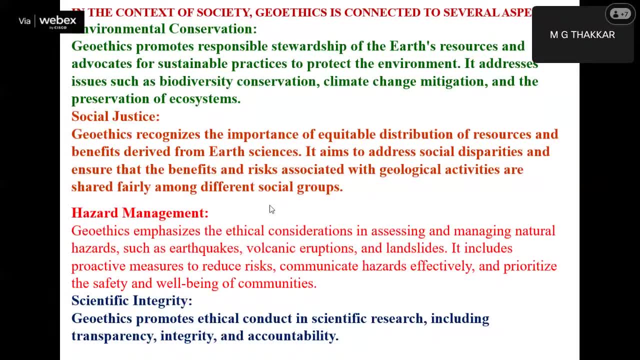 created. so, in context of the society, geoethics is connected to several aspects. one is environmental conservation. geoethics promotes responsible stewardship of the Earth's resources and threats for sustainable practices. to promote the environment, it addresses issues such as biodiversity, deconversion conservation, climate change mitigation and the preservations of ecosystems. in terms of the 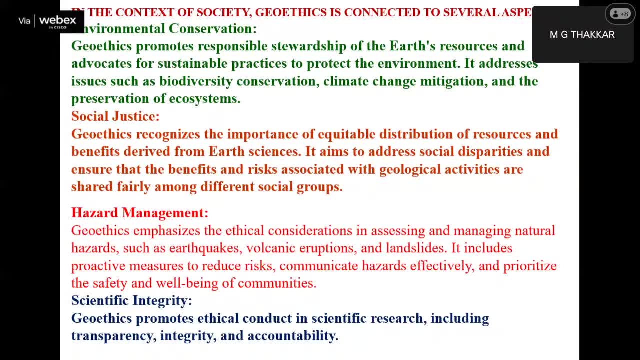 social Justice. Geoethics recognize the importance of equitable distributions of resources and benefits derived from the Earth's Sciences. it aims to address social disparities and ensure that the benefit and risk associated with geological activities are shared fairly among the different social groups. it also pertains to the hazard management because 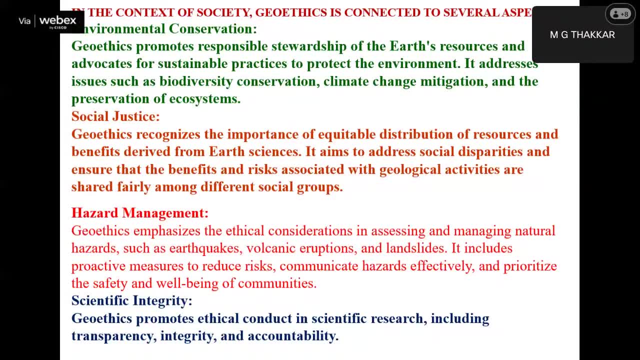 geoeuthics, Emphasize the uh ethical considerations in assessing the managing and managing natural hazards such as earthquake, volcanic eruptions, landslides. it includes proactive measures to reduce risk, communication issues um to mitigate hazard effectively and prioritizing the safety and well-being of the communities. 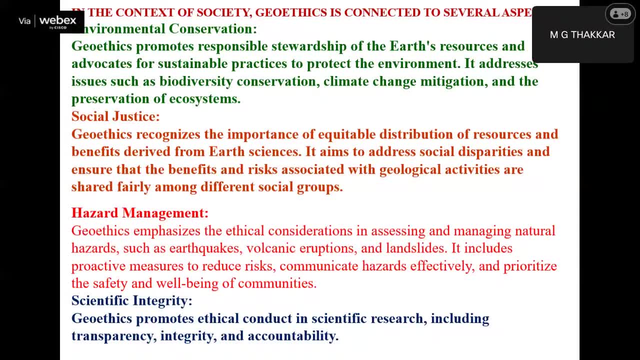 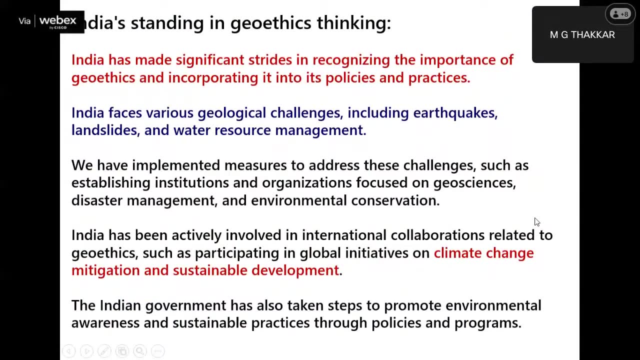 It also pertains to the scientific integrity that geoethics that promotes ethical conduct in scientific research, including the transparency, integrity and accountability. But looking to all these aspects, we should know that where the India is standing next, where India is standing in geoethics thinking, India has made significant strides in recognizing 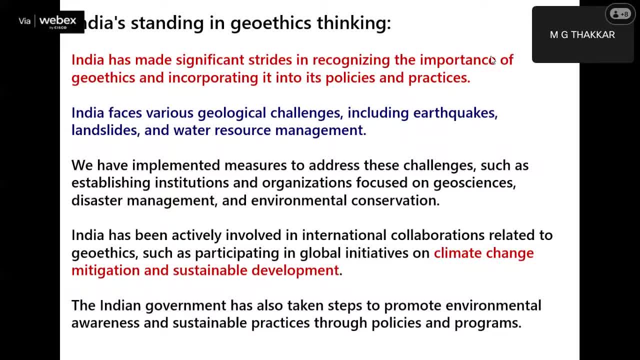 the importance of the geoethics and incorporating it into the policies and practices. India faces various challenges, including earthquakes in landslides and water resource management. We have implemented measures to address these challenges, such as establishing institutions and organizing Organizations focused on the geosciences, disaster management and environmental conservationists. 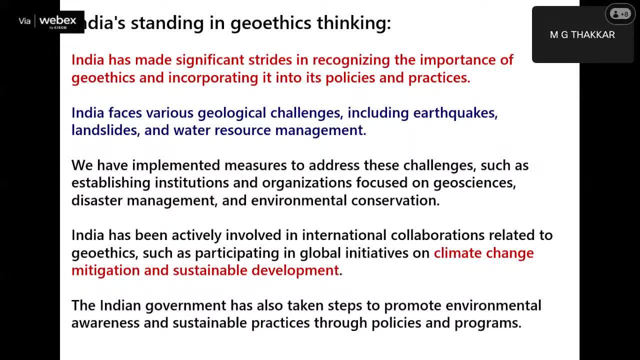 India has been actively involved in international collaborations related to the geoethics, such as participating in global initiatives on climate change mitigations and sustainable development. The Indian government has also taken steps to promote environmental awareness and sustainable practices through policies and programs. 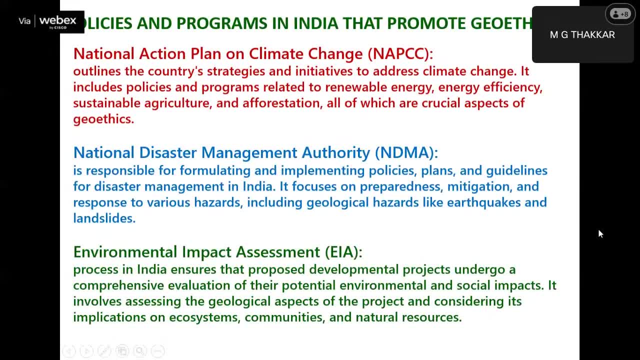 We will focus on some of the positive aspects which India has actually taken. All these stakeholders and the processes or the initiatives and missions. they might have some lapses, but the Indian government, government of India, and the state governments of each and every state, they have started several programs which basically, somewhere they 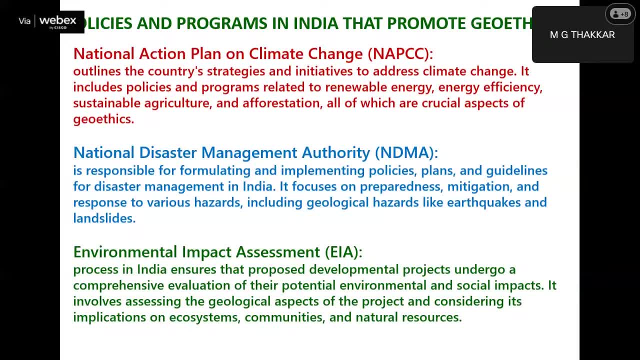 are actually touching to the geoethics. So we have some policies and programs. So let us look focus on some policies which the Indian government has taken over: The National Action Plan on Climate Change, NAPCC, which outlines the country's strategies. 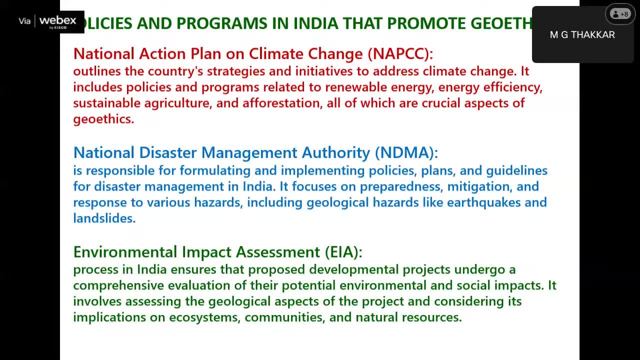 and initiatives to address climate change, and it includes policies and programs related to the renewable energy and climate change. Thank you. Now we have to look at the different factors which the government is taking, particularly the energy efficiency, sustainable agriculture and afforestation, all of which are crucial. 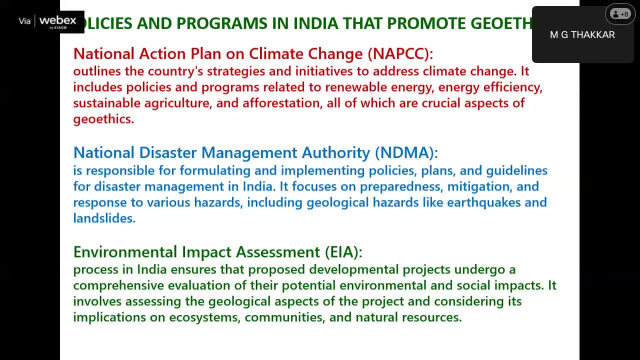 aspects of the geoethics. Another is National Disaster Management Authority. It is responsible for formulating and implementing policies, plans and guidelines for disaster management in India. It focuses on preparedness, mitigation and responses to various hazards, including geological hazards like earthquakes and volcanoes, and landslides. the environmental impact assessment. 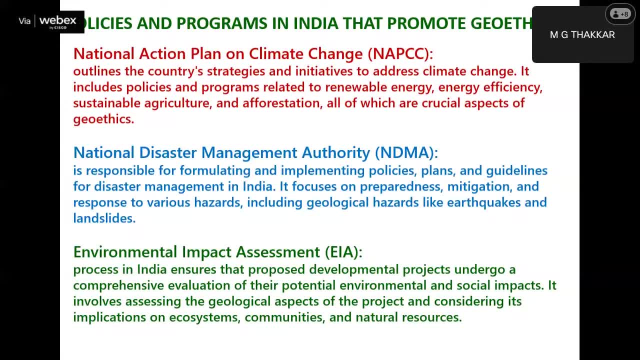 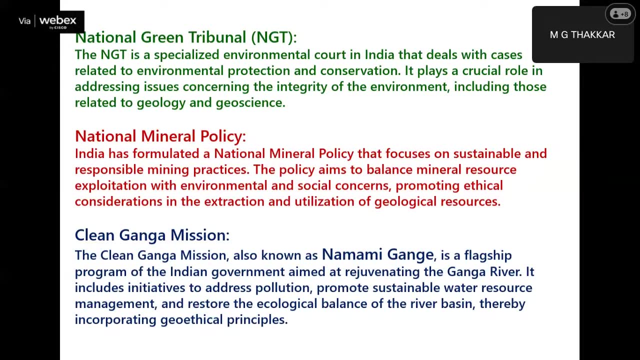 is one of the processes, which is also important in terms of the geoethics. another institution is a national green communal. this initiative ngt is specialized environmental court in india that deals with cases related to the environmental protections and conservations. it plays a crucial role in addressing issues concerning the integrity of the environment, including those 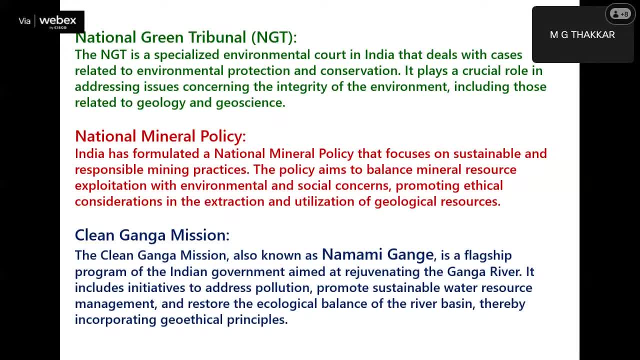 related to the geology and geosciences. the national mineral policy that india has formulated, national mineral policy that focuses on sustainable and responsible mining practices. so these all are basically our initiatives in india, but how far we really uh go in terms of the uh ideal geoethics, that is a big questions. but as far as the initiatives are concerned, we 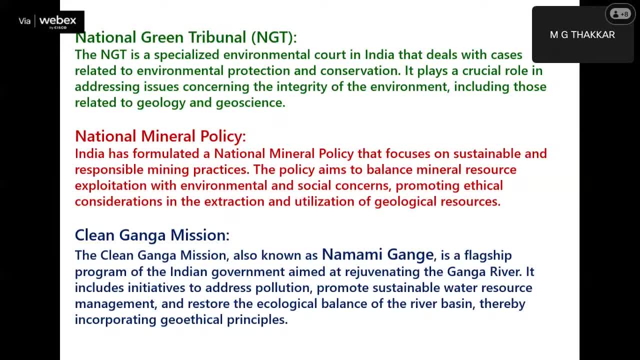 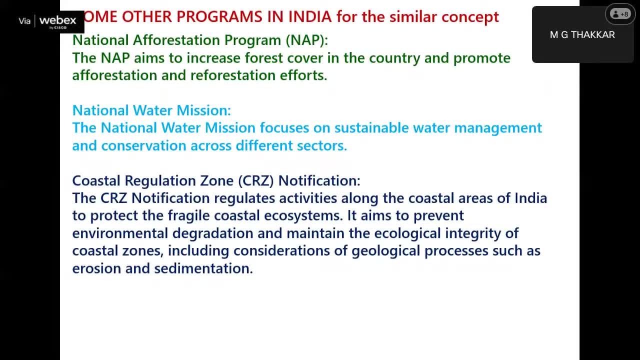 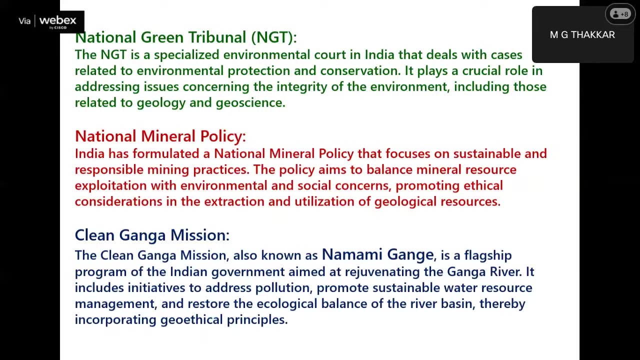 have done enough work. another mission is green, clean ganga mission that is also known as namami. ganga is a flagship program of the indian government aimed at rejuvenating the ganga river. it includes initiative to address pollution- pollution in the river and also to promote sustainable water resources management. and. 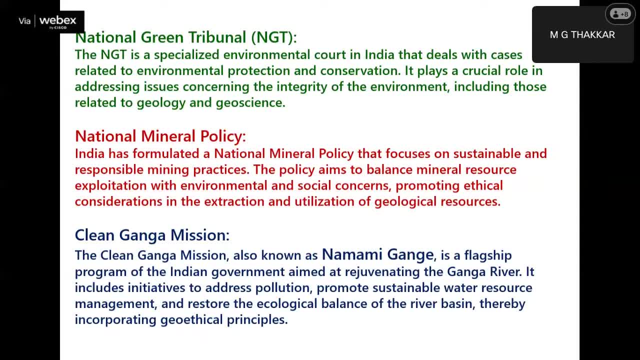 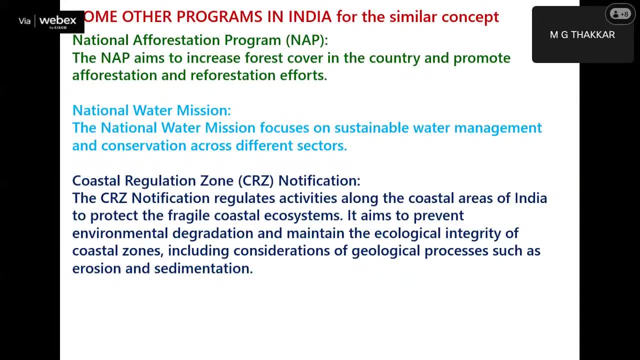 restore the ecological balance of the river basin, thereby incorporating geological, pre geoethics principles. some other programs are also there: the national afforestation program, national water missions, coastal regulation zone notifications- that also actually, uh, it comes under the umbrella of the large umbrella of the geo ethics. there are some other. 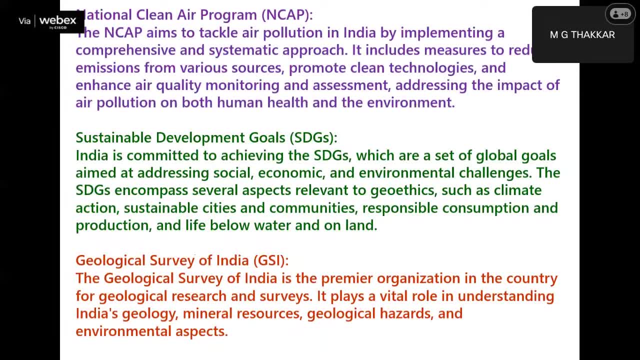 programs, national green clean air programs, sustainable development goals of the un, unesco. that also is taken care in most of these programs. gsi geological survey of india is also a prime uh premier organizations. i think it is 172 years old. this is the prime organization in the country for geological. 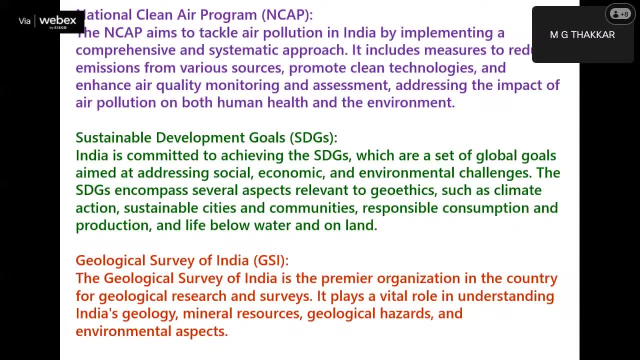 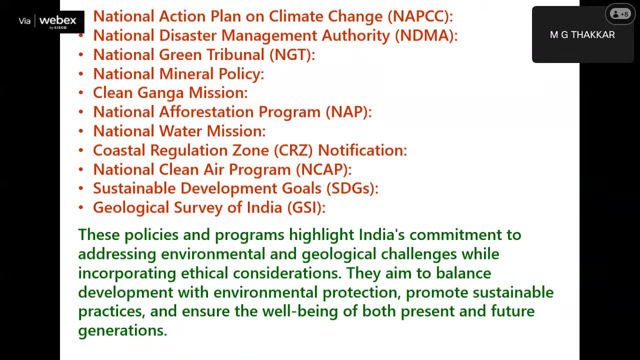 survey. It plays a vital role in understanding the India's geology, mineral resources, geological hazards and environmental aspects, So, by and large, to conserve, preserve and protect these geologically important sites. some natural sites of geological importance for the academic. 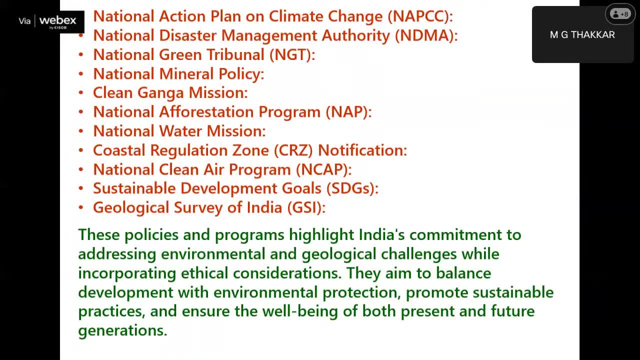 and research. the stakeholders. major stakeholders in India is Geological Survey of India And, I think, several sites they have actually conserved and preserved in India more than 50 sites are known and they have made a point of geotourism. So, looking to all these policies, the programs, 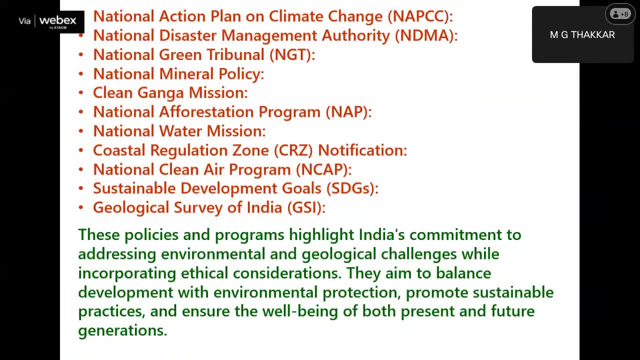 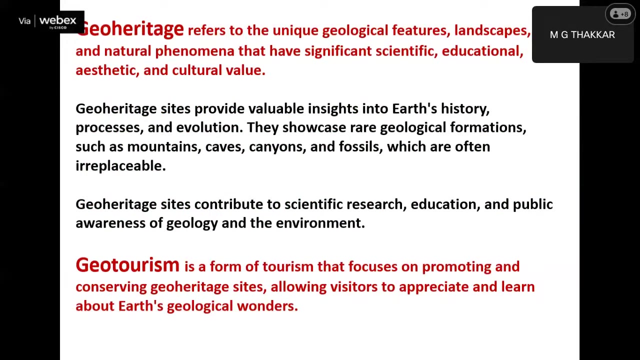 that highlight India's commitment to addressing environmental and geological challenges. while incorporating ethical considerations, they aim to balance development with environmental protection practices and ensure the well-being of both present and future. but really, do we really working on the protections as per the rules? which is actually applicable? 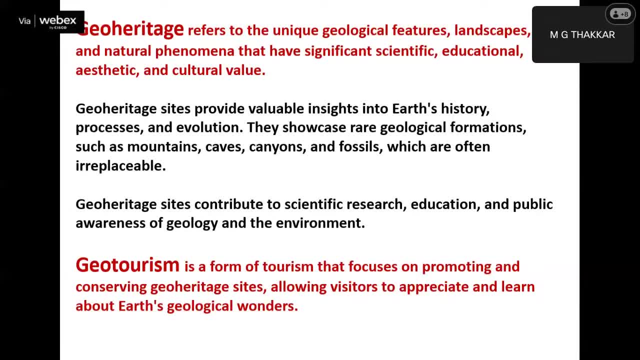 for the in the world and to make the Geopark, selecting several hundreds of geo-heritage sites. we have to think about it, not we still need further discussions about making the Geoparks and making, ultimately promoting, the geotourism. so so, geo heritage, as everybody knows that it refers to the 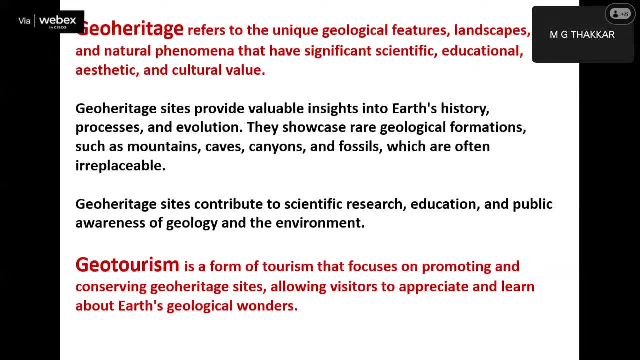 unique geological features, okay that landscapes or nature phenomena that have significant scientific and educational, aesthetics and cultural values. geo-heritage sites provide valuable insights into our history, processes and evolutions. they showcase our the rare geological land formations, mountains, caves, canyons, fossils, which are often 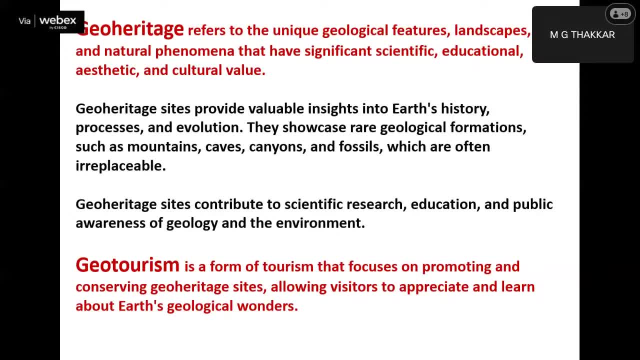 irreplaceable. so geo heritage sites contribute to scientific research, education and public awareness of geology and the environment. so how we can actually conserve and preserve this geo heritage site there is. the only one way we can do is geotourism, because it involves the 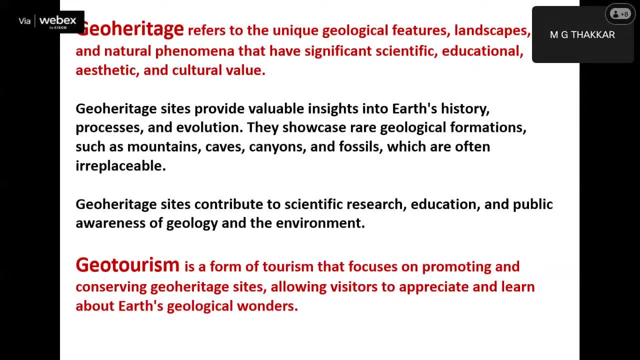 revenue. also, it involves the, the benefit to the government and also benefit to the society in terms of the, in terms of the getting knowledge. okay, so geotourism is a form of tourism that focuses on promoting geo, promoting and conserving the geo heritage sites, allowing visitors to appreciate the. 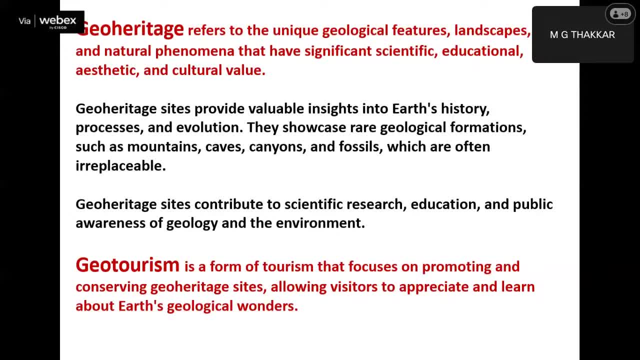 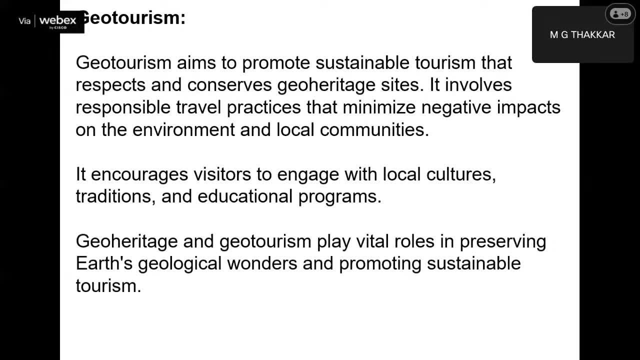 geological wonders and learn about Earth's geological wonders. it aims to promote sustainable tourism that respects and conserves geo heritage sites. it involves the responsible travel practices that minimize the negative impact on the environment and local communities. it also encourages visitors to engage with local cultures, traditions and educational programs. geo heritage and 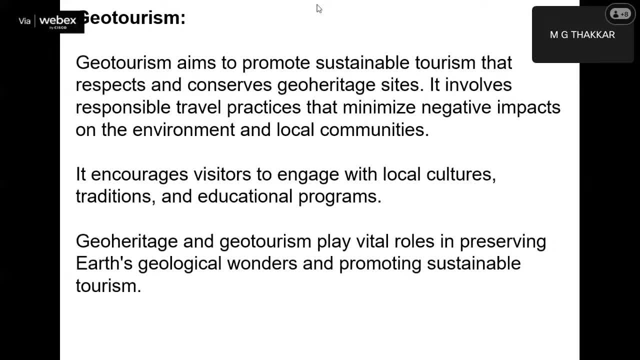 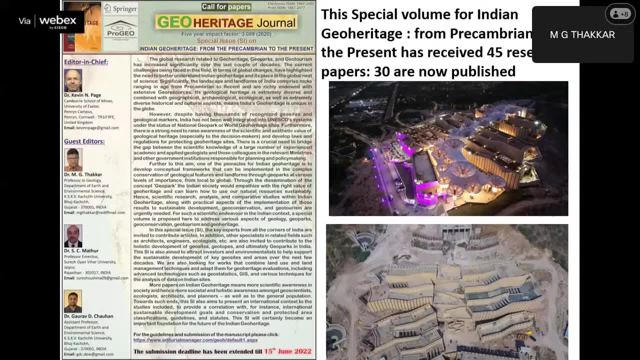 geotourism play vital role in the development of the geological heritage sites, preserving us geological wonders and promoting sustainable tourism. so looking to all these aspects- right from the geo ethics to geo heritage, to geotourism and conservations in india last several hundred, several times of years, maybe several decades- we have identified several. 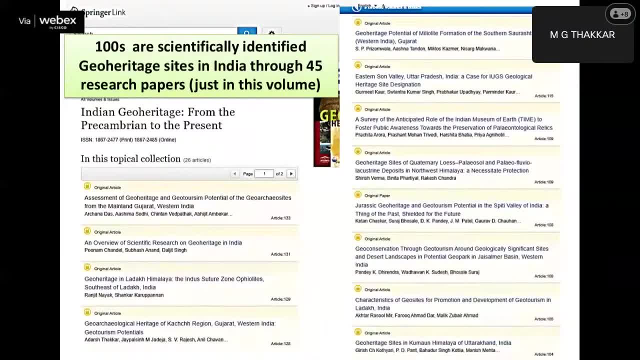 hundred sites, maybe more than 300 sites, have been identified in recent years. in recent years last, i mean last two years, uh, we proposed a separate volume in geo heritage, a separate volume, so indian volume name. that that special volume is named has as the: uh the indian geo heritage from the 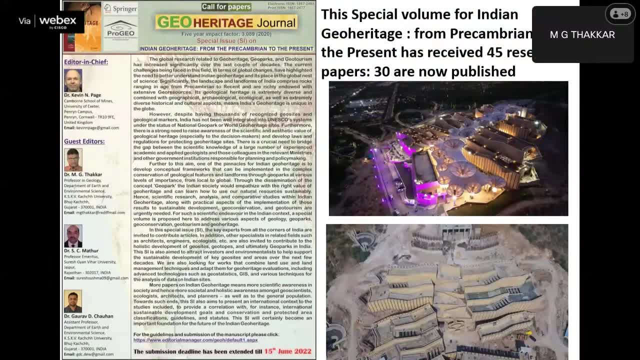 pre-cambrian. to the present, it has received more than 45 research papers and 30 are now published. the uh, the uh very important and striking- is in the history of the geo heritage journal, this is the largest volume, having 45 research papers. so this paper actually uh encompasses. 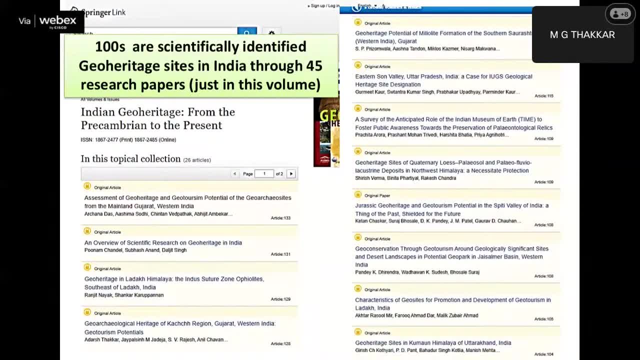 almost more than 100 geo heritage sites we have. i have just given the glimpses of some 30 uh published papers, name and what actually. it actually uh highlights different sites. so it is very interesting to see how we have identified several hundred sites geo heritage site. but are we 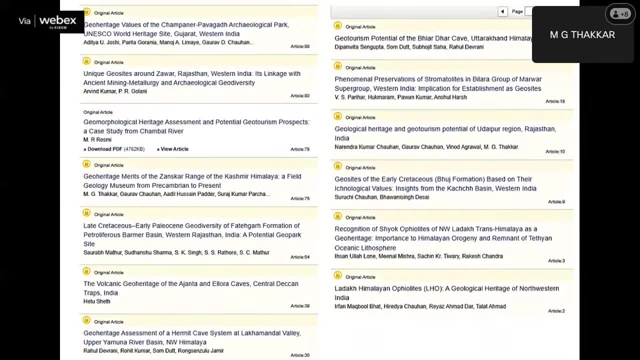 really capable enough to make the uh geo paths, which encompasses several, several geo heritage sites, with the criterias which international commission or the unesco has given uh regarding the land and some other infrastructural facility. since i have worked in kutch, mostly last three decades i have worked in kutch, so some of the couple of the sites actually we 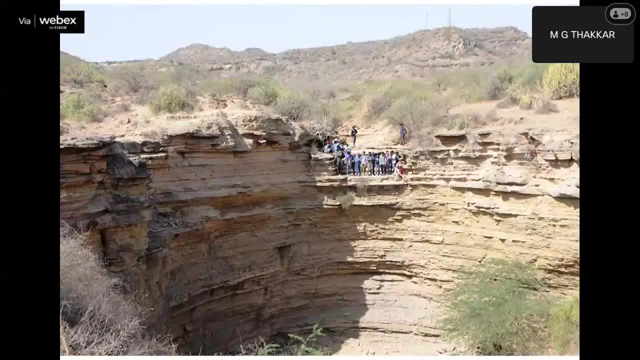 have identified some hundreds uh geo heritage sites in kutch, but here uh i can, because of the time constraint, i can show you only couple of geo-rated sites which are of very important and some of the sites which basically are now in the verge of uh vanishing. so let us have uh the the. 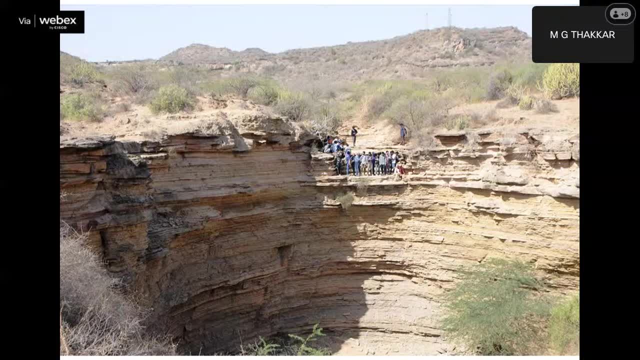 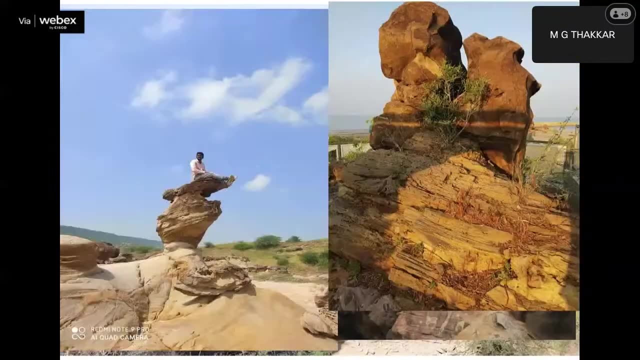 uh, kind of slideshow where you will see some of the sites. this is the sites where, uh, it is very important for the active tectonic point of view and near tectonic point of view. the big nick point: uh, this is a gorge. uh, next, it is a gorge which is within the periphery of the city. 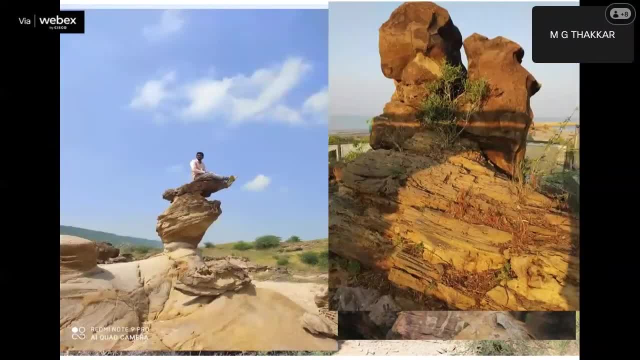 uh, then you can have several other uh geo heritage related sites which are of geomorphic, geomorphological, which is the geological importance, because kutch has jurassic and cenozoic geology, which is known to the world, which we have several uh hundreds of sites, out of which some of the sites which 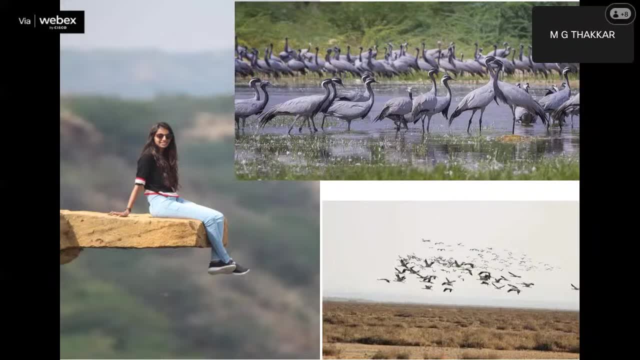 are ecologically important. let us look here some of the ecologically important sites in terms of the culture also. so these sites are now in the verge of actually verge of extinctions. if you look larger scenario, if you see in Gujarat maybe there are another 50 or 100 sites, I'm not 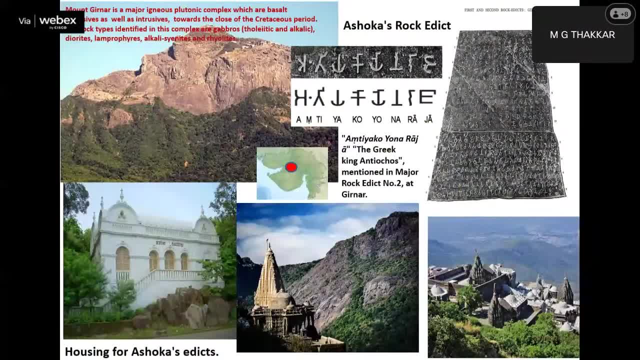 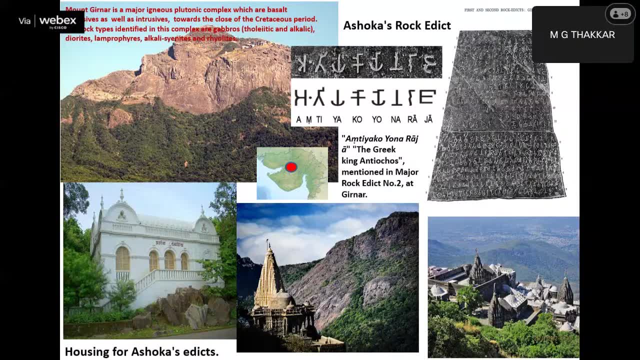 explaining each and every site, but this site it is very important in terms of the sea level changes Last 200,000 years of the sea level changes. there are very important features that shows that last interglacial period. So in terms of the quaternary to Mesothuike. 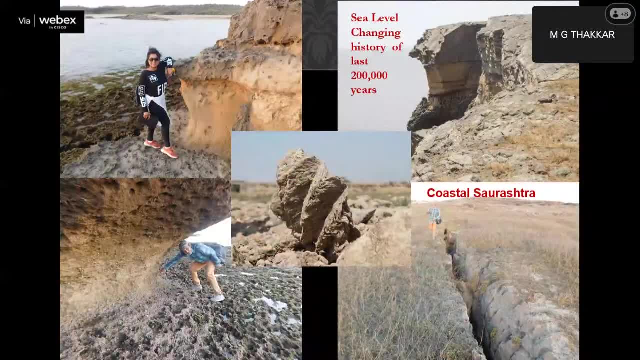 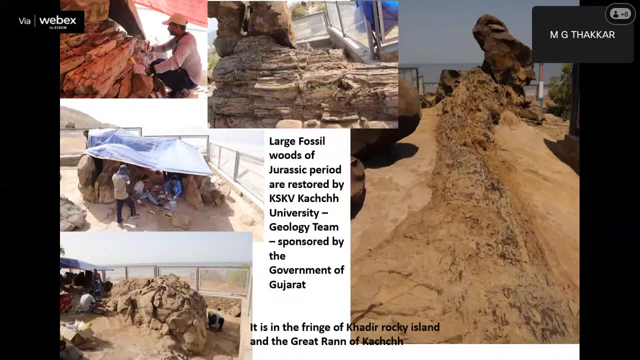 we have hundreds of georator sites, But out of these hundreds of sites in Gujarat, this is the only one site which we actually conserved and preserved, which is Jurassic Fossil Wood. This is basically. we got the funds from the government. 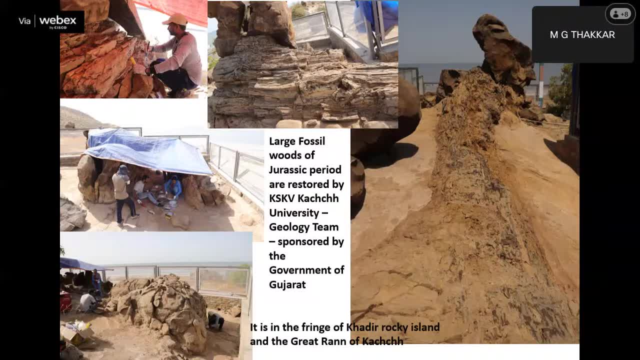 of Gujarat Ministry of Tourism, as well as the district administrator like collectors. So this is a very important site which we preserved. Earlier it was very in bad shape. this Jurassic Fossil Wood, Around this Jurassic Fossil Wood, we have found very good ecologically. 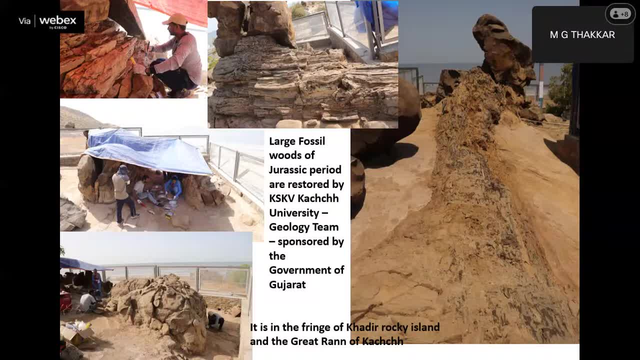 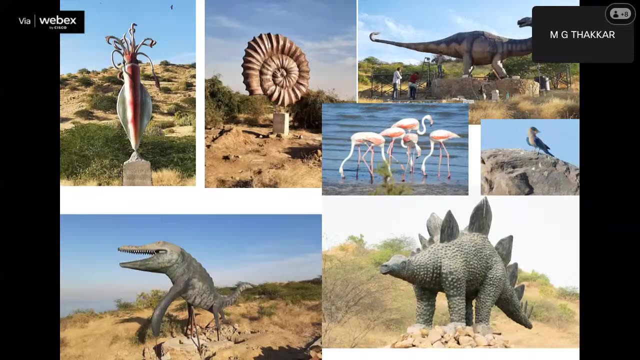 important sites. Next, you can see the Jurassic Fossil Wood site As migratory birds, frequently in the winter season they are coming. So by and large we can have a very good trail also. So in terms of the trail activities or the several 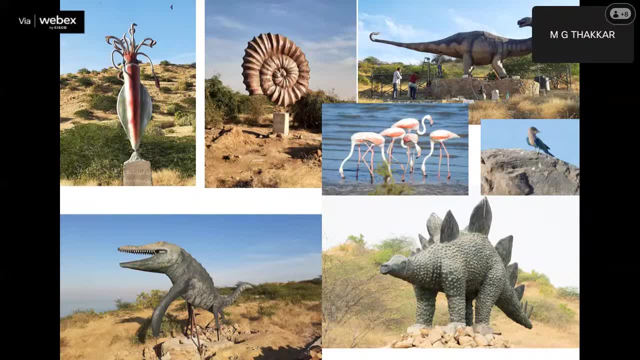 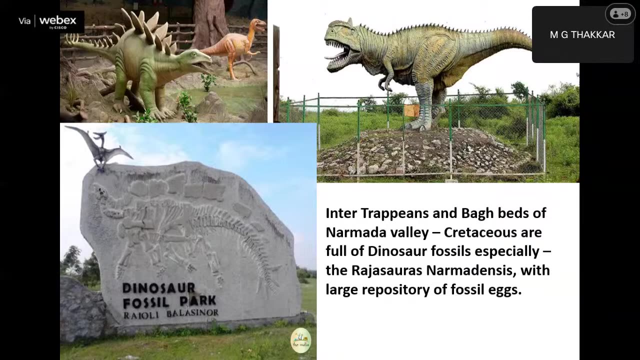 tablures of several vertebrates or invertebrate animals are also implanted over there, so that you can have a very good sense of closeness to the land. Next, you can see the Rhaeoli dinosaur park. This is one of the very important sites in. 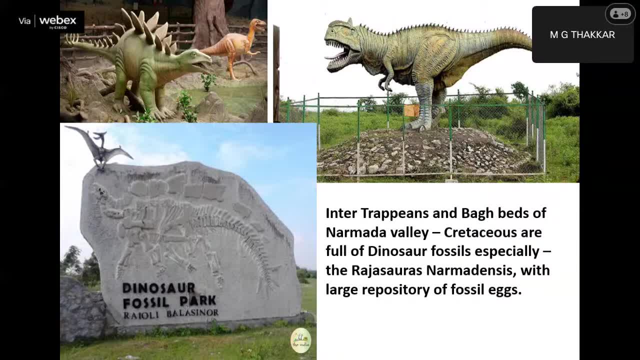 India, the Rajashorus dinosaur. It is actually Rhaeoli dinosaur park, which is well-developed. It is the only well-developed site in India, with almost investment of almost 60 to 70 crore rupees- And there is another site in Pooch, which is Agra. This is a large water. 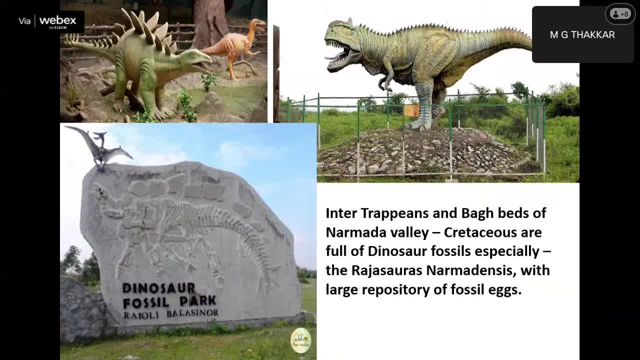 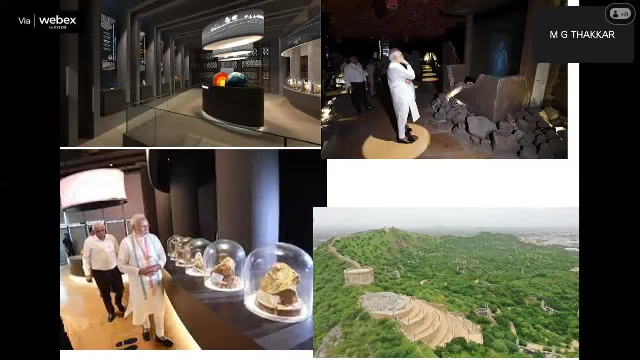 actually the dream project of our Prime Minister, Narendra Modi. It is actually earthquake museum. but actually this earthquake museum is we can convert it into the one of the geosites or geopark, because several hundred fossils are there and the processes with three-dimensional or 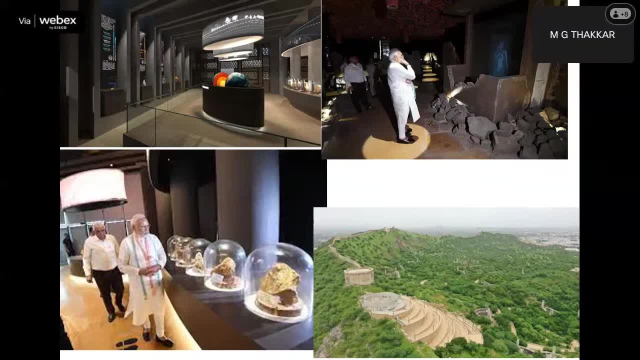 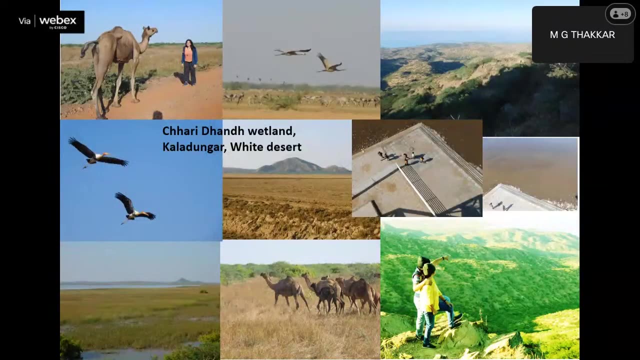 four-dimensional picturization is also given and it is one of its kind and it gives the actual earthquake and other scientific geological activities to the common people. So these are some of the sites which is going to be vanished within few days or few months. So next few slides. 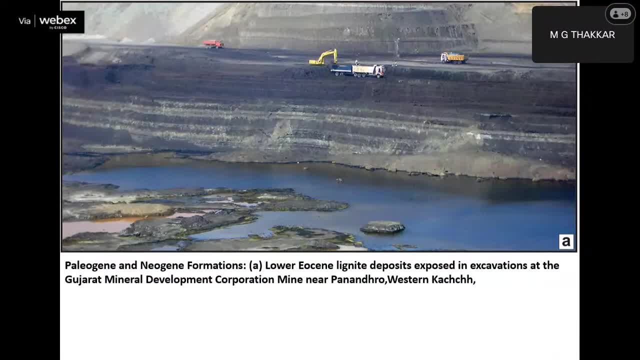 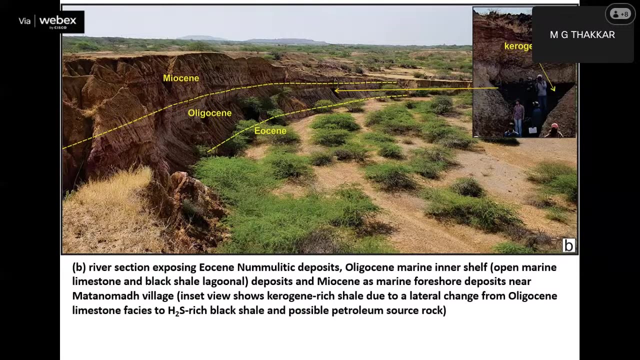 that is actually dedicated to the geologist. I think next few years you will see this kind of these sites and these are very important in terms of the several geological processes- PETM process or any paleocene-eocene boundary, eocene-olecocene boundary, formation of the petrochemicals or hydrocarbons. 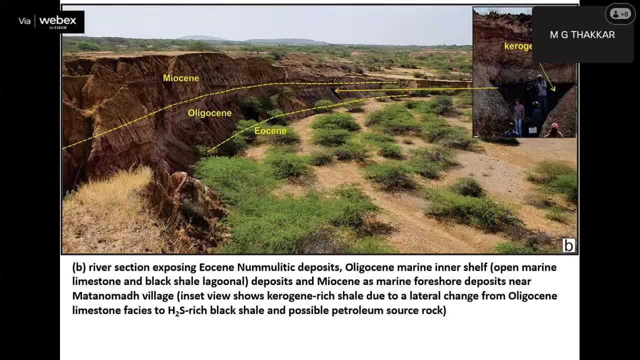 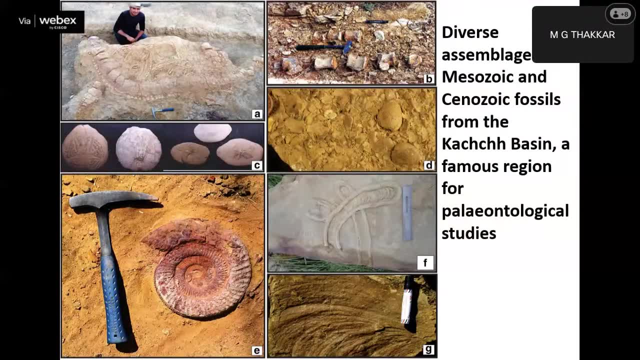 This site is very important and I think within few days, this condensed section of eocene-olecocene-myocene is going to be vanished. So we have to now think about the future generation geologist, but since we have started the practices of geotourism, 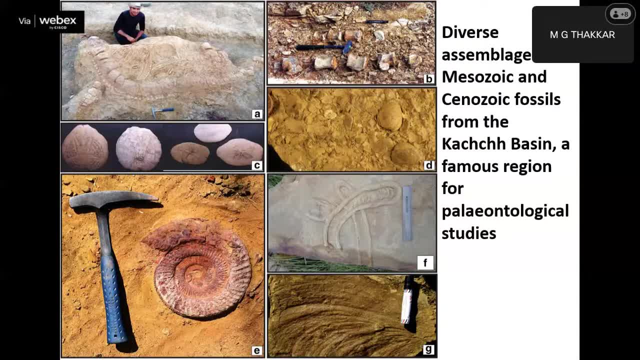 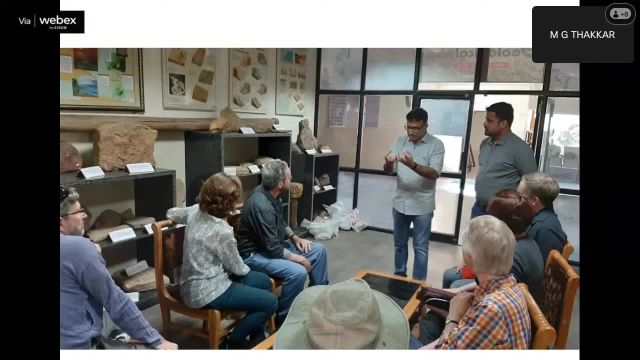 I think we will be able to at least conserve some of these sites With our efforts. when I was in Kutch University, we actually formed this department of Earth and Environmental Science where there is a state of art museum where almost 10 000 fossils and other rock collections are there. 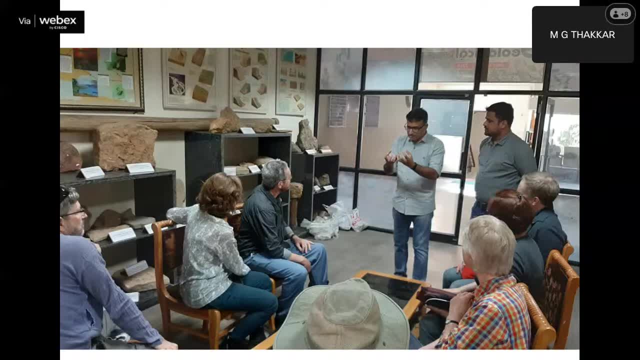 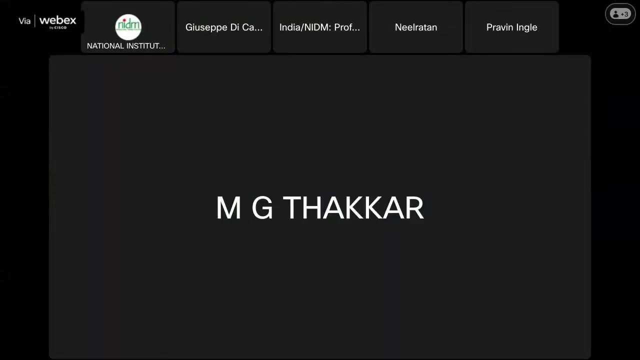 for the those. actually they wants to study intricately the culture, geology. so such kind of uh practices can also be started in a cluster level in each uh area so that we can at least preserve some of these specimens. thank you next. thank you very much. i think you have given a brief description how. 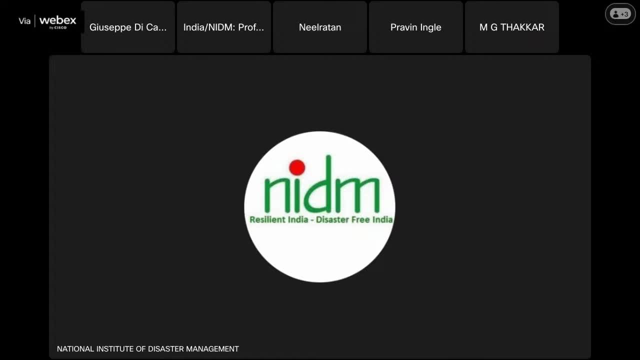 you are working towards saving the geo heritage sites. hello, yes, am i audible, sir? yeah, yeah, thank you very much, sir, for joining us and, uh, i think i cannot see sir. any question now. if it will be, we will share you over the email. oh, sure, so i think. 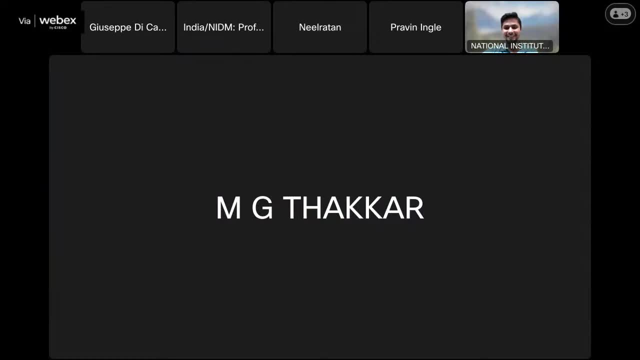 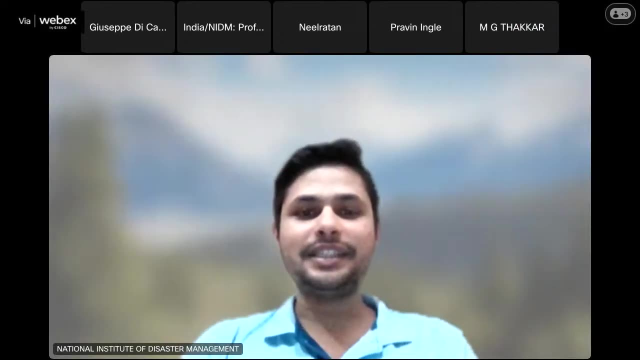 it is over the time, five minutes, uh over, yes, yes. now moving to our next speaker, dr sylvia papaloni, italian geologist, researcher in the field of natural hazards and risk science writer, also sees an international frontline scholar on geoethics. in 1996 she earned her master's degree on 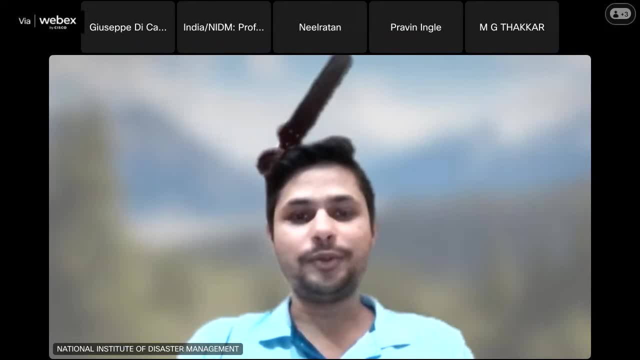 geosciences from spangia university of rome. in 1997 she obtained the professional qualification and enrolled in the geologist register and in 2001 received her phd in earth sciences. a phd geologist researcher and currently a researcher at national institute of geophysics. 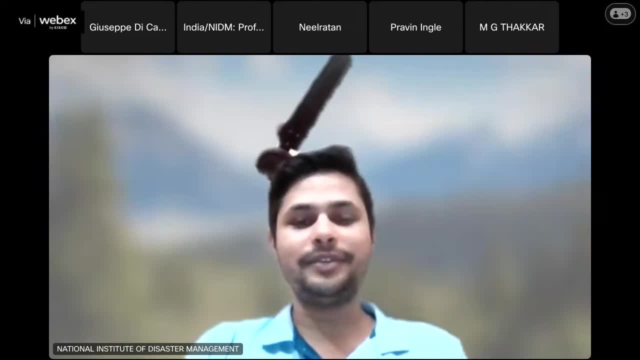 and volcanology, rome, italy. her scientific activities are focused on natural risk and hazards, geomorphology, engineering, geology and ethical and social aspects of earth sciences. she is founding member and general secretary of international association for promoting geoethics and she is known for her fundamental contribution to 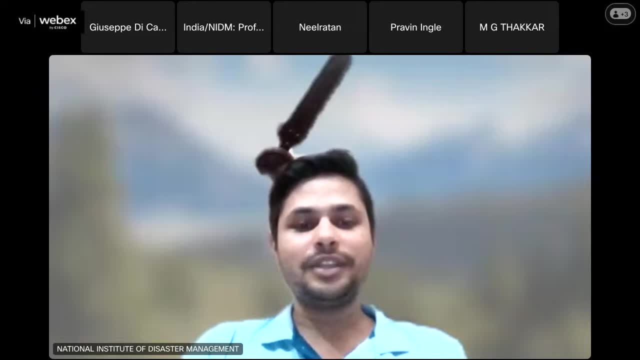 development and promotion of geoethics. she is working on creating awareness about the growing impact of human activities on biogeological system and how to promote geoethics as a responsible way of thinking and managing the planet for creating safe and healthy interaction among humans and 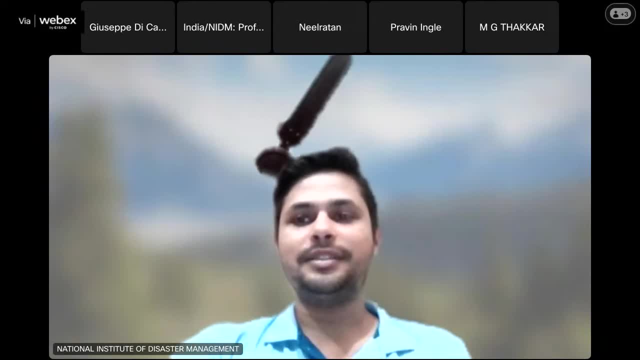 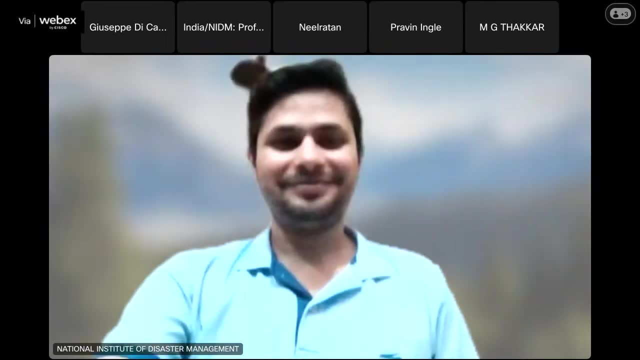 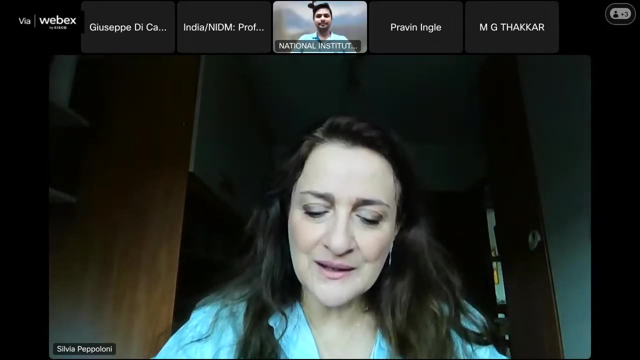 other biotic and abiotic entities forming the earth system. with this i welcome you, ma'am, and thank you very much for joining us today over to you man afternoon, everybody, and thank you for this introduction. uh, first of all, allow me to to thank professor parkash and the ipg india for the kind 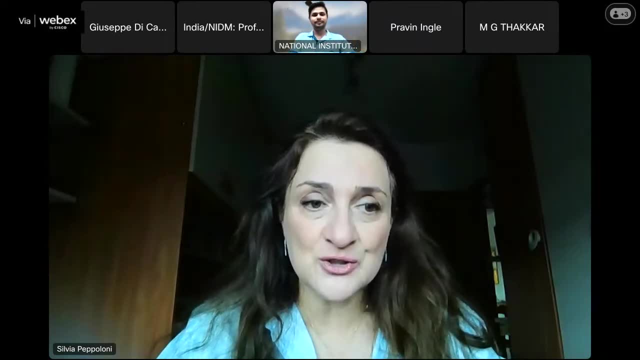 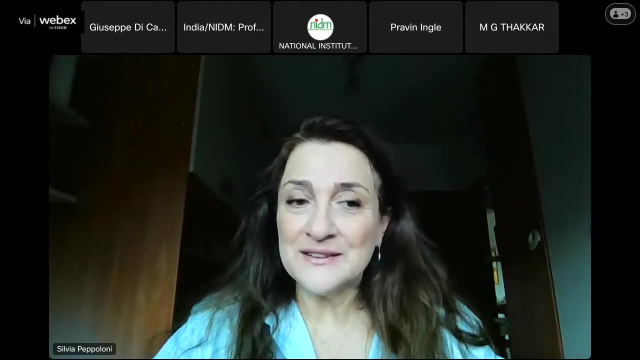 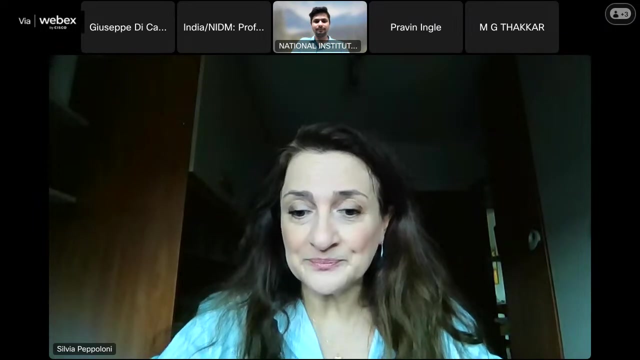 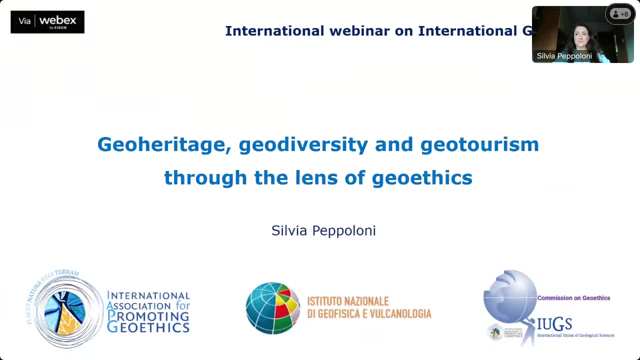 invitation to this webinar to celebrate the international geoethics day 2023. i'm impressed by by the great efforts that you have done and you are doing uh to develop uh geoethics in india and countries. um, i'll show my video. um, okay, okay, it works okay, well, i would like to introduce the concept of 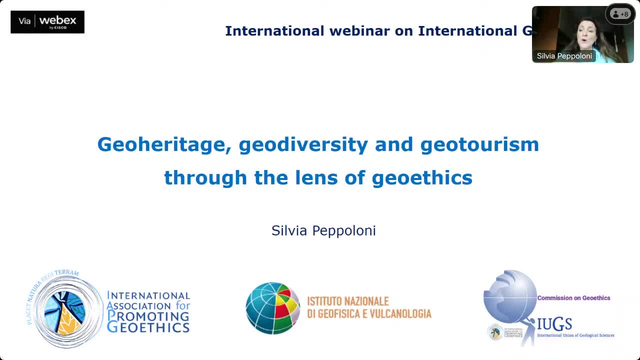 diversity and conservation and to analyze their meaning from a geological perspective, in other words, to explore the meaning from a geological perspective. so i would like to share with you a concept of geodiversity and geoconservation, their ethical and societal relevance, both for the geoscience community and society. 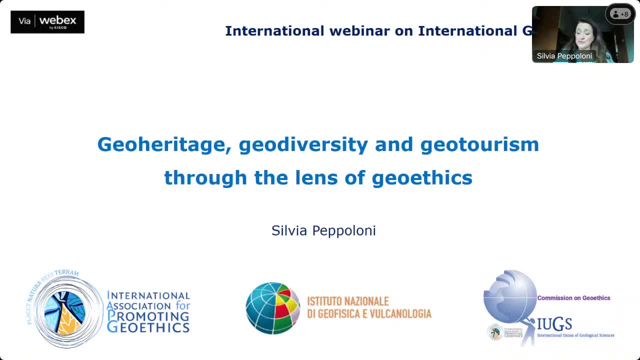 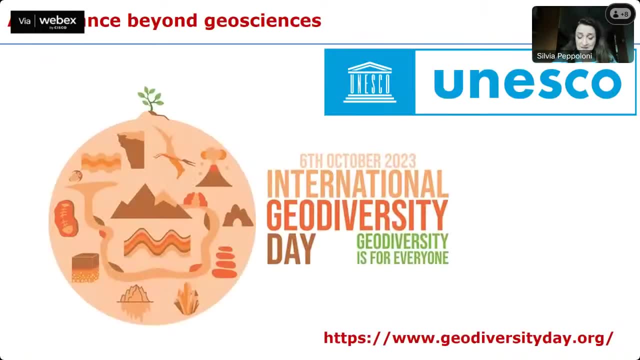 in line in line with the presentation of professor tankard before me. well, the concept of our geodiversity and your heritage, as well as geoconservation, have assumed great importance for the geoscience community and are getting a relevance also beyond the geosciences. 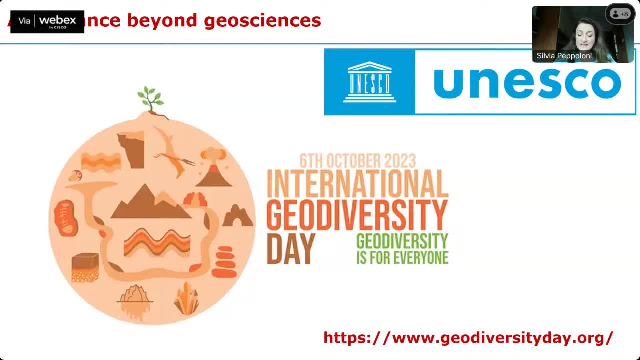 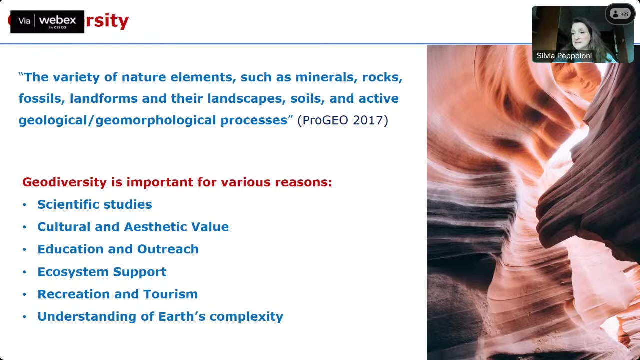 particularly. the concept of geodiversity is now internationally recognized for its importance for human beings and biodiversity, after the recent establishment of the international geodiversity day by unesco on 6 october of every year. but let's give some definitions to clarify this concept. geodiversity is the variety of natural elements such as minerals, rocks. 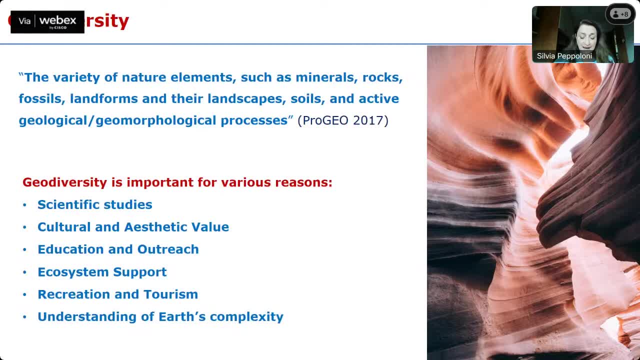 fossils, landforms and their landscapes, soils, and active geological, geomorphological processes that form and alter them and sustain life. so geodiversity underscores the various ways in which earth's geological history has manifested within a specific region. just as biodiversity encompasses the range of living organisms in an ecosystem, geodiversity encompasses the range of geological elements in a landscape. 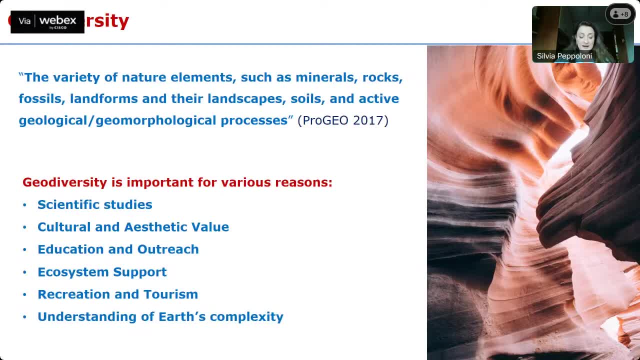 it recognizes that the earth's surface is a dynamic mosaic of geological processes and formations, each with its own unique history and significance. understanding and conserving geodiversity are important actions for various reasons. first of all, for scientific studies, geodiversity provides valuable insight into earth's histories, past environmental conditions. 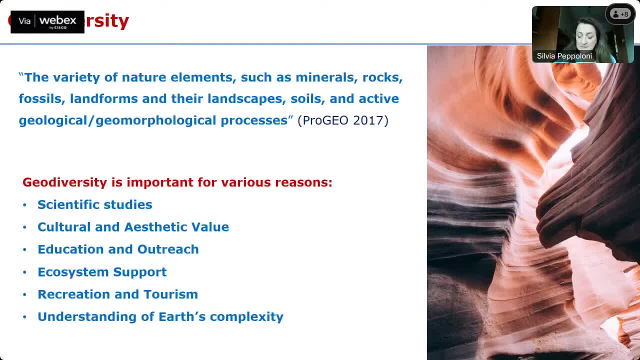 and the processes that have shaped our planet. it aids scientists in studies of land용 nutzen. geological史. he georgia, prada. an المفضلves for geogmus on labrador, of請 historical or artistic value for communities and also an education and outreach value. 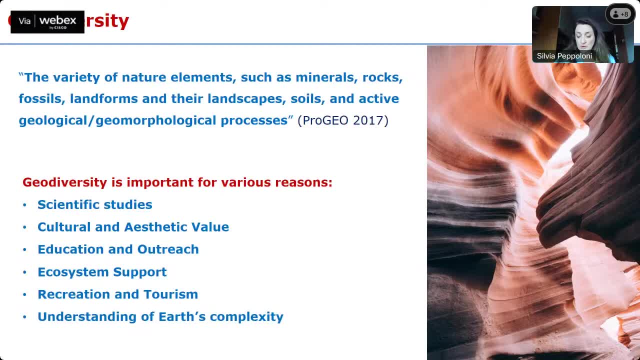 Geodiversity is a valuable educational tool helping to raise awareness about Earth's geological history and processes. It engages the public in understanding the dynamic nature of our planet. Ecosystem support. Geological features can influence local ecosystems by affecting soil types, water availability and habitat diversity. Protecting geodiversity can 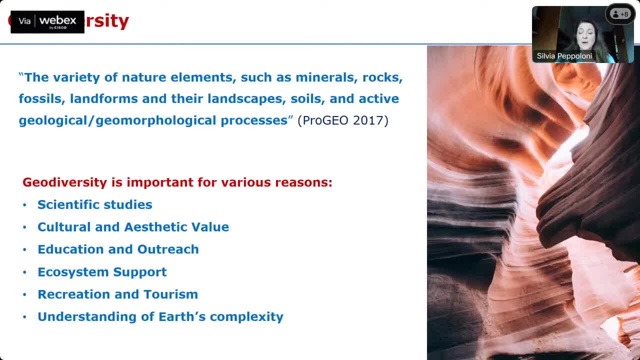 and directly contribute to biodiversity conservation, Recreation and tourism. Unique geological formations and landscape often attract tourists and outdoor enthusiasts, contributing to local communities and economies. Overall, geodiversity is a fundamental aspect of the natural world that complements biodiversity and cultural diversity, contributing to a holistic 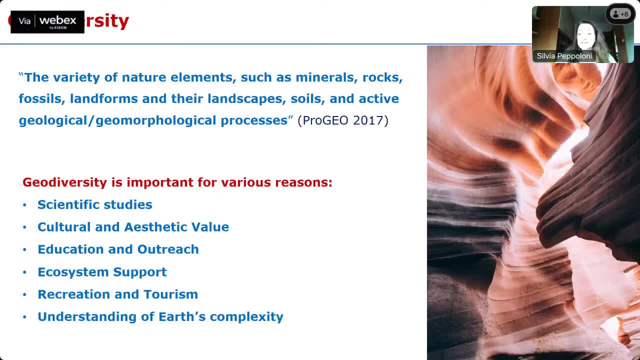 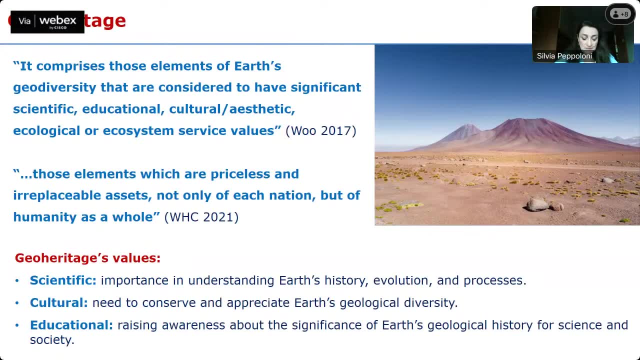 understanding of Earth's complexity and the interconnection of its various components. Geoheritance. Geoheritage comprises those elements of Earth's geodiversity that are considered to have significant scientific, educational, cultural, aesthetic, ecological or ecosystem service values, Meaning those elements which are priceless and irreplaceable assets, not only of each nation, but 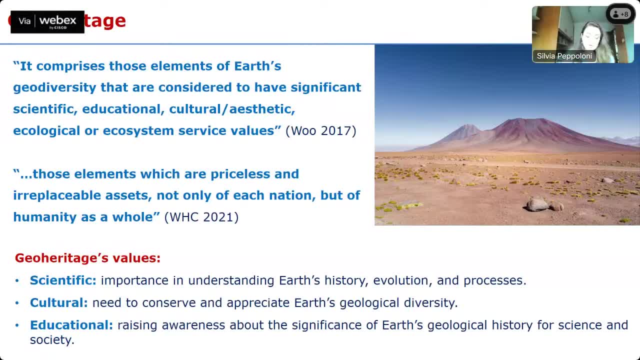 of humanity as a whole. So geoheritage refers to the unique geological features, landscapes and sites of geological significance that hold scientific, educational, cultural and aesthetic values. These features are often preserved and protected because of their importance in understanding Earth's history, evolution and processes. These features are often preserved and protected because of their importance in understanding Earth's history, evolution and processes. 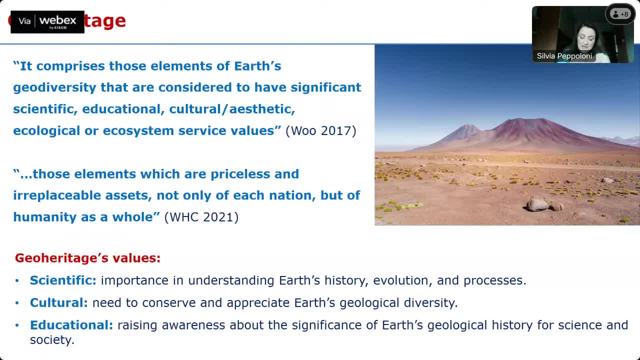 The concept of geoheritage emphasizes the need to conserve and appreciate Earth's geodiversity, similar to the conservation efforts directed towards biodiversity and cultural heritage. It also plays a role in education and rising awareness about the significance of Earth's geological history for science and society. 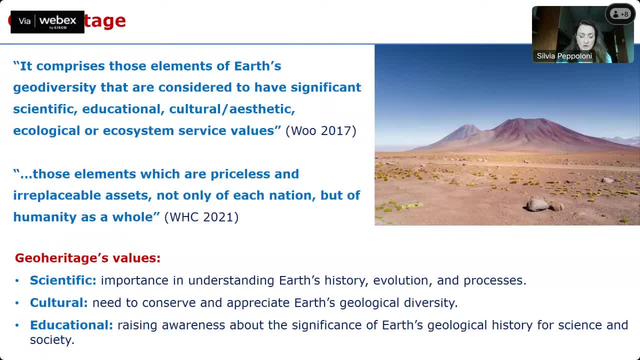 It also plays a role in education and rising awareness about the significance of Earth's geological history for science and society. It also plays a role in education and rising awareness about the significance of Earth's geological history for science and society, And geoconservation. 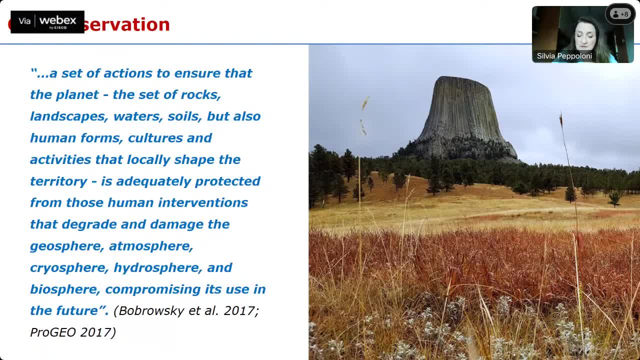 Finally, geoconservation consists of a set of actions. Finally, geoconservation consists of a set of actions to ensure that the planet, that is, the set of rocks, landscape, water, soils, but also human forms, cultures and activities that locally shape the territory. 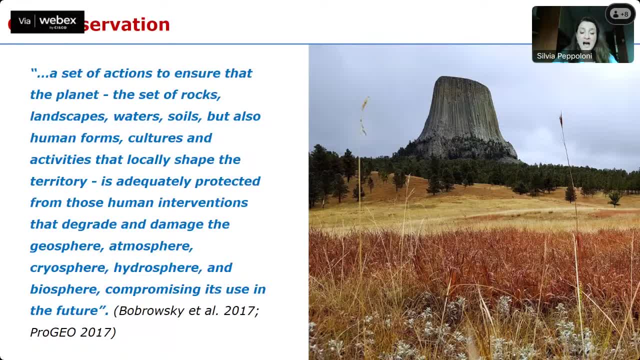 is adequately protected from those human interventions that degrade and die of human intervention. These are the two main why we must take action, Damage the earth system, compromising its use in the future. So, Joe, conservation refers to active and deliberate efforts To protect, to conserve and to manage. 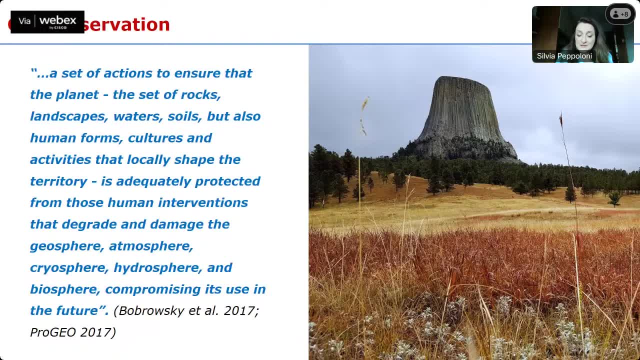 Earth's geo heritage, including its diverse Geological features, landscapes and processes. Similar to the conservation of biodiversity and cultural heritage, Joe conservation focuses specifically On preserving the planets geo diversity And the scientific, educational, cultural and aesthetic Values associated with it. Well, 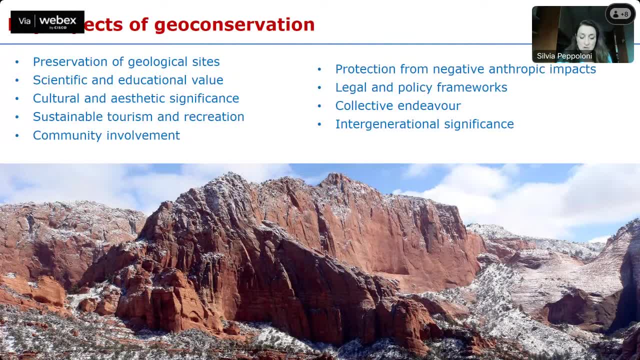 Key aspects of geo conservation. geo conservation includes Preservation of geological Sites. geoconservation involves identifying, designating and managing the specific geological sites and landscapes of importance. These sites can include unique rock formations, Fossil beds, mineral deposits, volcanic features and other geological elements. 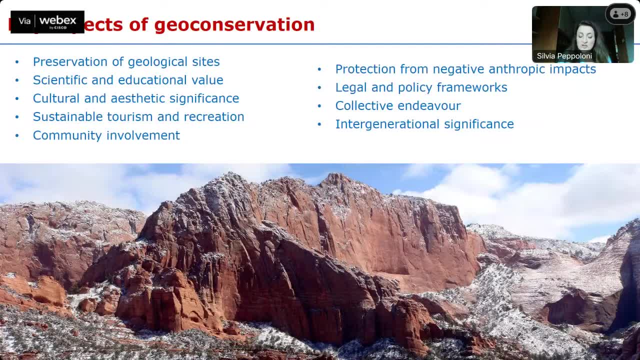 Scientific and educational value. Geoconservation emphasizes The scientific knowledge that can be gained From studying earth's geological history. Preserving geological sites provides opportunities for research, education And rising public awareness about earth's past And processes that have shaped it. 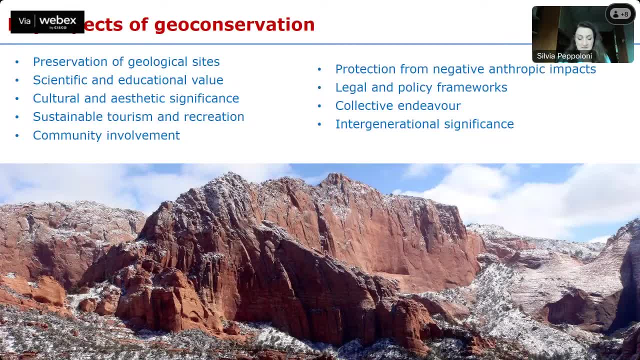 Cultural and aesthetic significance. Geological feature often hold Cultural and aesthetic value For local communities and society at large. Geo conservation helps maintain this connections to the past And fosters an appreciation for the natural beauty of earth, landscapes, Sustainable tourism and recreation. 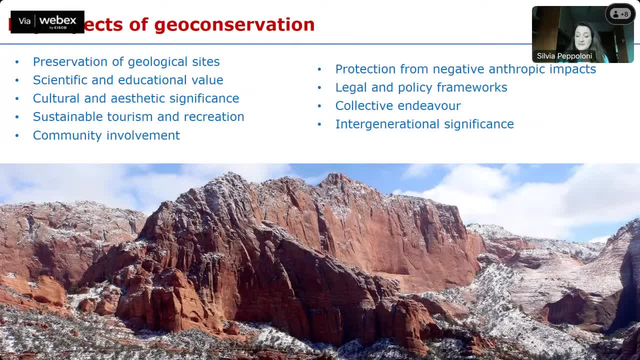 Geoconservation can support the development of responsible tourism and recreational activities that allow people to experience and learn from geological sites while minimizing negative impacts. community involvement: yes, engaging local communities in geoconservation efforts fosters a sense of ownership and encourage stewardship of geological sites. collaborative efforts ensure the sustainability. 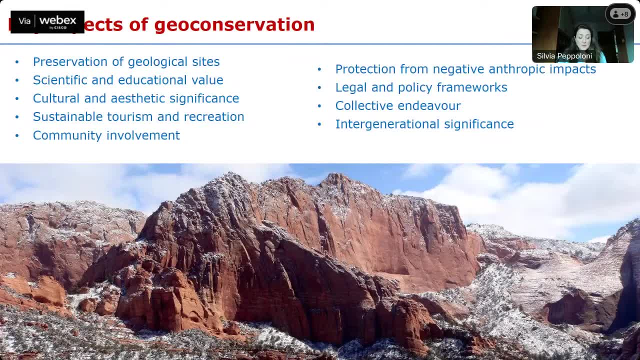 of conservation initiatives, protection from negative human impacts, engaging local communities to mitigate potential threats to geo heritage, such as urbanization, industrial development, mining and erosion, which can degrade or destroy valuable geological features. and more legal and policy frameworks. geoconservation often involves establishing legal protections, management plans and policies to ensure the long-term preservation of geological sites and 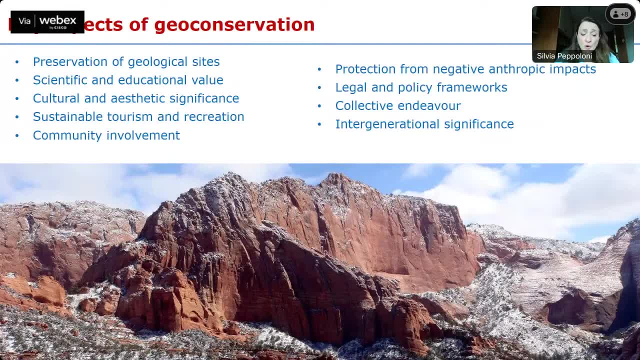 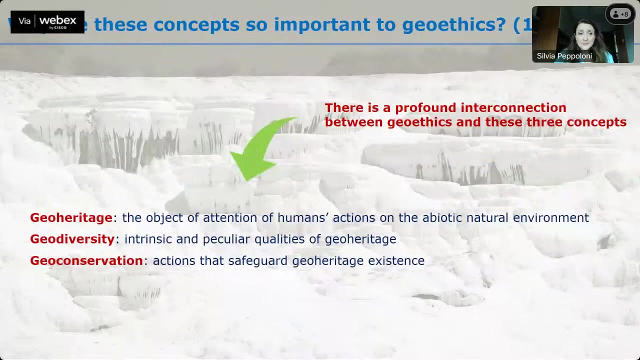 landscapes. and, finally, collective endeavor. geoconservation is an endeavor that involves all the components of a community- geoscientists, educators, politicians, policy makers, local communities and conservationists- in protecting geological sites and managing resource responsibly, even in the perspective of preserving sites for current and future generation, and therein lies its intergenerational significance. well, why are these? 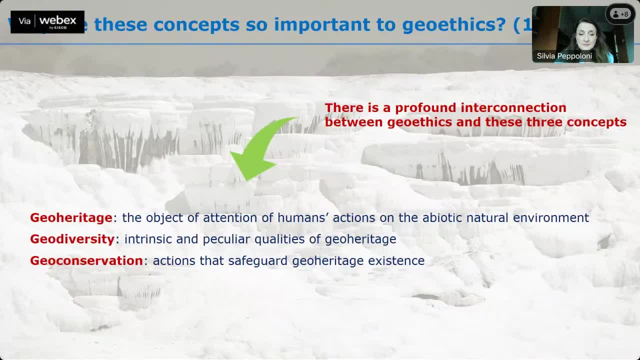 concepts so important to geoethics. there is a profound interconnection between, in this concept, geo heritage, diversity and geoconservation, respectively, identify the object of attention of human's action on the abiotic natural environment, and that is heritage, its intrinsic and peculiar qualities, geodiversity. 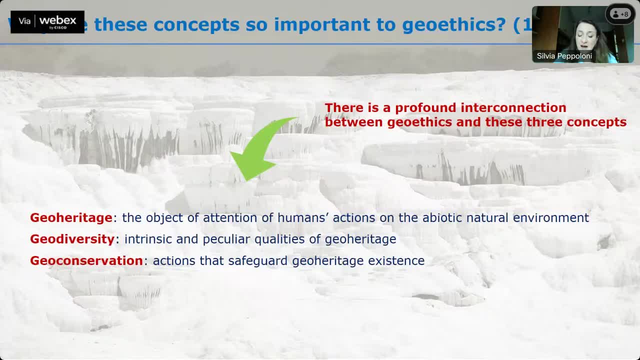 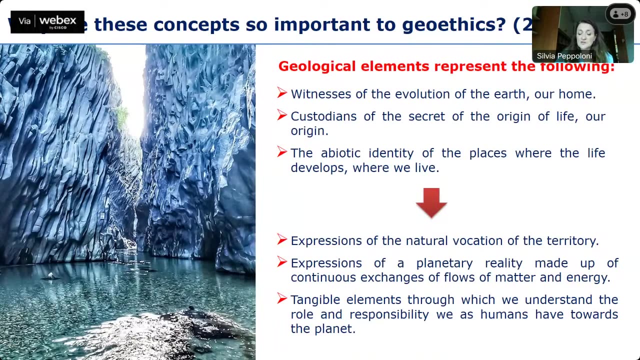 and the actually Actions that safeguard its existence. Joe conservation, Even in in a context of natural evolution. In the geological vision, the geological elements such as geosites, geological landscape And landforms are not considered simple components of the territory. 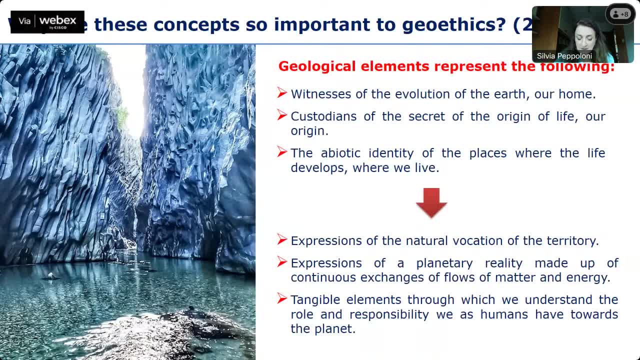 Which stimulate human curiosity. They are the witnesses Of the evolution of the earth, our own. They guard the secret of the origin of life, Our origin. they constitute the abiotic identity of the places We leave, The bedrock of those social, ecological systems in which forms and processes of human communities are 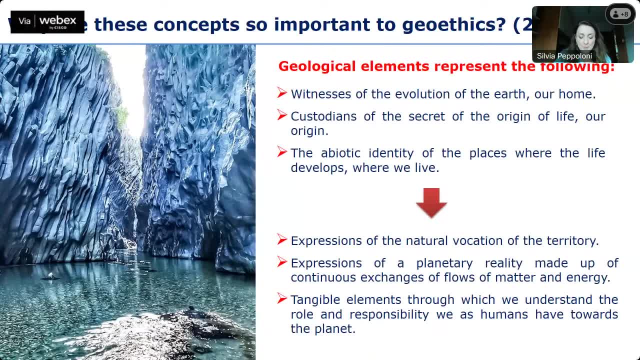 Interpret, Created in the forms and processes of natural ecosystems And for these reasons they express the natural vocation of the territory. They are geomorphological expressions Of a planetary reality made up of continuous exchanges, Material and immaterial, of flows of matter. 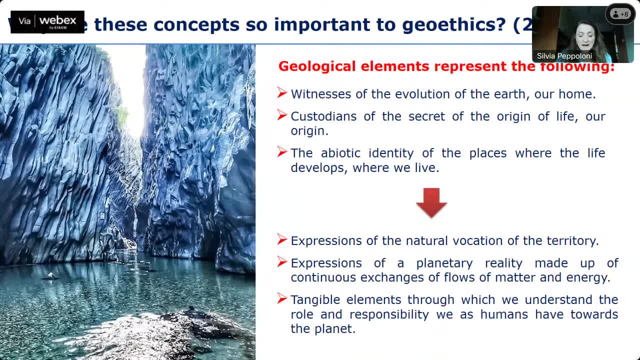 And energy between its constituent bio, Logical and mineral paths. And, finally, they are the tangible elements through which we understand the role and responsibility We, as humans, Have towards the planet, as in them we find answers to some of the existential questions We have always asked ourselves. 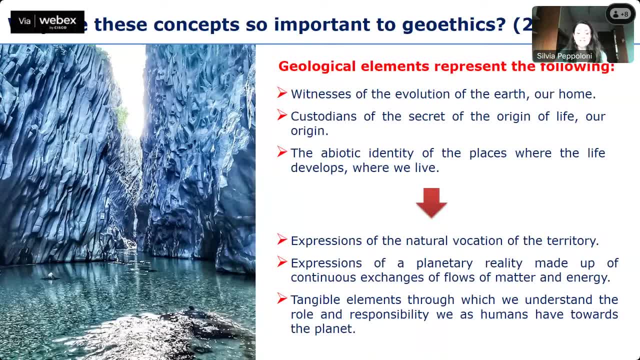 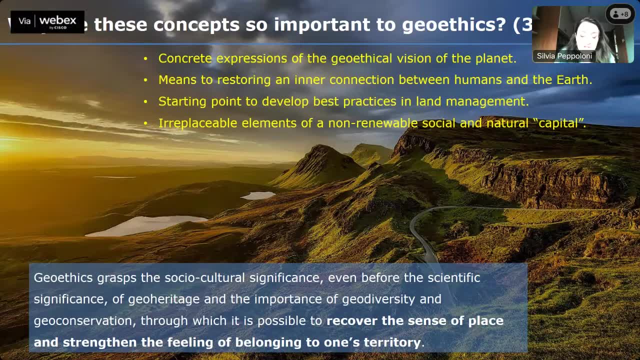 Basically biodiversity, the heritage, Basically biodiversity, the heritage And geoscience, And geoscience And geoconservation are concrete expressions Of a geological vision of the planet, Recognizing the very importance As a means to restoring an inner connection between humans and the earth. 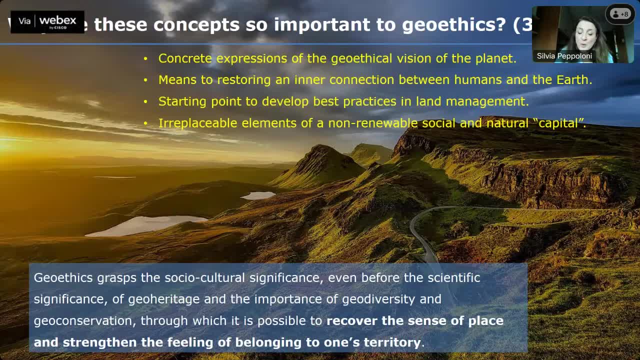 Is a fundamental starting point to develop best practices in land management. Geoethics grasps the social, cultural significance Even before the scientific significance Of joy, And the importance of diversity and geoconservation, So which it is possible to recover the sense of place. 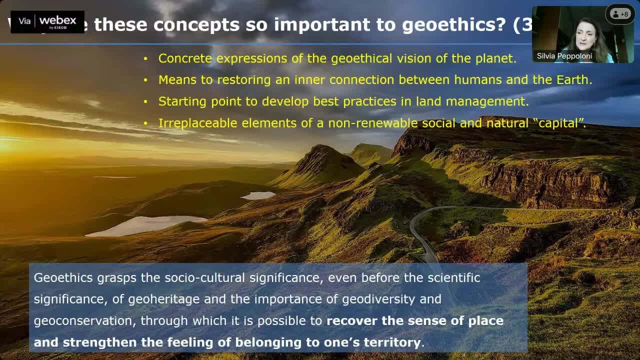 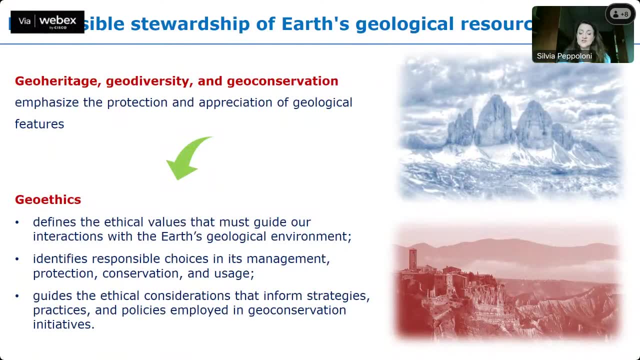 As 10, then the feeling of belonging to once the. So the connection between those concepts and your ethics lies in their share goal of promoting the responsible. So the connection between those concepts and your ethics lies in their share goal of promoting their responsible. 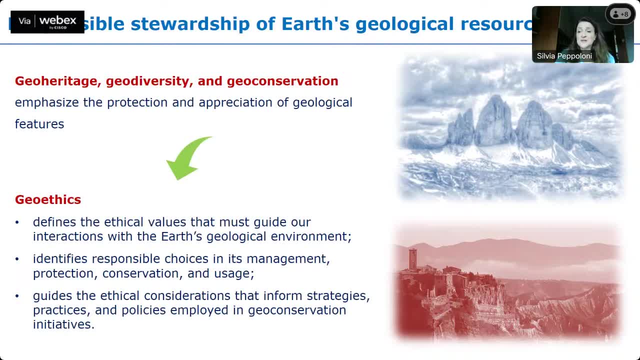 stewardship of Earth's geological landscapes and resources. While geoheritage, geodiversity and geoconservation emphasize the protection and appreciation of geological features, geoethics emphasizes the ethical values that must guide our interaction with the Earth's geological environment. 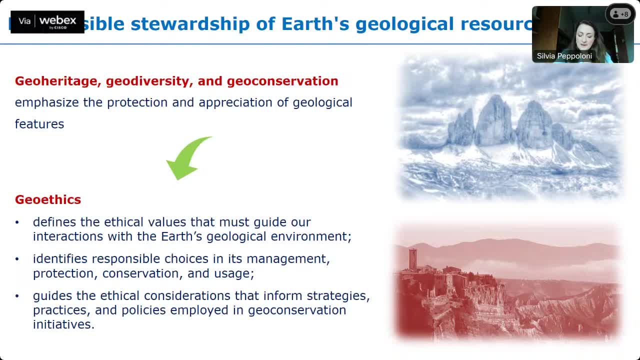 The interplay between them and geoethics involves making ethical choices: responsible choices related to management, protection, conservation and usage of geoheritage. prudent actions for using geological resources for the benefit of present and future generations. Geoethics guides the ethical considerations. 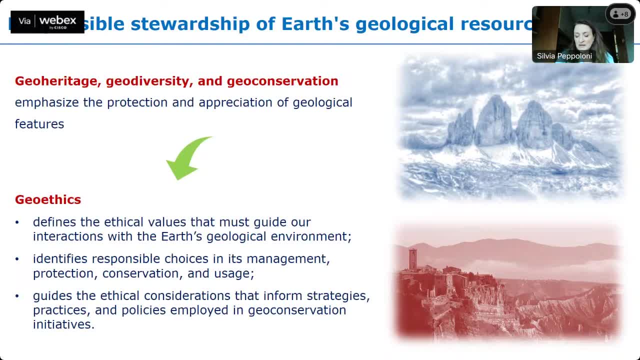 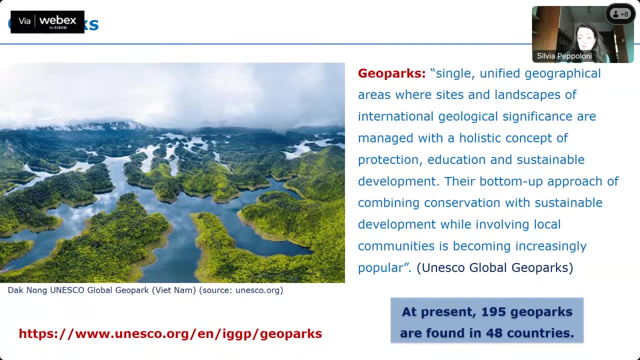 It informs strategies, practices and policies employed in geoconservation initiatives minimizing negative anthropic impacts. And finally, I would like to focus on other two elements already mentioned by Professor Tancar before me, two elements that are the tangible, concrete tools through which geoethics 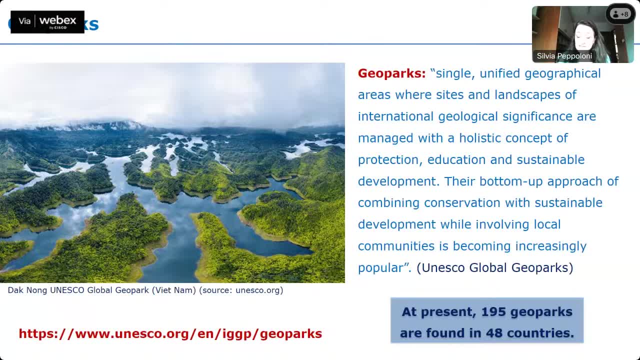 promotes the protection of geoheritage and enhancement and conservation of geodiversity. I'm referring to geoparks and geotourism. Geoparks are protected areas that showcase and conserve significant geological heritage. They aim to protect, conserve and promote geological features, landscapes and processes. 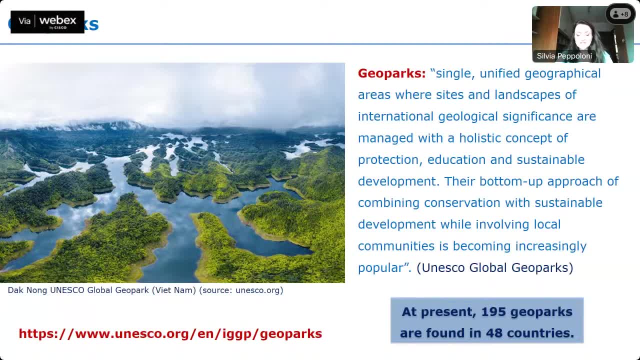 while also fostering local heritage, Thank you, And I hope that we can both reflect on the environmental importance of geoparks in our communities and we might be able to leverage them now, when we should continue to yesterday's discussion. So let me now turn it over to Rosy andNDray, who are going to be our speakers today. 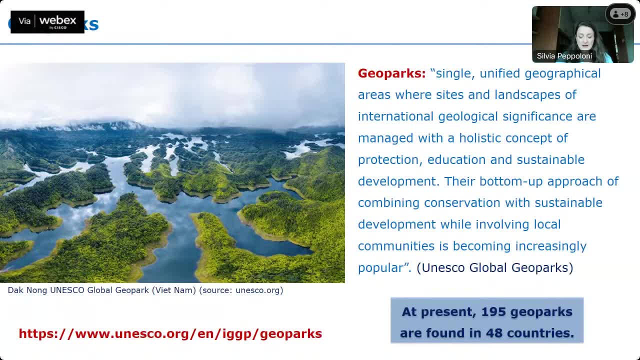 ROSY GIANNARO. Alright, I'd like to acknowledge our panelists for the program today. We've had a lot of questions about geoscience, geoscience, geoscience, geoscience. So we have one of unique guests and he'll start us off by sharing his reflections on 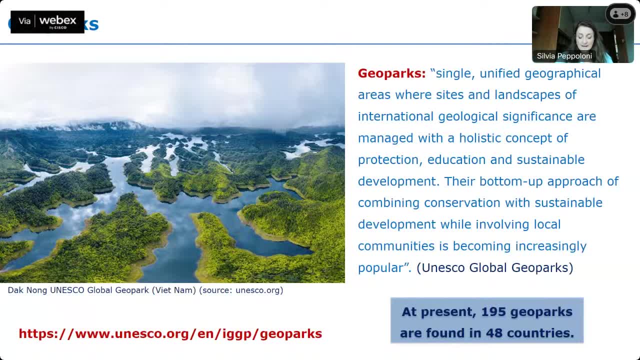 how geoscience plays a very important role in the development of geopolitical stakeholders, the development of global climate change And, of course, one of the most important ones is the development of global geoscience Interpretive center, trains, guided tours and educational programs that provide visitors with insights. 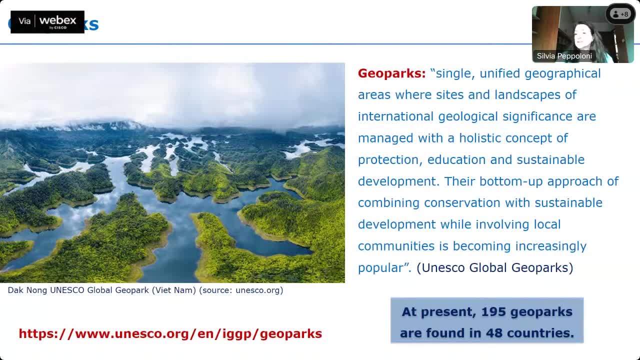 Into the earth: history, past climates, tectonic activity and more As consequence of the moment. As consequence, visit in the parks Allow rising public awareness about the importance to understand the geological processes And to protect and conserve geological diversity. 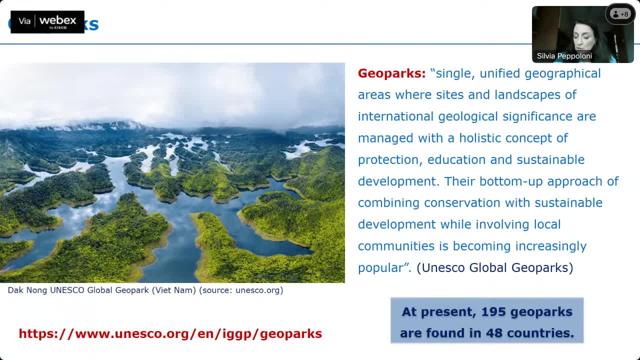 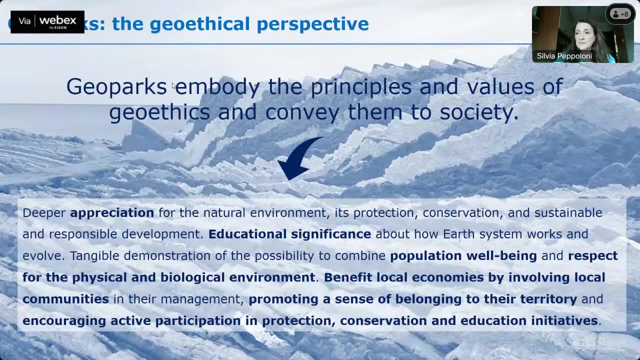 They are typically managed by local authorities and organizations in collaboration with the local communities, to balance protection, conservation, education and economic activities In a geological perspective, Embodied the principles and values of, and convey them to society, Values such as a deeper appreciation for the natural environment, is protection, conservation, and sustainable and responsible development. 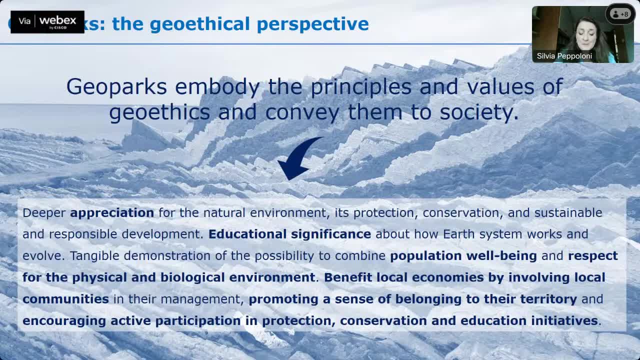 Educational significance about how our system works and evolve, The tangible demonstration of the possibility to combine Population well being and respect for the physical and biological environment. Furthermore, Joe parks benefit local economies By involving local communities in their management, Promoting a sense of belonging to the territory and encouraging active participation in protection, conservation and education. 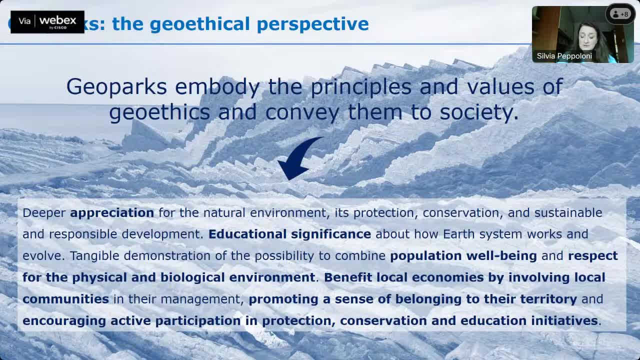 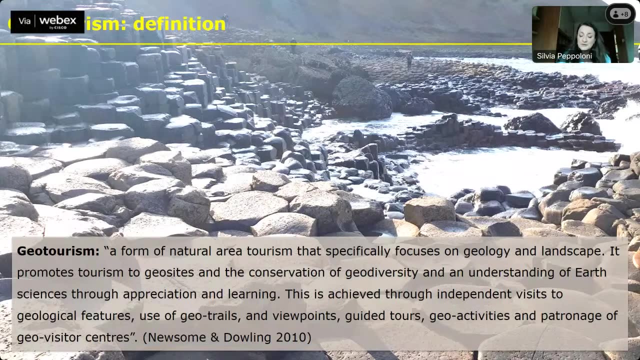 And encouraging active participation in protection, conservation and education. All these benefits Are also true for geotourism. It's a form of sustainable tourism that offers To visitors the experience of the geological heritage, The enjoyment of geological landscapes, the knowledge about trucks, minerals and the geological history of a specific region. 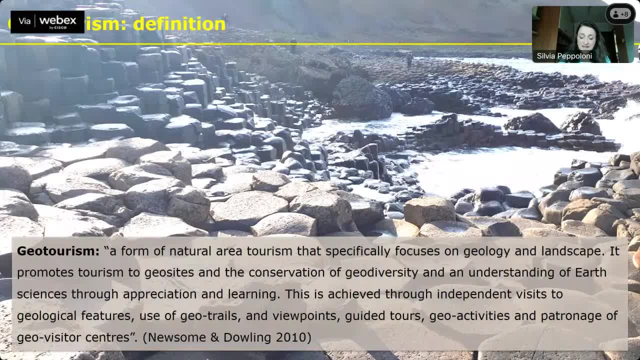 And by encouraging responsible visitation and rising awareness, geotourism Helps safeguard these valuable resources for future generation. The definition of in these slides is provided by new song and doling in 2010.. The form of natural areas that specifically focuses on geology and landscape. 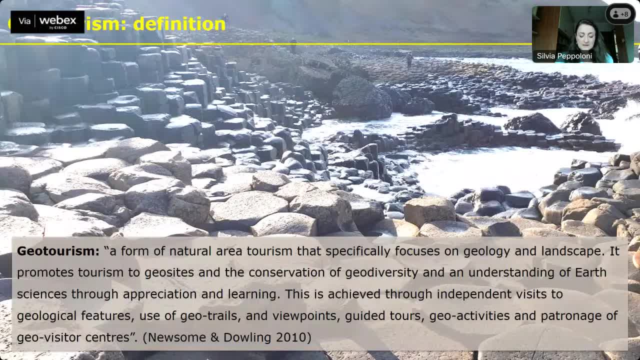 It promotes geotourism to Joe sites and the conservation of Joe diversity And an understanding of earth sciences through appreciation and learning. This is achieved through independent visits to geological Feature, use of geo trades and viewpoints, Guided tours, Joe activities and patronage. 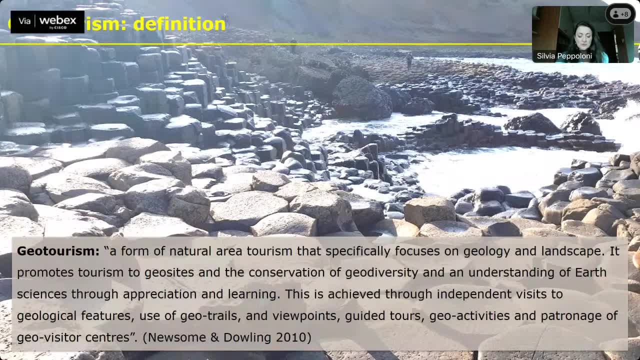 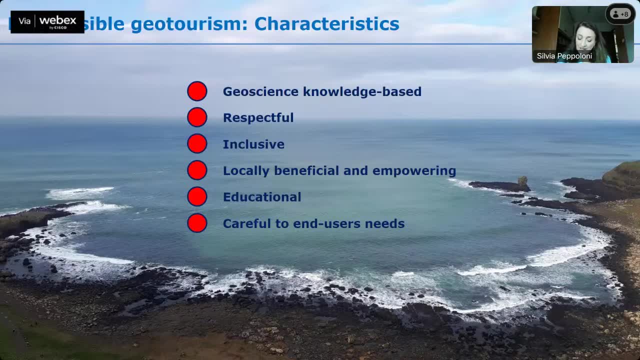 Of Joe visitor centers. So Joe tourism as a, And then undeniable, educational, cultural and economic potential. But to unfold, it's a full potential. Joe tourism must be practicing, respecting certain requirements, The same that that are already applied, in the enjoyment of your parts. 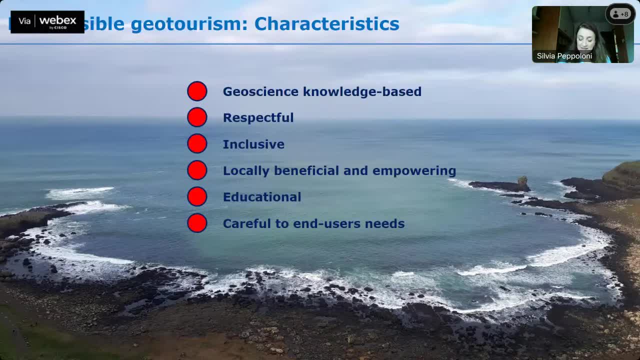 Requirements that must be implemented even And when the jail tour is. the destinations are not included. We've been protected natural areas. to the same, in Joe ethics, We refers To the concept of responsible Joe tourism. Responsible Joe tourism is Joe science, knowledge based, respectful, inclusive, locally beneficial and empowering educational. 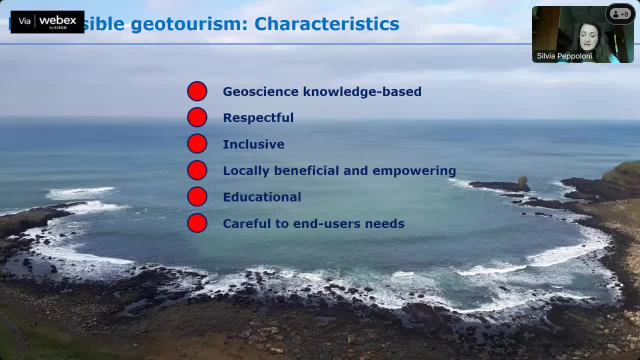 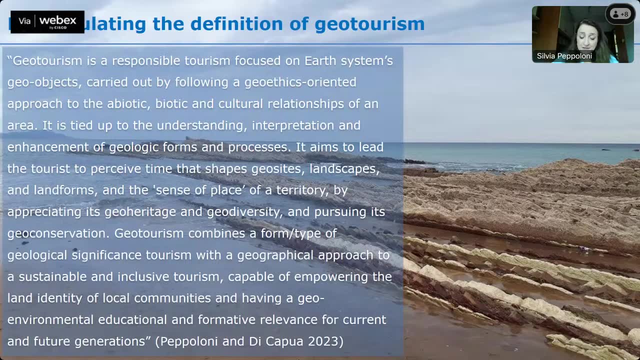 Careful to end the user's needs. So I think that encourages a responsible approach to Joe tourism and suggests That the definition of Joe tourism should be adjusted To incorporate the joint principle of Joe of responsibility. And so this is the the, the definition, the last definition we have proposed. 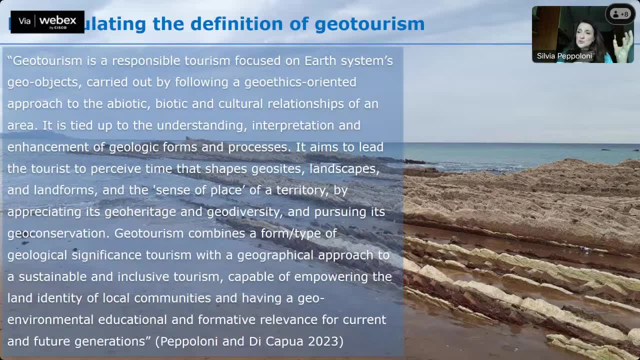 Uh to to, Uh to to Connect to Joe. tourism to Joe to Joe, ethics. Joe touring is a responsible tourism focused on earth systems, Jail objects, carried out by following a joy ethics oriented approach to the a, B, a, biotic and cultural relationships of an area. 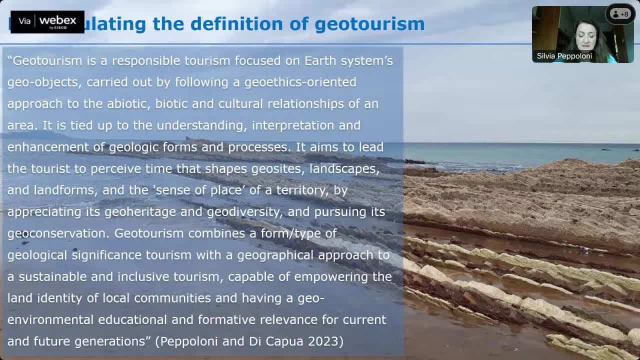 It is tied up to the understanding, interpretation and enhancement of Of geological forms and processes. It aims to lead the tourists to perceive Time that shapes Joe sites, landscapes and landforms And the sense of place of the territory, By appreciating its heritage and Joe diversity. 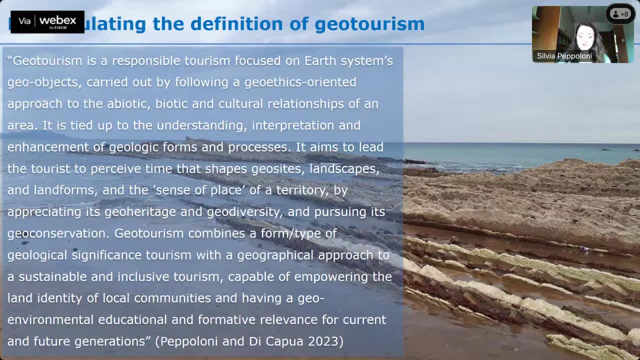 And pursuing its Joe conservation. Joe tourism combines a form, type of geological significance Tourism with the geographical approach To a sustainable and inclusive tourism Capable of empowering the land identity of local communities And having the Joe environmental, educational and formative relevance for current and future generations. 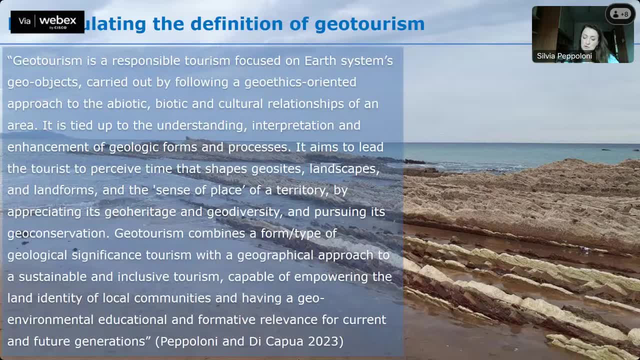 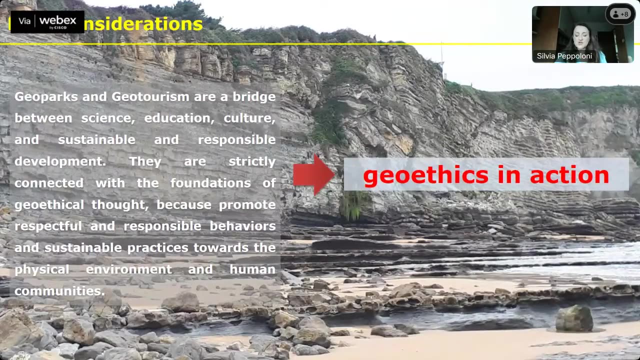 It is important to highlight that responsible Joe tourism cannot be separated from adequate geological And geological training of Joe tourist operators. So the park and Joe tourism are a bridge Between science, education, culture And sustainable and responsible development. They are strictly connected with the foundation of Joe ethical thought. 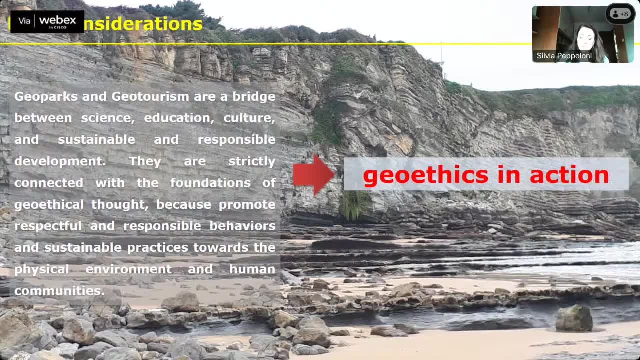 Because promote respectful and responsible behaviors And sustainable practices towards the Physical environment and human communities. In simple words, they exemplify Joe ethics in action. so I I finished, I conclude, And I again I thank you for the attention and I thank you also and congratulate with the India. 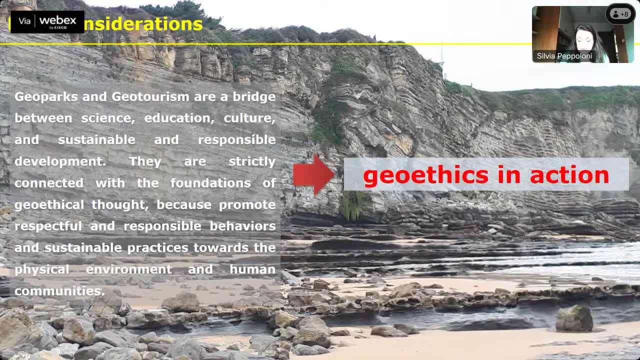 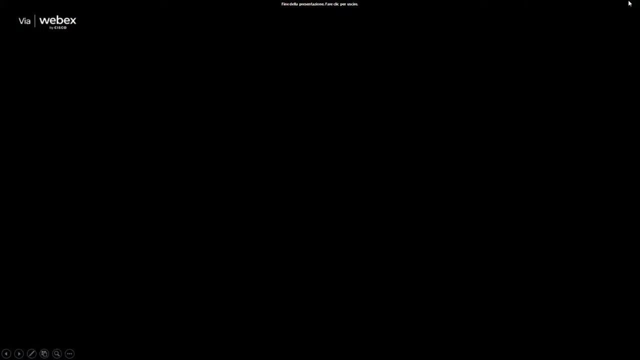 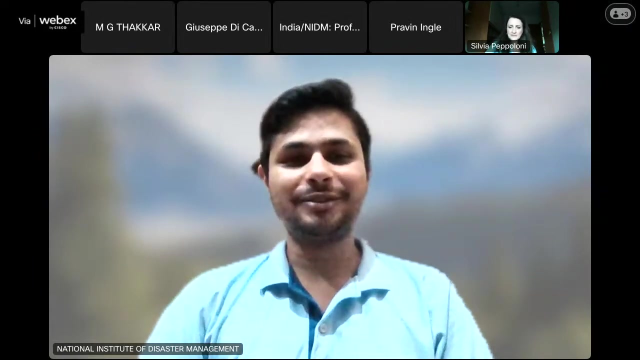 For the great job done to develop Great example, A great service for all the Joe science community. Thank you all. Thank you very much, ma'am, and I thanks again you for joining us and providing us with the insights of your ethics on your tourism. Once again, thank you very much, ma'am. 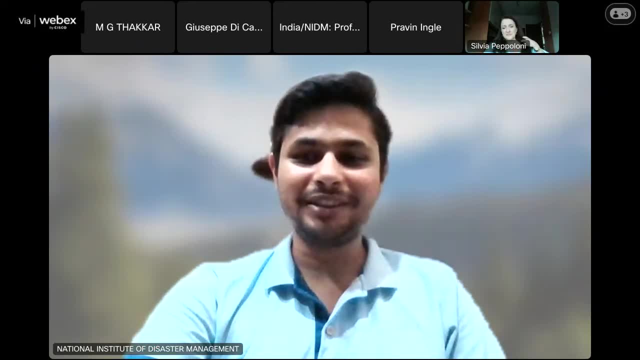 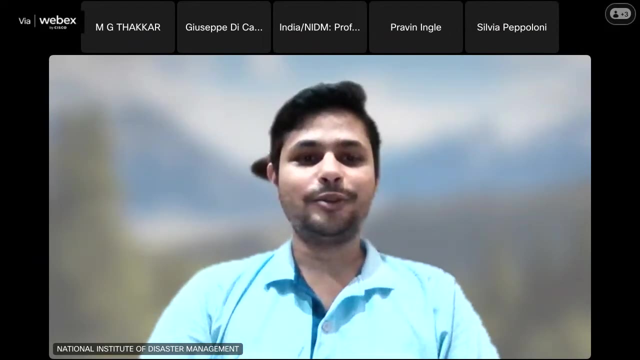 This time I cannot see any question, so if we will have, we will share it with you. So thank you. So, moving to our next speaker, Dr Kusha. he has more than 15 years of rich experience In institutional leadership, capacity building, teaching. 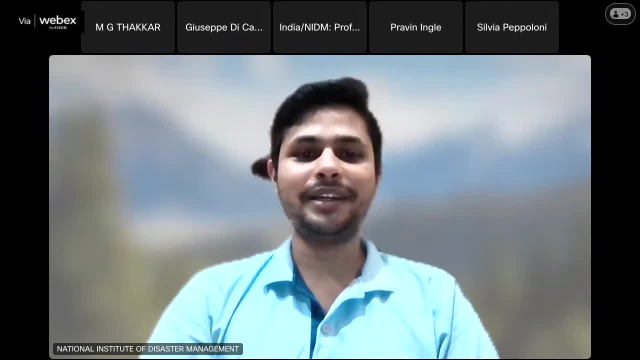 Research and publication in multi disciplinary area of environmental and sustainability. his expertise lies in sustainability Education and across disciplinary understanding of environment. He had obtained his PhD in interdisciplinary aspect Of environment from prestigious Jawaharlal Nehru University and for the same was awarded distinct. 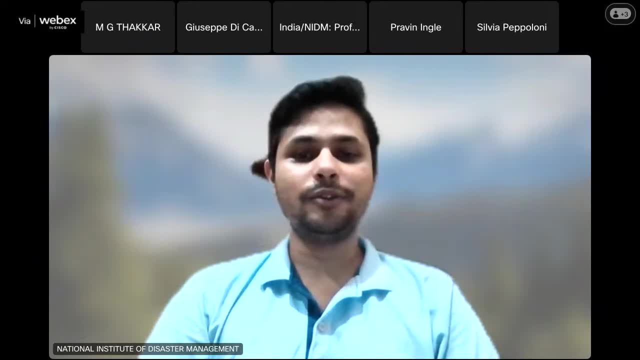 like academic excellence medal, the president of India gold medal, He is an institutional builder and also he has been established. also he has established the prestigious LEED lab for capacity building program in green building with GBCI and USGBC at MIT University, Haryana. 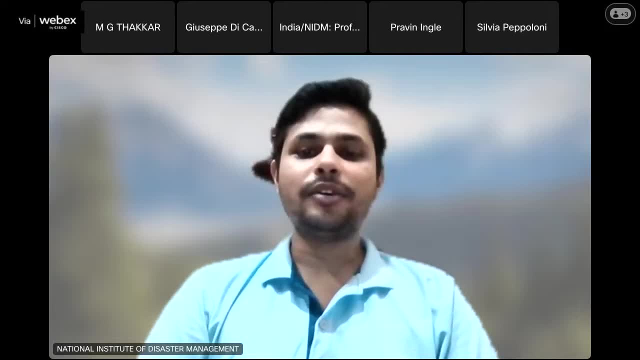 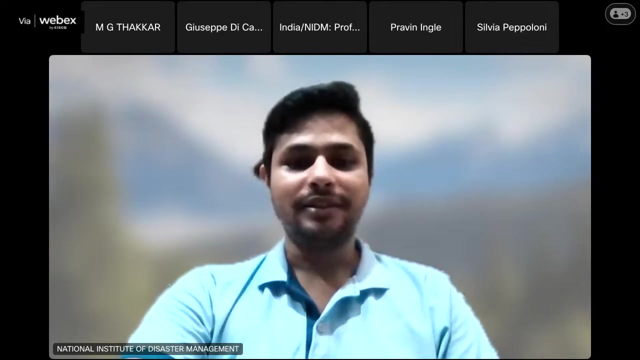 He is actively engaged with research work and also guiding the students for their PhD thesis. He has undergone several FDPs capacity building program summer courses and delivered popular lecture on earth and environment science, including INSPIRE program for science popularization. With this I would like to hand over the stage to Dr Rajendra. over to you, sir. 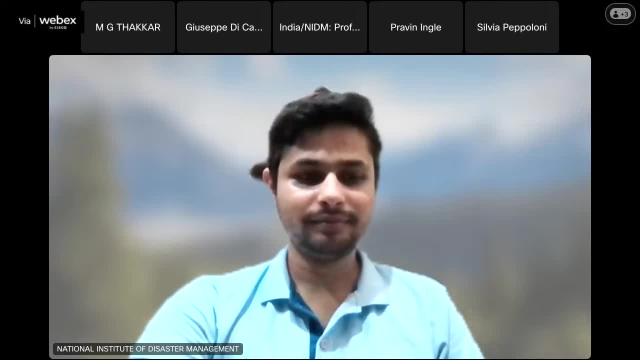 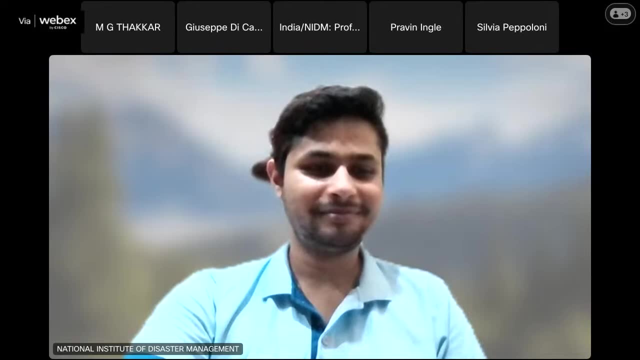 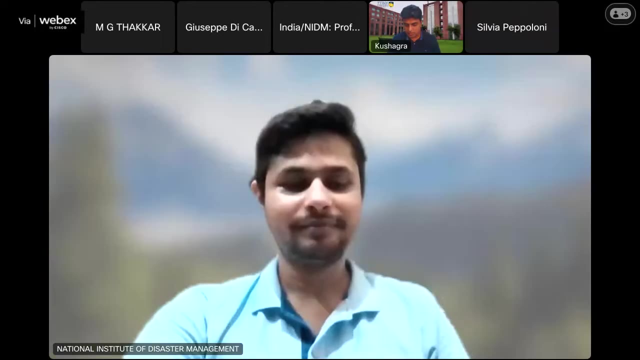 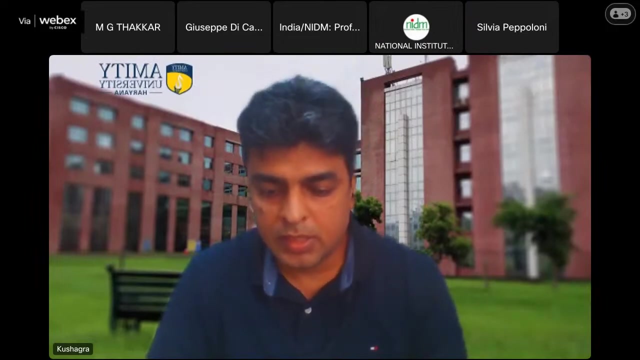 Sorry, sir, you are muted. Am I audible? Yes, sir, you are audible now. Thank you very much for generous introduction and respected dais, particularly professor Prakash and professor Thakkar, who is like teacher for me, and along with that our old professor Dr Rajendra Dehriji and Professor Dr Ratshaya Khan. 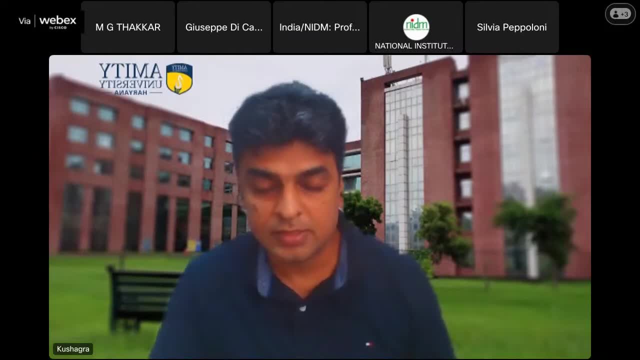 So you are welcome to speak to us, ARIYANA. Thank you very much. Thank you very much, sir. Yes, sir, you are muted. Yes, sir, you are audible now, partner in this evolution of the concept of geoethics, from Italy, Dr Capua and Dr Silvia. 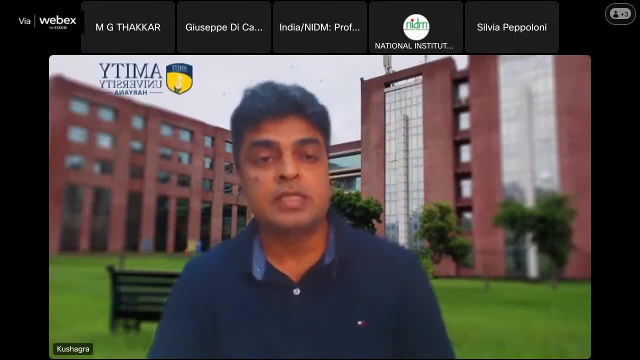 So today we are celebrating day four- geoethics- And in this context, since our previous speaker has already given a framework- particularly Silvia, who is very much into the theoretical construct of the geoethics- what to do, what not to do- 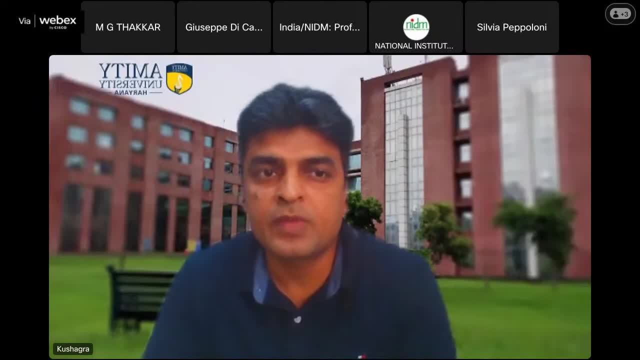 along with Professor Thakkar, who very briefly introduced about not only his own understanding but also the government initiative to streamline, or you can say the mainstreaming, the concept of the geoethics through- I mean in totality- through different actions and program. 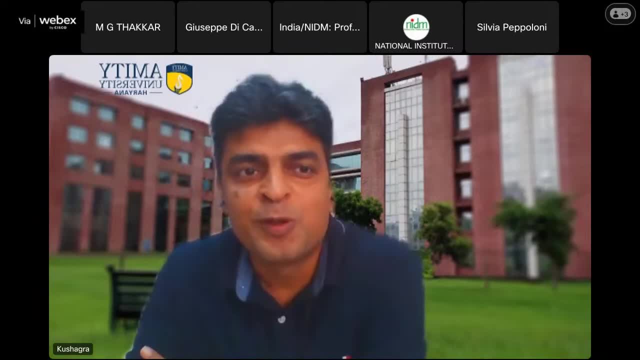 So my role become very difficult to bring out perspective on the geoethics. So I choose to discuss on the ethical consideration. What does it mean, Ethics means and how? geology and geoethics, or you can say in the larger context, environmental ethics, and why there is a need of such kind of discussions. 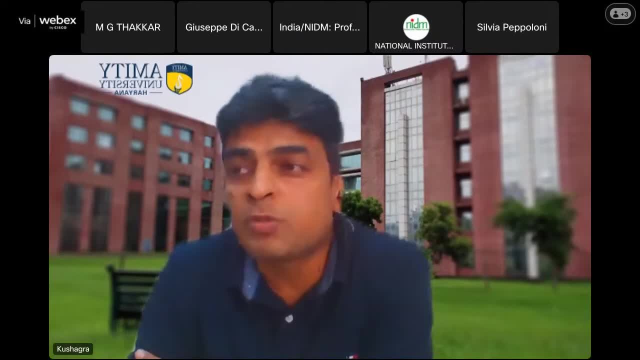 And the observance of the scientific implementation in the field through some of the human actions, and I will also try to put some cases studies very brief, to mainstream this concept, Which, which is, which is, which is a need of time I can see. 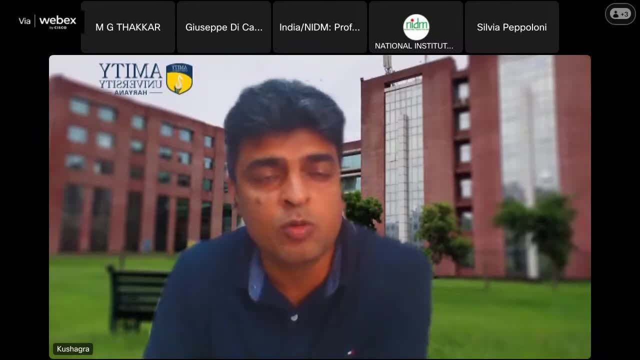 So I want to start with one of the very famous quote, and so we, we all know the Mount Everest- And when Mount Everest name came, then Edmund Hillary and then, in Norway, named Nargen came- comes in our mind. But before that, there was one very energetic mountaineers who passed away, unfortunately unable to conquer the Everest. 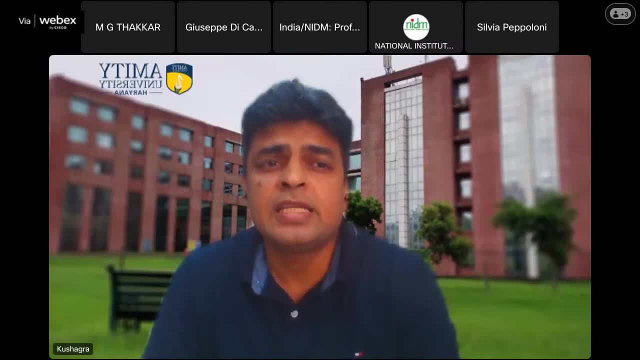 He tried. he goes for many expeditions but failed. and his last expedition he was found fugitive and his dead body was recovered only after many decades. So very famous people used to ask why you want to conquer Everest. So it is. it is a very simple question but very difficult for mountaineer to explain. So he told 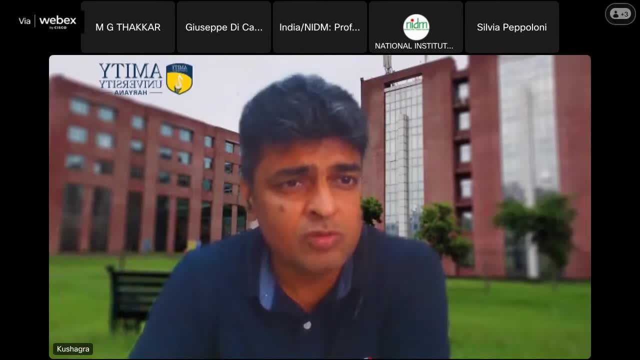 Once he told, and it is very famous now, that I want to conquer Everest because Everest is there. So this is the construct today I want to make For the geo heritage or geo ethical consideration. Whatever you see, we enjoy the life, interact with the nature. 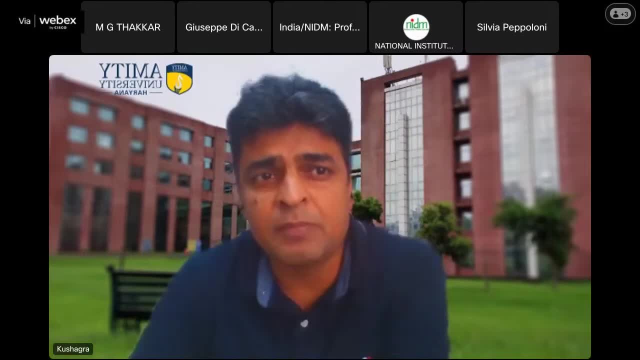 It is only because it is there. Or I can say, while my sustainability class I used to emphasize this concept- that we are using resources. Suppose you are using the timber. It is because timber is there. Our forefather has not exploited it completely. 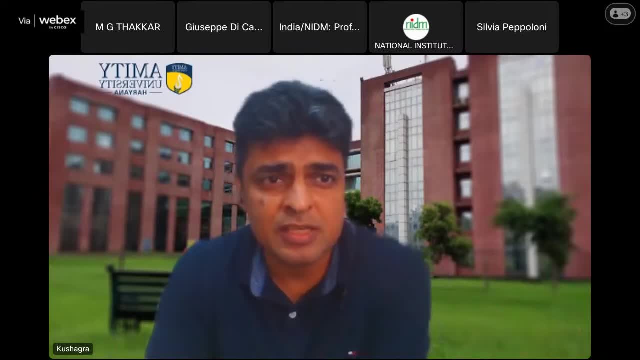 So this is the question that is very prominent nowadays, and here we can bring out the consideration of Geo ethics in that particular sense. so Ethics, morality and mutual association Is basically make us different from the animal. Otherwise human being is in the biophysical term, but nothing more than animal. We are animal. 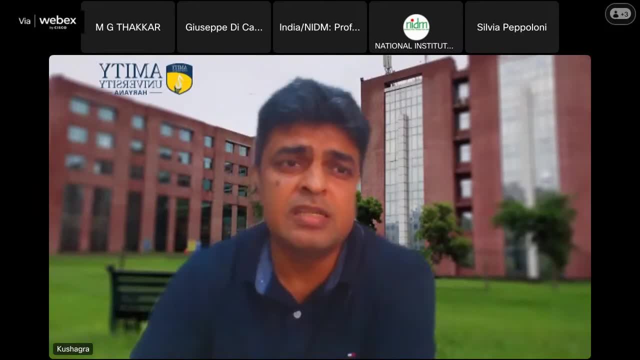 Only difference is that we are social animal, So certain I'm, the character are impinged upon me. That is completely social construct And that is the ethics. So ethical consideration is basically dependent upon The kind of interaction we enjoy, Association enjoy with certain things, with particular things. 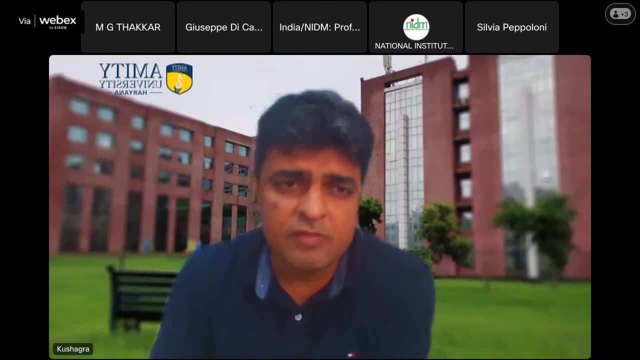 Like we live. so Indian, Indian, um, um Indian philosophy is very much into the nature. I mean we, not we not only care about our family, our- uh, our village or our community, But we also care for the viewership tree. 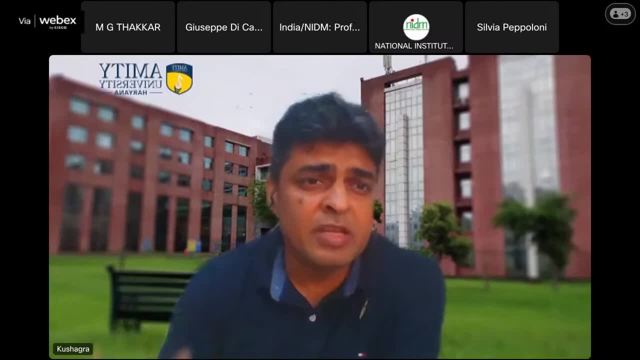 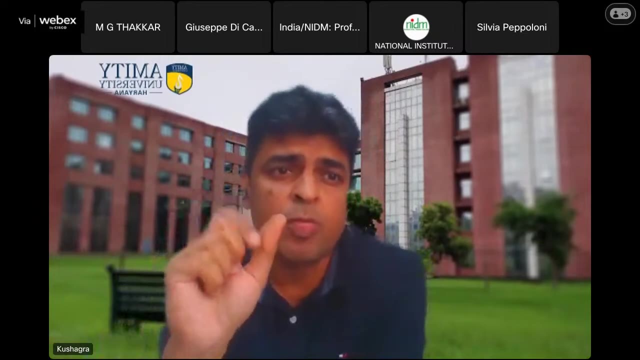 You are, see the forest, we are very much connected, very much associated and you course of time, It become in our value system. So, uh, 1 thing I also try to bring from the Sylvia presentation: that definition of you ethics. you mentioned a term value. 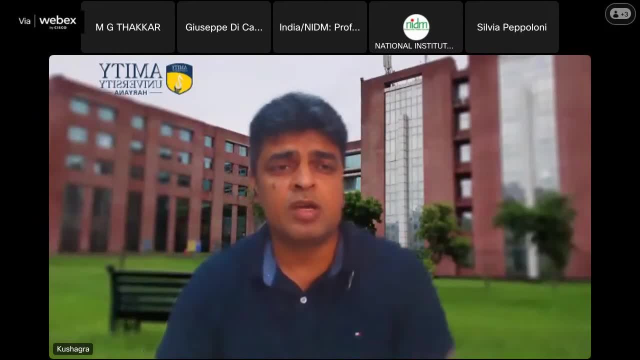 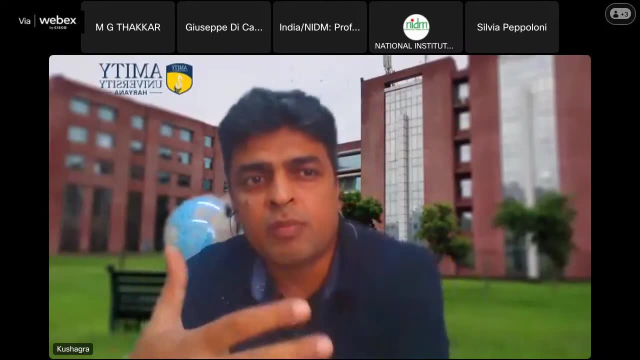 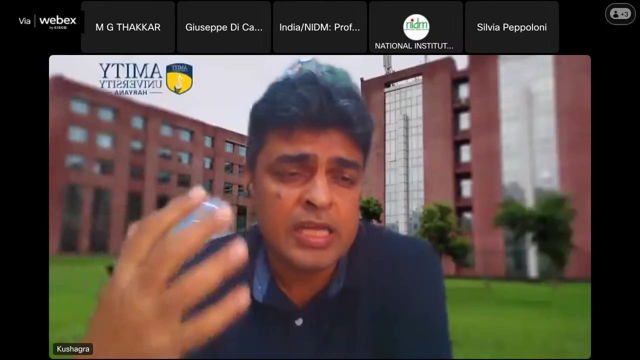 So this value system is very important to uh to uh formulate the concept of ethics. So so we have the the level of our association or layer of level of our contact or interaction with any particular thing. It is basically foundation of uh uh ethical. 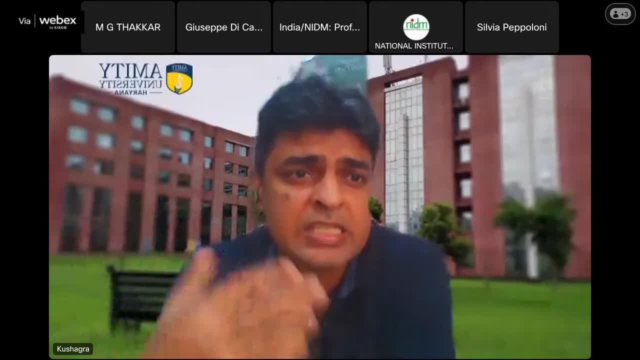 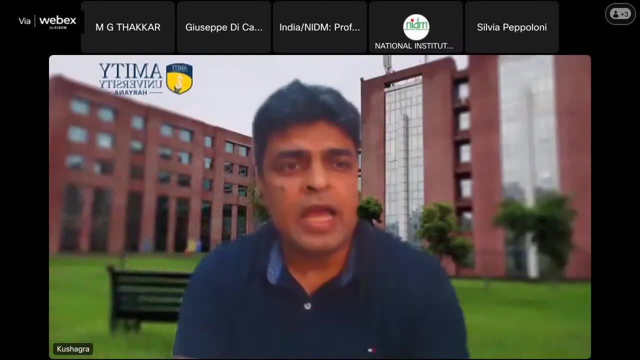 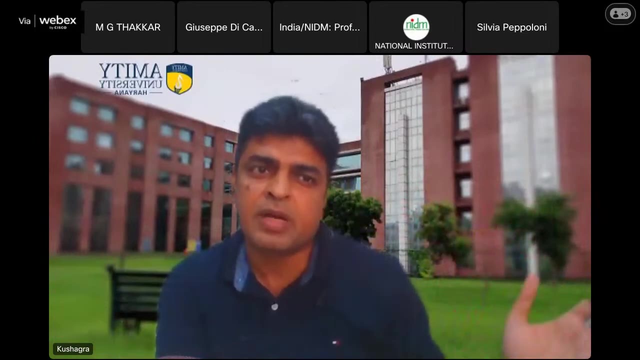 Consideration that uh put forward and it decide the action, or with that particular uh uh thing I can say So, uh and that. so the our association in present- and that is basically uh, directed or streamlined by the our association with that particular thing in the past. 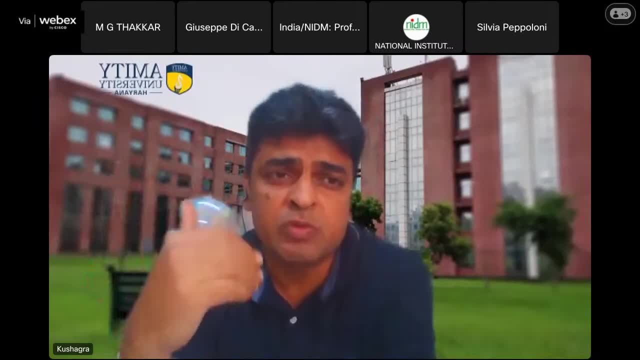 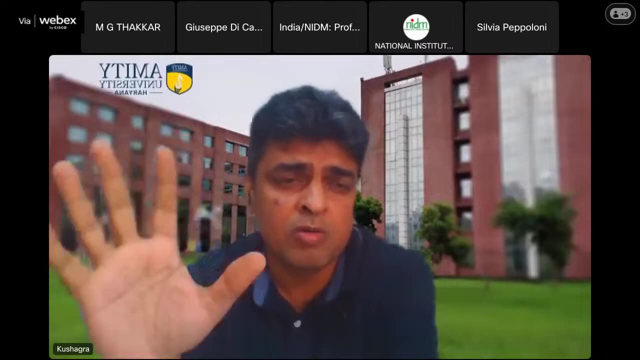 Basically going to give you what kind of association we will have in the future. So the past, in our interaction with the past, Is very important, whether it is with the Plant, whether it is with the nature, with the soil, with the rock, with the mountain. So it is very important that how we see our past 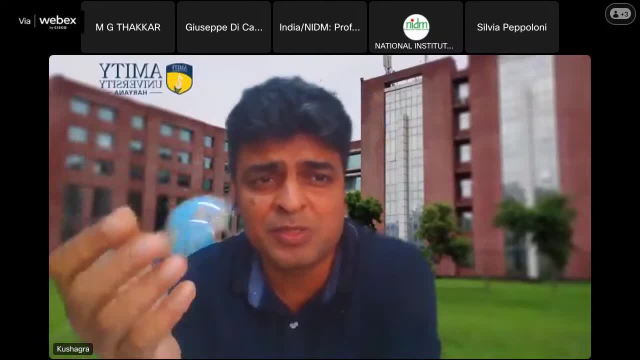 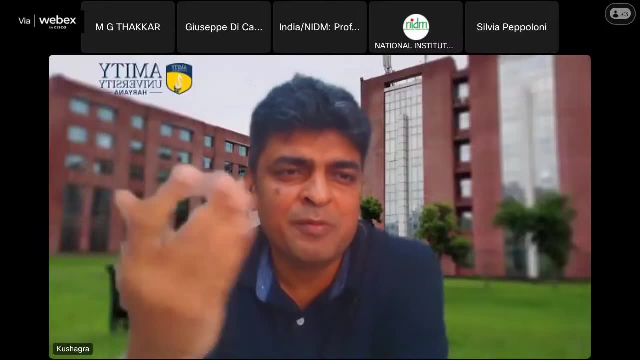 So 1 of the very important thing I want to mention over here: when you go for the class, uh, particularly when you teach the rock and minerals, So we come, we say very, I mean, although it is a very social code, if you want to. 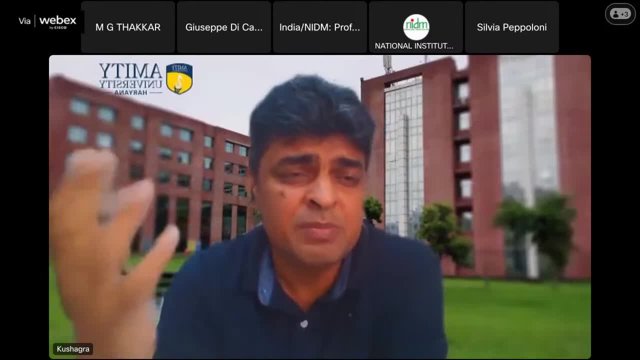 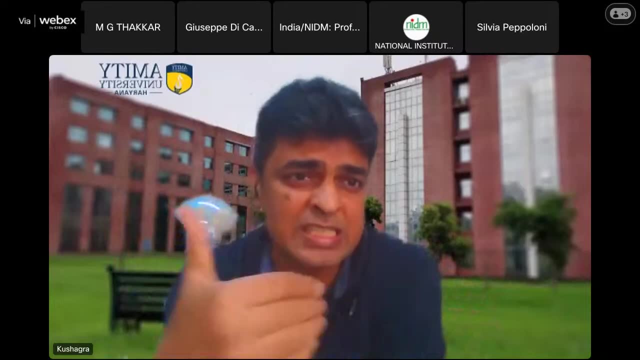 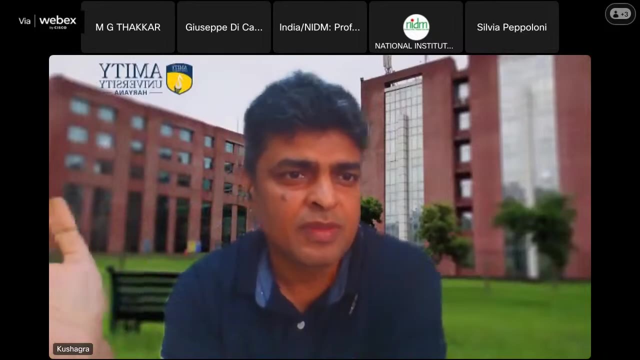 If you want to experience Past, touch a rock. it means the rock is nothing, but it is the. it will. going to give you a story from its Genesis to what it is today. The, the, the kind of changes it, uh, it face due course of geological time history. 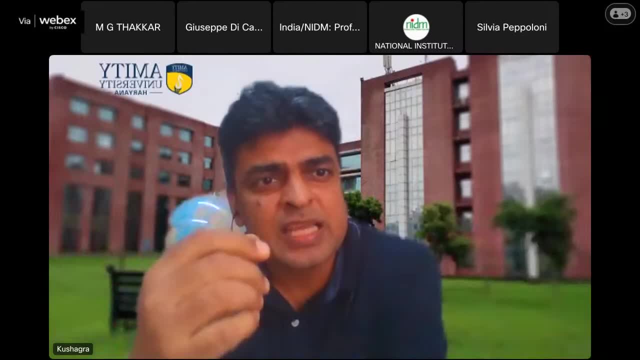 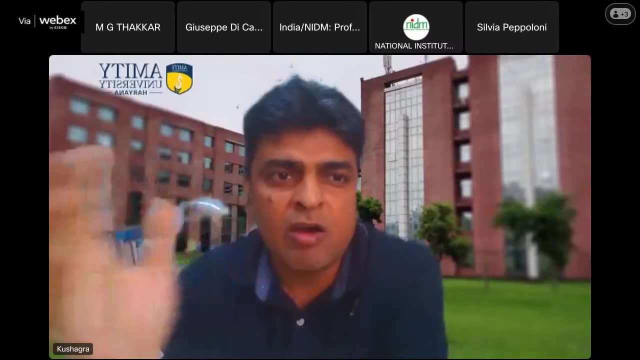 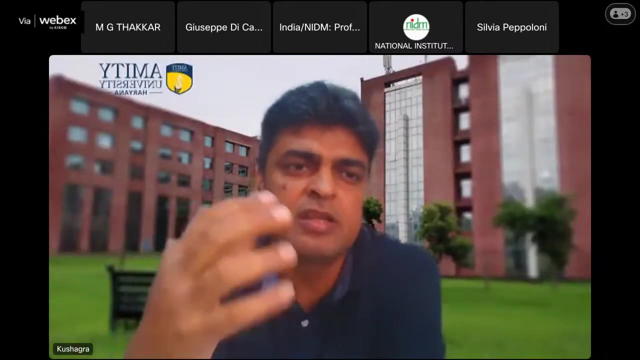 So. so in that sense, past can be visualized at 4 different layers. The 1st 3 layers is basically, Is our association with the living organism. 1st, 3 association and the last, 3rd, 4th level of association. 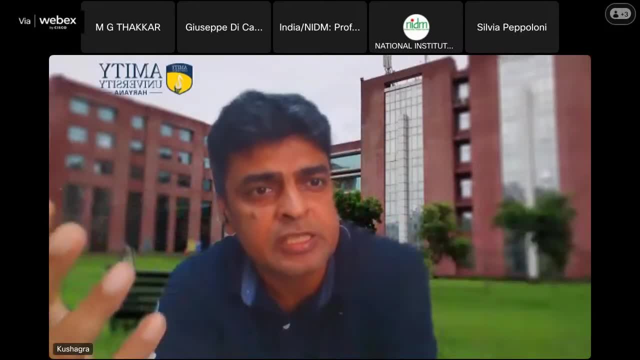 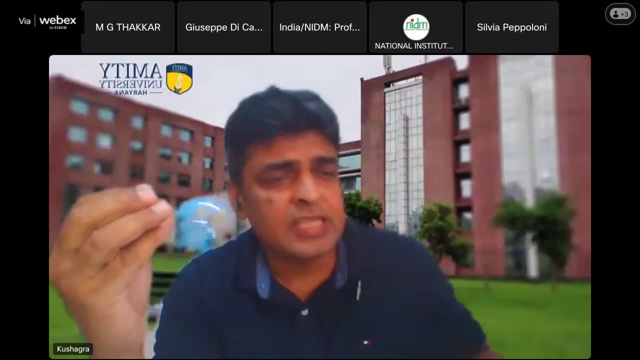 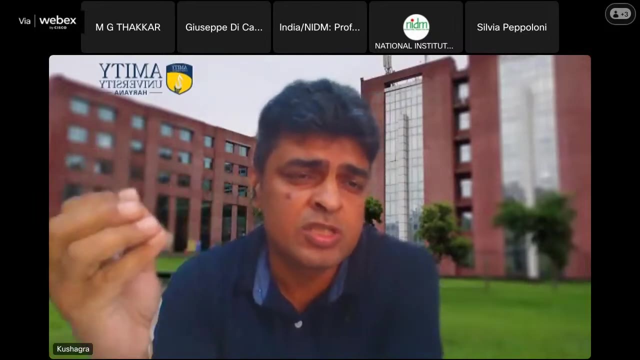 Will be our association with the non living aspect of the nature. So what are those for? the 1st 1 is the Historical. so anything we see It has some historical connotation, like if see, we see the red 4, or we see the some, uh, and so that is the historical. 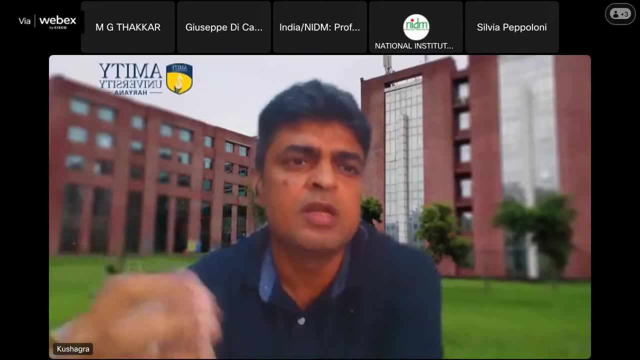 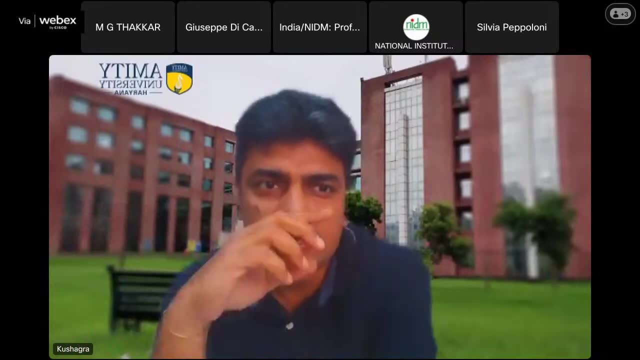 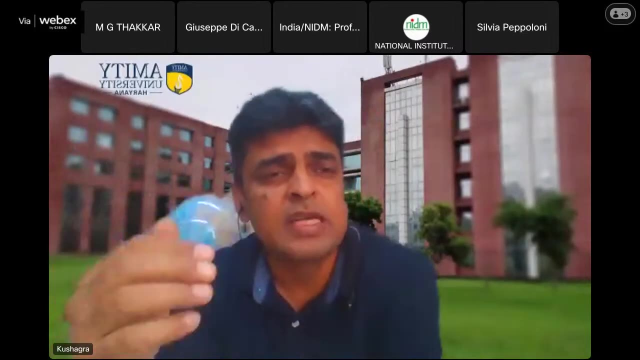 So we have a very different sense of belongings To that particular moment, because we feel that it is from our plan or it is from our race. It's human being. uh, for that result into that. we are so advanced in the past or we are not advanced in the past. that kind of 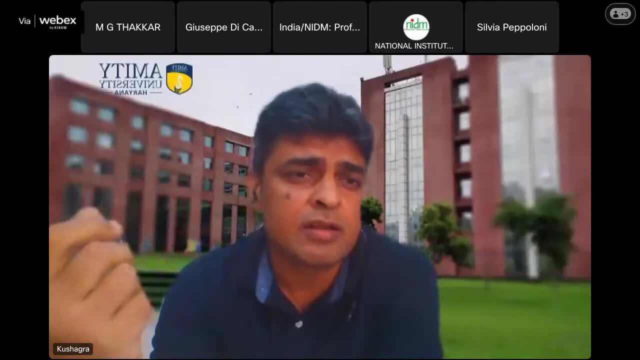 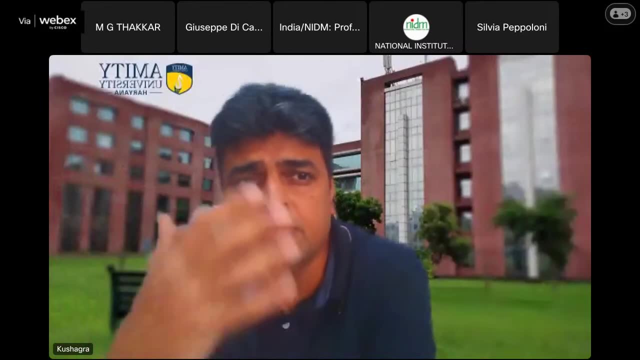 If you go further deep down than it become. So where we correlate ourselves with our evolution, the story of evolution, like we go to and we find The morale, the paintings, rock painting, That is 10,000.. 1st, 3.. 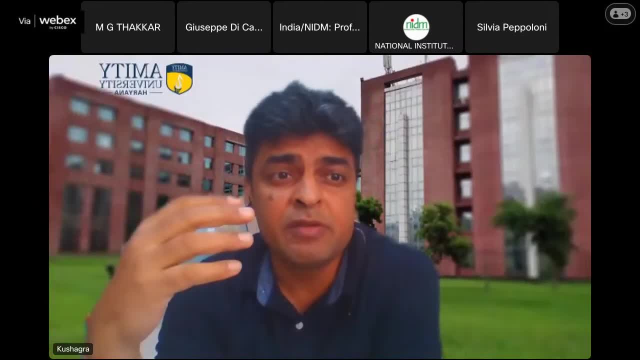 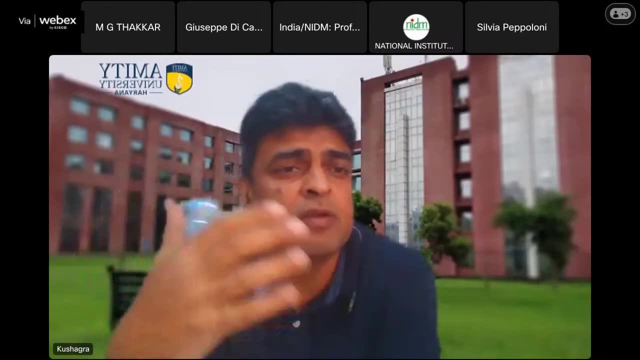 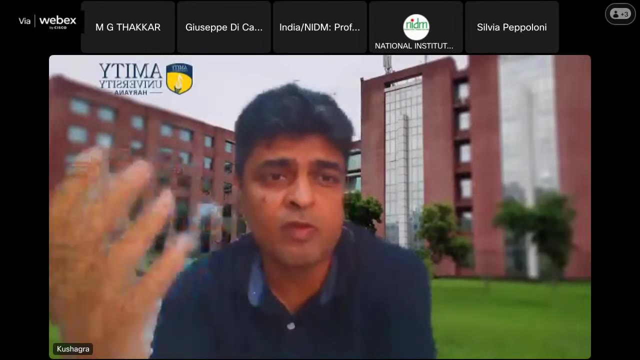 painting that is 10 000 to 30 000 year old. then we we feel that how our forefather is about to enjoy the life and what kind of consideration or constraints they used to feel so similarly, everyone we try to connect ourselves that we are from the same clan and the mother, lucy, is the 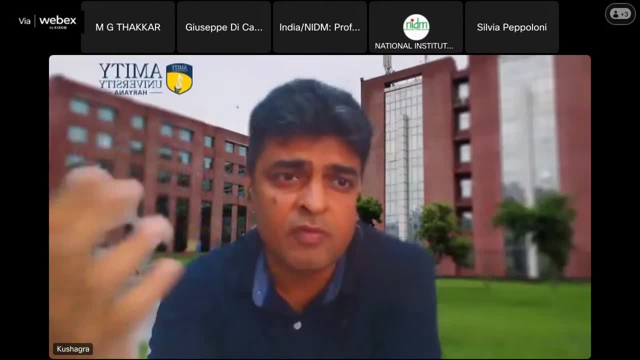 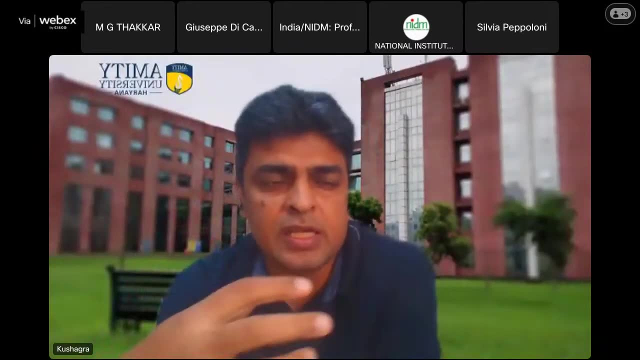 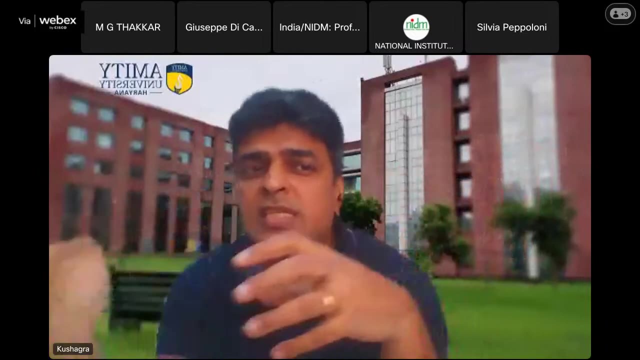 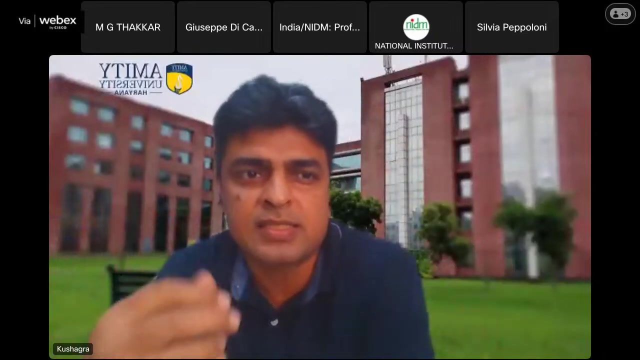 central point where you all get originated. we originated from africa and moved to the asia, some clan goes to the europe, kind of thing. so ecological material, we think. third association is basically- you can see now we are moving some distant- so now the living organism and that is called paleontological. so the third level to see the past is paleontological. 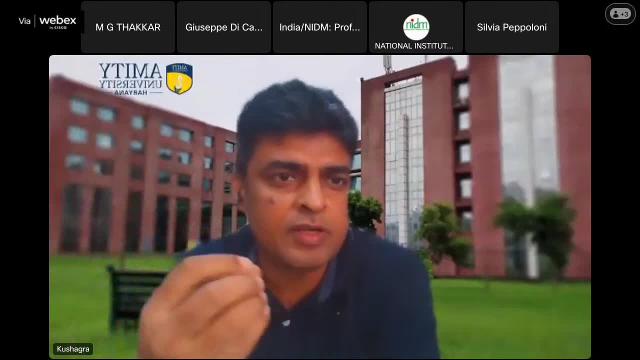 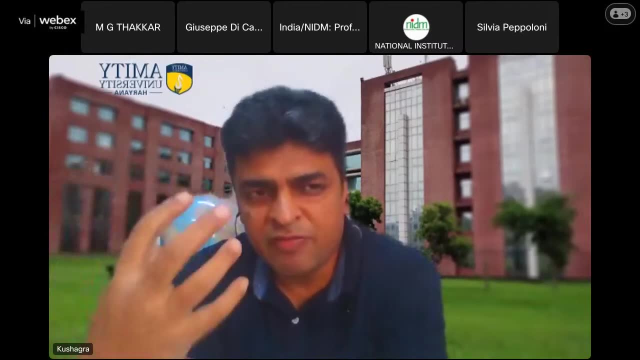 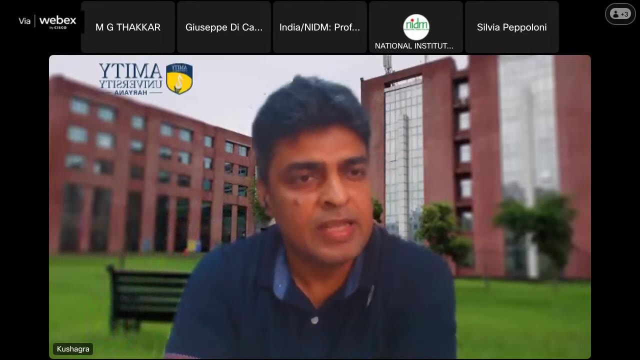 when you see the fossils of a dinosaur, or egg of a dinosaur, or a head of the primitive elephant from sybalik, so we have feeling that it is living organism also known on this land where we are dominating today. and the fourth last, but very much central for today discussion, and that is the 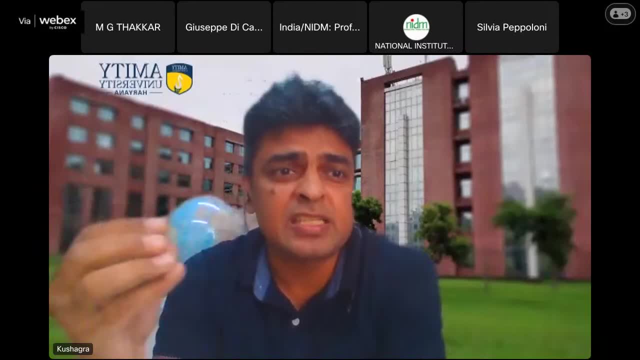 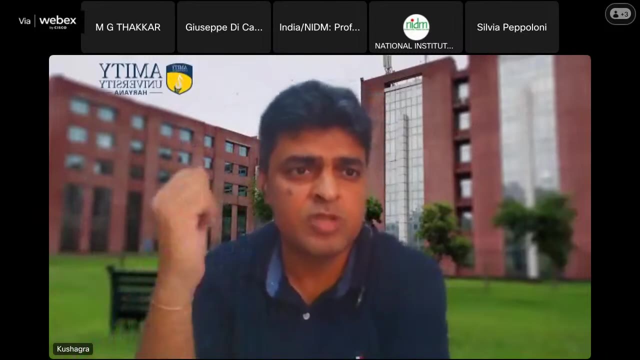 geological. geological means anything that is from the past, that is for the geological time scale. whether it is living or not living, it doesn't matter, but it carry how, how earth form and how it passes through different geological time scale and it come today. so our association with all there is four, five. 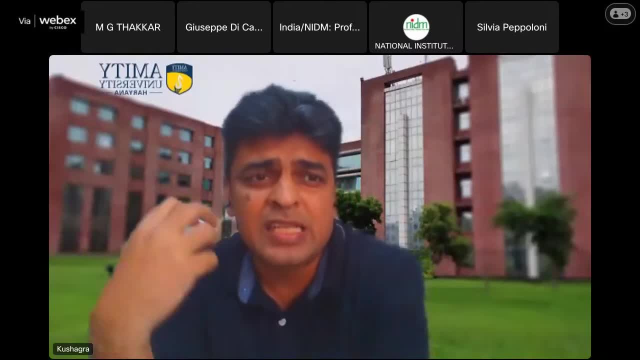 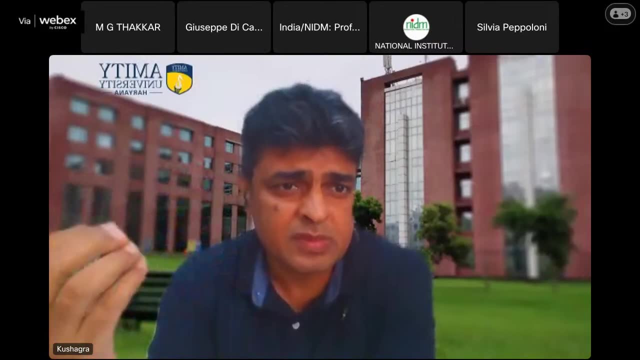 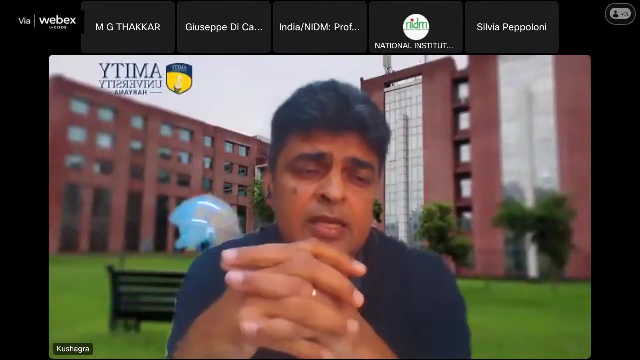 five layers, four layers of the past determine the kind of ethical consideration to that particular particular thing or particular material. so so there is two aspects. one is the live, while biological, one is non-biological. what is geological in the nature, even in biological, they are a different. 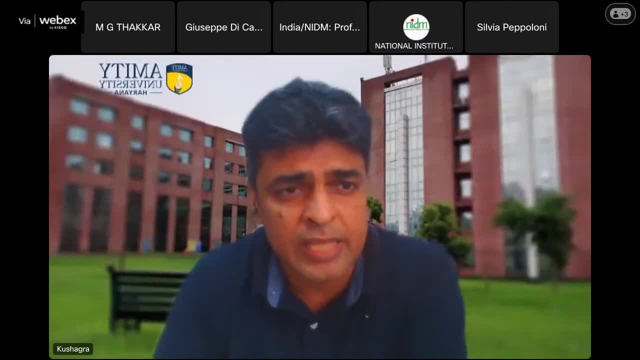 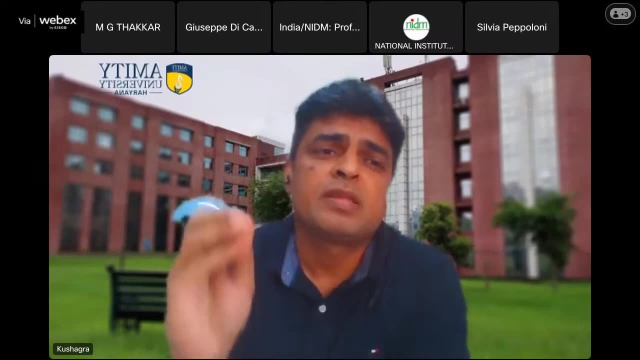 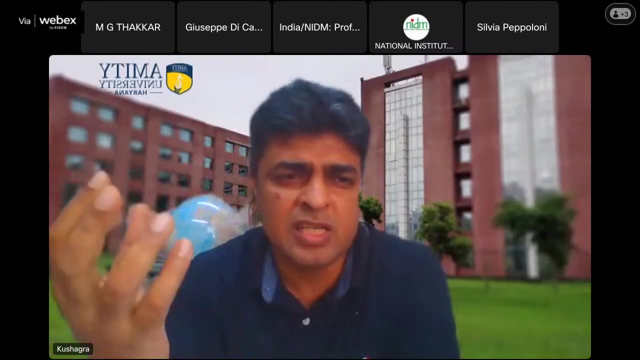 gradation of our ethical, ethical, a ethical consideration like, uh, typical biological ethics, uh, i am going to little bit, uh, emphasize over here. then we do lot of genetic experiment with the bacteria, so their, their ethical consideration, they won't come in my mind whether we have to do. 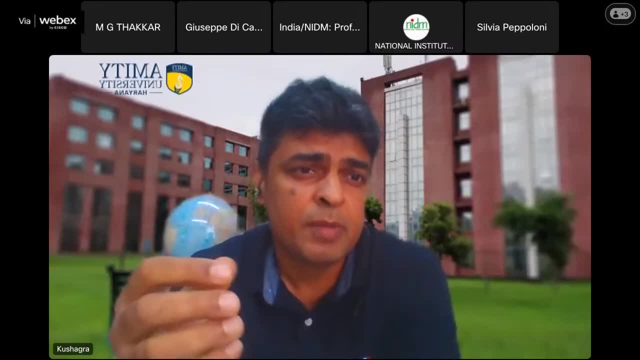 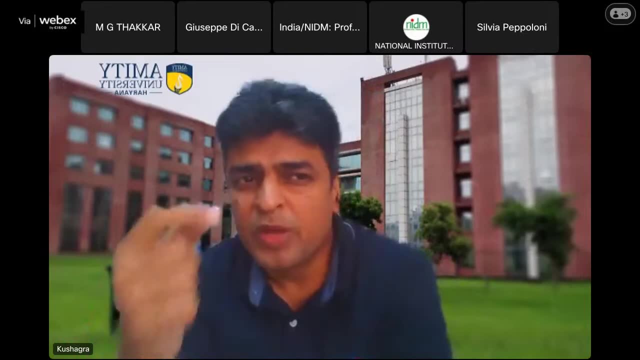 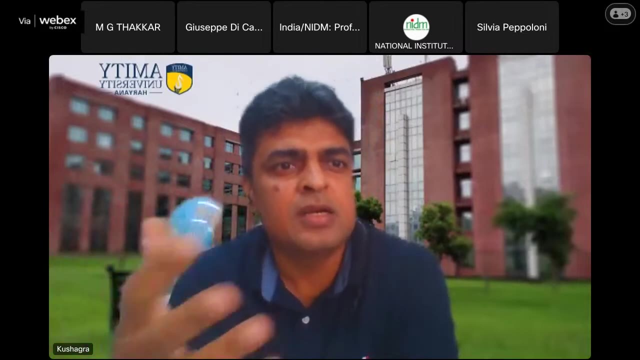 whether you have to change their genetic makeup or not. but when it comes to the human being or larger animal, then certainly ethical consideration has started coming, whether we have to change their genetic makeup or not. We have already, I mean, come up with the Dolly, I mean the hybrid. 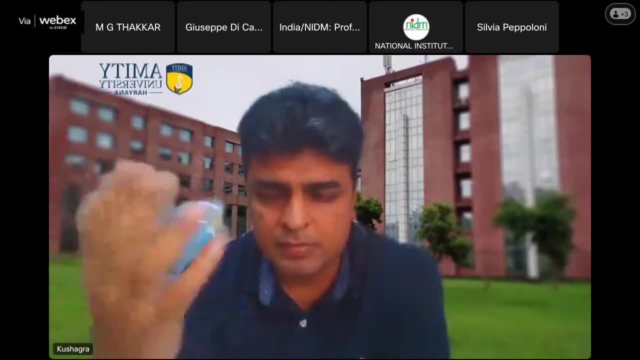 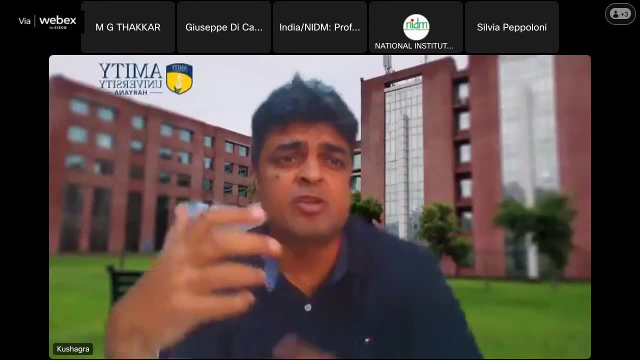 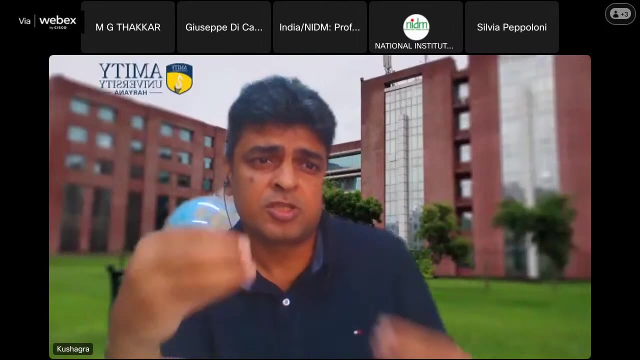 hybrid. I mean, I just forget the name particular, but we never think of to make clone of the human being because there is a lot of churning in our mind whether we should do such experiment with the human race or not. So the central point is that the kind of association with all the material, 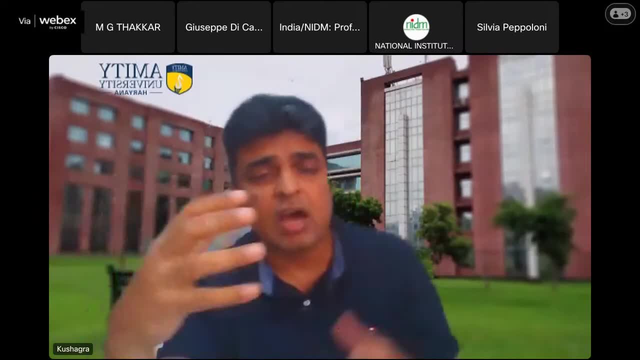 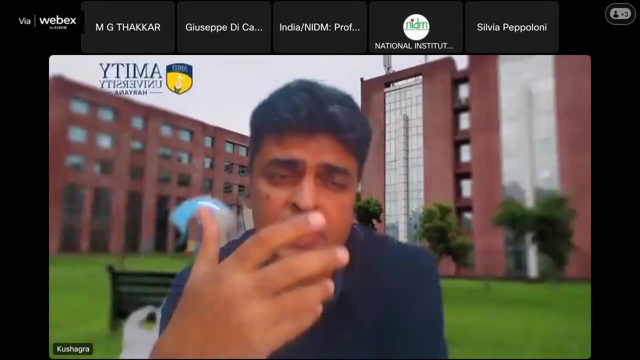 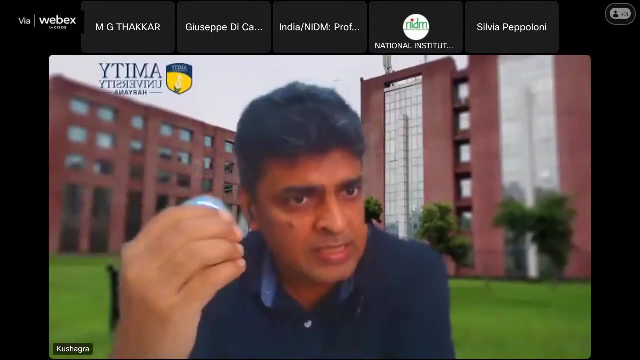 or thing we have it decide our ethical consideration, our ethical parameter. So, similarly, if then, if you go to the non-biological, or beyond a particular timeframe, geological in nature, then certainly there must be geological consideration, But our theoretical constructs, construct suggests, social constructs, suggest suggestions. 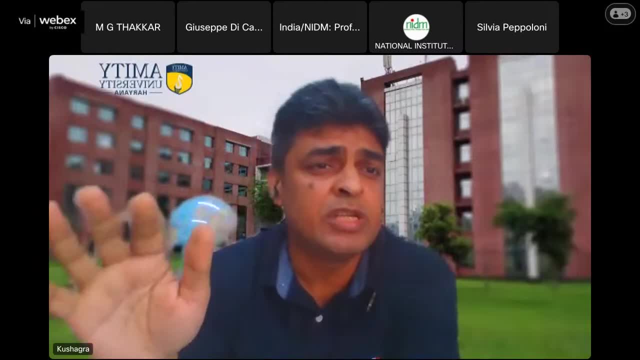 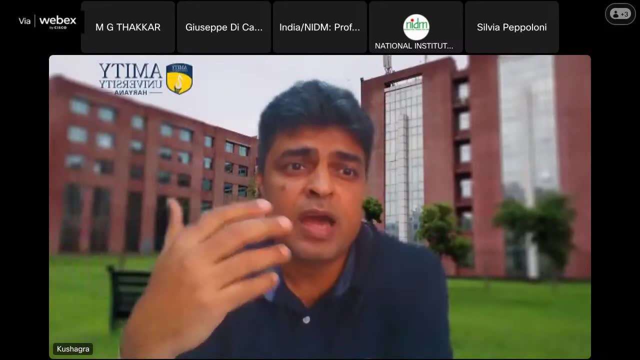 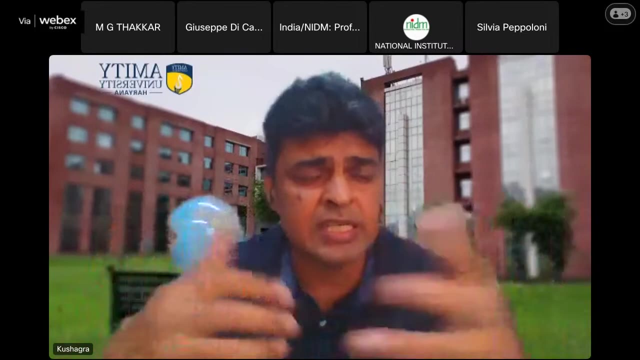 that the extent of the ethical attachment is going to be a little bit lesser than what we have with the first three, whether it is historical, paleontological or archaeological Now, but suddenly we started talking about geoethics in such extent then, it comes to our mind So: 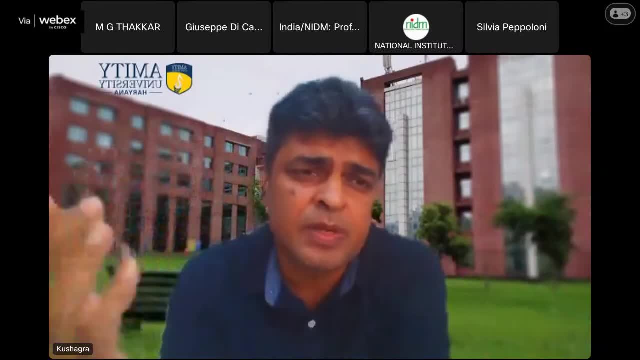 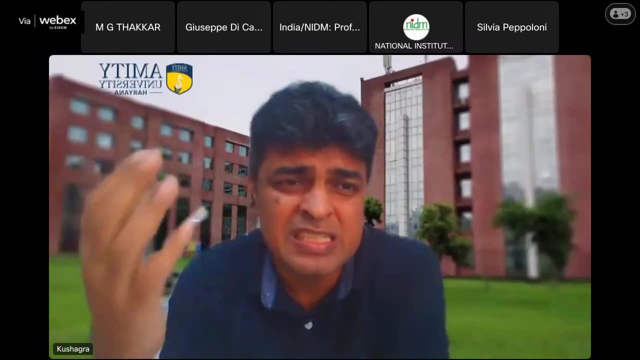 geoethics. it seems some off-beat subject. Why is typical geologist or typical student of earth science or environmental science or sciences why there is a need to go through the geoethics And, similarly social science? people might think. what is need a science people is talking about. 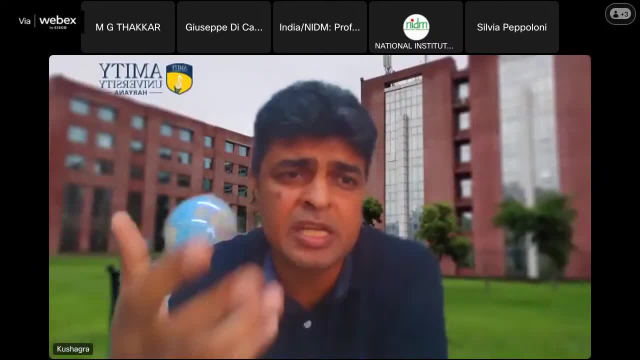 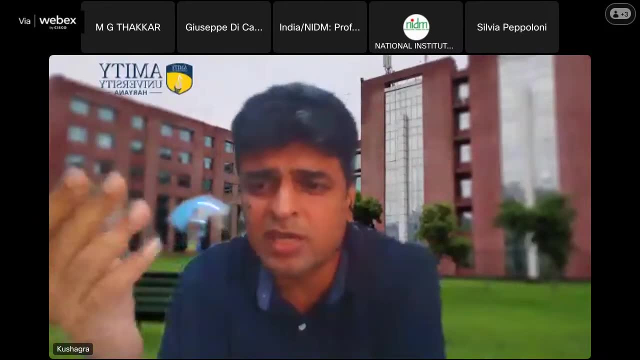 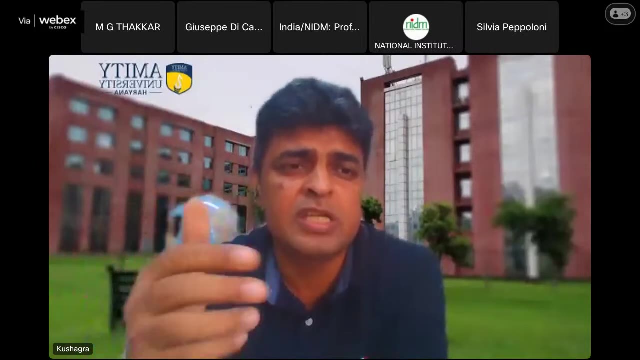 the ethics. It is our domain, we take care of this, But there is very fundamental reason to it And I am going to give you three, four different examples how it is required to discuss today why to consider geoethics for our day-to-day activity, whether it is 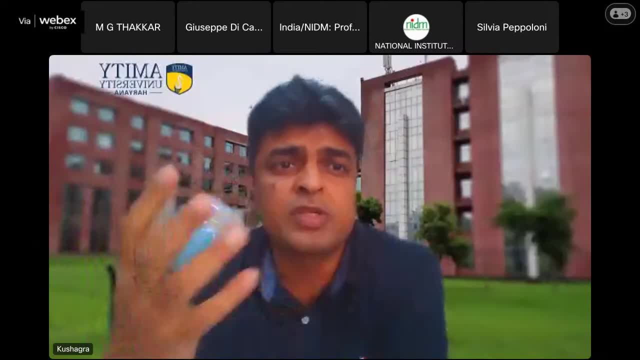 a profession, whether it is the kind of work we do and interaction with the nature. So I will give the first example. I will put my case with the very first example, and everyone know about it And it is a well-discussed topic. 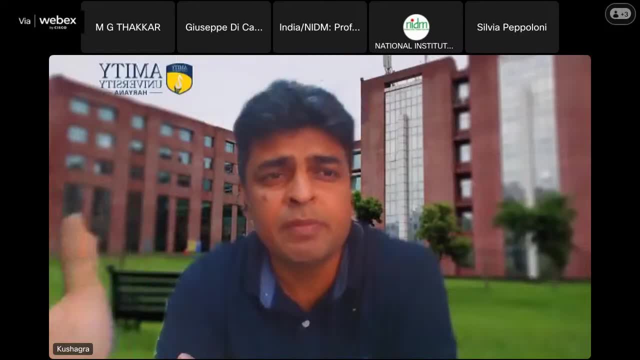 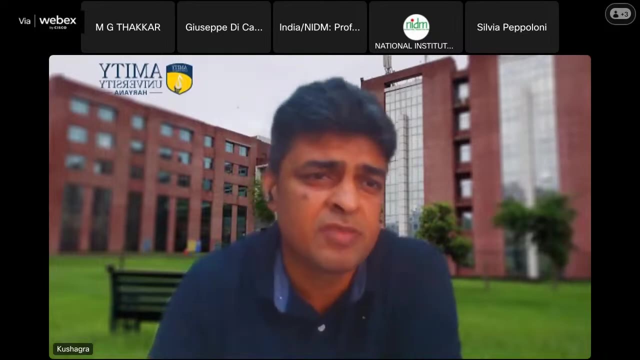 that is, Aral Sea. I am pretty sure that everyone knows about the Aral Sea. Aral Sea was the fourth largest reservoir of fresh water on this planet. fourth largest reservoir. The area of Aral Sea was 1960 or 1950, as you can hope be the more conservative. The area was 68,, around 70,000. 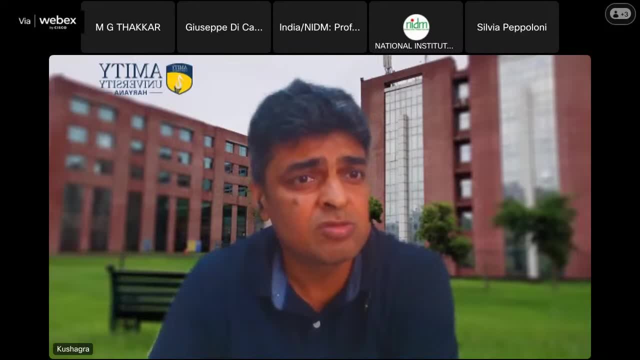 kilometers square, square kilometer area it had. So just imagine how big it is. In context of Indian you can say it is larger than many a state like the Jharkhand. it is larger than the Jharkhand, So big the water body it is. it was, But now it is shrink to 10%. 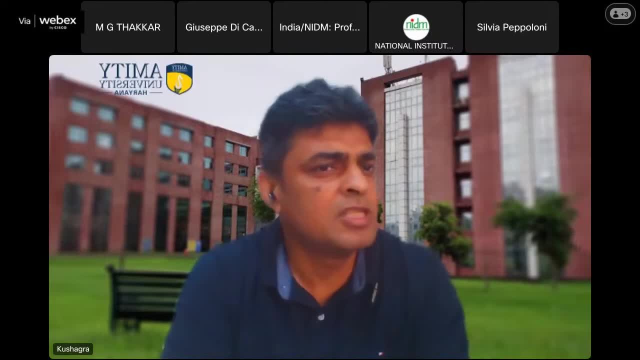 Now it is turned into the toxic desert. There is no water and hardly over 10% water left, and that too, after making a dam in the north side. What happened to that, And who is responsible for that? So the finger might turn toward us. It is the science people, it is the geology people. 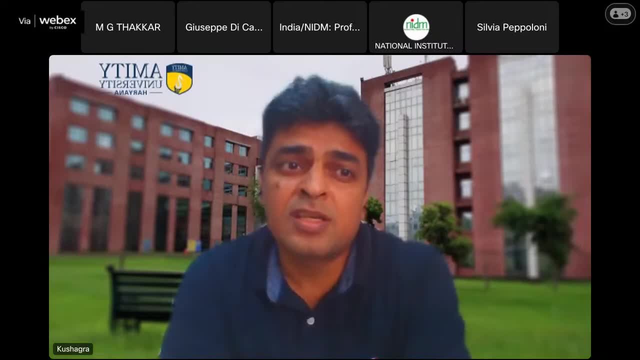 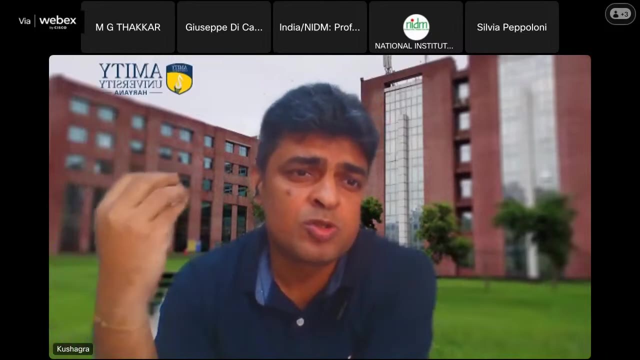 it is the engineers who plot the destruction of Aral Sea to the sea, the kind of destruction of Aral Sea And also the region you also know, because we want to have the more economic development, we want to produce more cotton, so the two rivers that used to fed the two 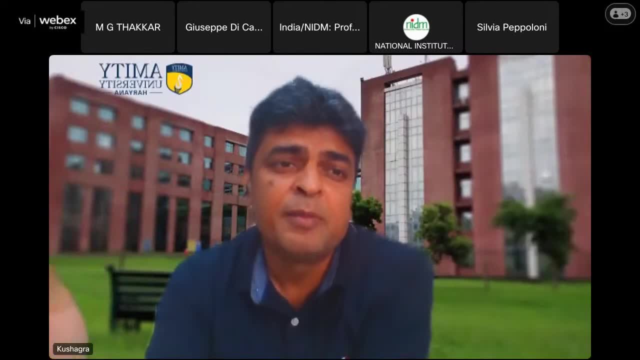 great civilizational rivers, Amod area and sea area. they used to feed the Aral Sea, but we had to divert entire water for cotton production, Although we had gained some short-term- I mean the developmental trophy. Yeah, Yeah, Yeah. 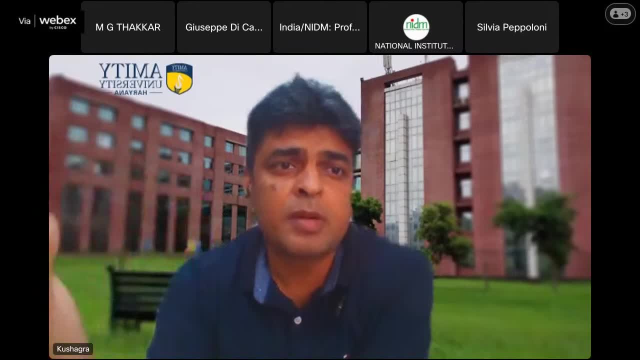 product producer of the cotton, russia become the uss. it was the time of ussr, but nowadays if you go you can find in the navy vessel inside a desert. so that's why there's need to talk about the geoethical considerations. that's why we need second case study. i put my case with the example. 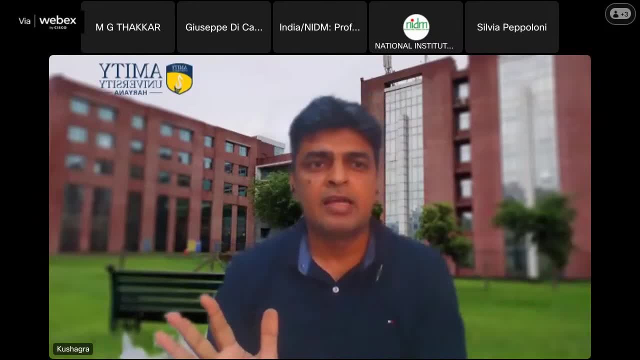 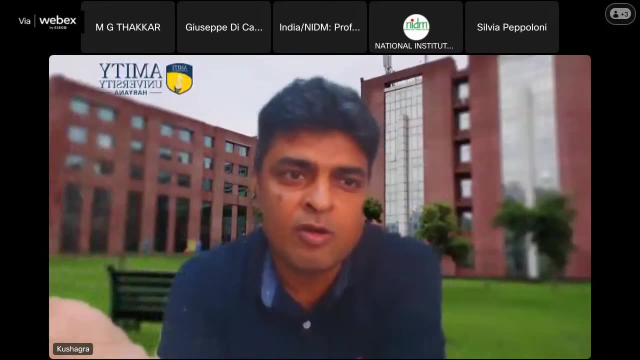 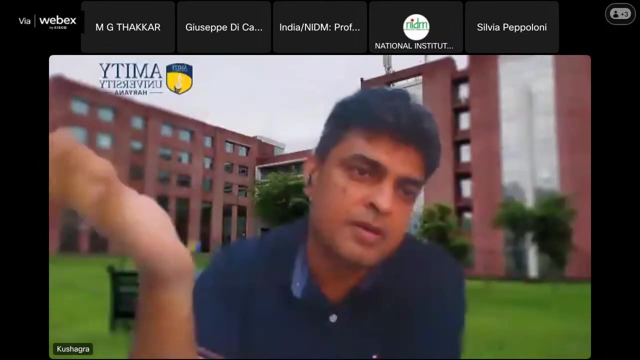 the river, very, very holy river in india, not jamuna ganga. i am going to talk about the jamuna. so zamana originated from jamanetri and it fall down from the mountain to the plane at dark pathar and from there it passes through several township and finally come to delhi. from delhi, it moves toward one of the holiest place of the hindu culture, mathura and brendavan, where lord of it was the activity place of the lord krishna, and then it finally merged with the great prayag raj. but it is. it is very interesting to know that from jamuna 3 reaching up to delhi, we squeeze out. 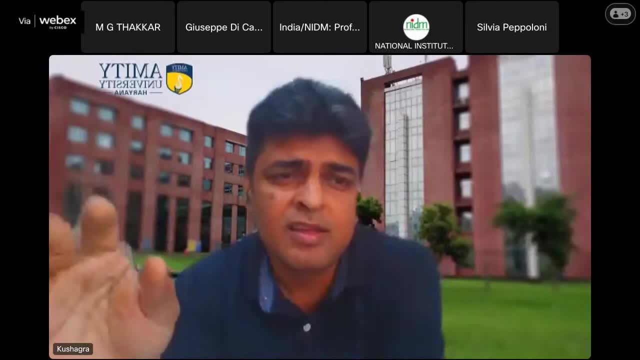 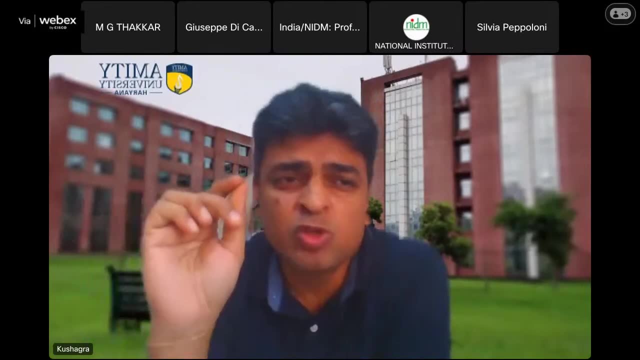 all water from yamuna. there is no water when it enter to delhi. they just see. and who is behind that? it is educated people, it is professional people. under the dictate of the ruling class, they squeeze out all the river. forget. i am not going to talk about that. 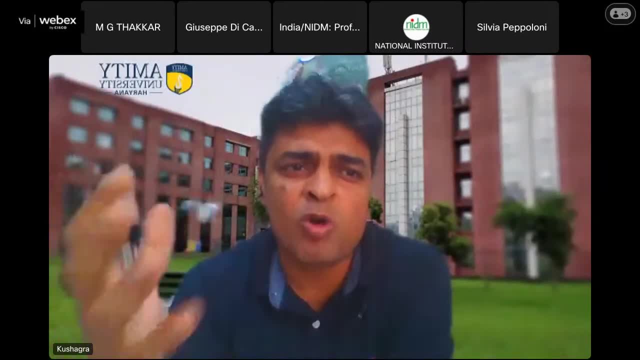 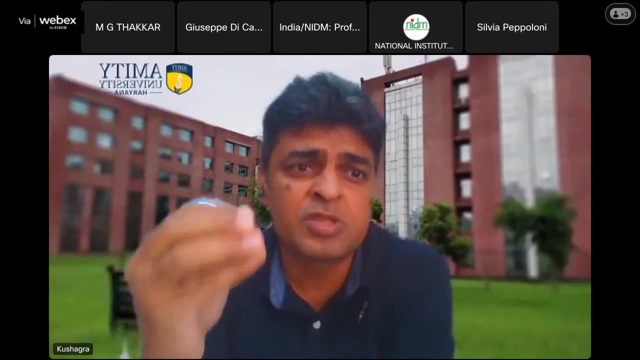 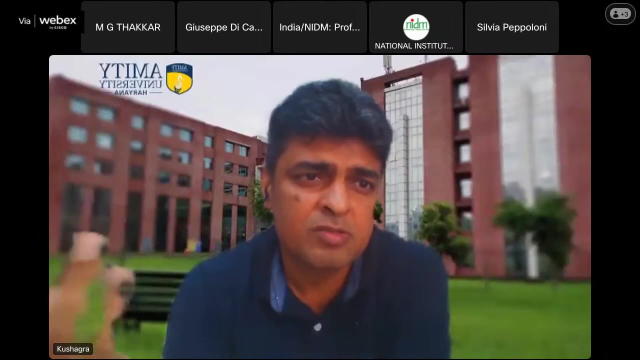 we have to produce agriculture productivity, but at the cost of the cutting down a river. so how long your productivity is going to survive? and whatever you see- well, i mean the in the ramuna. nowadays it is nothing, but it is our domestic waste. so this is the kind of and third, 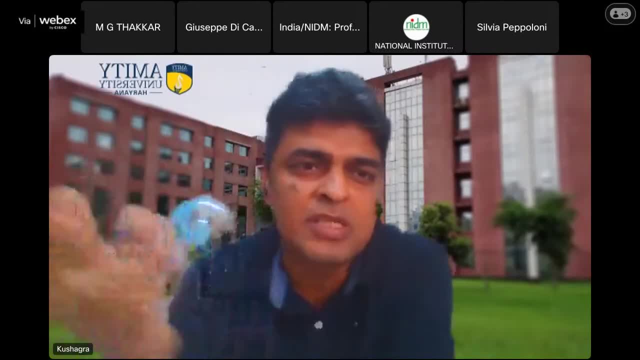 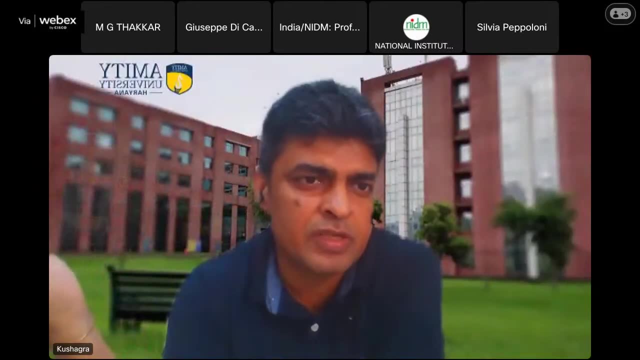 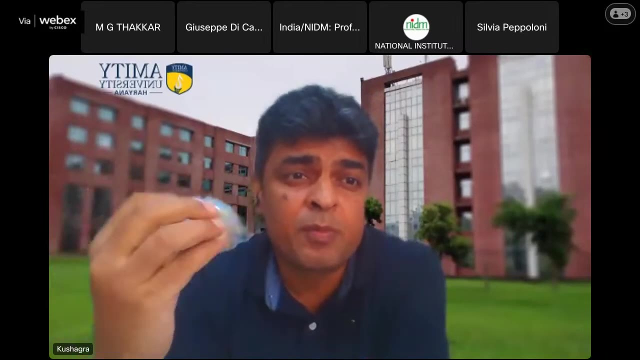 that is very. i mean the recent nature that some of the tragedies that we face in the natural disaster, natural calamities, but the last, in the last week we it is in the tista, in the assam, in the north sikkim, where 1200 worth of quarter worth of a power project has been bust, bust out because of. i'm in the 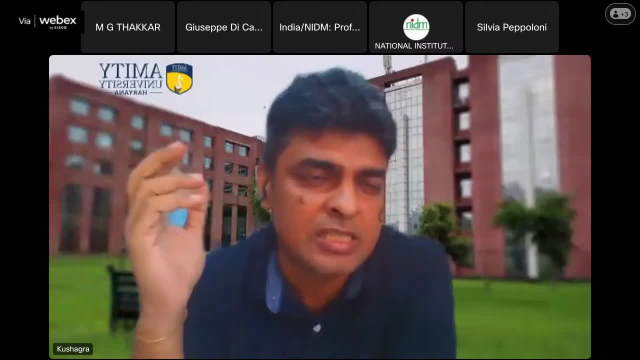 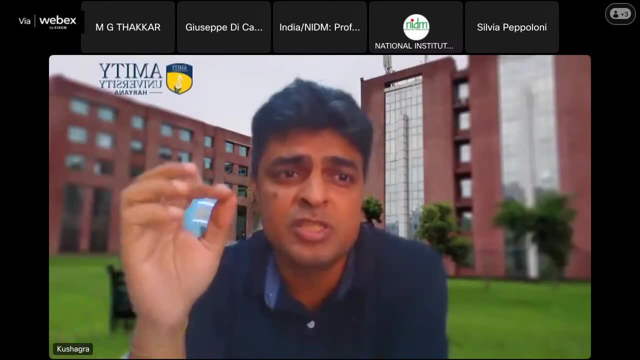 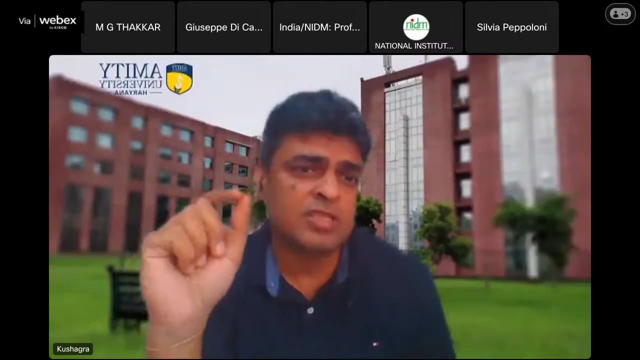 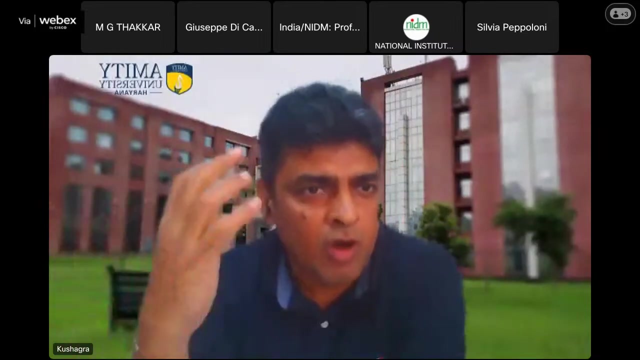 glove, i mean the brusting of the glycerin lake. so that's why there is a need to understand, to stabilize the concept of the geoethics. so geoethics is going to talk about your association, your value system, with the nature and it's great. it's great that we have very good social construct and how to go to i mean the 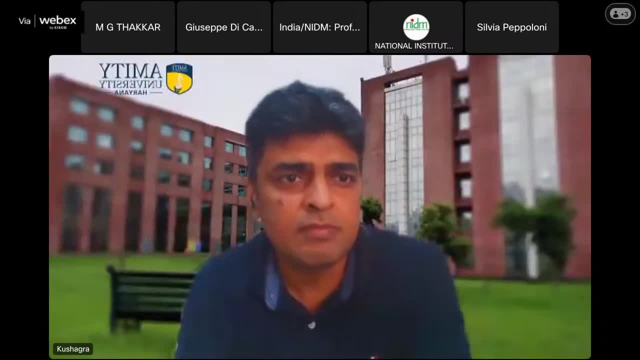 preserve how, but how we are going to develop the value system, who, what are the way we are going to be able to do that? and there is. i agree that there is a. there is a degradation of the social, social ethics as well, but at the same time, we have collapsed as far as our geoethics is. 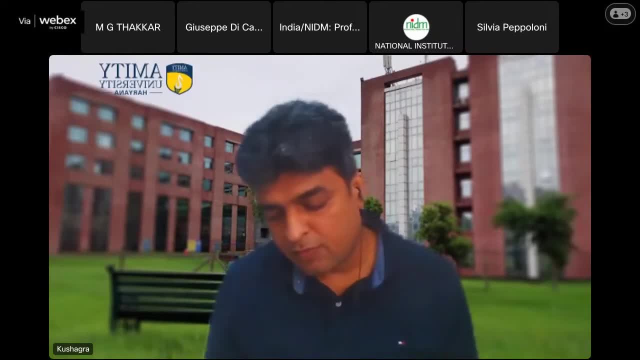 concerned. so these are the some of the aspect of the problem. so let's talk about the. now i have discussed the problem, but let's talk about what is the hope you have, the kind of the human activity and their impact. the impact on us is basically result of the our intense social behavior. 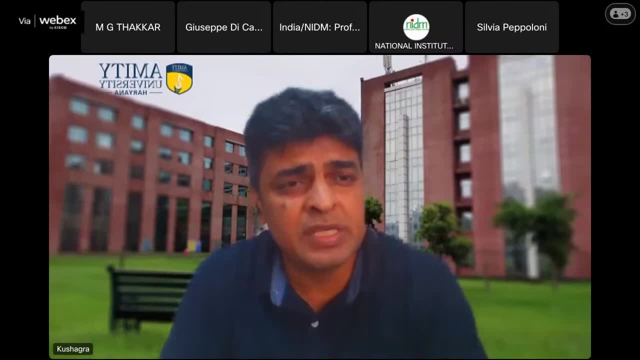 it's we responsible and this i. social behavior is nothing but it is. it is summation of our individual behavior. a very good example is the your table salt that we consume every day. every people, not a single person on this globe who do not have the table table salt daily, but i know it contain. 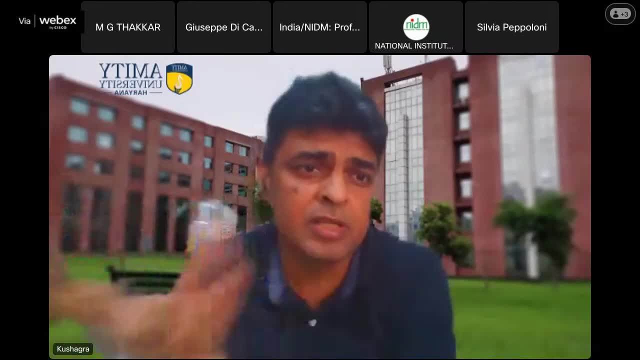 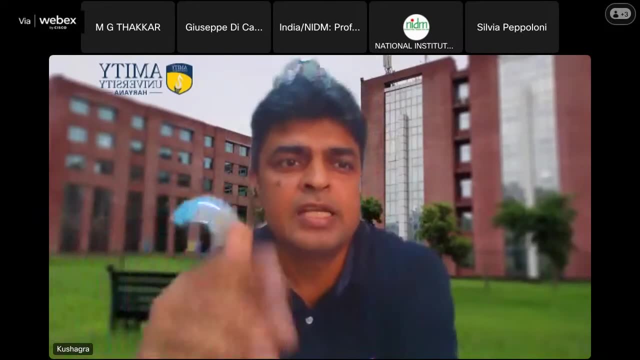 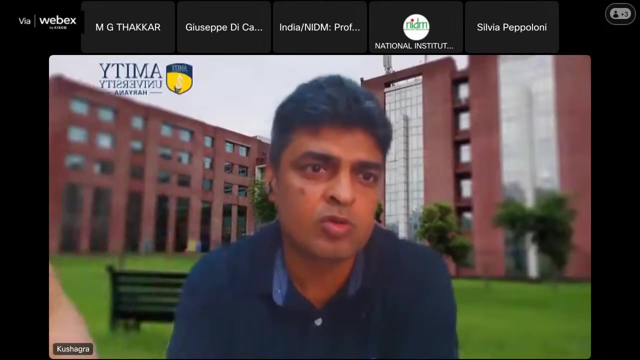 microplastic. it is the same plastic, then everyone is used like anything. so it is going to ocean and from a churn down turn into the microplastic and deposit it at the course, at the shoreline, where your salt is extracted and it finally transported to every household. 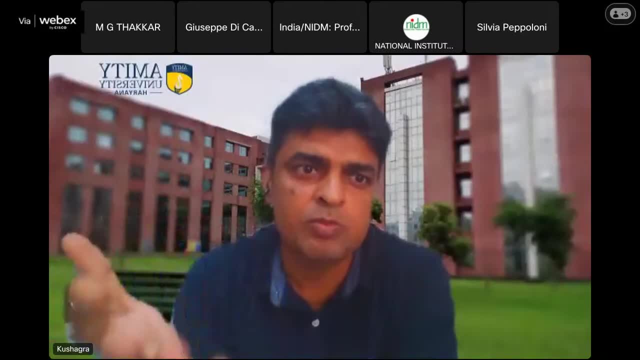 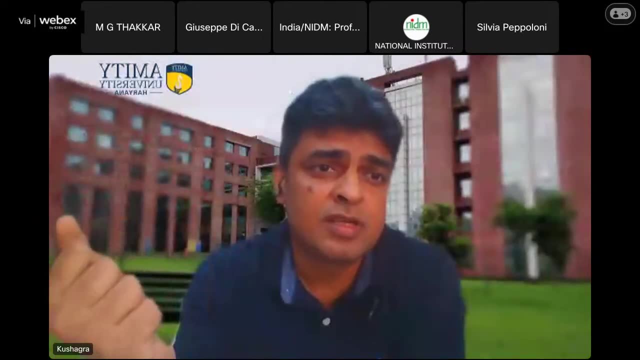 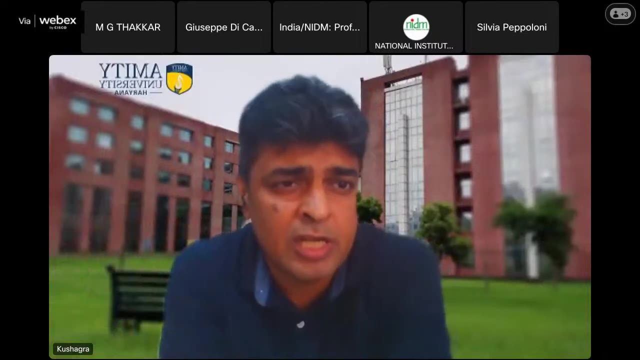 then look, see and consume the microplastic that you brought on this earth in last 100, hardly 100 year, for the last 100 years. so what are the solution? so a very, very enough innovative uh approach has been adopted by some countries, particularly latin american countries. 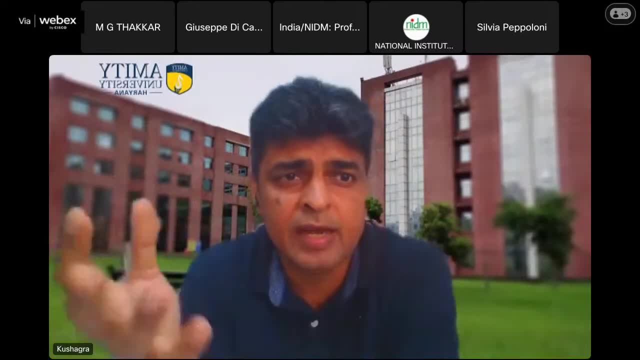 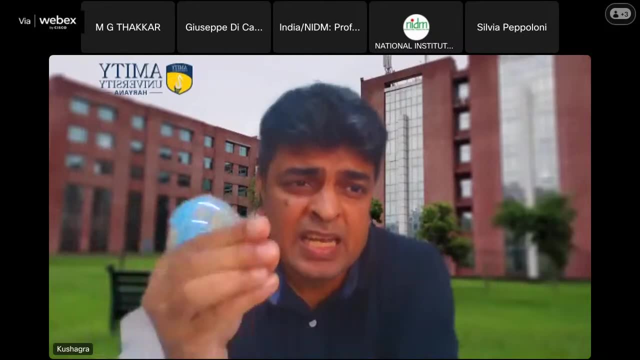 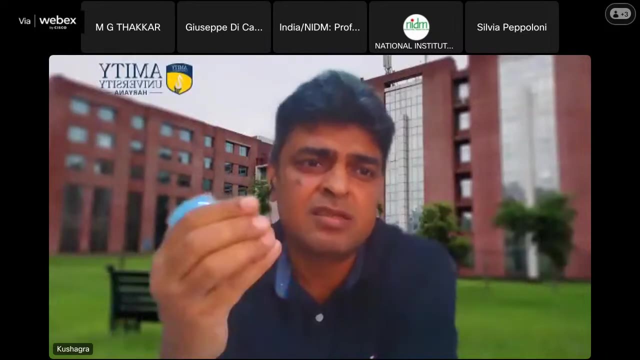 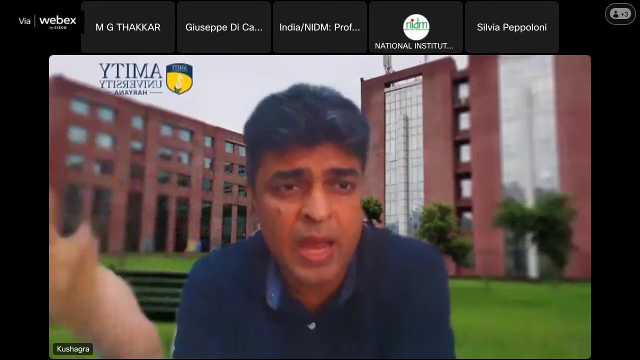 new zealand is that, for example, in few cases study from the canada that bring a completely new perspective to it and that is giving legal rights to natural resources, geological, natural legal rights. i mean give a. so although in indian constitution in in 175 years back, it talk about the conservation of forest, conservation of nature, conservation of. 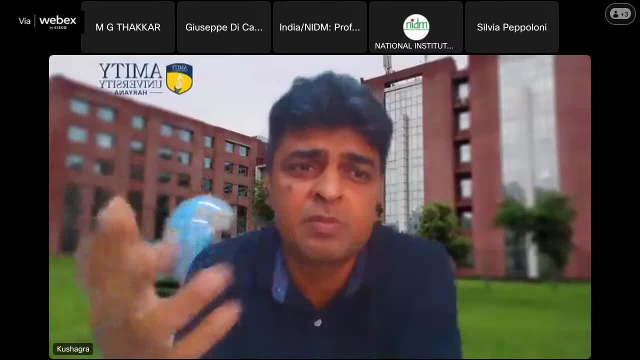 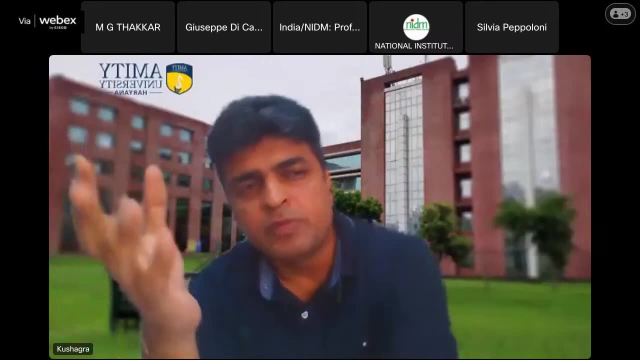 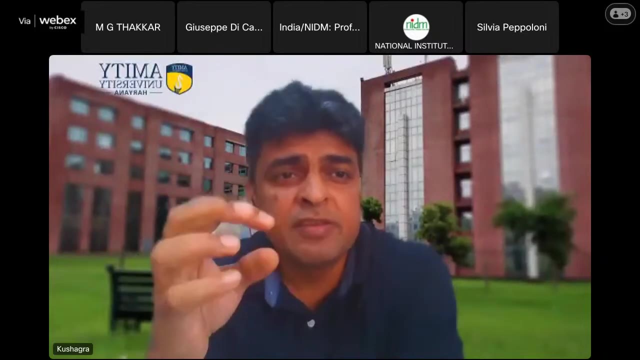 water, but that one mandate, not mandated, but it is in the directive principle. what should be? but the, the, the. the story begins with the, bolivia, a latin american country. it give legal status to river. it means river is like a human being and if you give a legal status to a, 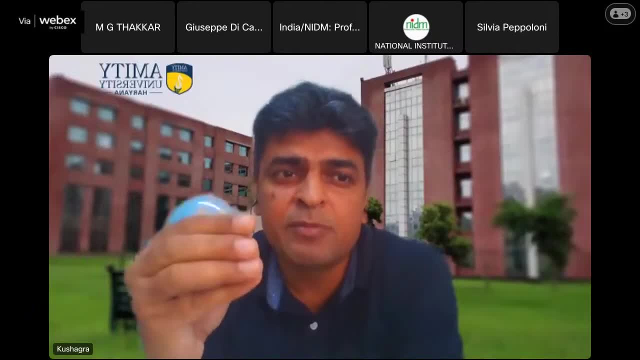 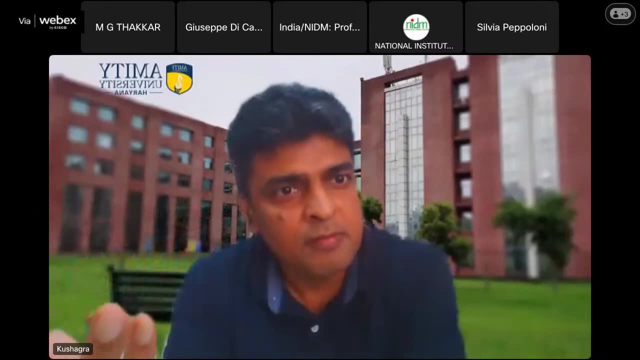 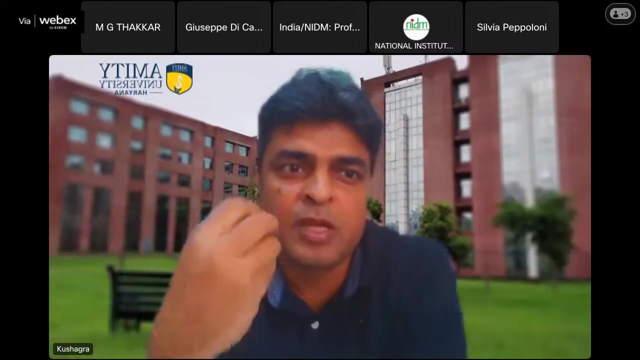 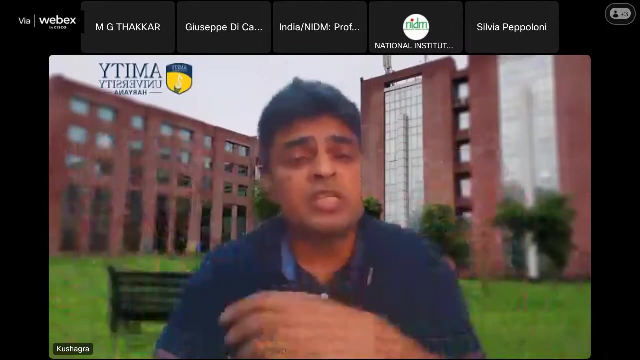 river. it means to have the all the fundamental rights, what the human being has, we enjoy. so, and what? what can be the fundamental light of the river? free flow, conservation of their ecological system, and what, what not, what not? i am seeing what not. so so now it is become the mandatory for government to safeguard their fundamental conservation of their fish and sea, while watching and what the reality also means, that the entire, the whole peoplefمر of the ocean is there for food and sustainable Shelley. it needs to be manged, these rights in some way kind of question, by definition. you know that this is a political and something raise the sama, the treatment of spending all these. 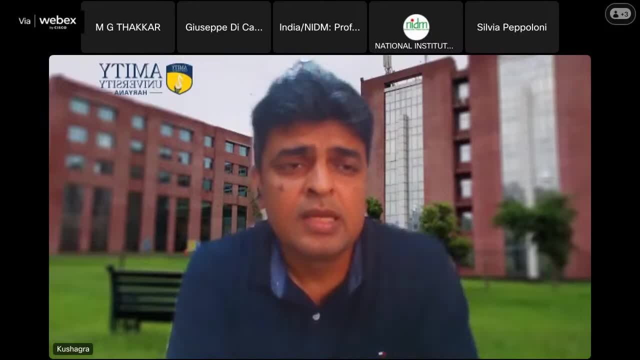 right, i mean the fundamental right of a river. this is one example, another very good example from: uh, new zealand, uh, particularly, i think, in north island. uh, there is a, there is a, our originals, although the term is not a term, is very racial. so there is maori. 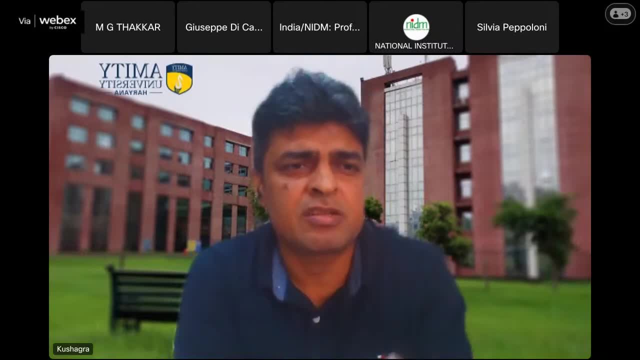 they, their, their entire livelihood is basically in the nature, with the river, with the mountain, with the national park. so everything is is a part of their life. so that particular system has been given a living rights and who make the custodian? it is the maori people and government representative. 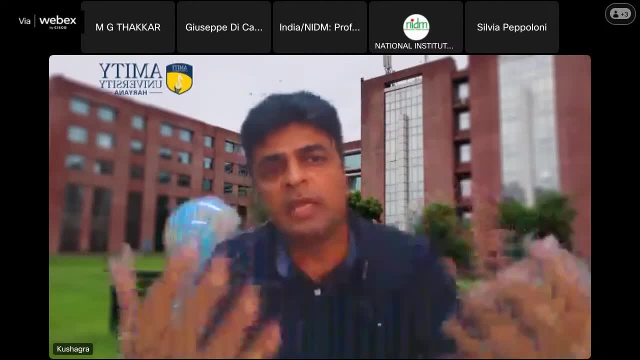 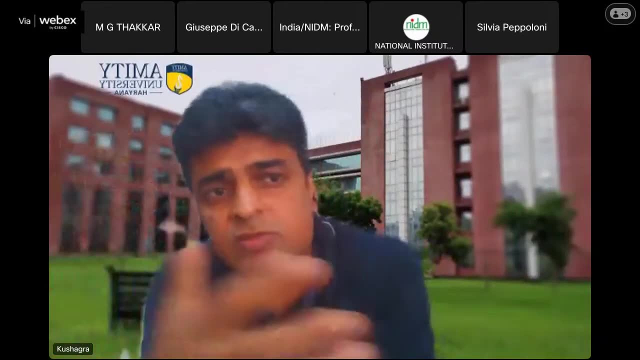 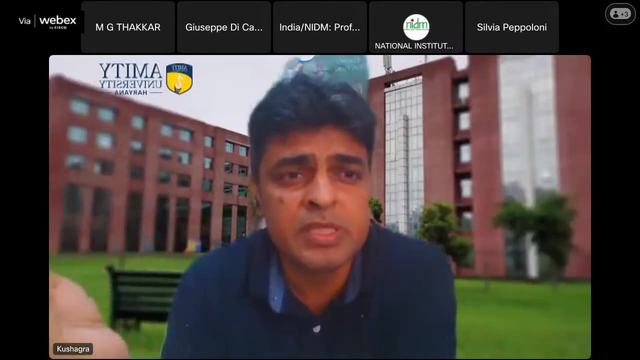 is their custodian or they are the guardianship. so, with the help of guardianship and now this is a very good case study, but why? i am talking in the context of india, india also- that effort has been- i mean taken by one very famous uh judgment 2017, uthrakhand high court- given legal personal value status to river. 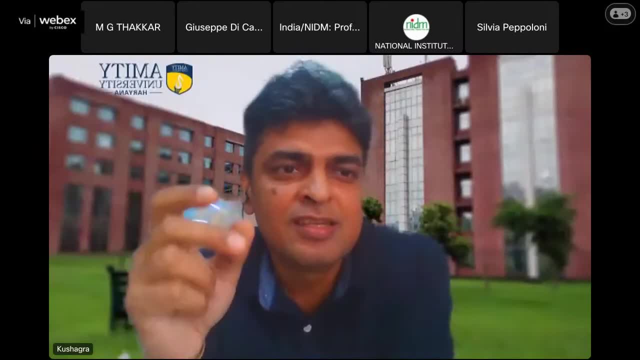 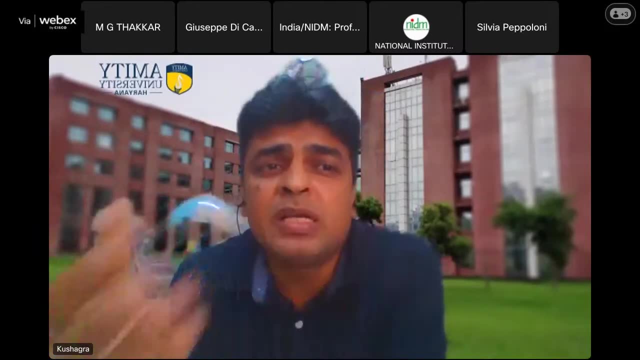 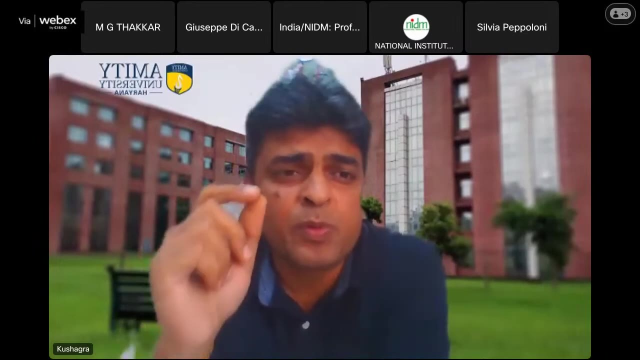 yamuna and ganga, and who make custodian? the custodian was our guardianship was by the chief secretary of state. unfortunately, only the government represented were the guardian. so the fallacy is the philosophy was that it is the government. many proposals or many projects. 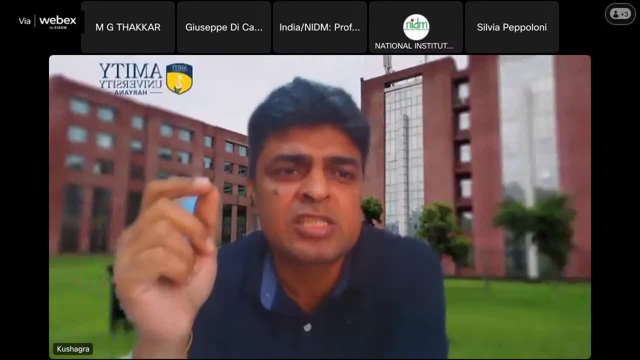 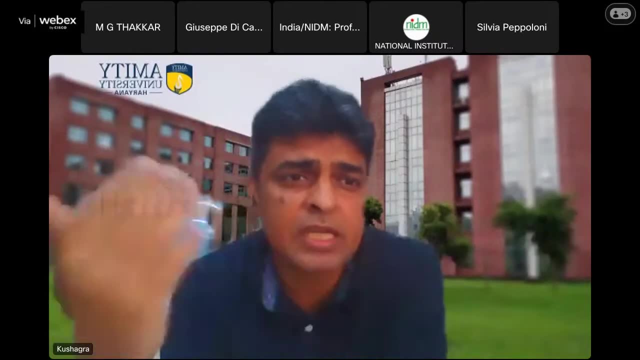 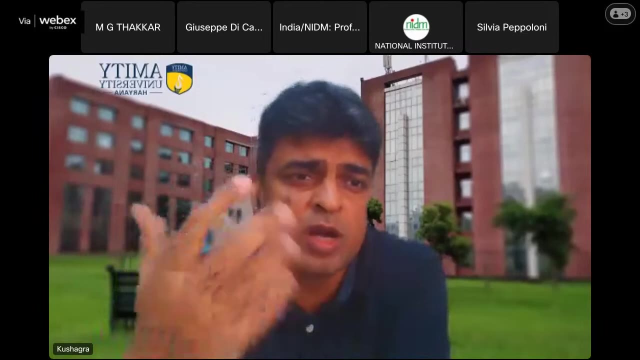 are majority of time is not in interest of the river, whether it is making a dam or making a multi-purpose project including the extraction of river and others. so government of india has a very good case to to- to i mean the file in the supreme court against. 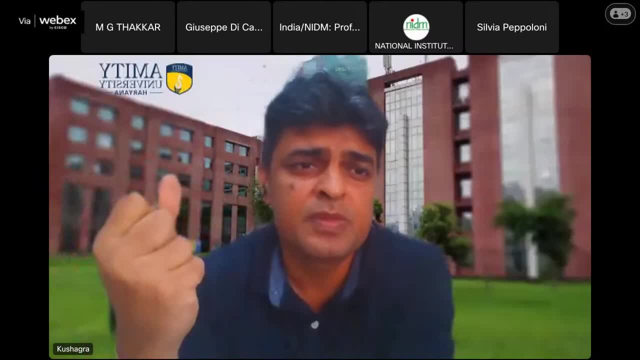 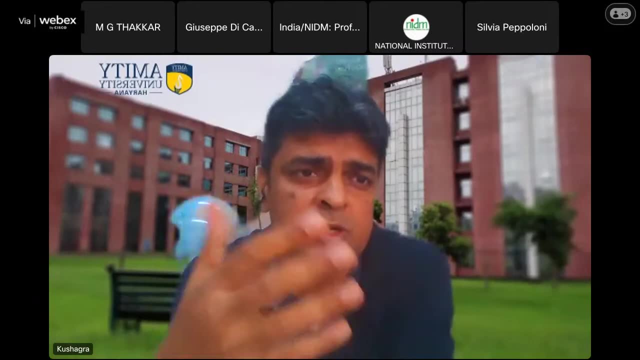 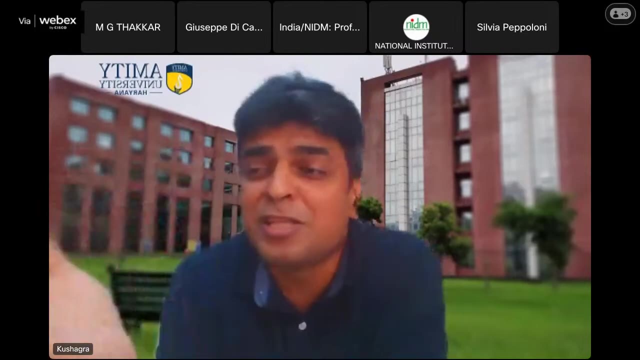 this declaration because they have very good point. and the point is, if you make a guardian soup to the guardian of the river, to a government imply, then what about if some damage is caused by river? suppose there is a flood in the river. so very, very, very interesting, i mean a very funny. 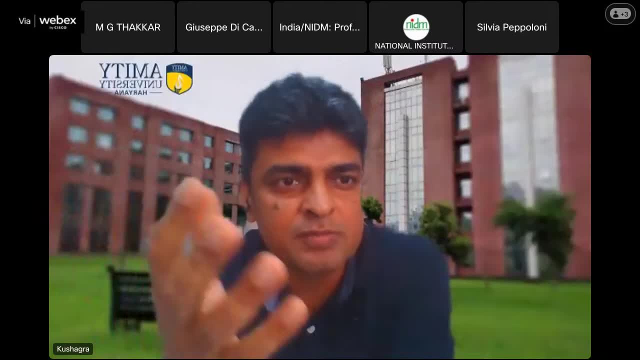 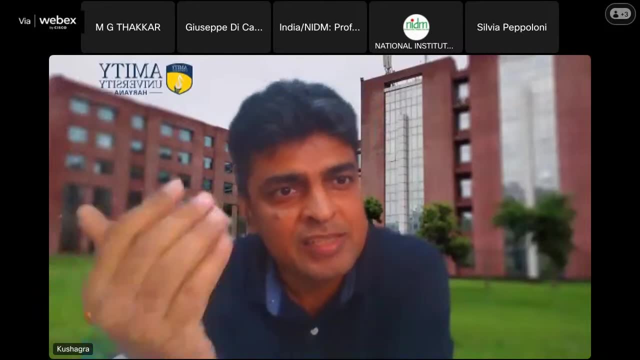 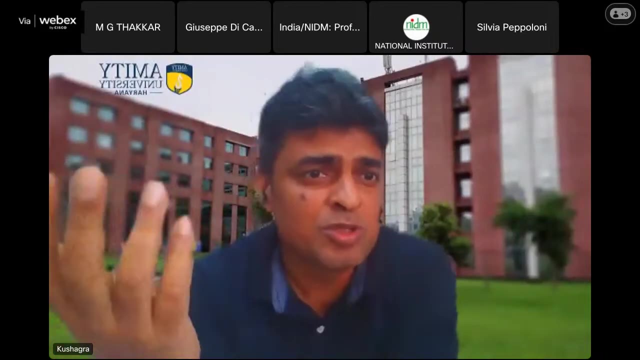 thing. so government come up with the supreme court then okay, kindly quest this order, because if the river is very infamous for the flood and if the damage is going to- i mean the ask for compensation, who is going to pay? that the chief secretary is a very i mean the pedestal paid imply of the 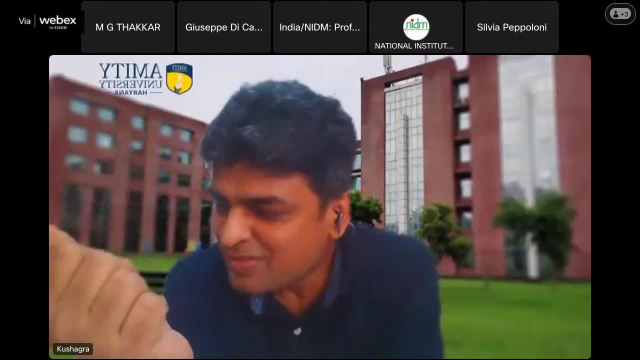 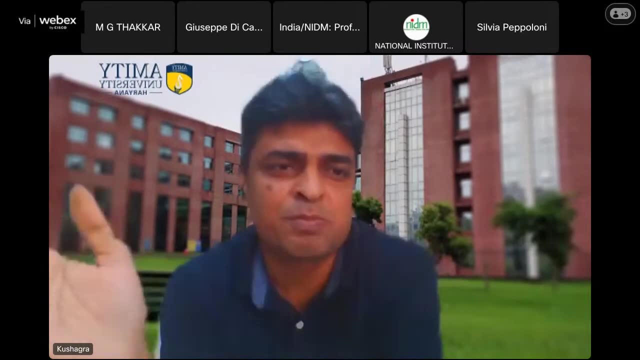 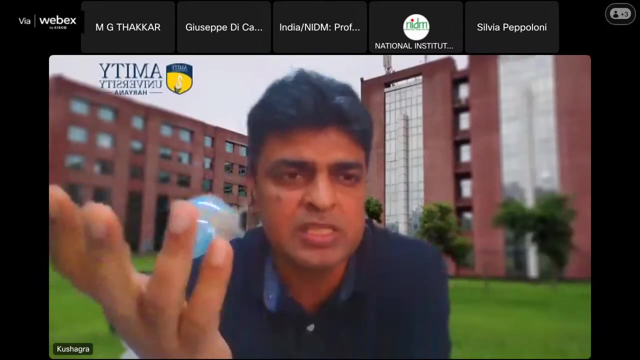 government why he is going to pay all these things. so, on this very simple legal reason, supreme court rejected this. i mean the quest, the order of. so it was always very good opportunity that we should learn from the other experiences, but instead of providing proper safeguard to river, 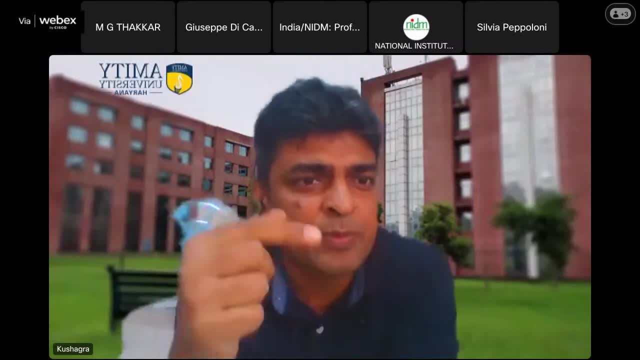 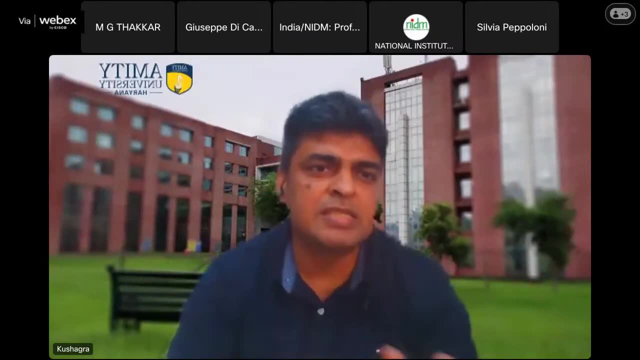 supreme court taking the uh escape route and rejected the plea. so this is one of the expect that i already mentioned: i will try to streamline or mainstream the concept of the geoethics. so, uh, last but not least, i again quote john mallory: and i want to conquer everest, and he told very famous, 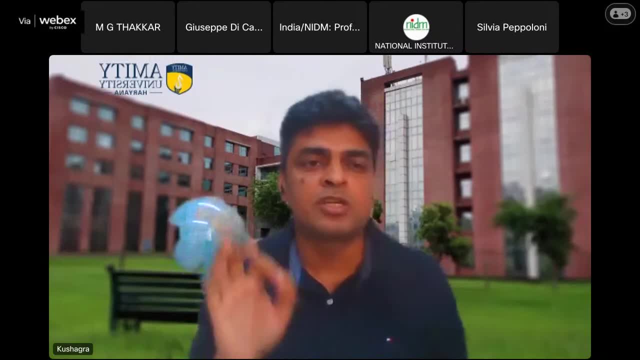 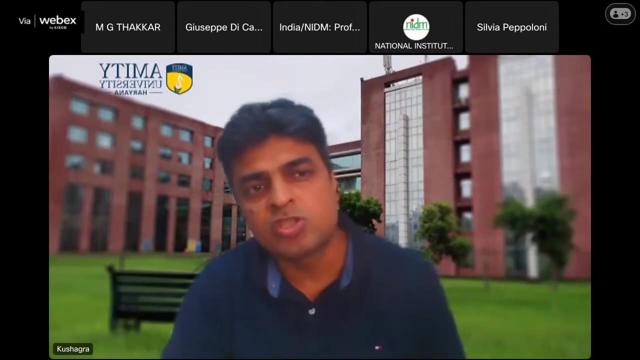 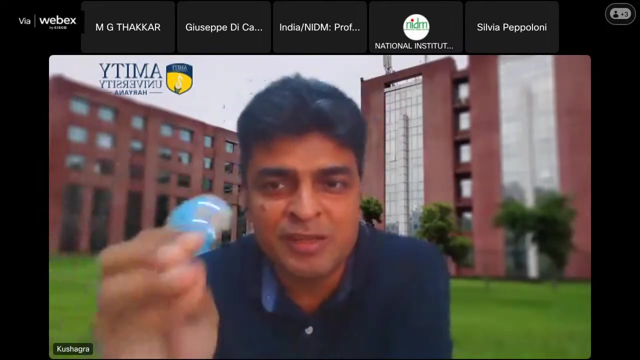 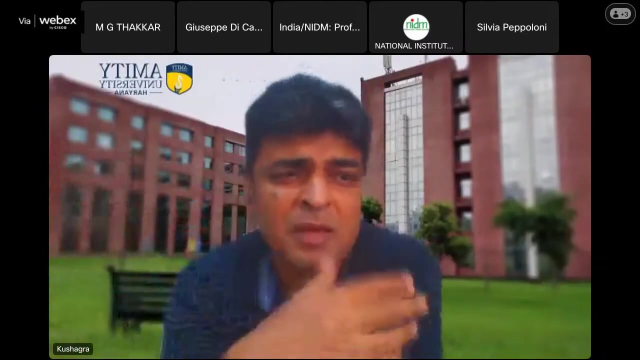 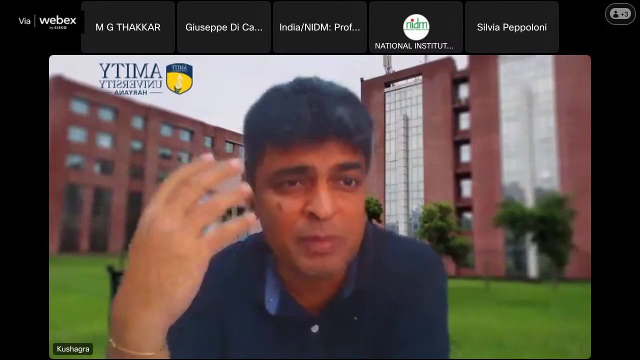 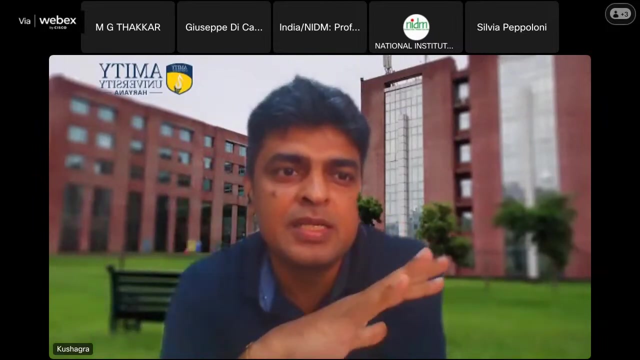 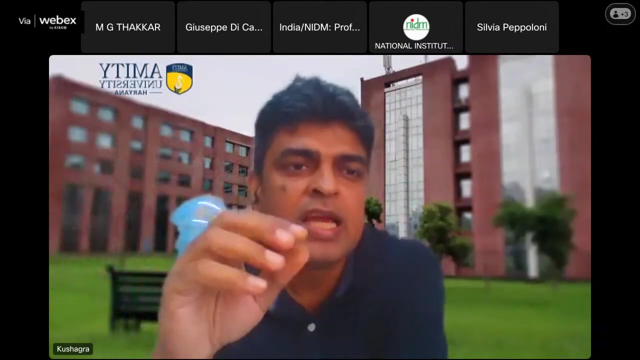 because it is there. so it is very pertinent to preserve our geo heritage sites. stones, the one of the interesting topic, although the name is very complicated, i'm very difficult to remember. even i used to forget. so if you is, overlap the entire life scale, life of the earth, i mean geological time on a watch, 24 hour watch, and also overlap 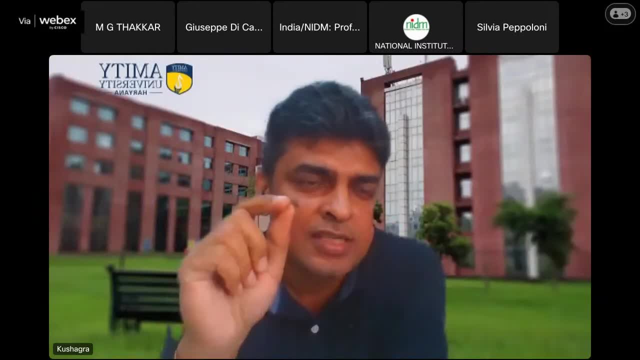 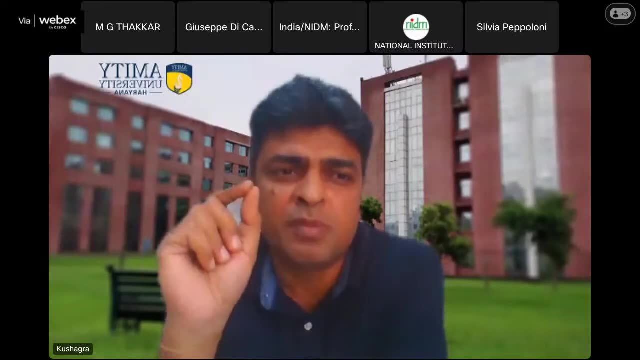 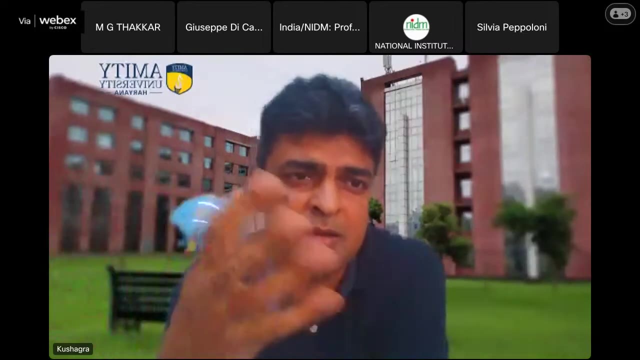 the human existence on this earth, then we'll find the human being on this earth for last three second: Human beings- I mean, it is not the human sapiens but, a little bit earlier, like the human kind of species. So we are here for the last, just last three seconds. 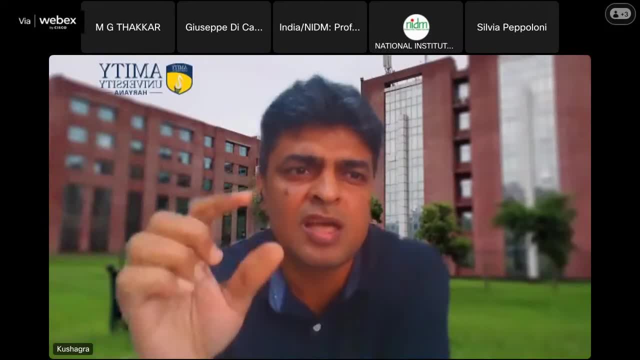 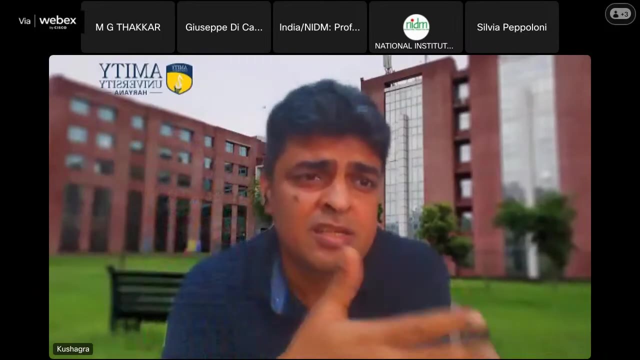 Out of 24 hours, our existence on the earth, for the last three seconds, And in just last three seconds, effectively much, much less, or even the fraction of a second, because last 500 or 600 years is very important, and that too last 100 years or 150 years. 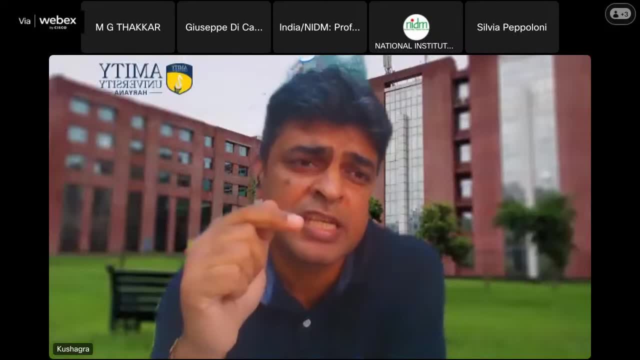 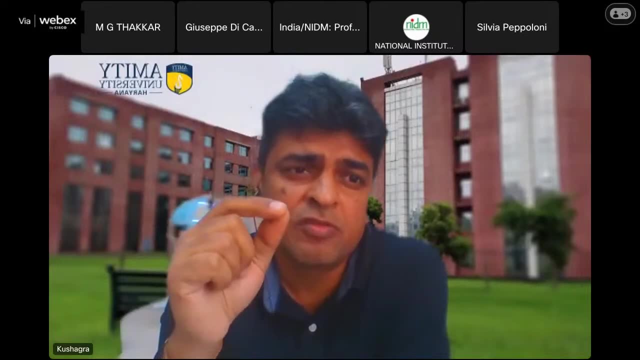 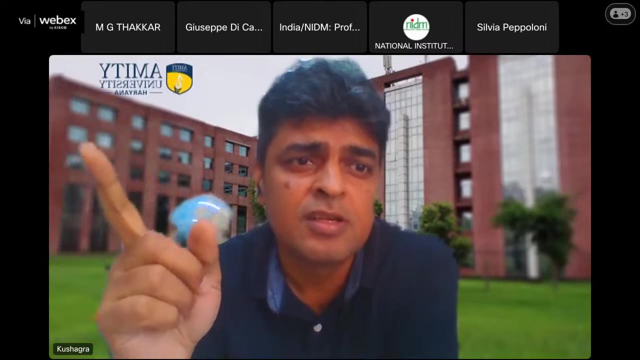 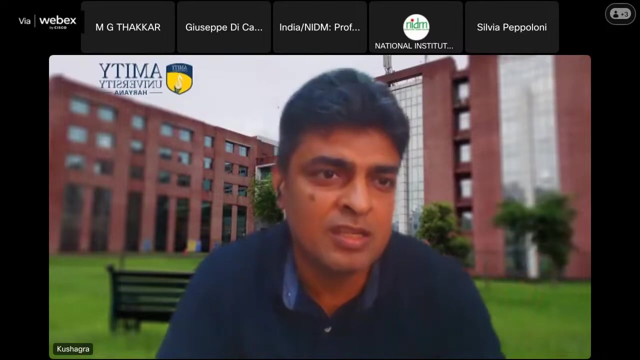 The fraction of second, the activities of our fraction of second make such a situation that nobody is going to say with the full confidence that we are going to stay on this planet for the next second. So with that word I conclude my case. I hope I am able to contextualize the today webinar. Thank you very much, And my regards to all my teachers and participants. Thank you very much. 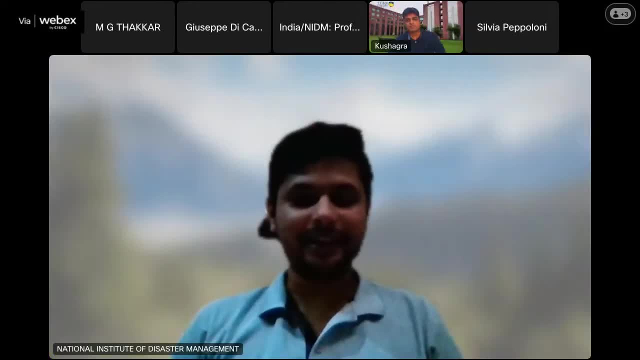 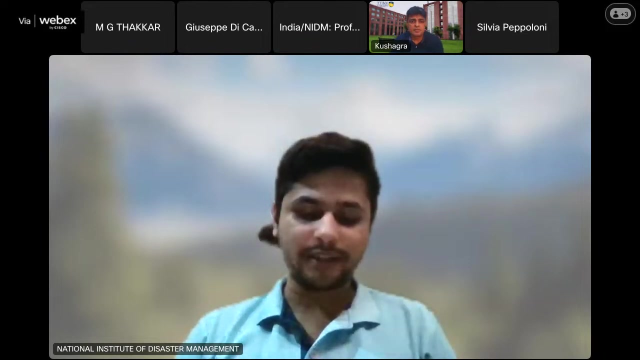 Thank you very much, sir, for joining and enlightening us with the knowledge. Now I would like to invite Dr Parveen, Assistant Professor GS Tompe Art Commerce and Science College, affiliated to SGB Amaravati University, to give summary and way forward for this webinar. 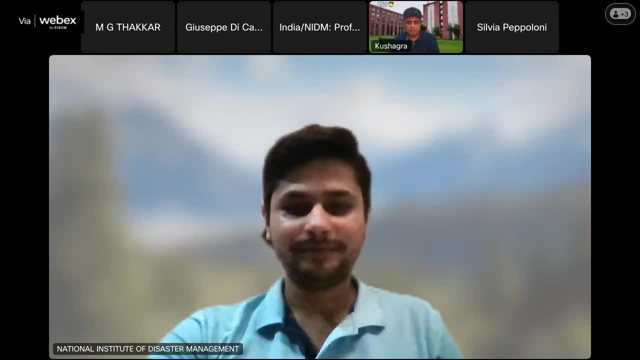 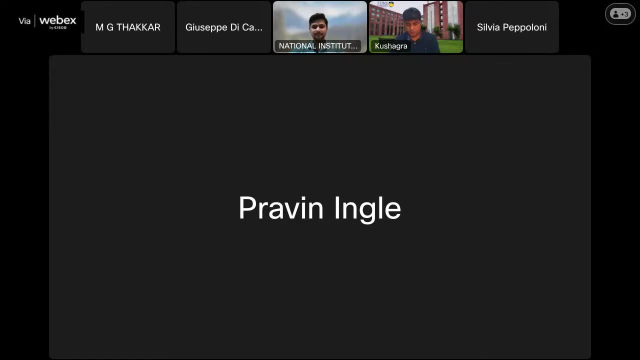 Over to you, sir. Am I audible? Yes, sir, you are audible. Okay, okay, Camera is on or off? Yes, sir. Thank you, sir, For giving me the opportunity for summary and of thanks. Dr Thakkar said that your tourism visitors have diverse. 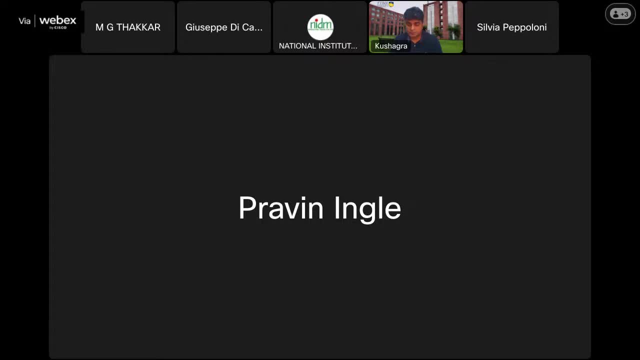 Motives and interests. Interpretation therefore needs to meet The requirement of a border spectrum order. audience from from the needs the specific website related geological and educational information for the dedication tourist and those actively seeking to learn about the geology of an area to the broader interpretation. 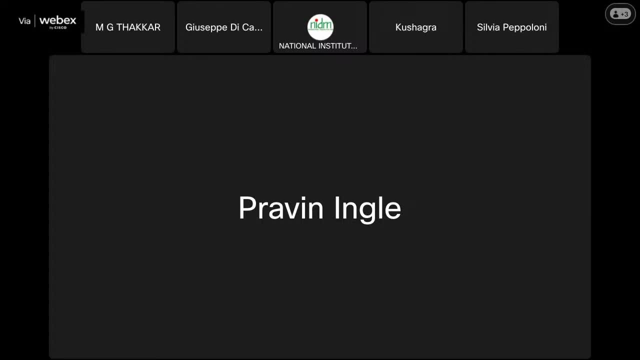 that will engage and enthuse the casual tourist and those who simply wishing to be there, and enthuse the casual tourist and those who simply wish only so that their experience is enhanced, but also that their awareness of geoheritage and the need for its conservation is increased. 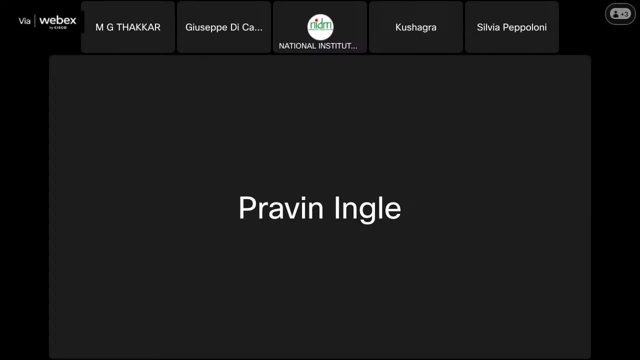 Dr Sylvia Cipollonea and Dr Tushagra tells about the geoethics and geoconservation depends on better public awareness, understanding and support which tourists and geotourism has a vital contribution to make in achieving these goals. 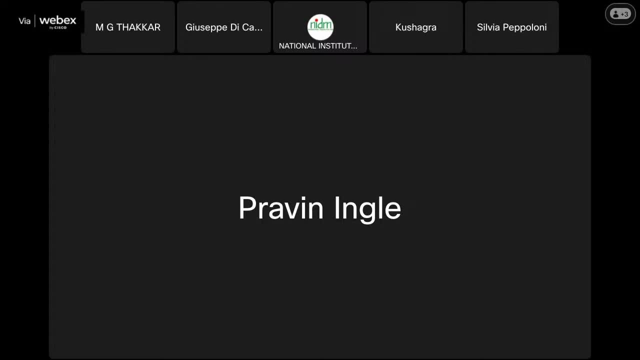 Strong geological stories that appeal to the imagination are essential, but the visitor experience for both dedicated and casual tourists can be enhanced through exploration of the connections between geoheritage and the cultural landscape. Now it's time for oath of thanks. Good afternoon all. I feel honored and privileged to 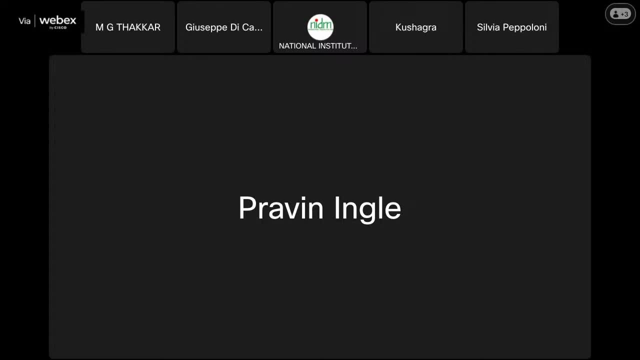 get the opportunity to propose a vote of thanks on this special occasion. I would like to thank all the honorable delegates who blessed us with their presence. I am also very much thankful to all the program advisory committee members and the invited speaker. Words are not. 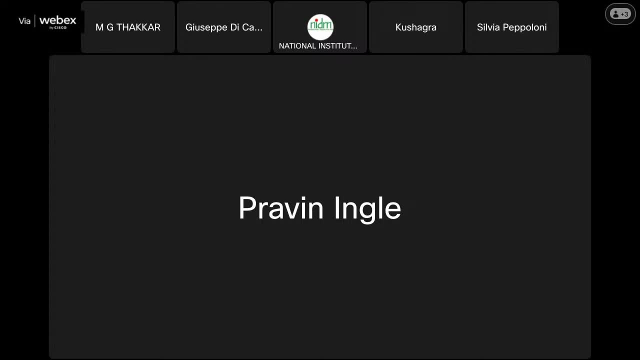 enough to thank their constant guidance and support to shape the webinar. On the behalf of the organizing committee, convey deep regards and heartily thanks to all, to our honorable guest Professor Mahesh Thakkar sir, who graced us with his kind words, and sincerely thanks to. 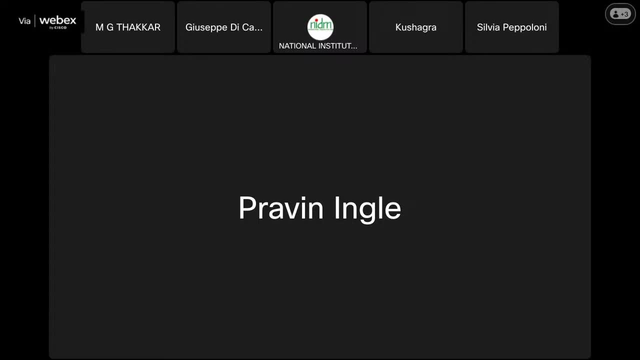 Dr Sylvia Pipulonia, Dr Gurusipa D Kapua and Dr Pushagra Rajendra, sir, for his valuable guidance. Today my words are not enough to express gratitude to Professor Surya Prakash, sir, and Rajendra Ratnau, sir, for his. 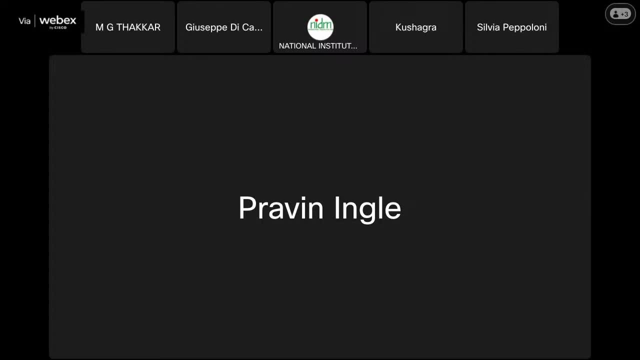 for his help and guidance that radiated a source of energy with us. I would like to thank head of department Professor, Dr Yadav Kumar Malve, Dr Neeraj Khan sir and Shubham sir, who helped us and supported us at various stages. 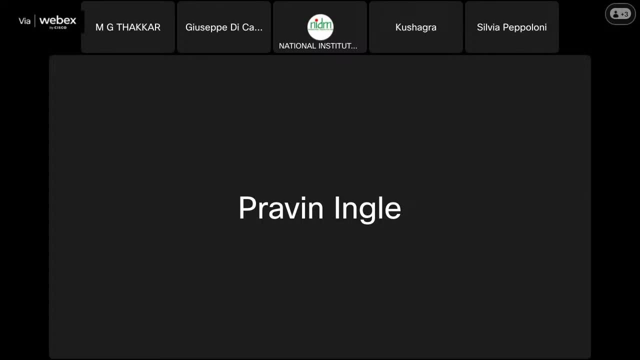 I am very much thankful to the NIDM team members, because it will have been impossible to organize it with their support. If time is money, then today you have spent millions for us. Thanks to all of you for making this event successfully. Thank you, sir. 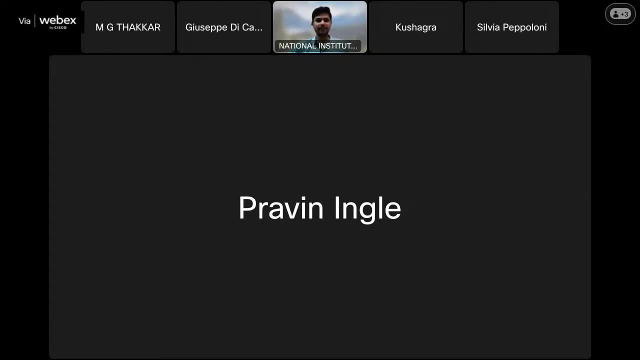 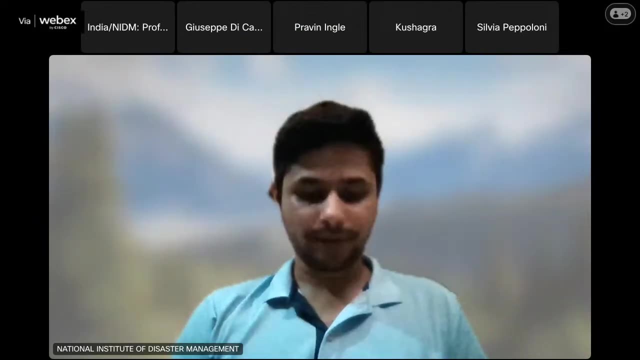 Shubham sir over. Thank you very much, sir, For summarizing the session and also giving vote of thanks. So now I would like to request Dr Yadav Kumar Malve, head department of geology, SGB, Amravati University, to give closing address. 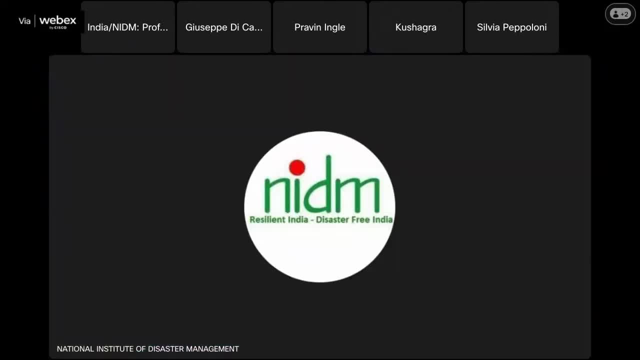 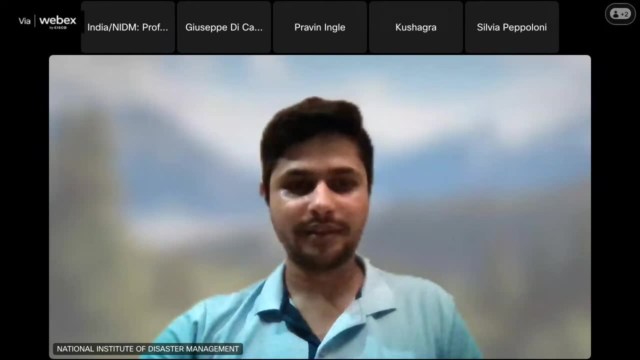 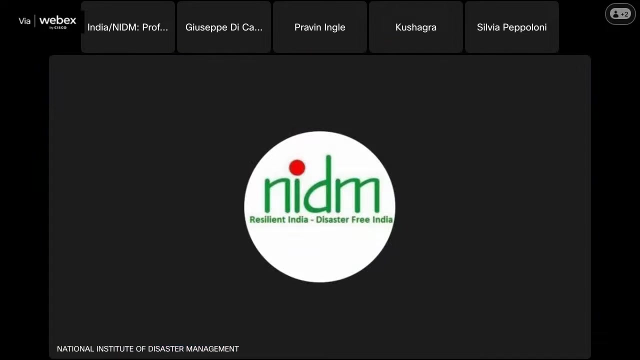 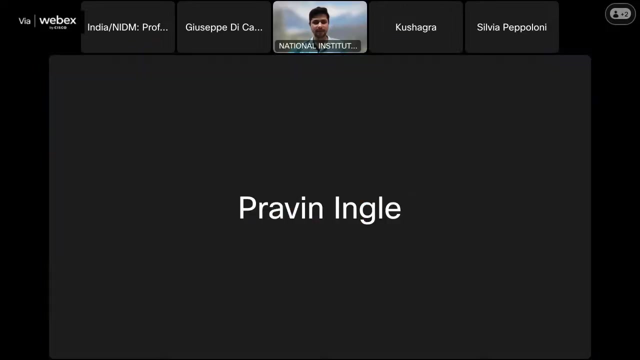 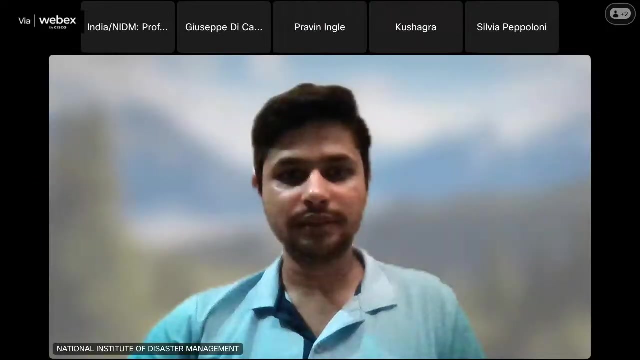 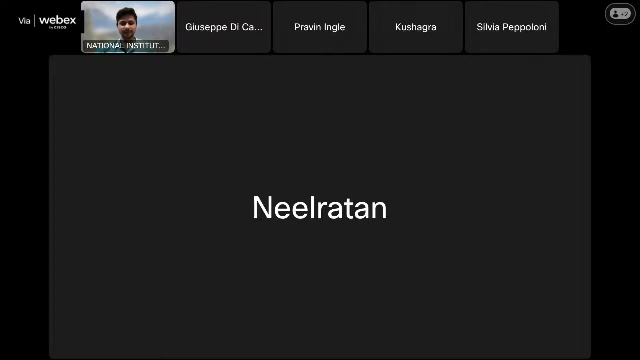 for this webinar. Hello, Hello. Yes, sir. I think he is unable to connect with us, So I request to English. and What of thanks has been done, sir? Closing remarks Someone? Neel Nathan. why not you give the closing remark, Neel Nathan? 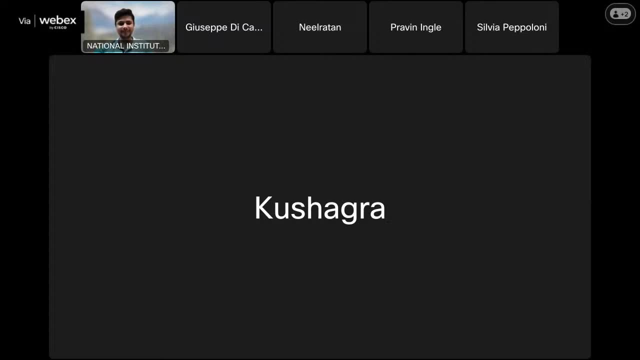 Why not you give the closing remark? Okay, I can also give closing remarks. First of all, I am thankful to Suvir Prakash sir for his guidance Program was very good. All speakers given their talks in very informative way, And it was. 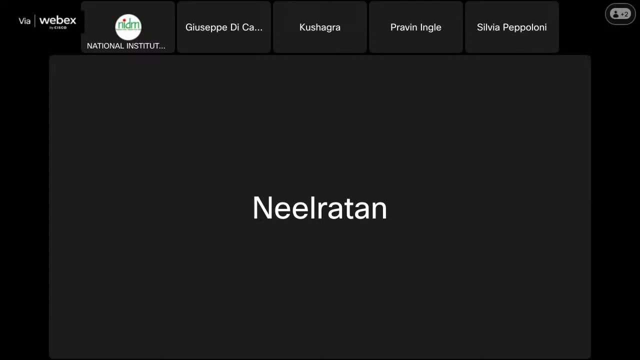 very informative program. By this program we are able to know about geo-ethics, geo-heritage, geo-tourism and geo-conservation and broadly we got sense about geo-heritage, geo-conservation and geo-ethics. 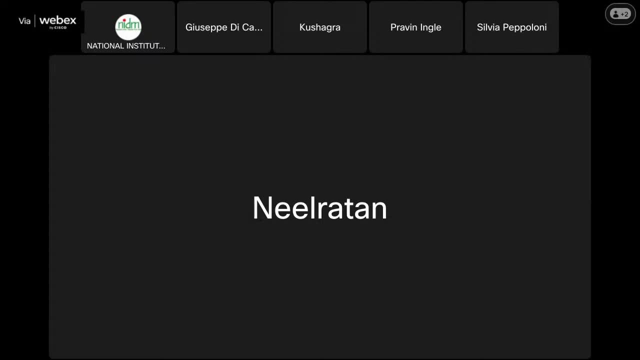 So I am thankful to each and every one and all speakers, and all at each. So thank you very much. I have a request to host, if few are there also can on the video so that we have a screenshot. Yes, So request all the panel. 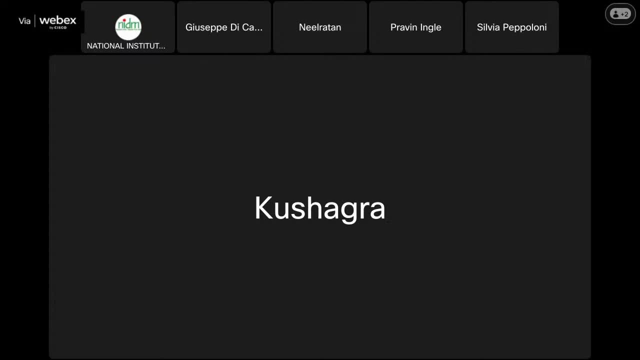 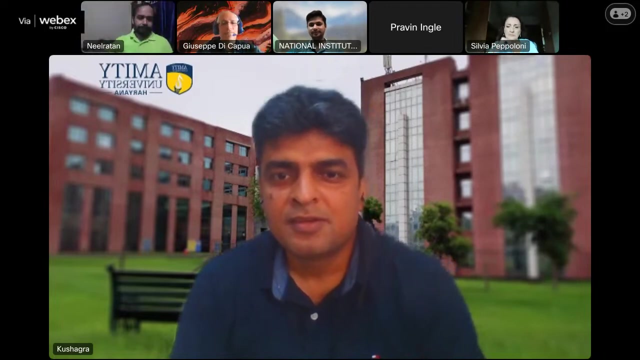 so that open their video and you have a screenshot. So one please request. I also request to all the speakers to open the video. Praveen is there, Yes, Neel Ratan, you also. So this is possible. Okay, that's great. Now, sir is also. 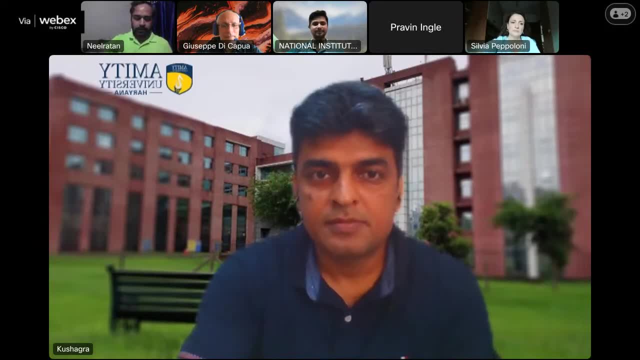 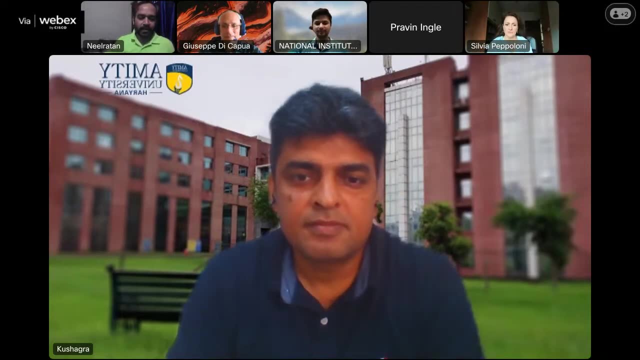 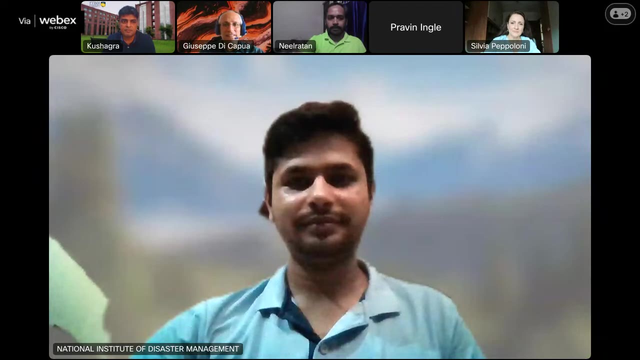 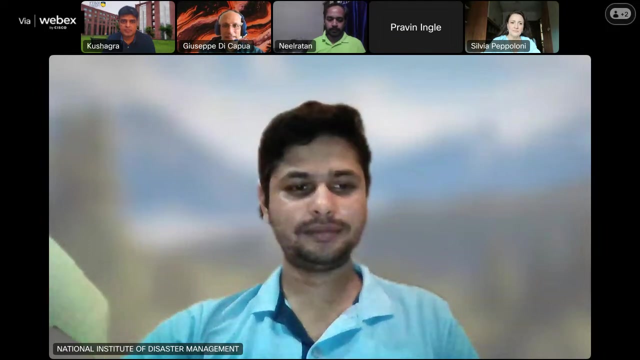 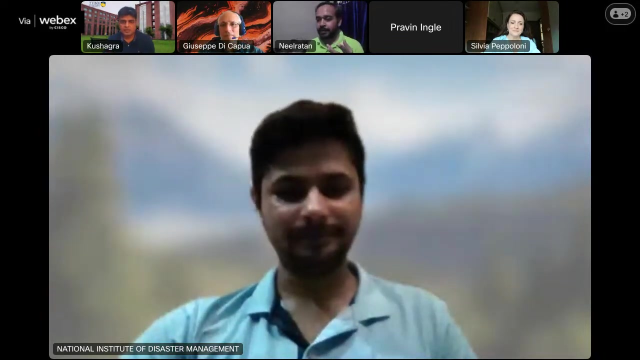 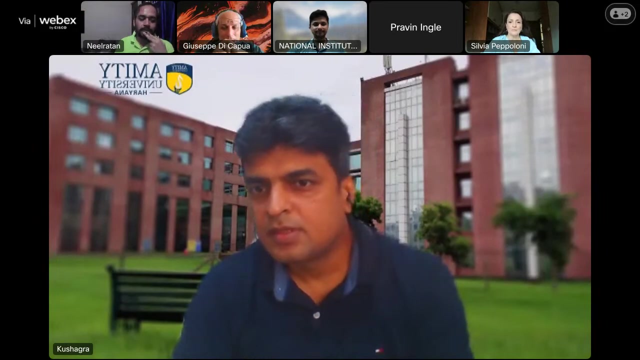 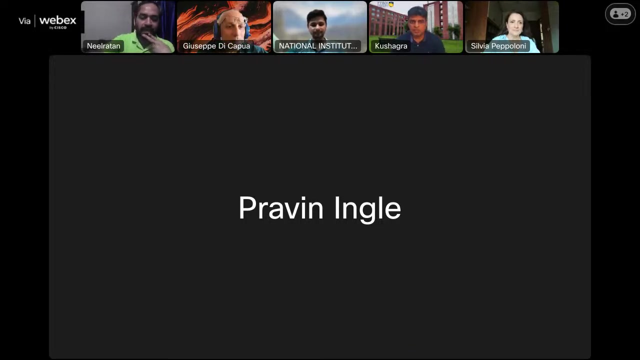 there. So I am taking print screen. you can also take print screen of this. Yes, sir, I think sir is not here. Thakkar sir is not here. Thakkar sir may left, I think. Okay, Okay, Okay, So it is. 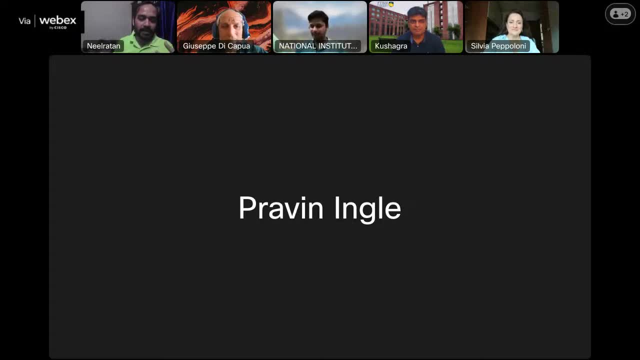 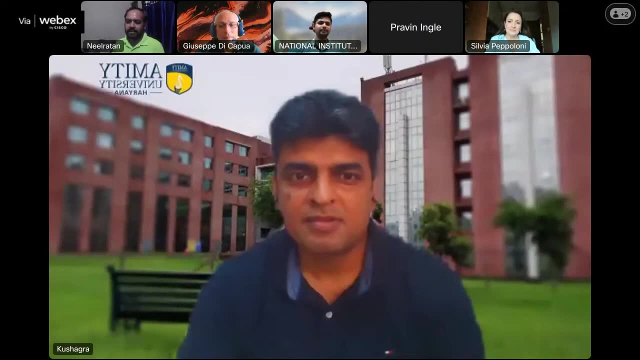 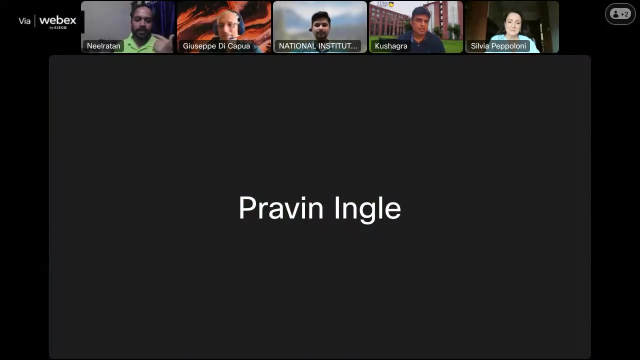 time to say goodbye, English, sir. please open your video. Yes, sir, Just a minute, Just a minute, Just a minute. Start video. Video start. Okay, Not possible. No, I think there is some issue. technical issue: Okay, no problem. No, this is time to say goodbye. 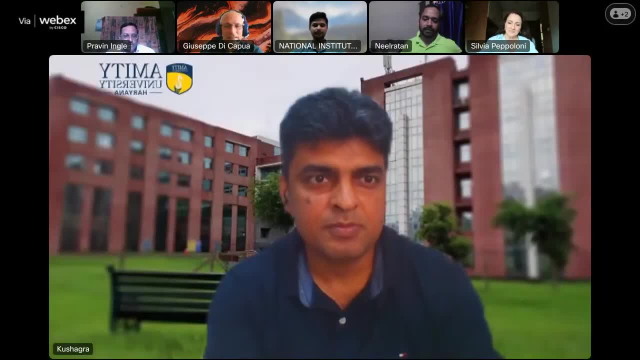 Bye, bye, Thank you. Thank you all for the. Okay, Oh, now he is here. So my pranam to everyone. Thank you for this opportunity. Thank you very much, sir. Thanks to all of you, Thank you, Goodbye to all. 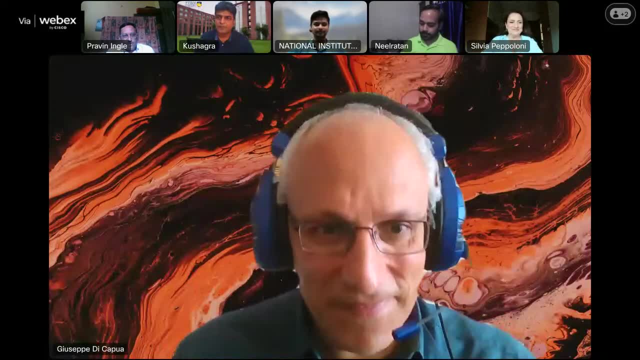 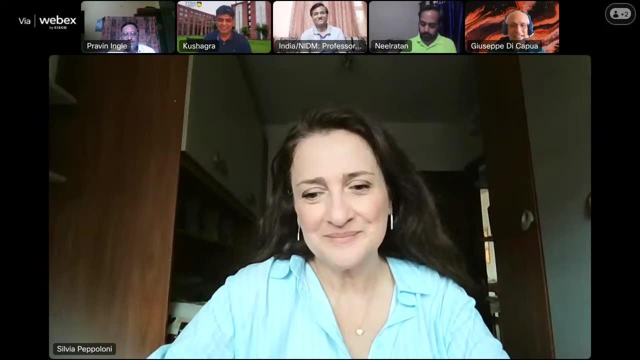 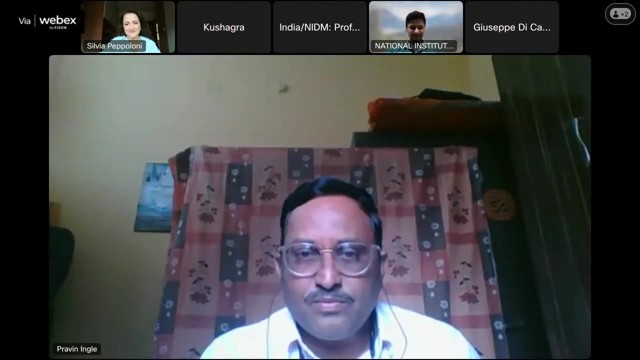